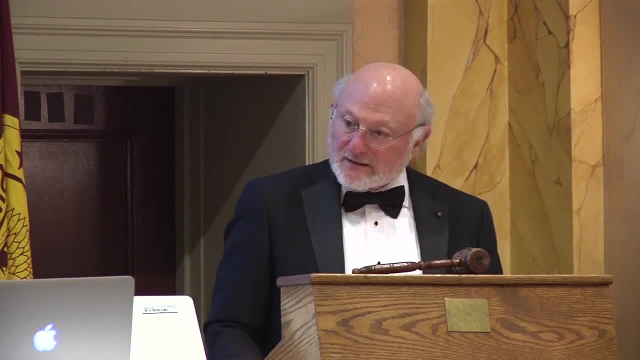 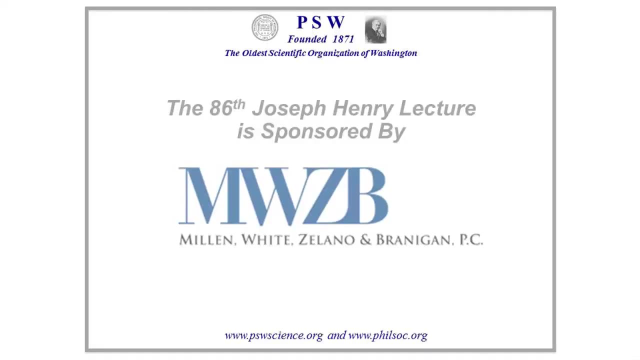 and a generous, anonymous donor. In addition, tonight's Joseph Henry Lecture is sponsored by Mill & White, Solano and Brannigan. You may wonder why a law firm is sponsoring a science lecture. Well, I do. Well, I happen to be a partner at that law firm. 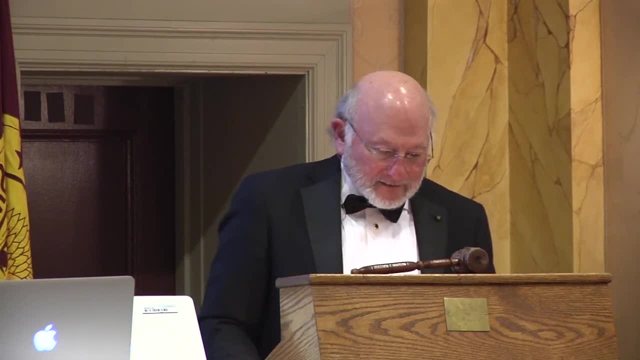 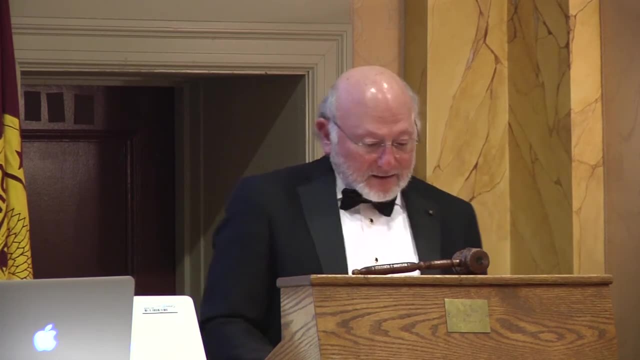 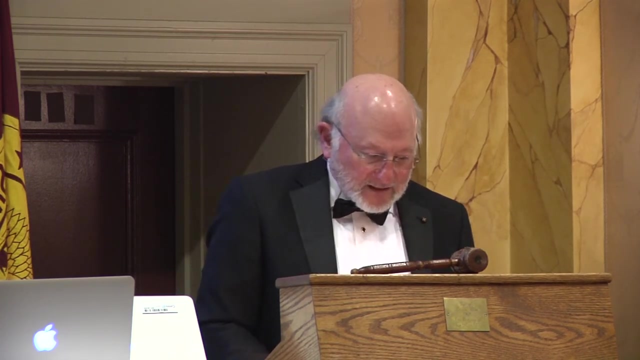 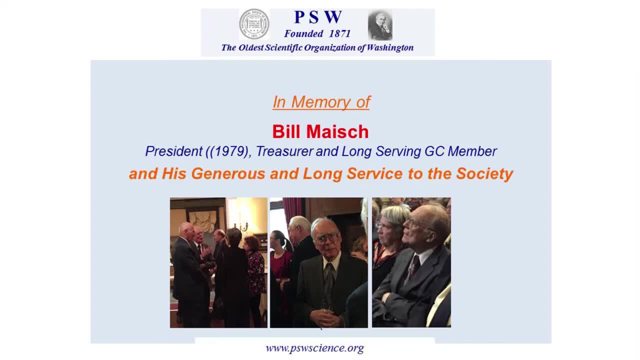 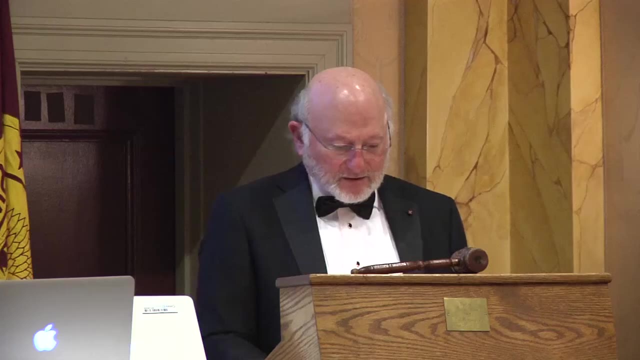 and he served the society in many roles over that time. He was president of the society in 1979, and was a member of the general committee in one capacity or another from the time I joined PSW about 12 years ago until this year. 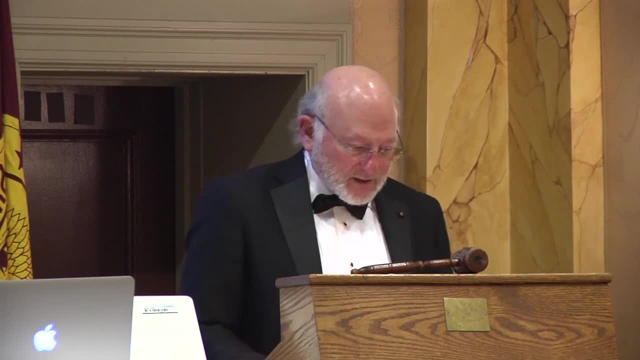 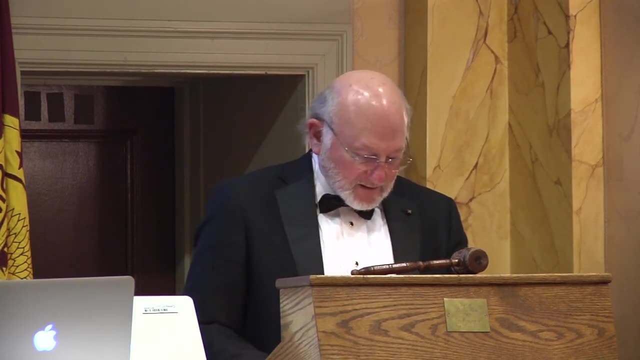 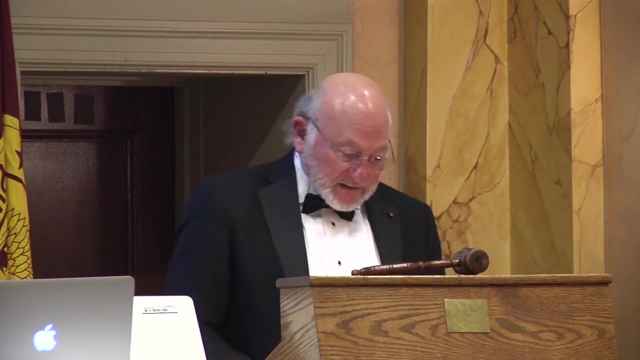 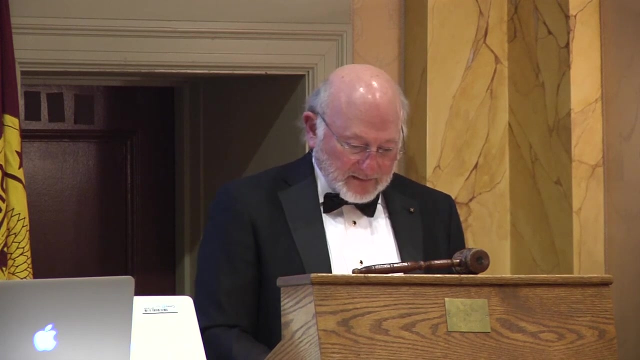 It's a small consolation that we were able to honor and celebrate Bill earlier this year at the 2374th meeting on 24 February, and we'll greatly miss him. I am pleased to announce that the following new members have been elected: Karen Jones, clinical director at Lantern Mental Health Center. 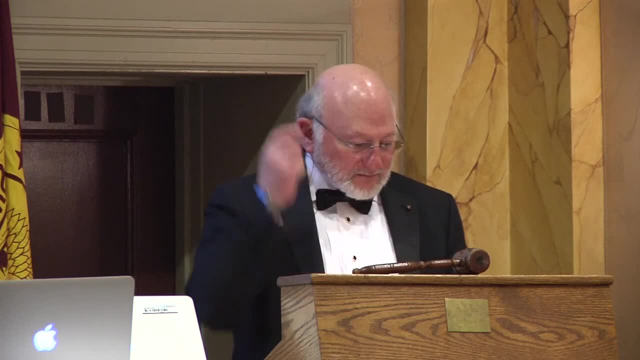 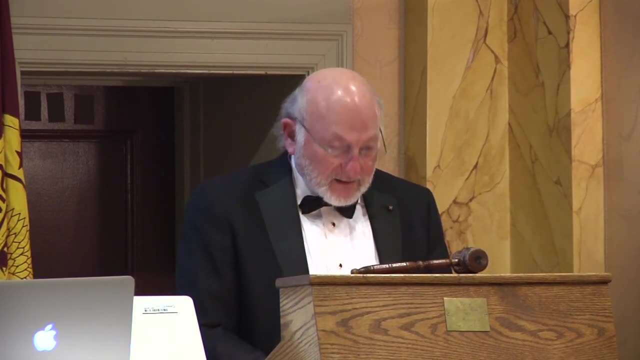 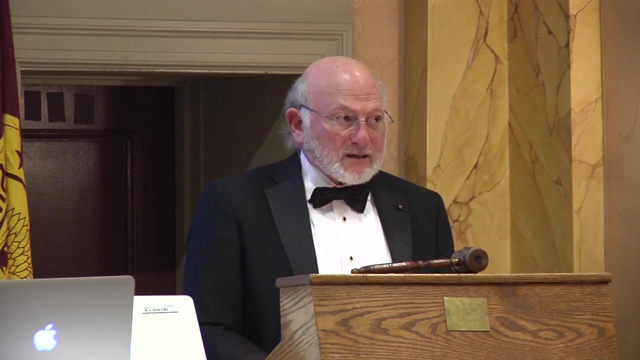 and an attorney interested in astrophysics, cosmology and genetics who found PSW on the web. Dennis Miller, CEO and president of science and technology international, interested in molecular biology, astronomy, physics, energy and environmental sciences and policy. 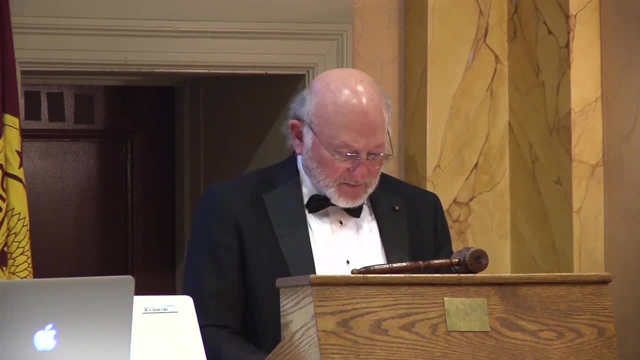 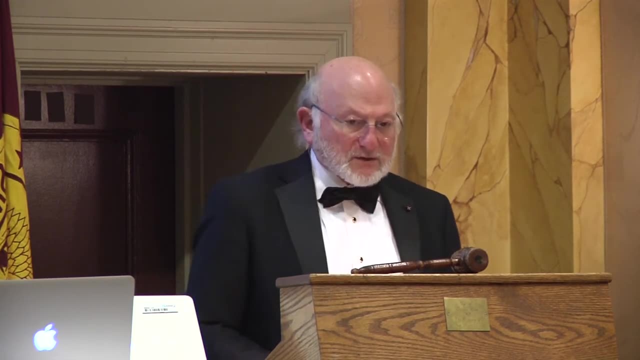 who comes to PSW through friends in the Cosmos Club And tonight's speakers: Deborah Fisher, professor of astronomy and geology and geophysics at Yale University. Hannah Ruth Wakefield- sorry Wakeford- postdoctoral fellow science and exploration directorate at NASA, Goddard. 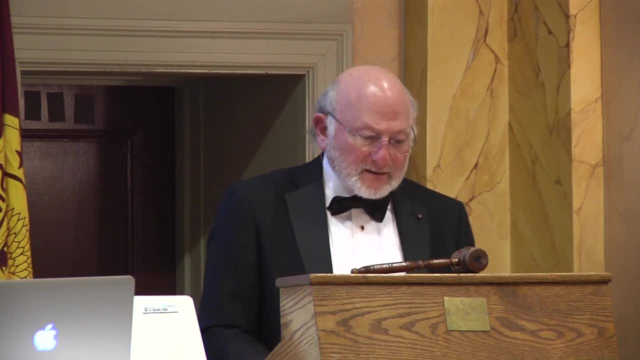 space biology and geophysics. Thank you, Sean Domigold-Goldman. scientist at the sciences and exploration director at NASA, Goddard SFC. Eki Rogerge, astrophysicist in the exoplanets and stellar astrophysics lab. 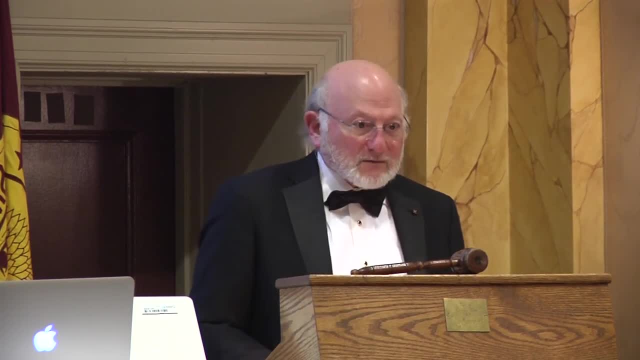 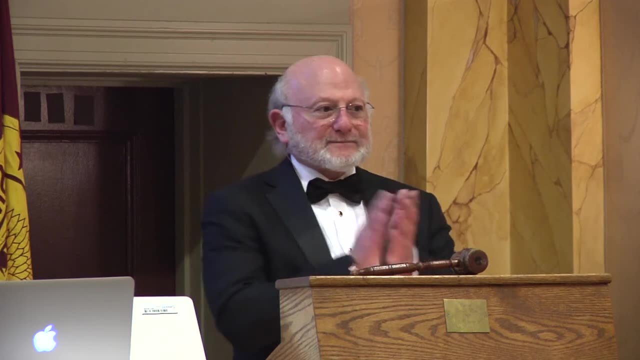 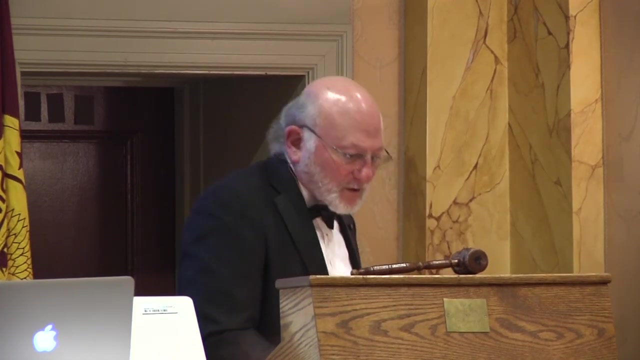 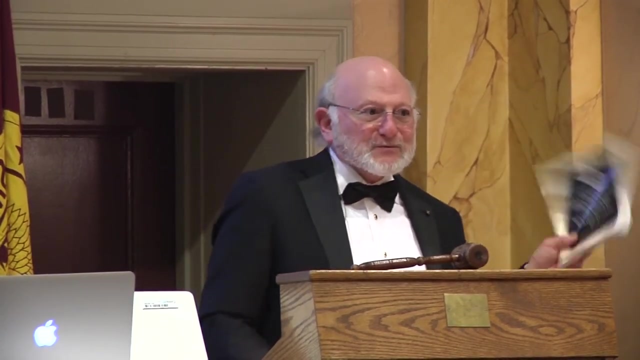 at NASA Goddard Space Flight Center and Mark Clampin, but he's already a member of PSW. Please join me in welcoming them to the society. Thank you. All new members and members who did not previously get a copy are invited to come up to the front of the room. 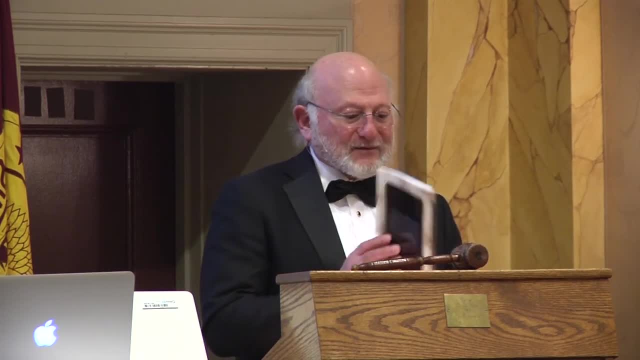 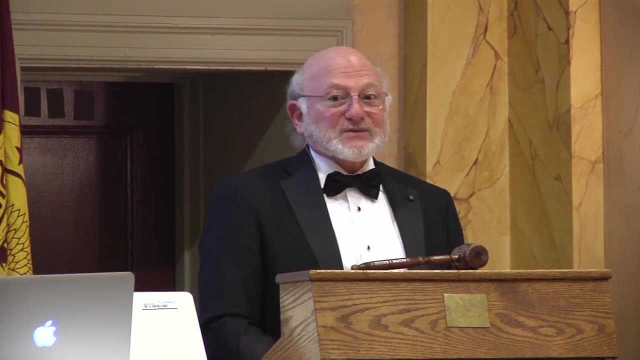 and get their personally autographed by me, copy of Viomon of the Bulletin on the Philosophical Society of Washington, where you can read why the Philosophical Society of Washington is named the Philosophical Society of Washington and understand a little bit why we are trying to do this. 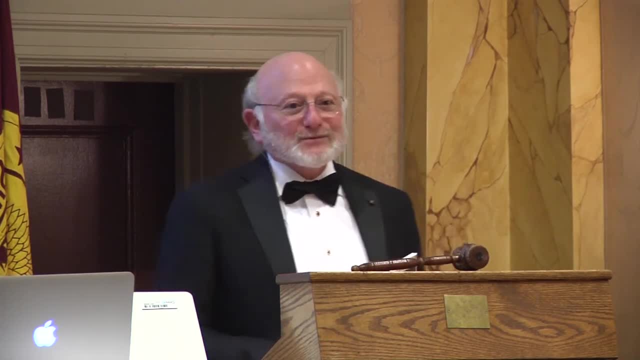 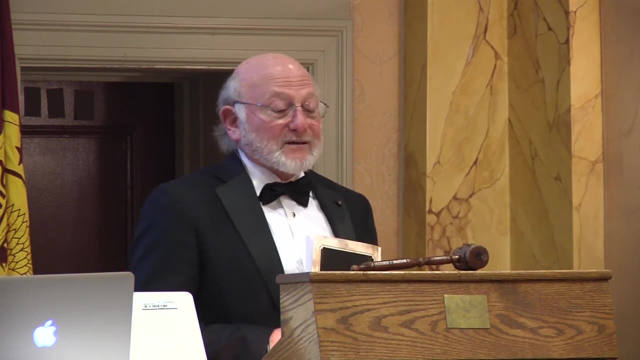 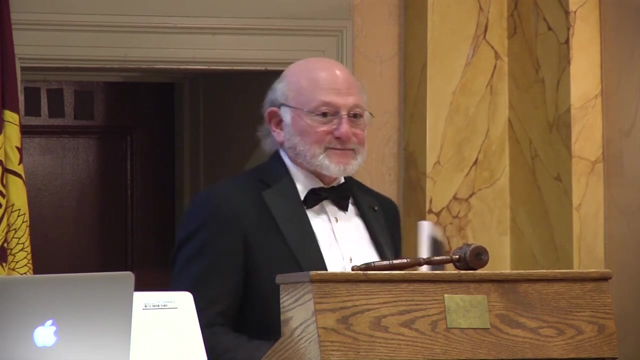 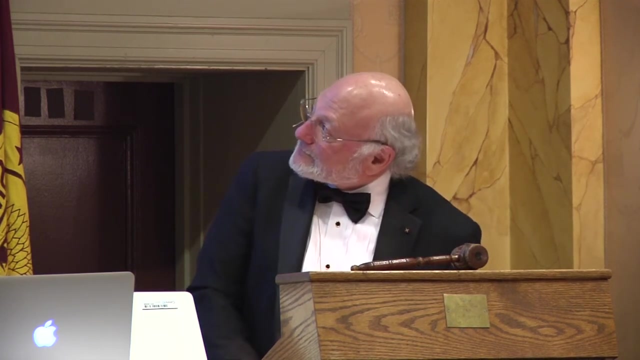 I'm going to kind of convince people to call it PSW or PSW science. It has always been about science, but back then philosophy meant natural philosophy to these founders, and natural philosophy was the term for science. Recording Secretary Preston Thomas. 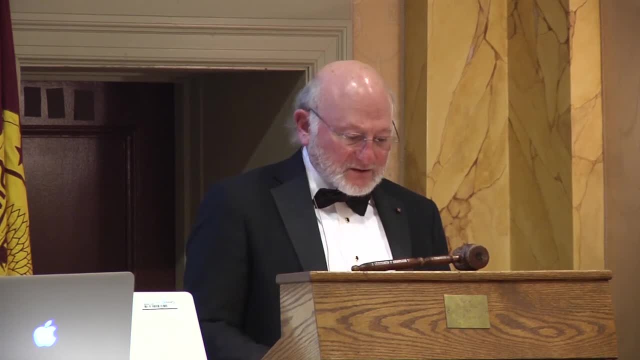 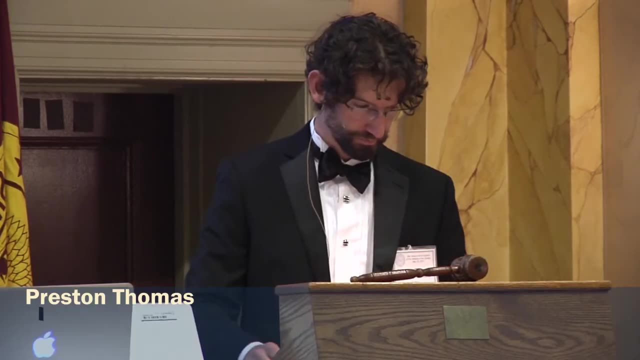 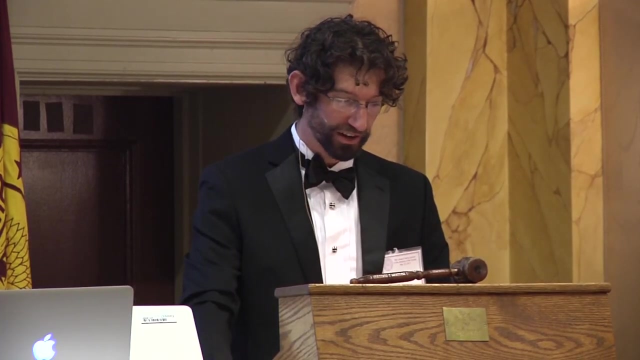 we'll now read the minutes of the previous meeting's lecture on malaria, CRISPR and gene drive by Tony James. At the Cosmos Club in Washington DC on April 28th 2017, President Larry Milstein called the 2,378th meeting of the society. 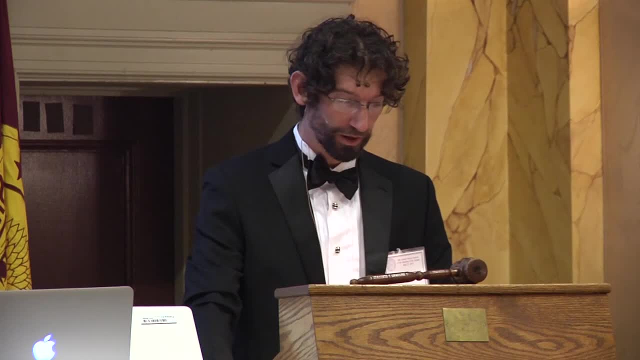 to order. at 8.11 pm, He announced the order of business and welcomed new members. President Milstein presented a summary of the 37th meeting of the society held in 2018.. The minutes of the previous meeting were read and approved. 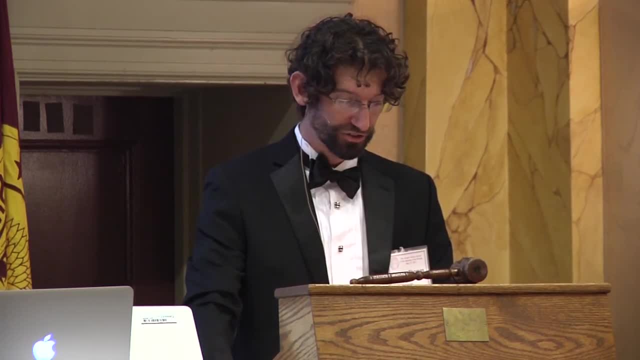 President Milstein then introduced the speaker for the evening, Anthony A James, a distinguished professor in the Departments of Microbiology and Molecular Genetics and Molecular Biology and Biochemistry at the University of California, Irvine. His lecture was titled The Mosquito: Synthetic Biology, CRISPR and Malaria. 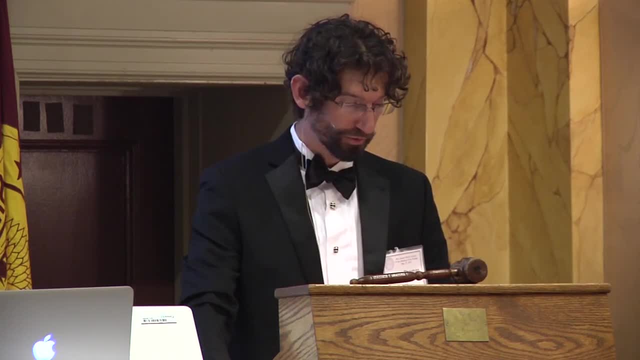 Dr James began by explaining that malaria has afflicted humans for all of recorded history and that it has affected humans for all of recorded history, and that it has affected humans for all of recorded history, with references to deadly recurrent fevers appearing in Mesopotamian cuneiform in 6,000 BC. 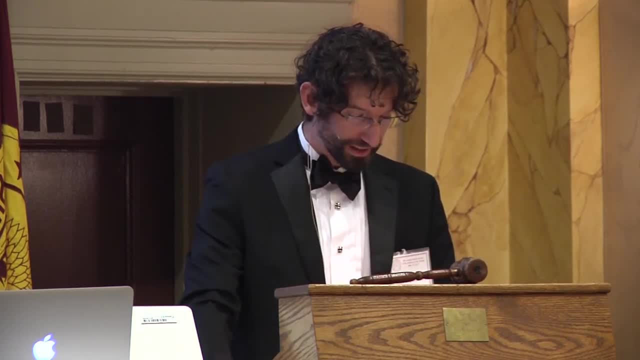 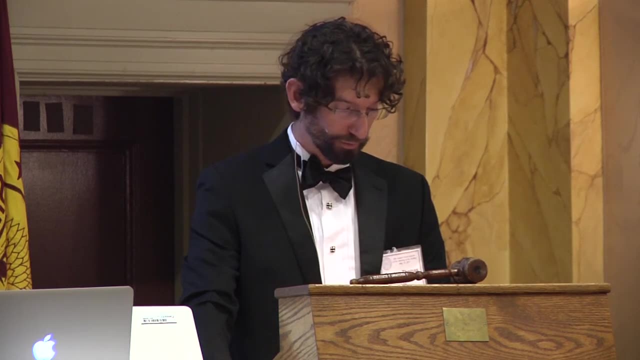 The famous Greek physician, Hippocrates, noted the link between swampy waters and fever cycles. Malaria is a blood-borne infectious disease resulting from a protozoan parasite that is transmitted by mosquitoes. Today, there are five species of malaria parasite that affect humans. the newest of which crossed over two humans within the last 50 years. The two species most deadly to humans are Plasmodium falciparum and Plasmodium vivax. Importantly, there are no free-living forms of the parasite. 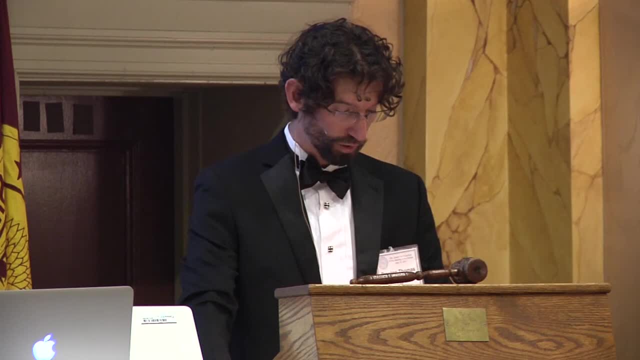 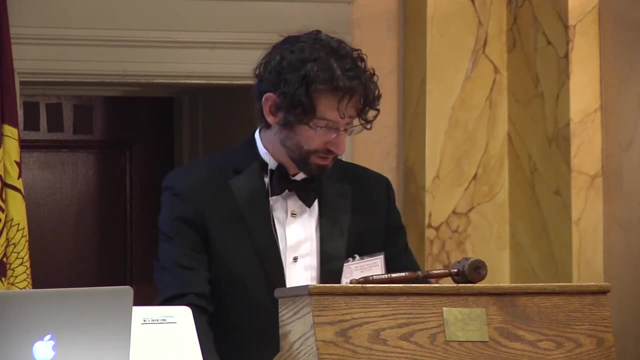 It exists only inside a suitable host. Malaria is only spread by adult female mosquitoes which feed on blood as a source of protein for nutrition and egg production. Malaria today is endemic in the poorest countries in the world, existing in all tropical and subtropical regions. In 2015,, there were 212 million- 20 million cases worldwide, resulting in approximately 429,000 deaths, 90% of which were in sub-Saharan Africa. Although we have many tools that are effective against malaria, including bed nets, spraying, eliminating standing water, 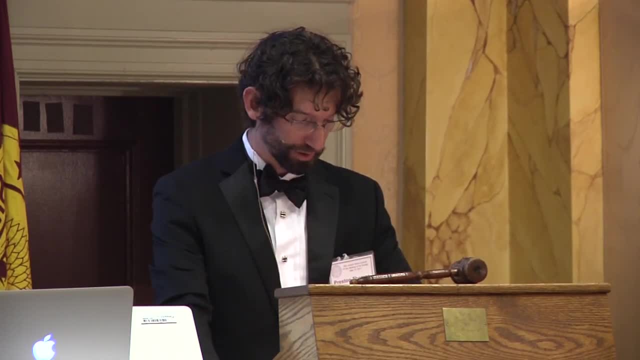 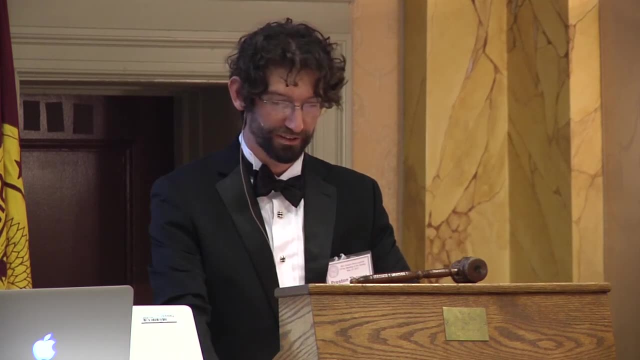 and anti-malarial drugs. for various practical, economic and political reasons, these tools have been insufficient to control malaria in many countries. To date, no effective vaccines have been developed against any protozoan parasite, including malaria. Dr James then described a promising new strategy of 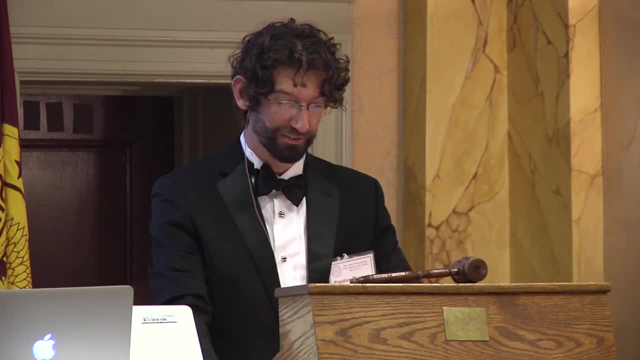 engineering mosquitoes with genes that prevent the transmission of the malaria parasite. To do this, scientists first search for mosquito genes that are activated when the mosquito feeds. They found suitable genes related to digestion. Next, they identified a gene in mice that reacted very strongly to human 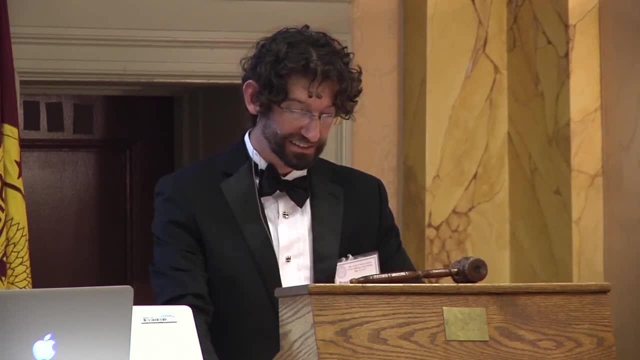 strains of the malaria parasite, neutralizing it. Splicing this mouse gene into a mosquito creates a transgenic mosquito that expresses antibodies in the mid gut and the salivary gland every time the mosquito feeds, curing the mosquito and eliminating transmission back to humans After developing a. malaria immune mosquito. the next task is to distribute these genes throughout the mosquito population. This can be done simply by breeding and releasing millions of mosquitoes, but a more effective strategy is to include a gene drive in the engineered mosquitoes: DNA that is Ensures that the anti-malarial genes are preferentially inherited when the mosquito breeds. 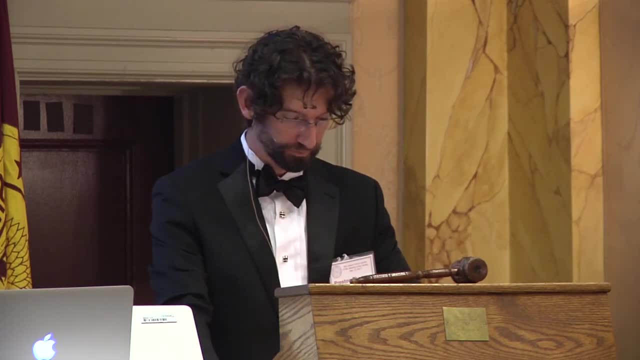 overriding the traditional Mendelian inheritance patterns. The creation of a gene drive is possible because it advances in the use of CRISPR Cas9 gene editing system, Which consists of the Cas9 nuclease, which cuts DNA, plus guide RNA, Which targets the cuts to a precise position in the mosquito DNA sequence. 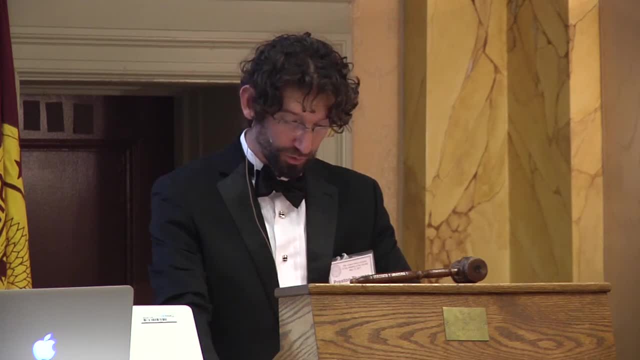 When the cell attempts to repair the cuts to its DNA. The most available model for reconstituting the cut section is the lab created plasmid containing the anti-malarial mouse gene. moreover, this engineered sequence also contains the coding for the Cas9 nuclease and got guide RNA. 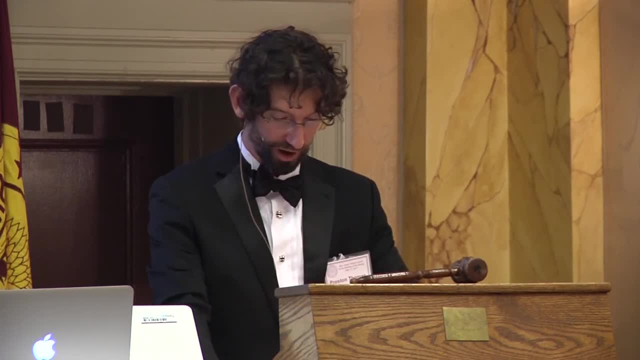 Which means that the repaired DNA will copy itself autonomously to the other unmodified chromosome, creating mosquitoes that have a 100% chance of passing along the engineered genes. Dr James explained that, in addition to the functional Parts of the engineered plasmid, plasmid, the nuclease guide, RNA and the malarial resistance sequence. 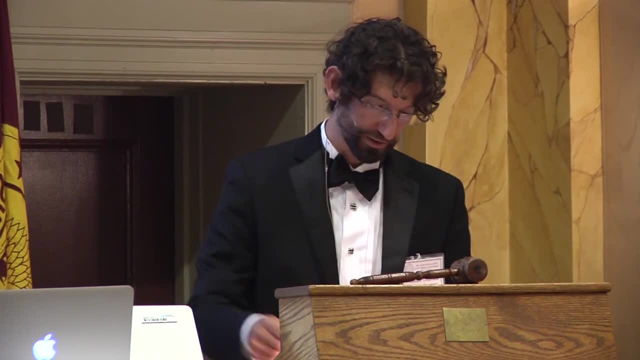 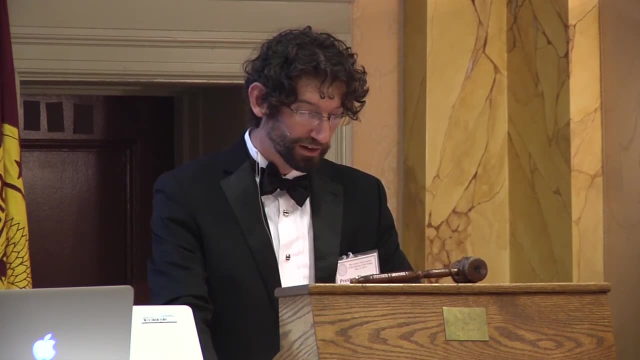 It also contains a protein for red coloring derived from a jellyfish that allows engineered mosquitoes to be readily distinguished from wild mosquitoes. Dr James noted that drugs, insecticides and vaccines all have well-established regulatory pipelines from discovery to development to delivery, But genetics based vector control does not. 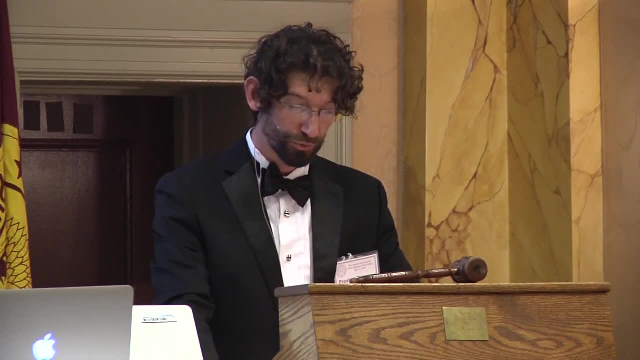 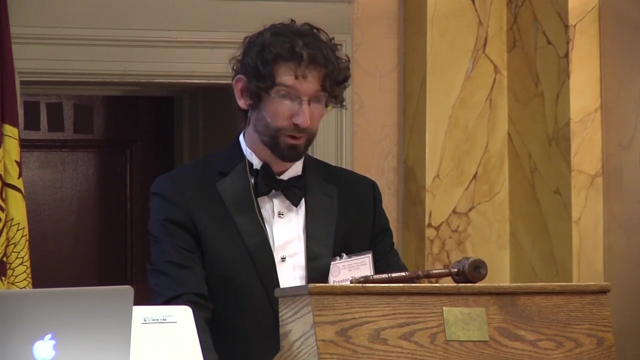 nonetheless, Dr James expressed confidence That carefully constructed, rigorously conducted phased trials will demonstrate to regulators, governments and communities The genetically engineered mosquitoes are safe and affect effective malaria control strategy that, when combined with existing tools, Could ultimately enable world health authorities to finally eradicate malaria. After the conclusion of the lecture, president millstein invited questions from the audience. 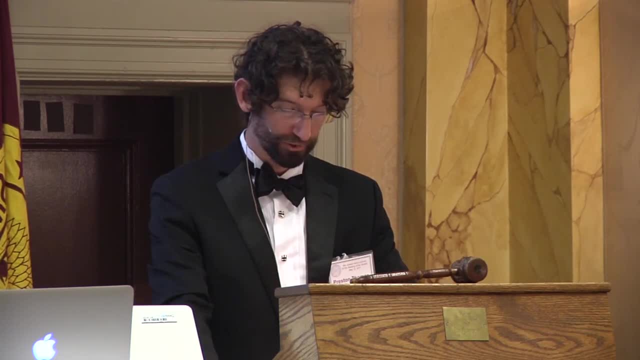 One questioner asks how the mouse gene confers malaria resistance in the mosquito. Dr James explained That the engineering conforms confers two forms of resistance. first, It creates antibodies that bind to surface proteins on the parasite the parasite uses to invade host cells. The second: in the second method, it simply coats the surface of the parasite in antibodies, preventing it from interacting with the host cells. 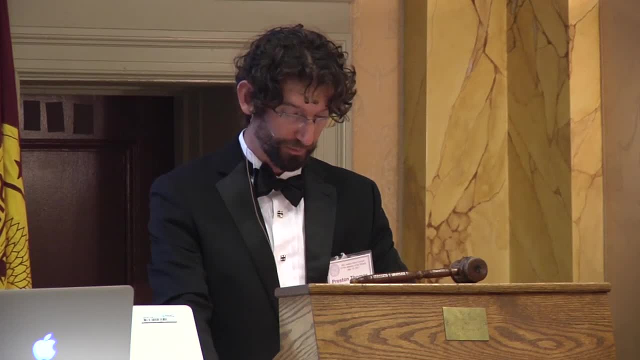 Another questioner asked why the engineered mosquito use genes from Matt, from mice antibodies and not human antibodies. Dr James explained that human resistance acts Only during the human blood cell stages and does not provide complete protection. So the mouse gene was chosen to target malaria completely and at the point of transmission. 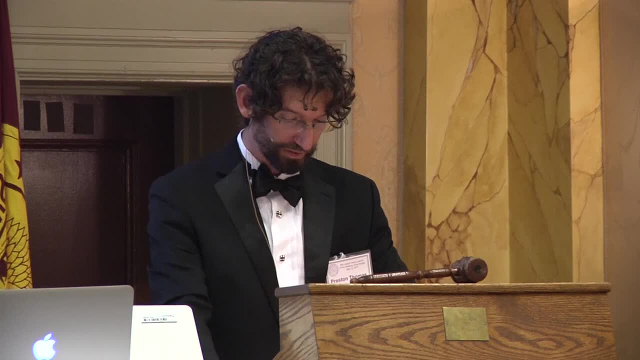 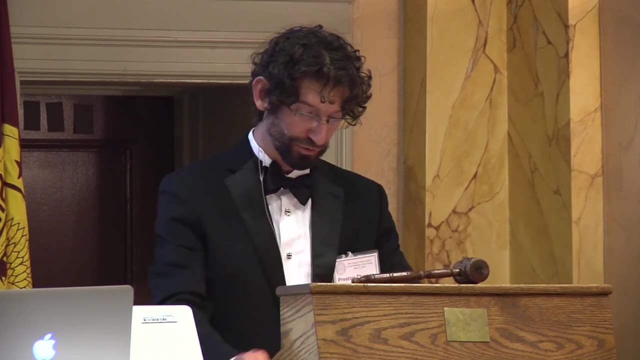 after the question-and-answer period: President millstein thanked the speaker, made the usual housekeeping announcements and invited guests to join the society. at 9: 59 pm, President millstein adjourned the two thousand three hundred and seventy-eighth meeting of the society to the social hour. 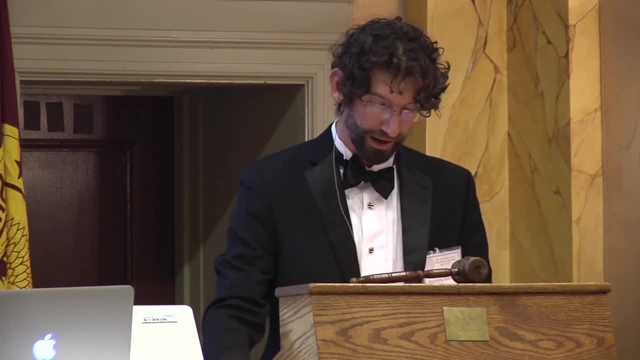 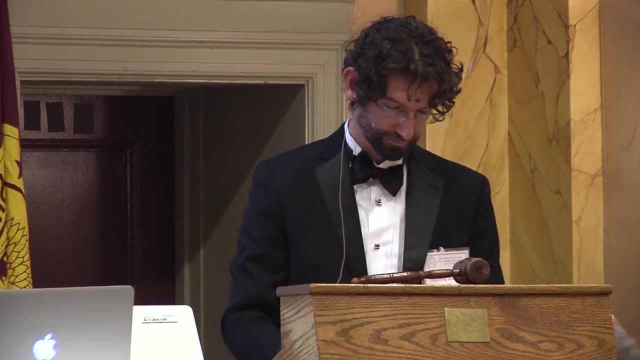 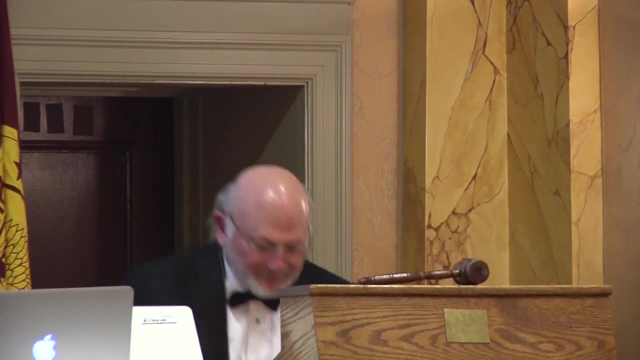 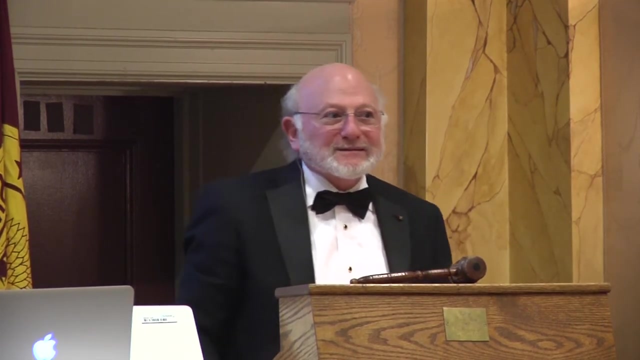 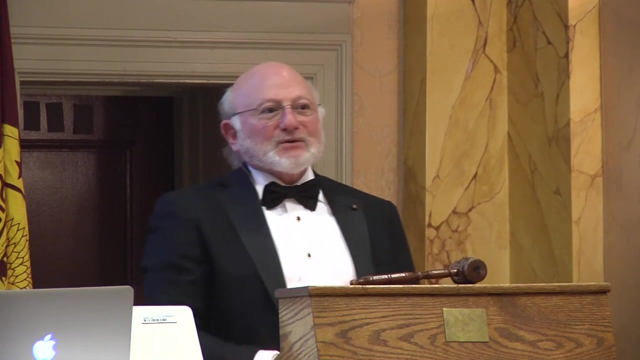 temperature: 24 C. weather: partly cloudy. attendance: 105. Respectfully submitted: Preston Thomas, recording secretary. Thank You, Preston. are there any questions, comments, corrections, additions to the minutes? If not, I will entertain a motion from a member to accept the minutes as read: Bob Hershey has motion a member second. 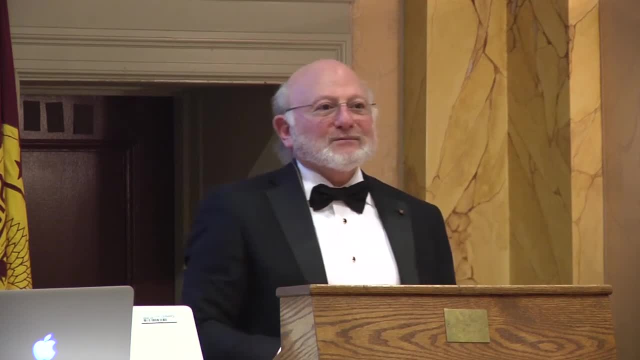 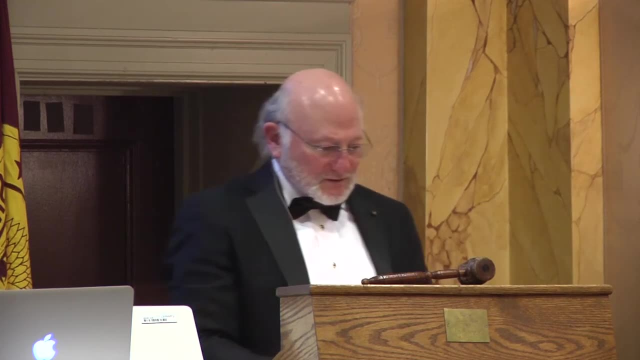 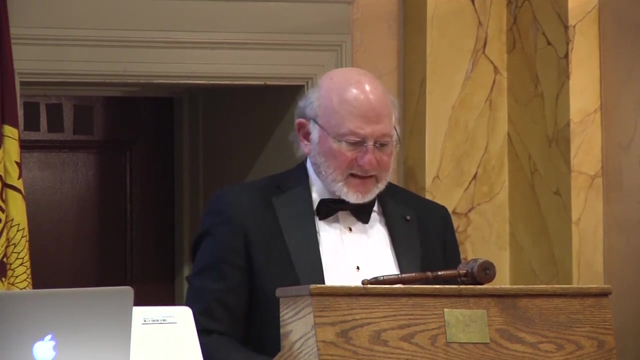 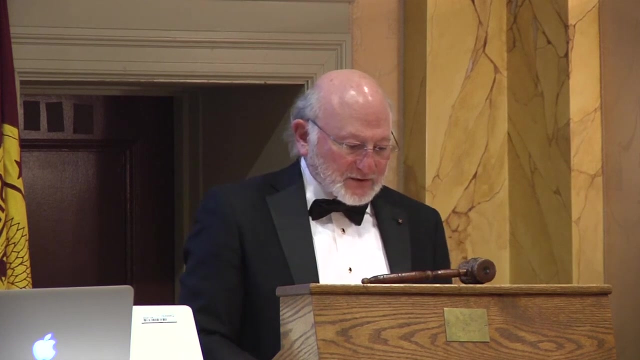 Eric. second. all members in favor. all members opposed. Minutes are accepted as read and will be posted to the website in due course. We now turn to tonight's meeting and the 86th Annual Joseph Henry lecture, which will be in four parts. It's my pleasure to introduce the topic of the lectures. 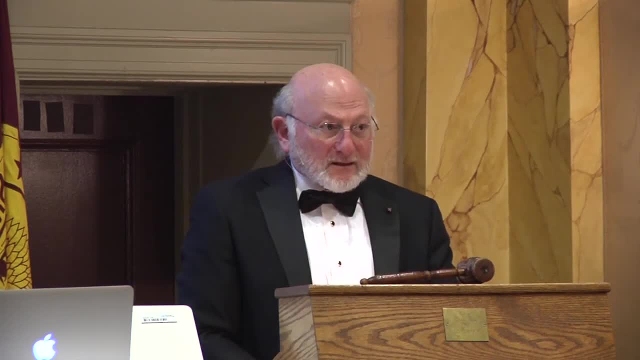 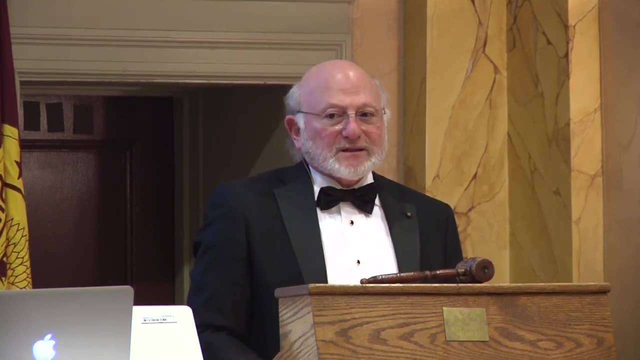 exoplanets in the search for life. just a few decades ago, the idea of planets orbiting stars far from our sun was a commonplace only in science fiction and Scientific circles. their likelihood was debated, with views tightly bound to theories about how stars and solar systems form. 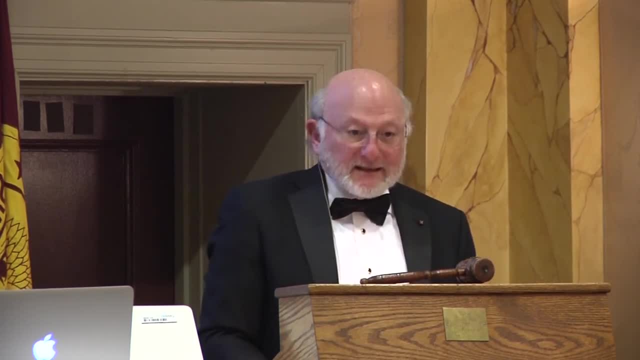 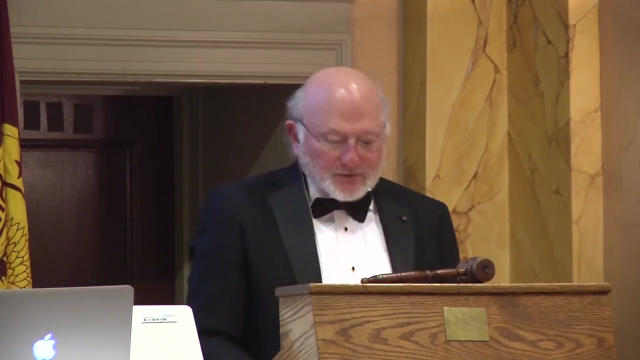 In the three decades since the first reliable report that an exoplanet have been detected, we have seen an explosion of exoplanet identification, Fueled conceptually by knowing that they actually exist and practically by vast improvements in methodology, computational capabilities and instrumentation. as of April of this year, three thousand six hundred and seven exoplanets have been detected in. 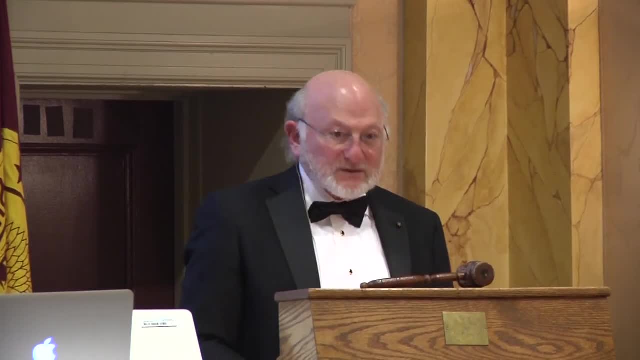 2701 distinct planetary systems, including 610 multi-planet systems and double-planet systems, and approximately. We know that current techniques cannot detect most of the exoplanets. They might exist around all the stars We can observe, and we are also just beginning to detect properties of the exoplanets that we can observe. 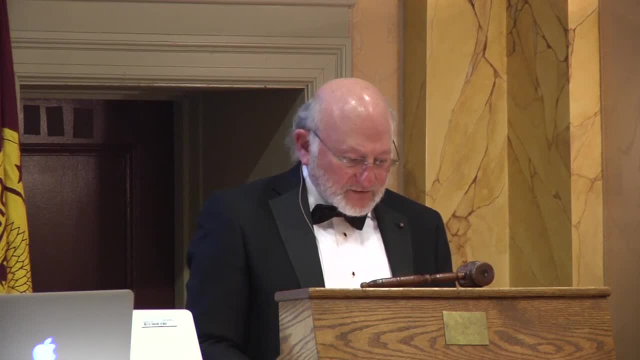 Beyond their mass orbital periods and distances from their sons. We've recently had our first observations of exoplanet atmospheres and a few indications of their composition. Just today, in fact, we read of a publication on the watery atmosphere of an extraordinary Neptune-like exoplanet authored by one of our speakers tonight. can I name it? 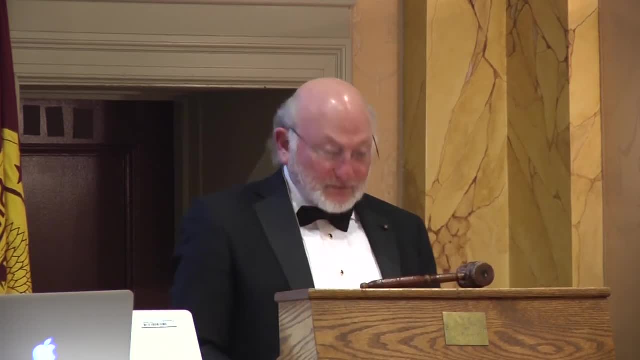 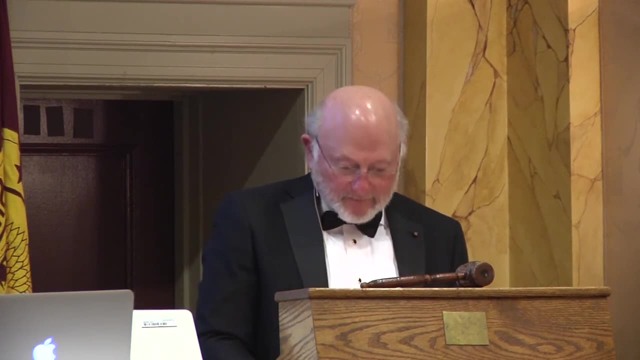 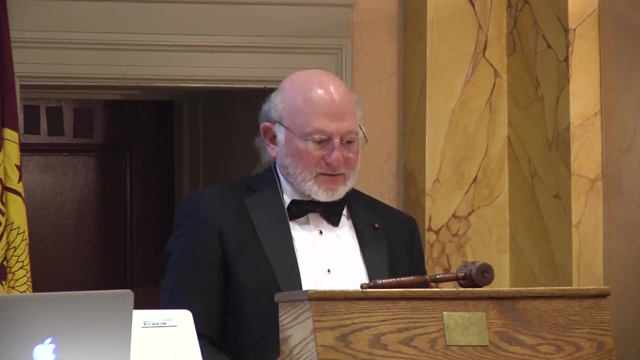 And her colleagues. Eventually- soon, actually, we hope- we will have sufficient resolving power and analytical tools to survey a statistically significant number of exoplanet atmospheres, to have our first empirical understanding of how many Earth-like planets there are that have atmospheres similar to our own and how many of these contain gases that we associate with life. 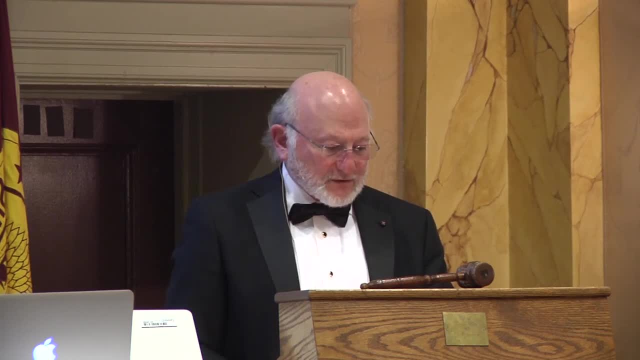 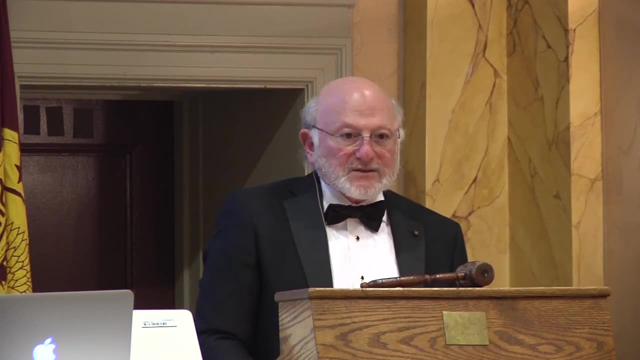 This series of four lectures will: survey our current knowledge of exoplanets, explain the capabilities and limitations of current detection techniques, discuss the TRAPPIST-1 system of planets, Explore prospects for improvement, Improving our abilities to study exoplanets and ways we may be able to find indications. 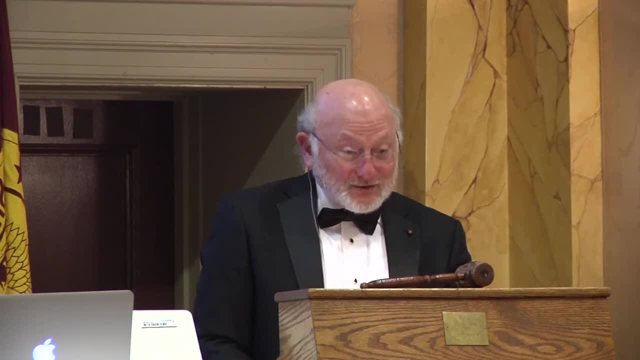 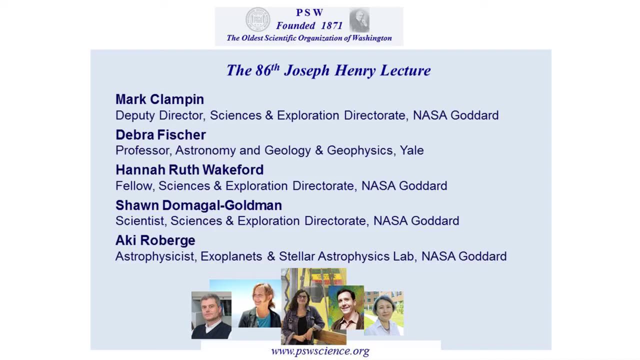 of life and at least tentative answers to the question. are we alone? Our four speakers on these topics will be Deborah Fisher. Hannah Ruth Wakeford, who is the author of the aforementioned paper that came out, I think, this week. Sean Domogold-Goldman. 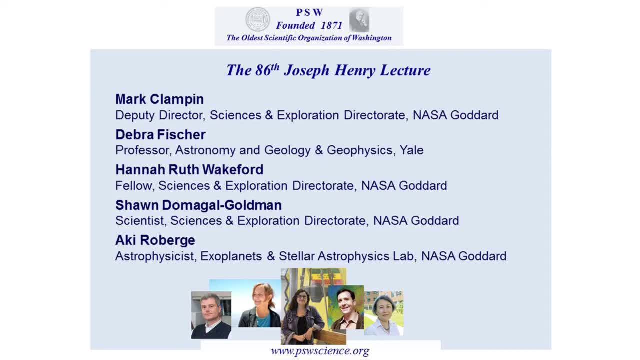 and Aki Roberge, And here to introduce them before their talks is Mark Clampin, Deputy Director of Sciences and Exploration Director at NASA Goddard Space Flight Center. Please hold questions for the question and answer period at the end of the lecture. 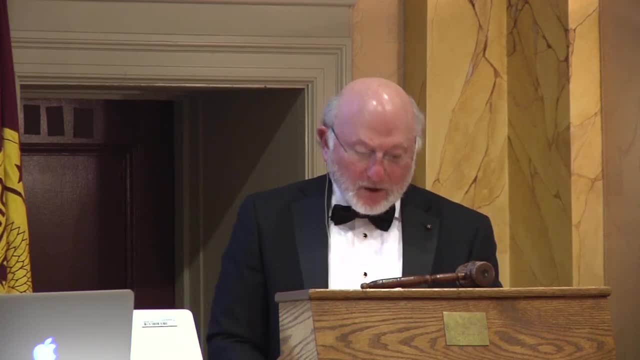 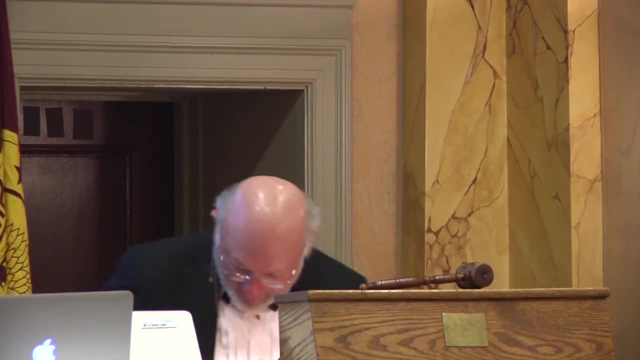 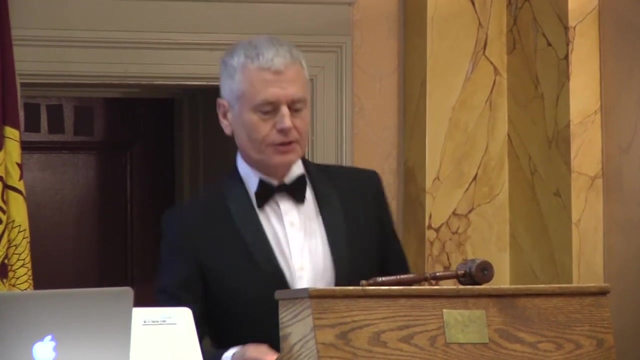 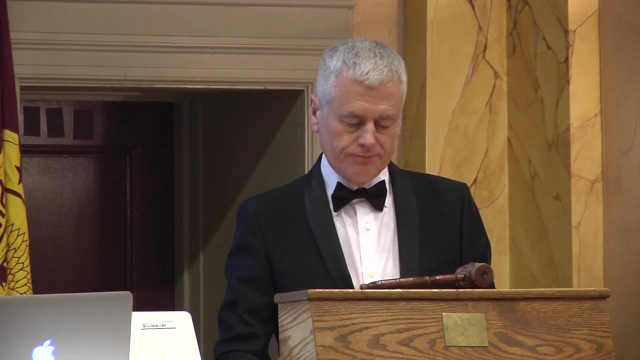 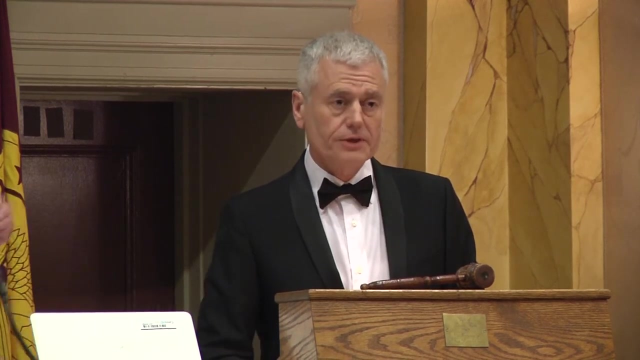 We'll have all of the speakers on the stage together with Mark for free ranging answers to your queries. Okay, good evening. So tonight's talk, as you heard, will be on exoplanets and the search for life. We have four speakers who are all very outstanding speakers and are heavily involved in this. 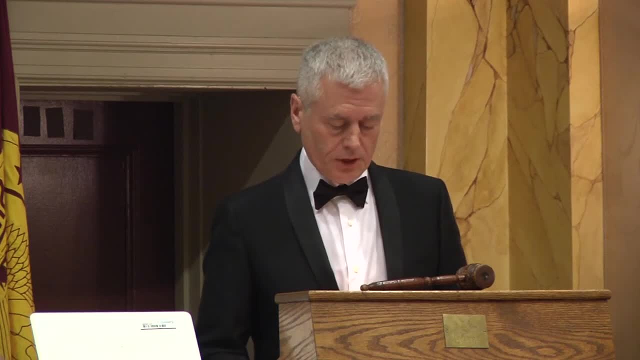 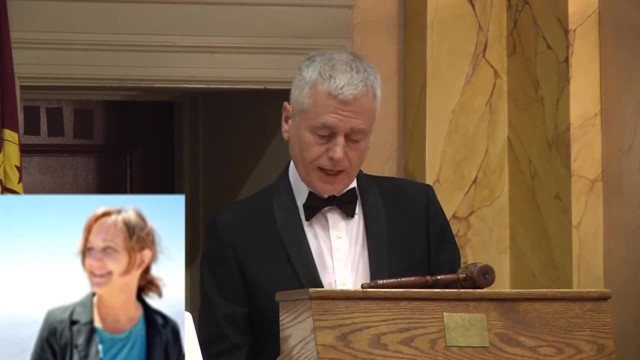 field and have made many of the sort of breakthroughs in this field. So let me start. Our first speaker tonight is Professor Deborah Fisher, and Deborah is a Professor of Astronomy and a Professor of Geology and Geophysics at Yale University. Hello, And a professor of Physics and Astronomy at San Francisco State University. Deborah began hunting for exoplanets in 1997, and she has discovered hundreds of extrasolar planets, including the first known multi-planet system. Among her many honors and awards, Deborah was elected to the SFSU Alumni Hall of Fame. 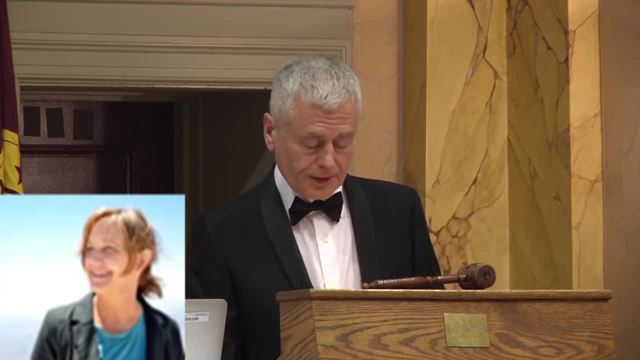 was a Cecilia Payne-Kuboskian lecturer and has been elected to the American Academy of Arts and Sciences And to the Connecticut College of Engineering. Deborah earned a BS and an MS in Physics from San Francisco State University and a 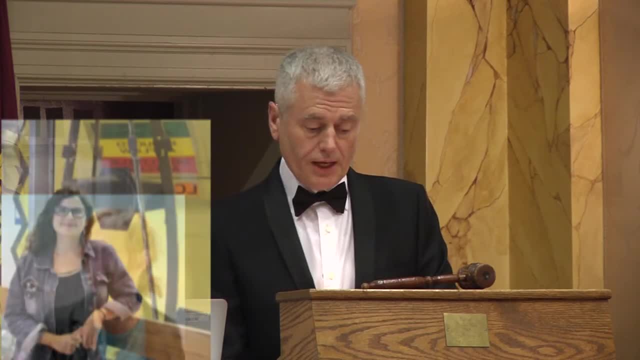 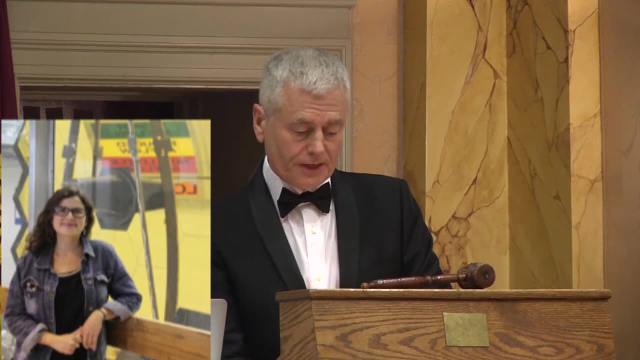 PhD in Astrophysics from UC Santa Cruz. Our second speaker tonight is Dr Hannah Wakeford. Dr Wakeford is a NASA Post-Doc Fellow at the Goddard Space Flight Center, shortly to be a 2017 Giacconi Fellow at the Space Telescope Science Institute. 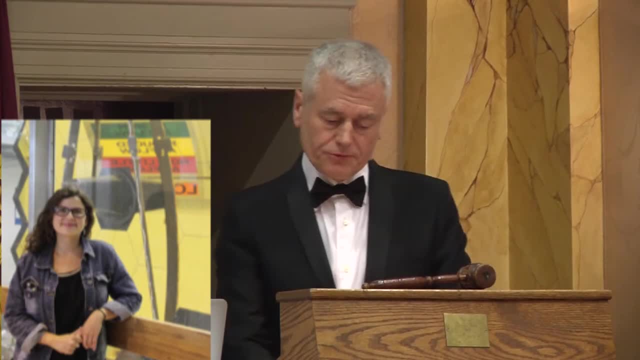 Hannah's work focuses on characterizing the atmospheres of exoplanets through the observations and the search for life With the Hubble Space Telescope, which is now in its 27th year of operation, and Hannah is the recipient of the Robert H Goddard Award for the Individual Scientific Achievement. 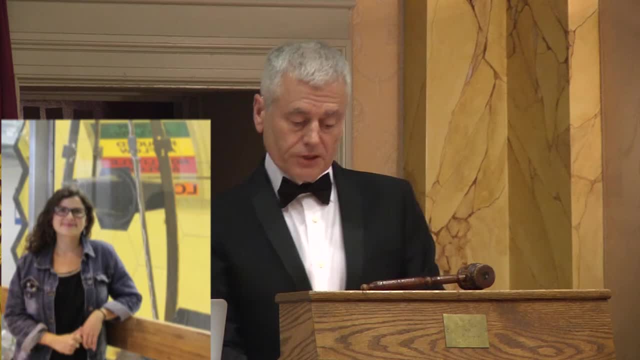 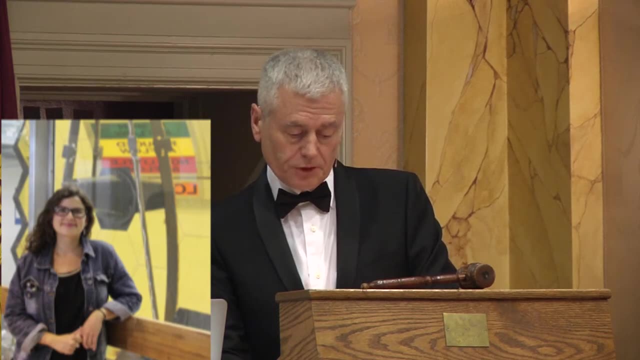 and her work on the TRAPPIST-1 planets. Hannah is an advocate for science communications and she has won a number of awards and commendations. During her PhD, she produced and hosted a weekly live radio show and was a regular 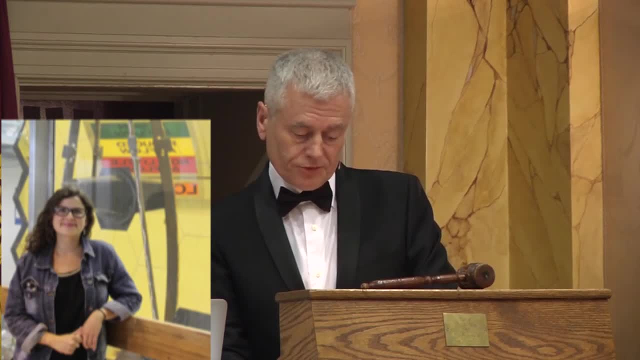 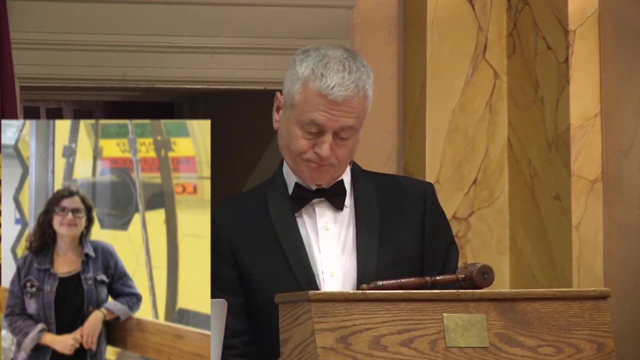 expert guest on BBC Radio Devon and a number of British TV news programs. Dr Wakeford is a professor at the University of New York and has been an expert on the science of communication. She has also appeared on a number of TV shows for the BBC, including BBC Horizon. 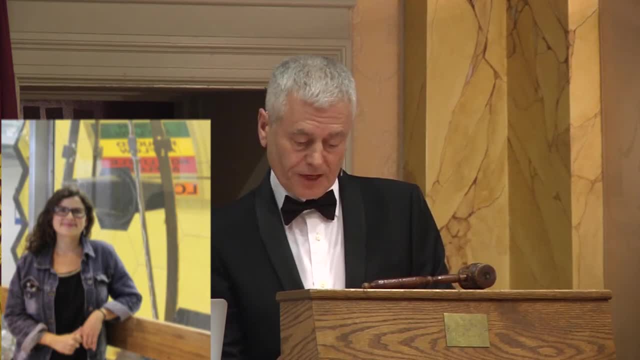 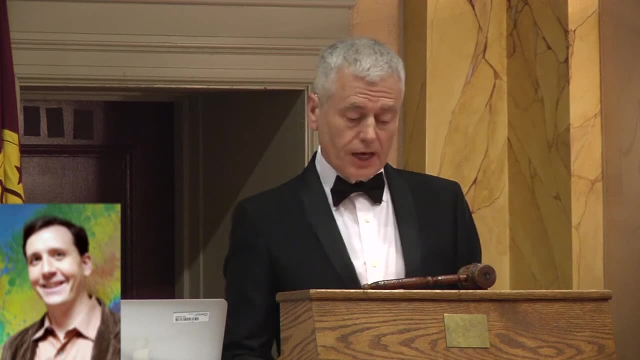 Hannah earned a BS and an MS in Planetary and Space Physics at Aberystwyth University and a PhD in Physics at the University of Exeter. Our third speaker tonight will be Sean Domago-Goldman. 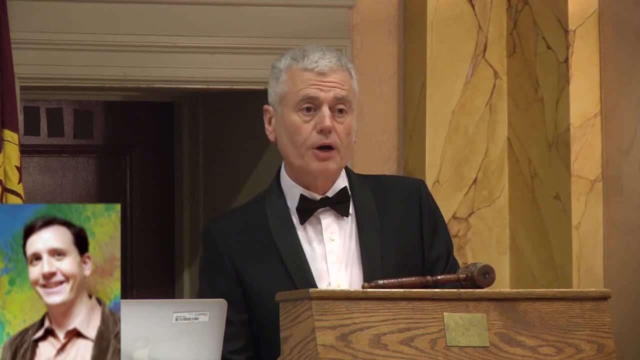 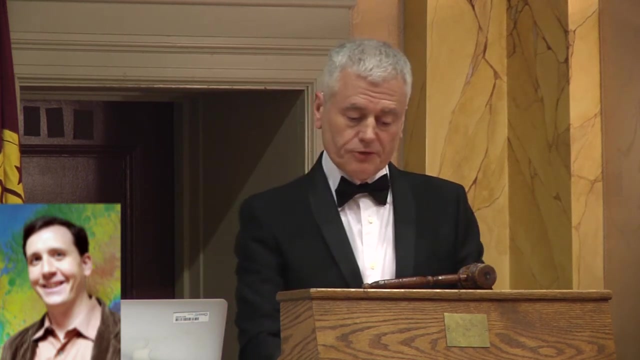 Sean is a research space scientist in the Planetary Environments Laboratory at NASA's Goddard Space Flight Center. He focuses on comparative planetology. As a member of multiple interdisciplinary teams, he simulates the atmospheres of other worlds, including those of ancient Earth, modern Mars, ancient Mars and other exoplanets. 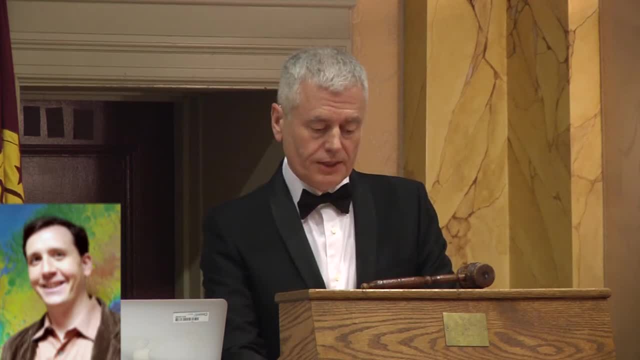 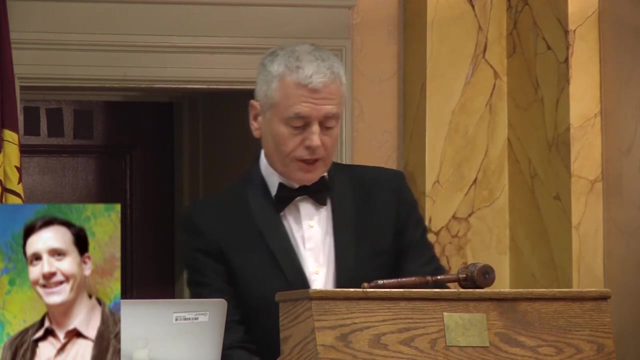 Sean is a member of the Curiosity Science Team, the XOS Science and Technology Definition Team and the HABEX Science and Technology Definition Team. He's also a member of the NASA Astrobiology Institute's Virtual Planetary Laboratory and the Rocky 3D Resolving Orbital and Climate Keys of Earth and Extraterrestrial Environments. 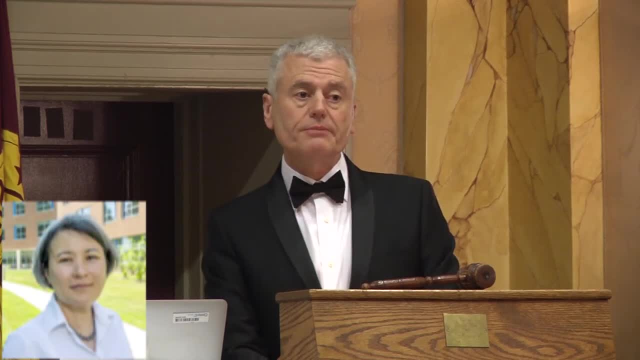 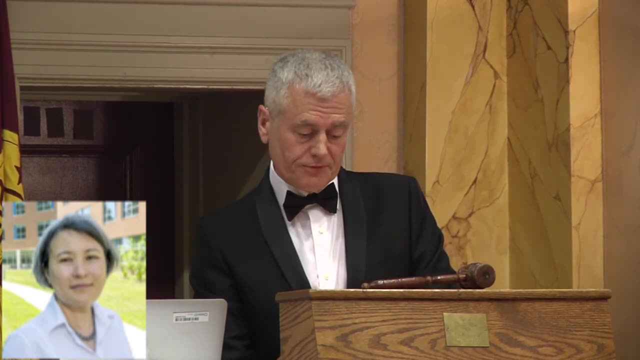 with Dynamics. Our final speaker this evening will be Dr Aki Raberge. Dr Aki Raberge is a research astrophysicist at NASA's Goddard Space Flight Center, and her research focuses on observational studies of planet formation around nearby young stars. 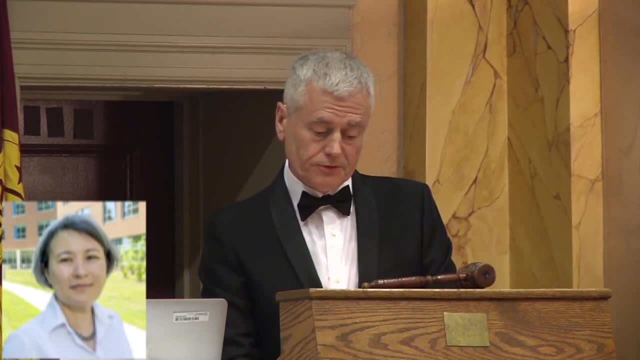 In addition, she's deeply involved in developing future space missions and currently serves as a study scientist for NASA's NASA Space Flight Center. Dr Aki Raberge is also a research scientist for the Large UV Optical Infrared Surveyor Mission known as LUVOIR. 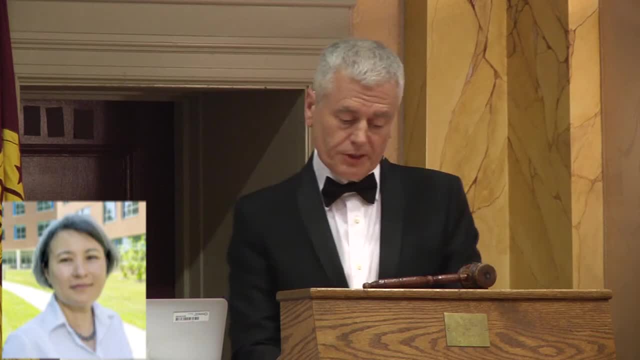 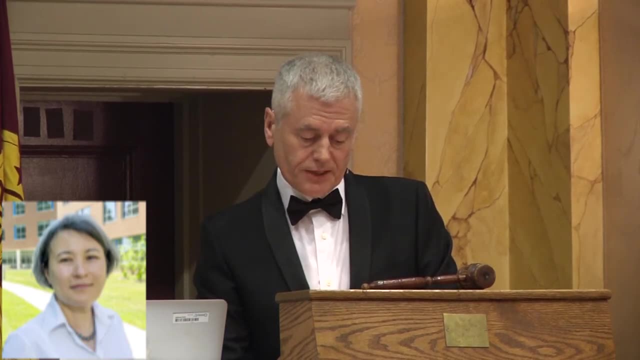 This is a highly capable multi-wavelength future space observatory with ambitious science goals. Dr Raberge received a PhD in astrophysics from the Johns Hopkins University and, after completing a bachelor's degree in physics with a planetary science minor at MIT, she 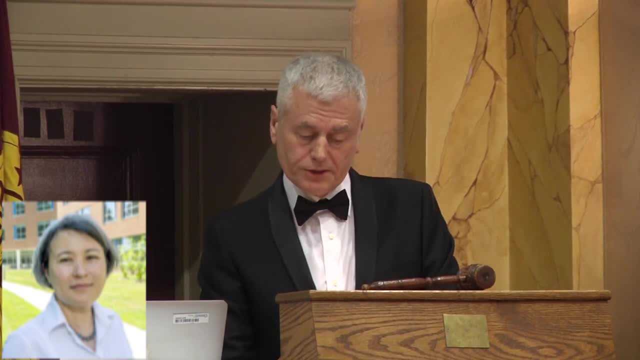 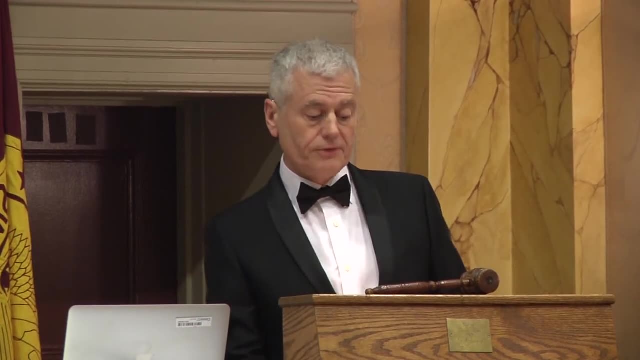 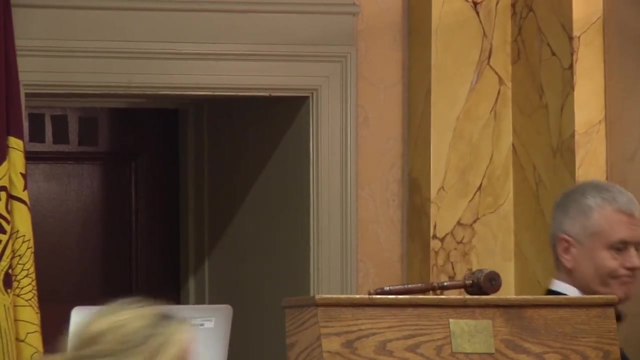 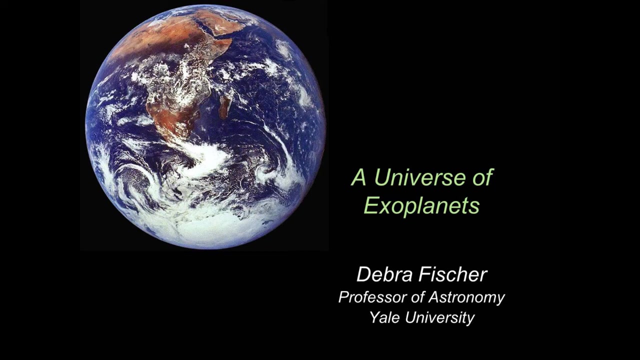 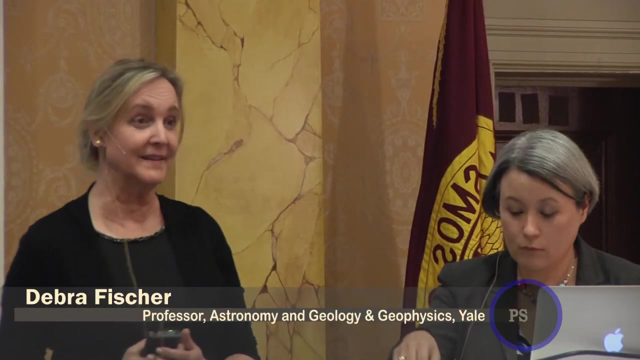 became involved with space mission development during her post-doctoral work at the Carnegie Institution for Science and later at the Goddard Space Flight Center. Dr Aki Raberge is a time I started working in the field, as you heard, in 1997.. At the time, there were three exoplanets. 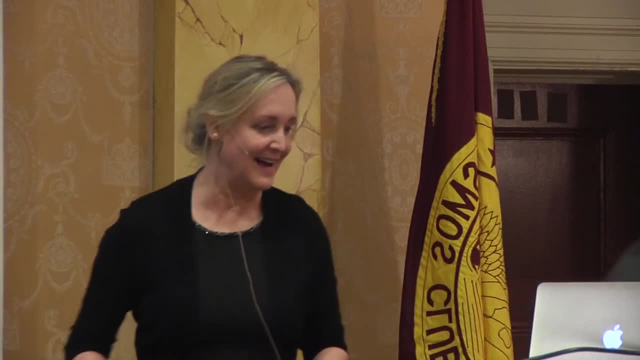 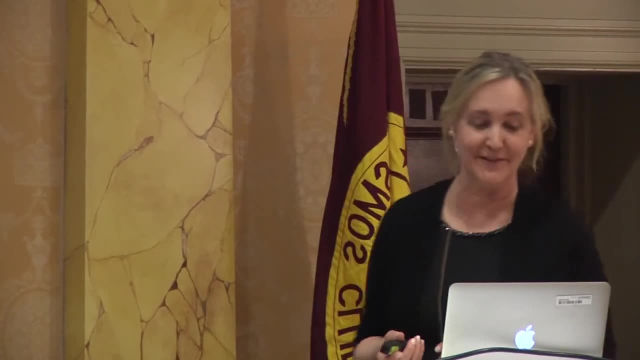 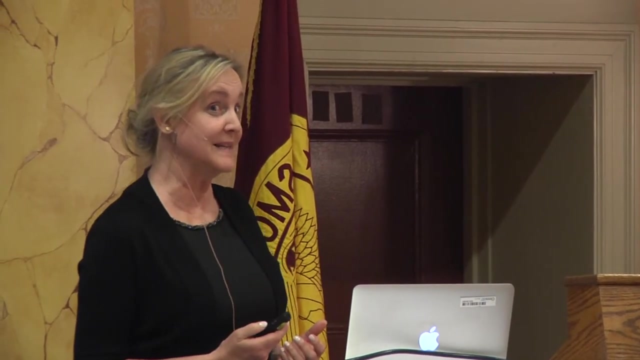 that we knew about, Thanks, And I have been incredibly fortunate and lucky to be able to work in a field that's just exploded underneath of me, So I'm going to tell you a little bit. I want to start by giving you a sense of our place in space and time. This might be something that 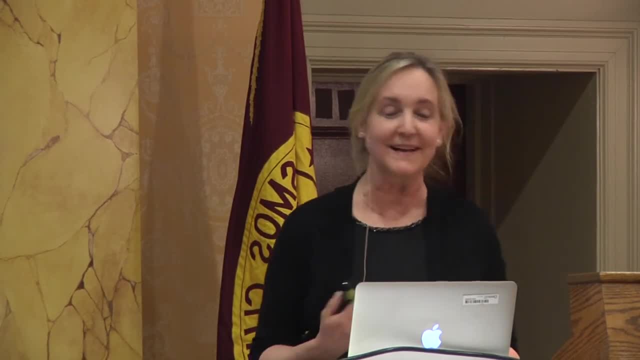 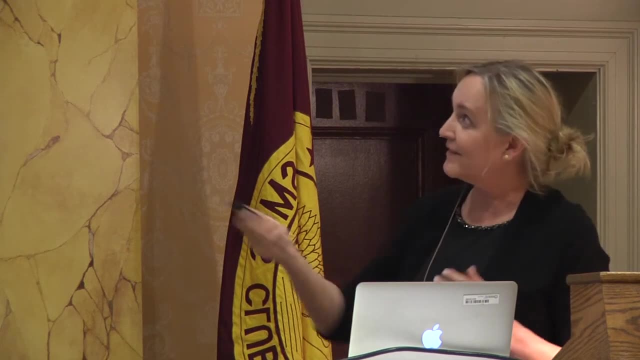 you guys are familiar with, but I think it's something that I always like to reflect on, And if, after all these years, I still find it amazing, I hope that you will as well. We think of here we are on this beautiful planet, right, But if we look, our planet is just a pretty. 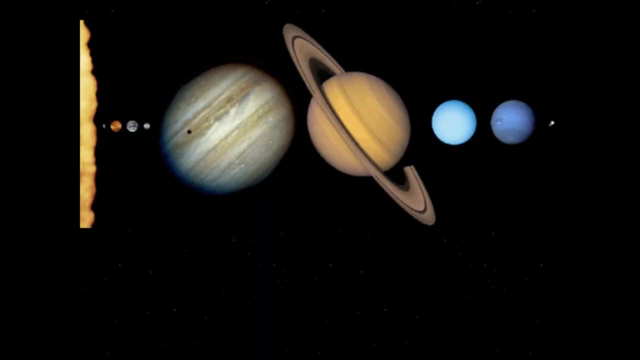 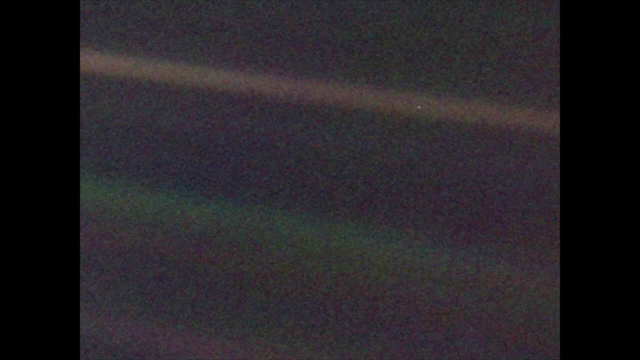 small, insignificant, little speck of a planet compared to Jupiter, Saturn, the other planets in our solar system. And, of course, here's the real view of our planet. You see it right, Everybody sees it. Okay, It's this little dot here suspended in a beam of sunlight. This is a picture of the Earth. 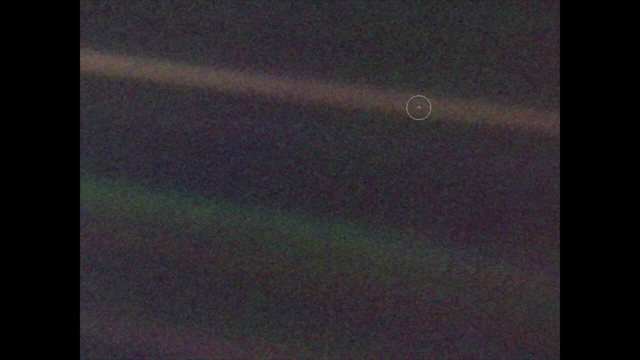 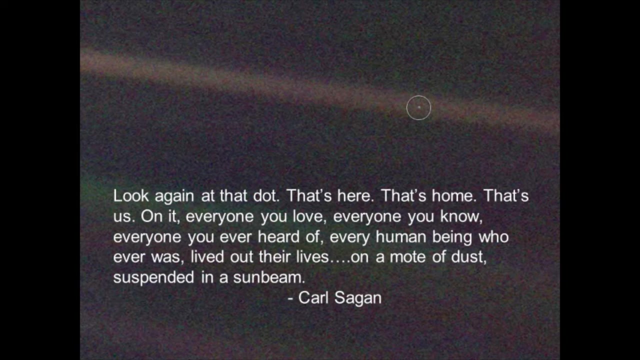 that was taken by the Voyager spacecraft as it was going into the outer part of the solar system. And as Carl Sagan wrote, look again at that dot. That's here, that's home, that's us On it. everyone, you know, everyone you ever heard of everyone, who, every human being, who ever was. 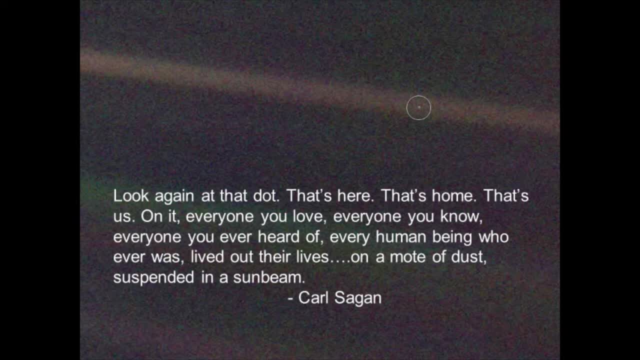 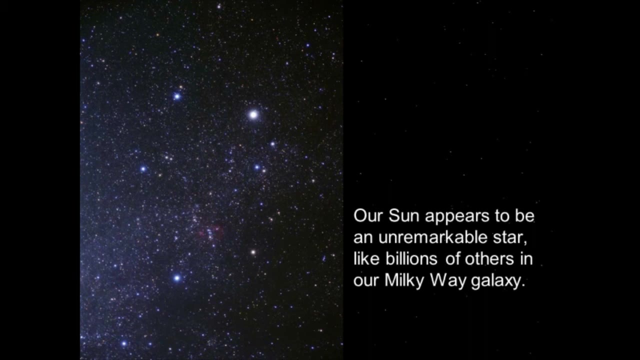 lived out their lives on a mode of dust. It's suspended in a sunbeam. This is the kind of picture that if we work very hard, we might be able to get of planets around other stars. Our sun is just a very ordinary star. right, It's fairly. 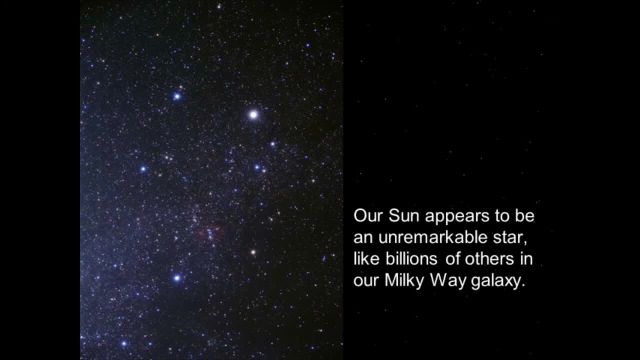 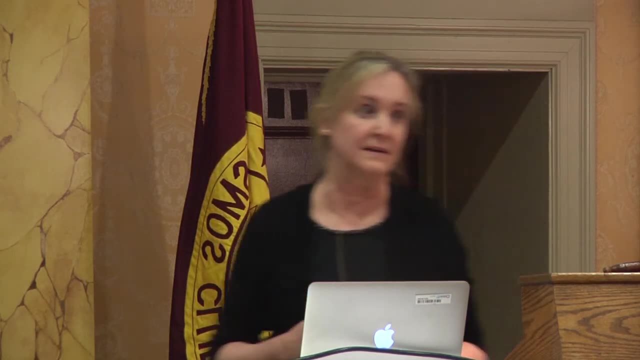 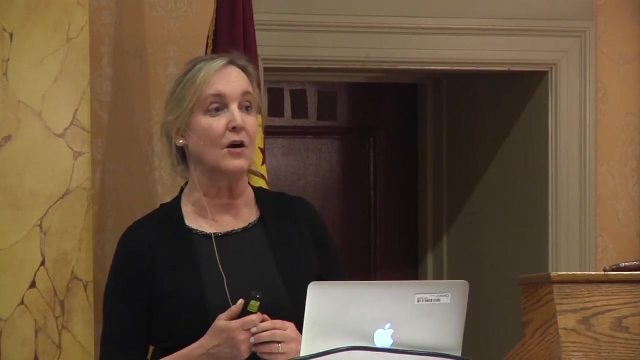 unremarkable. It's one of billions of others in our Milky Way galaxy. If you think about the most massive stars in the galaxy, there are a thousand stars like the sun, compared to those really rare, really massive stars. But the most common type of stars in the galaxy are not like the sun. They're much lower in mass. 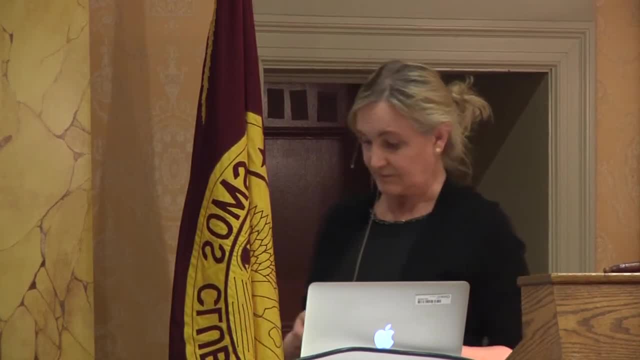 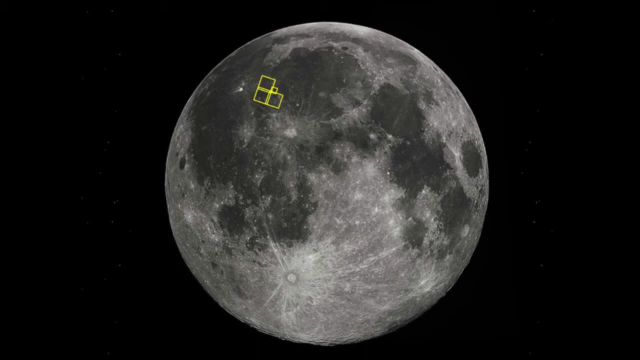 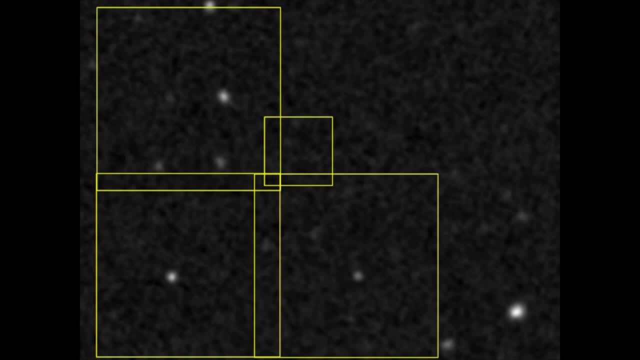 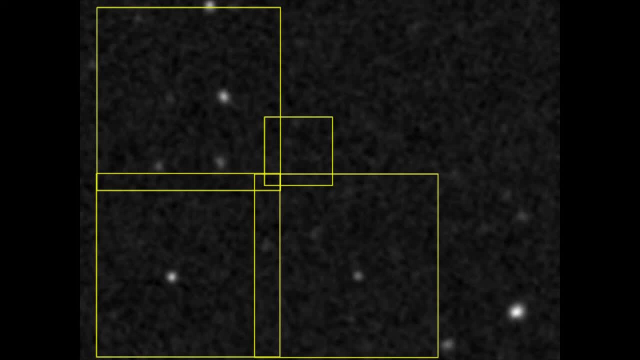 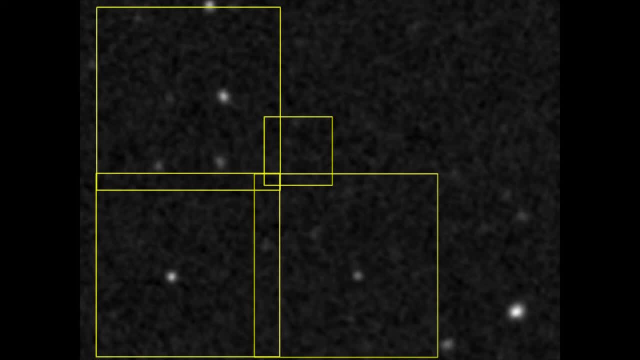 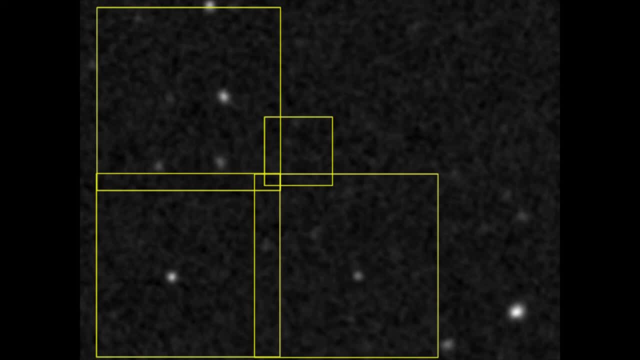 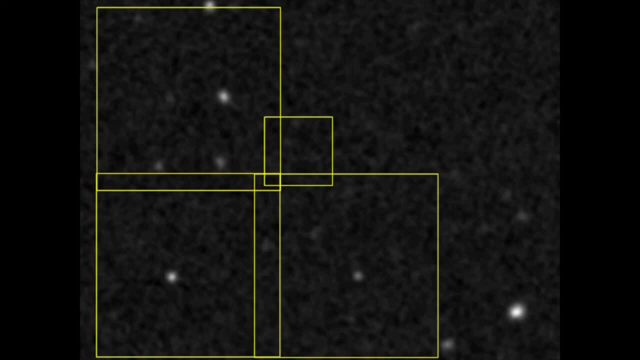 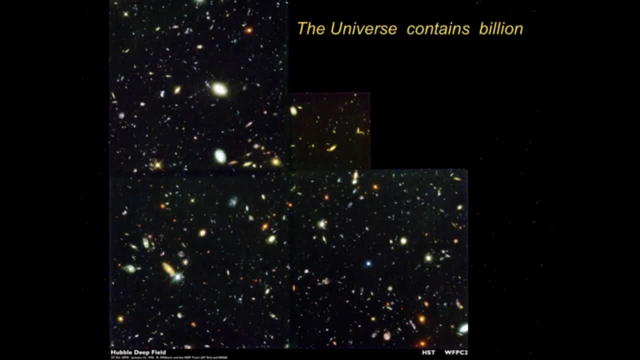 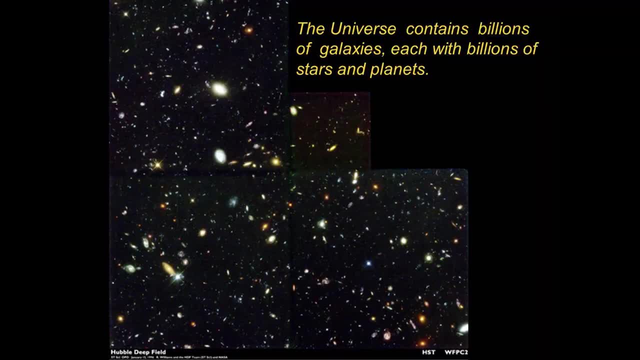 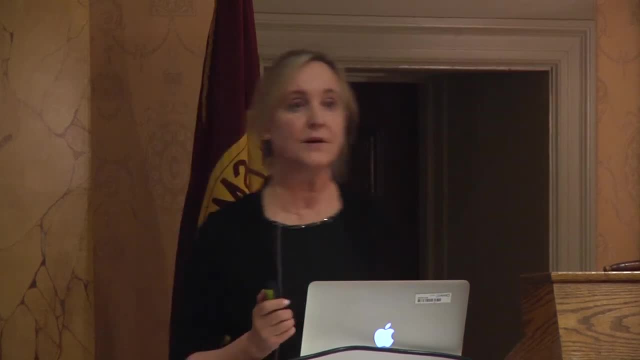 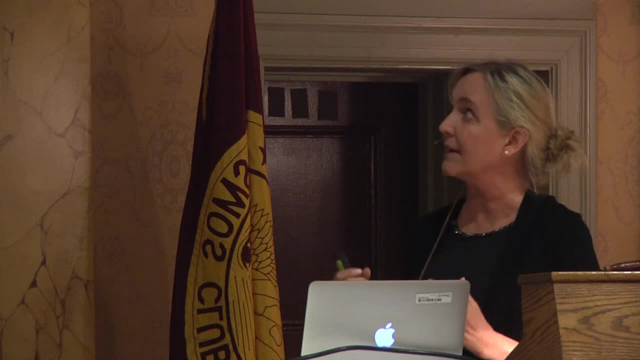 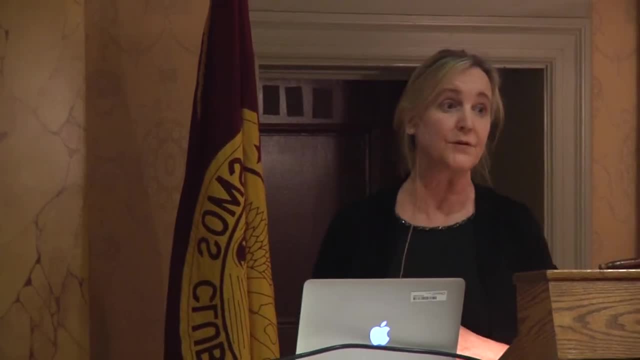 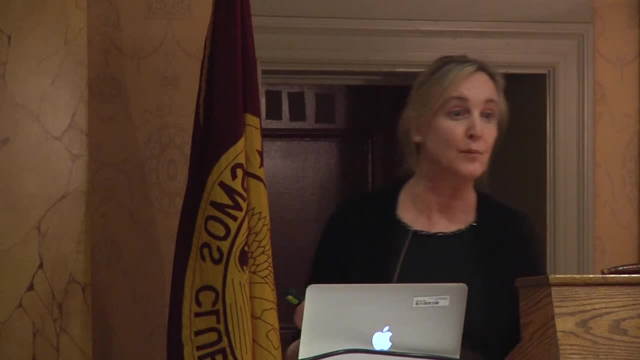 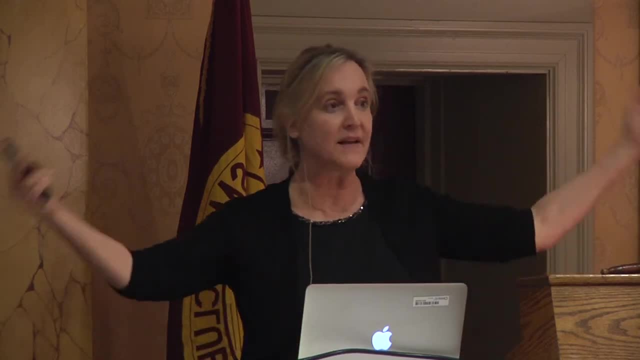 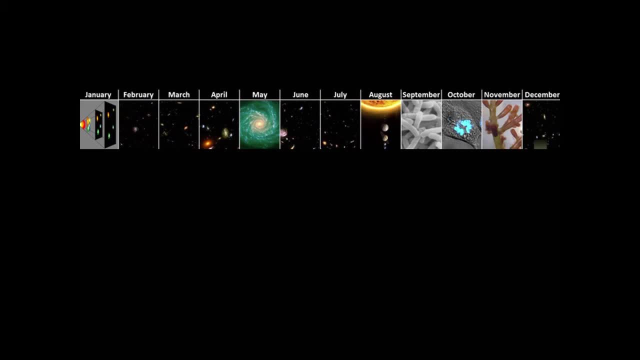 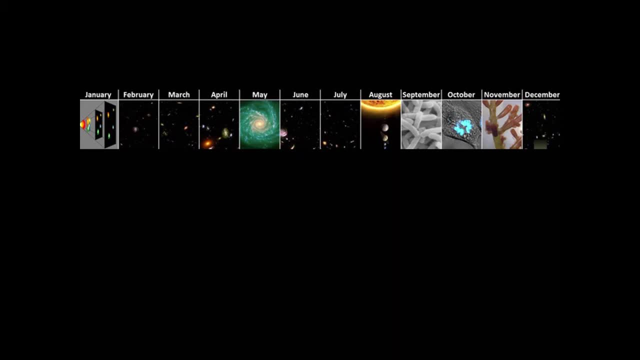 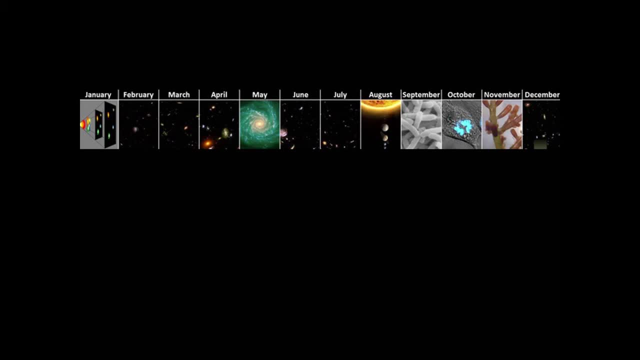 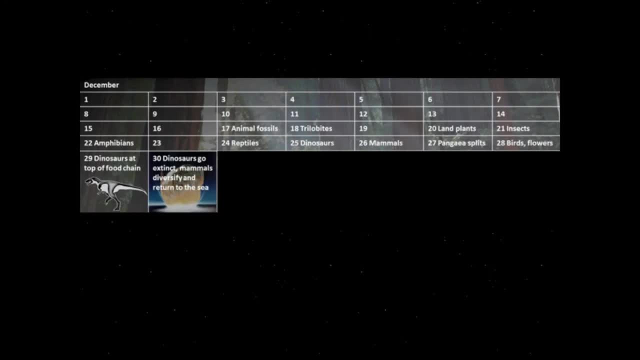 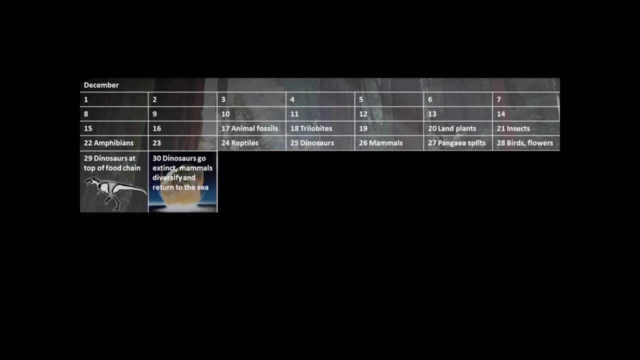 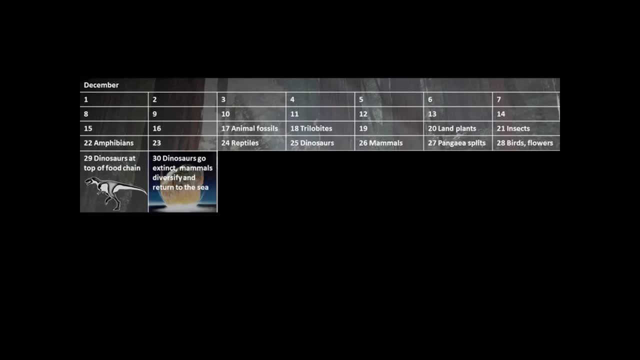 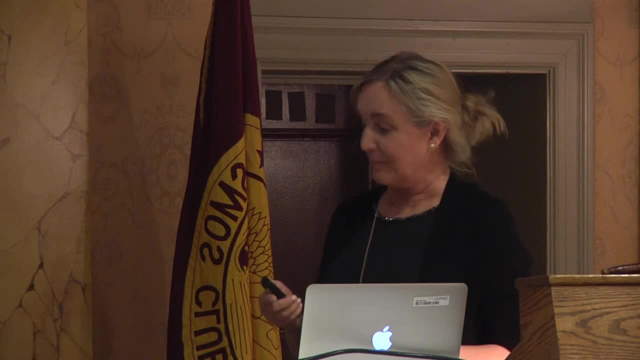 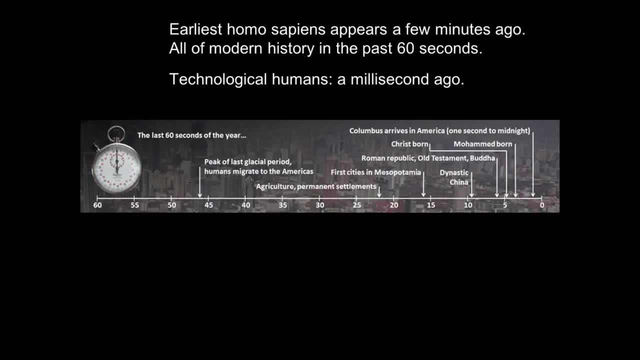 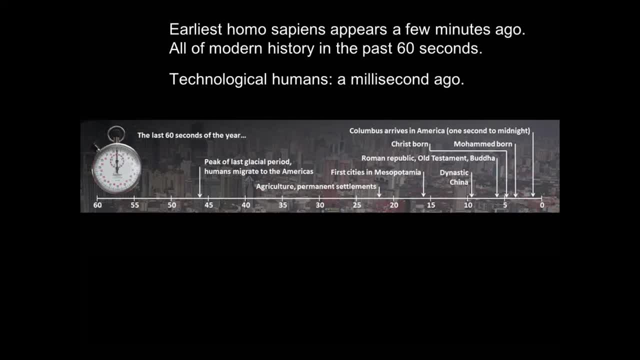 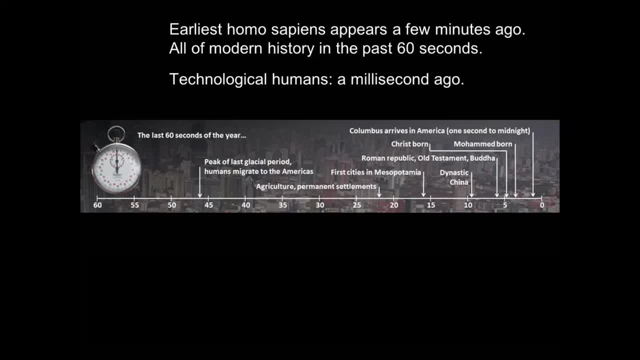 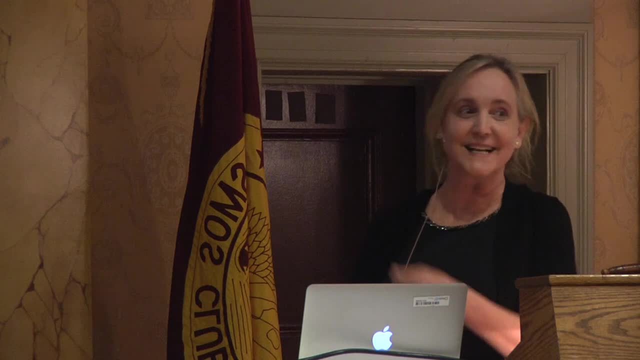 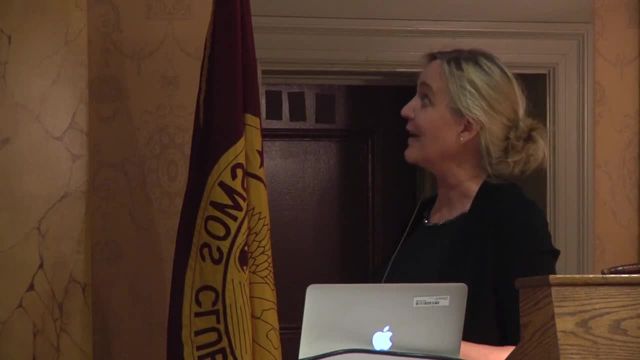 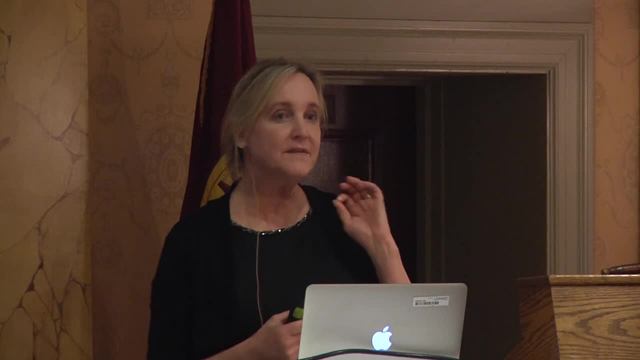 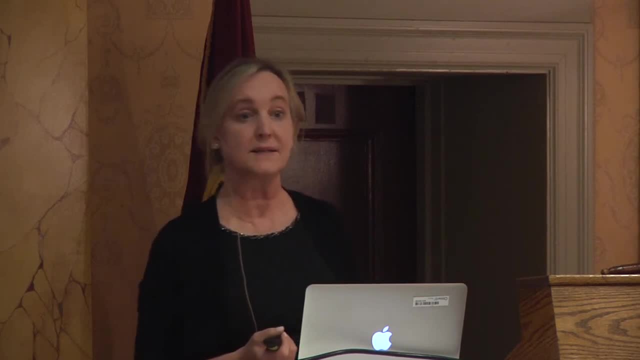 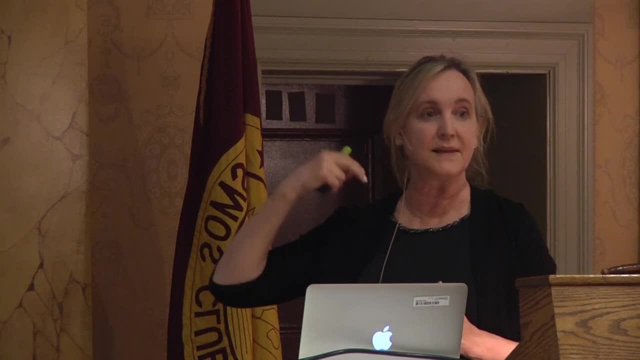 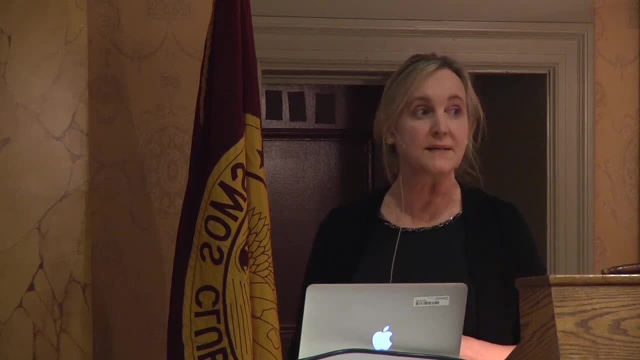 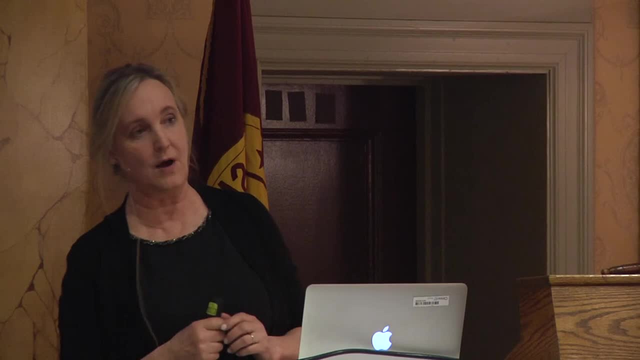 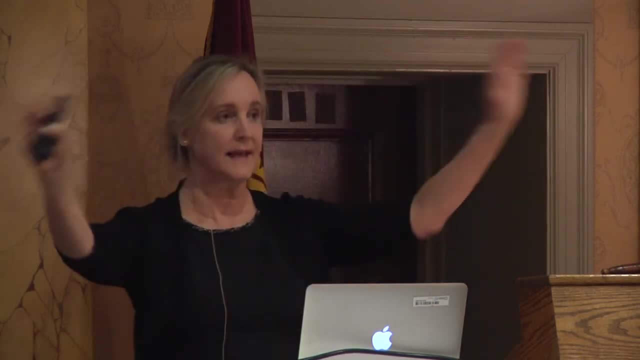 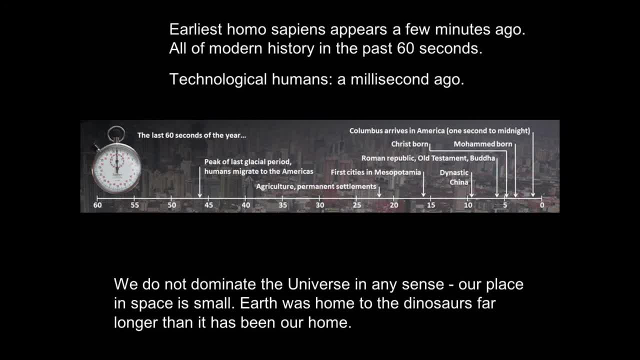 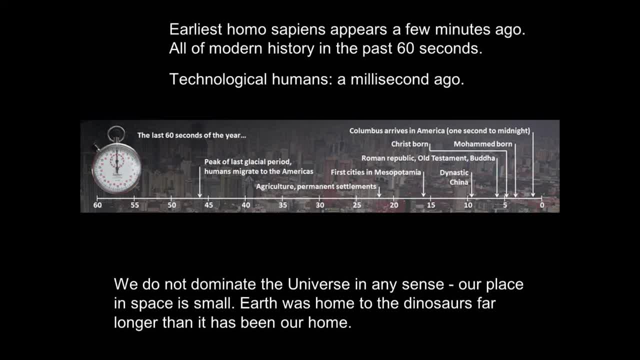 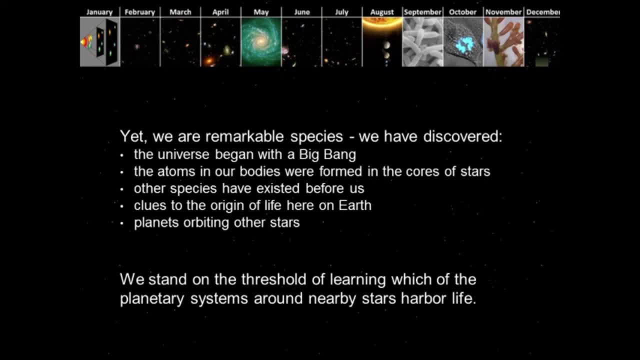 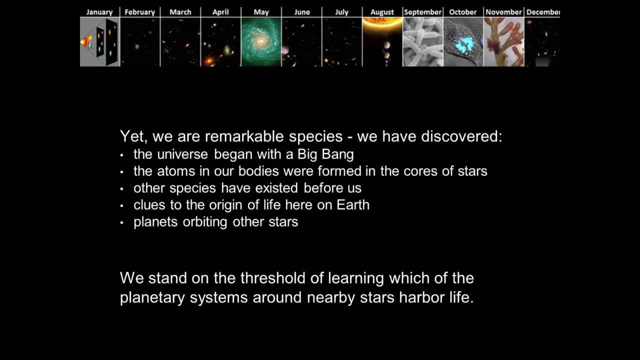 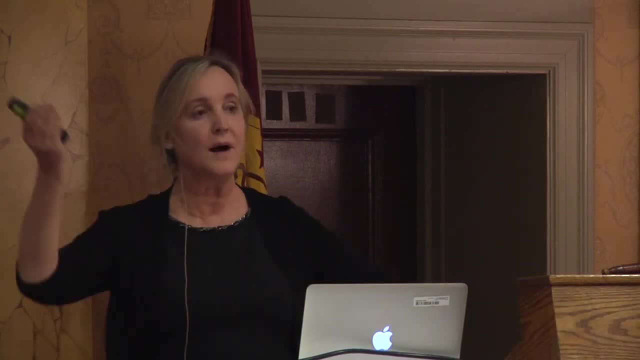 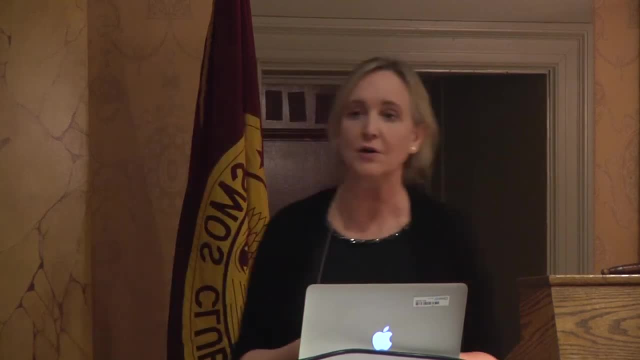 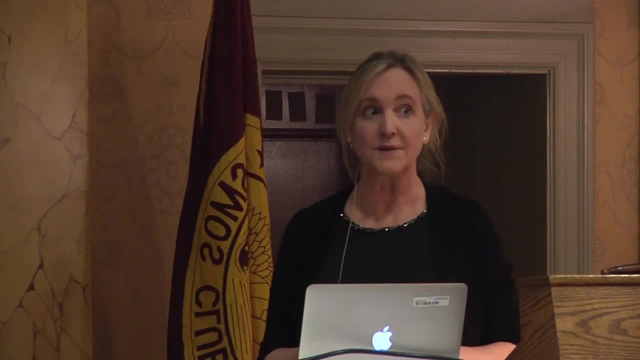 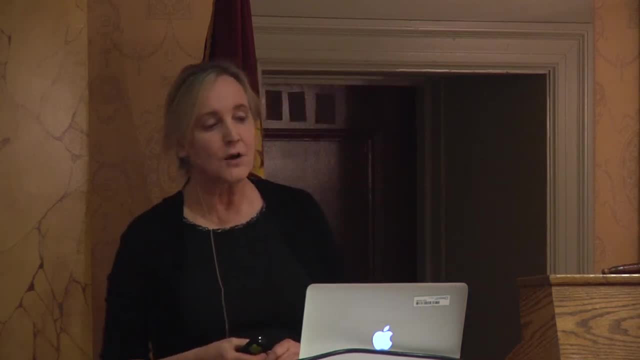 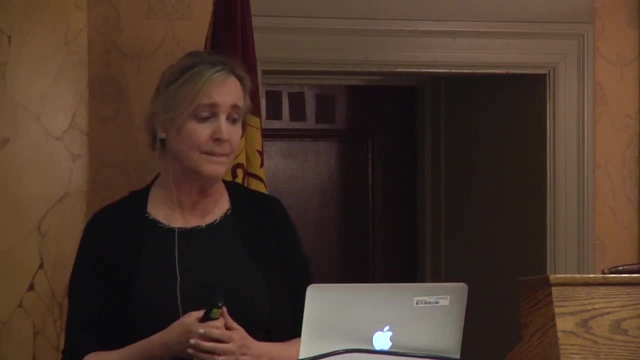 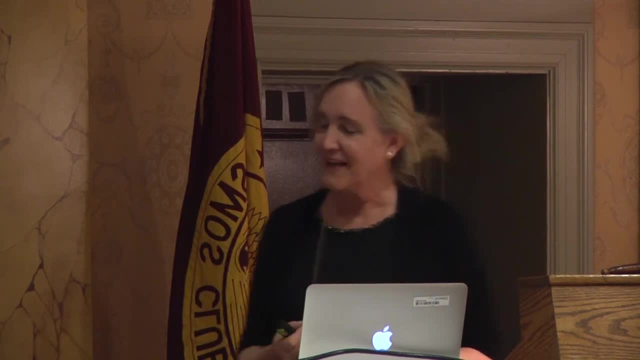 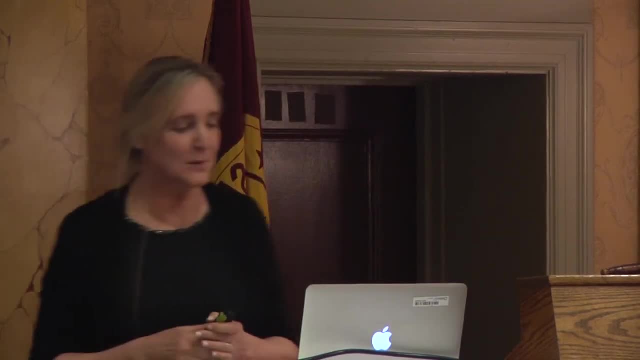 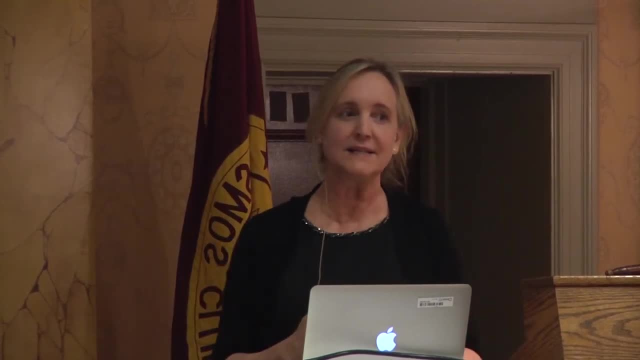 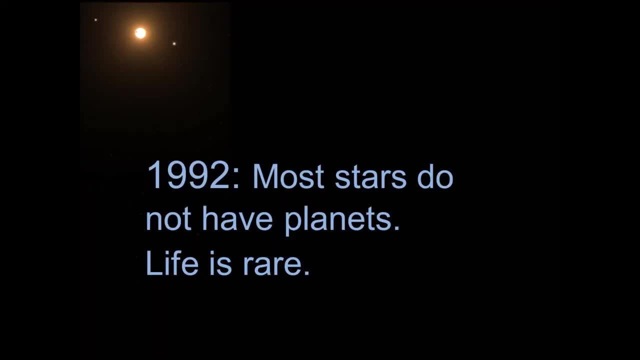 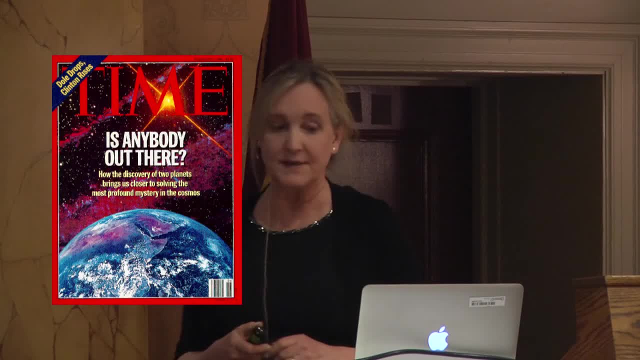 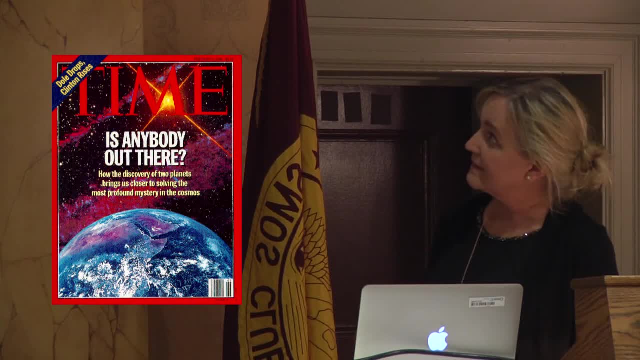 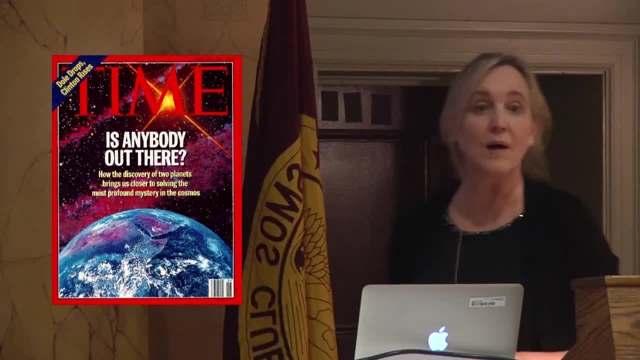 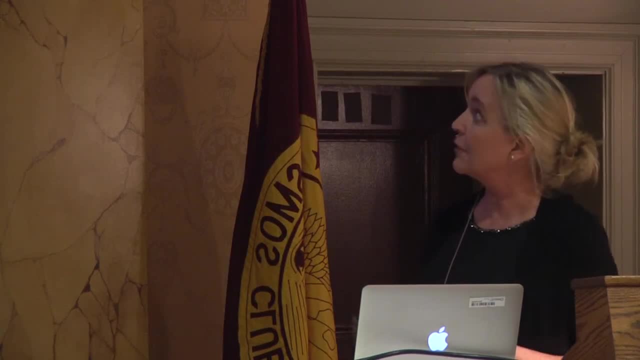 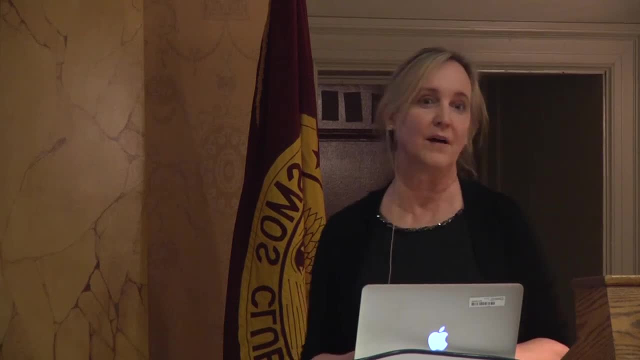 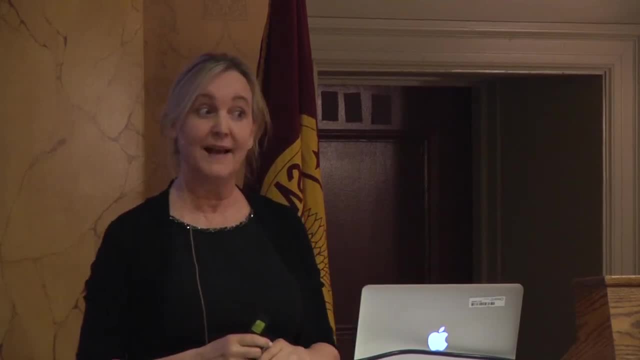 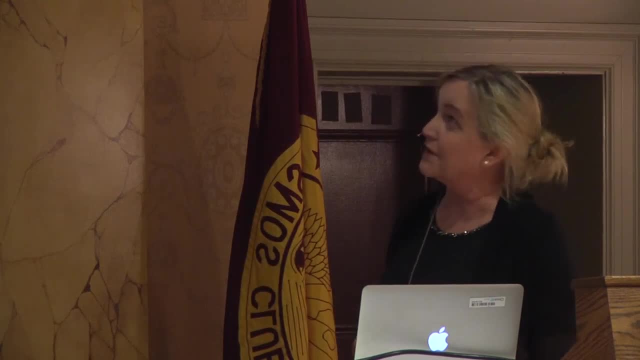 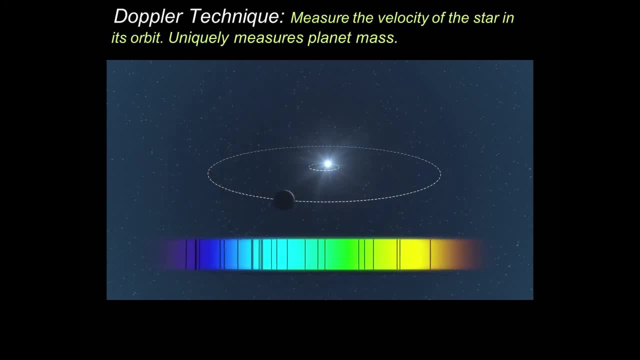 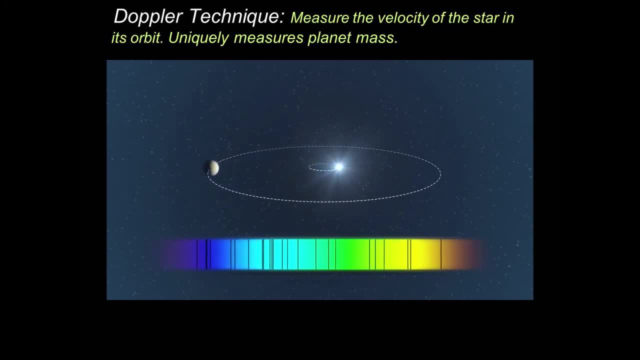 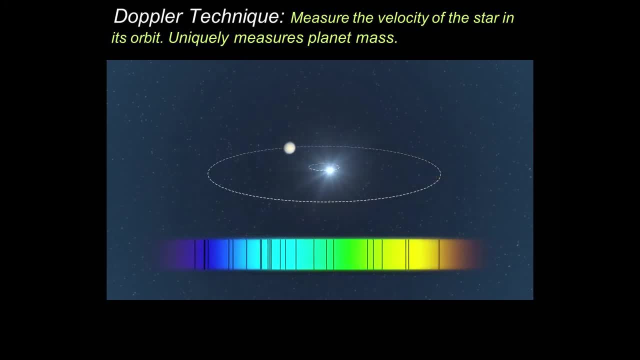 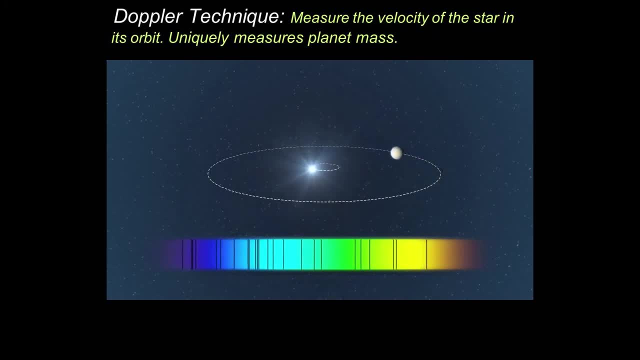 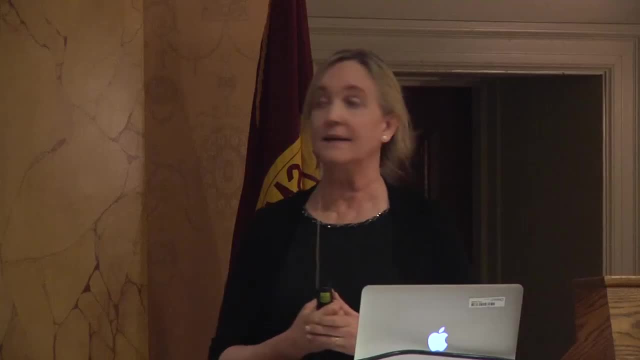 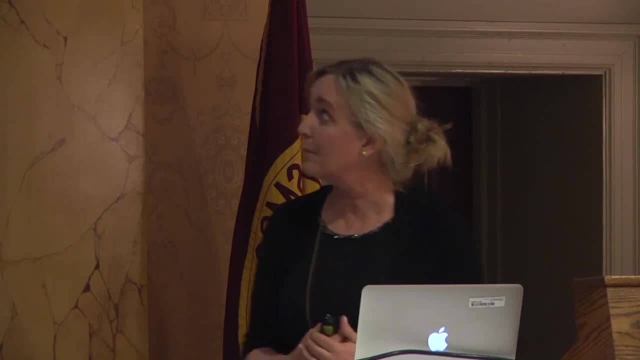 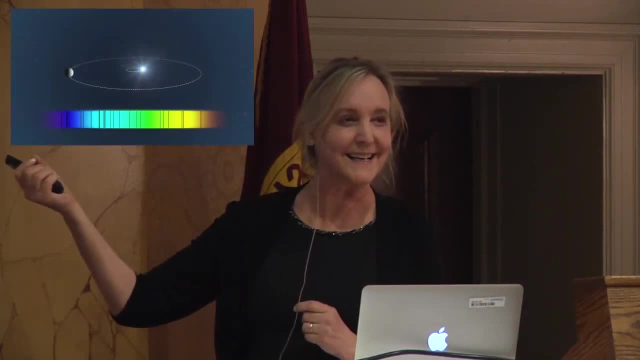 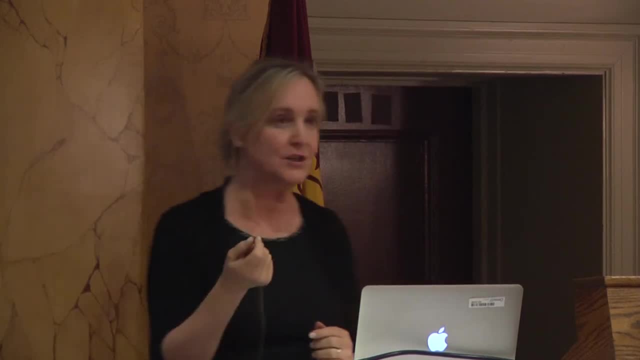 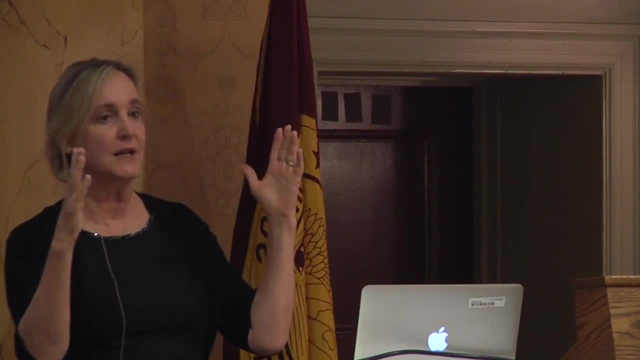 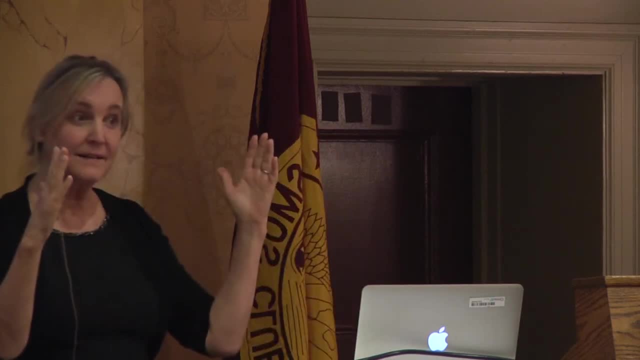 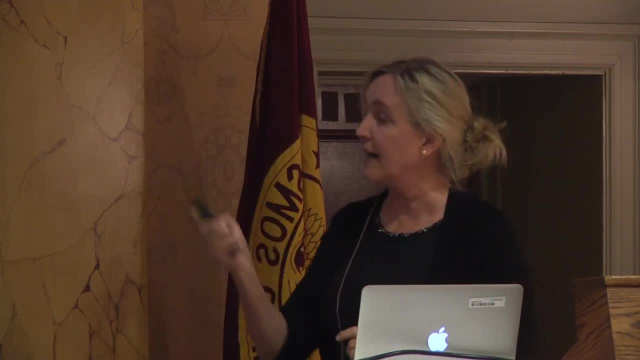 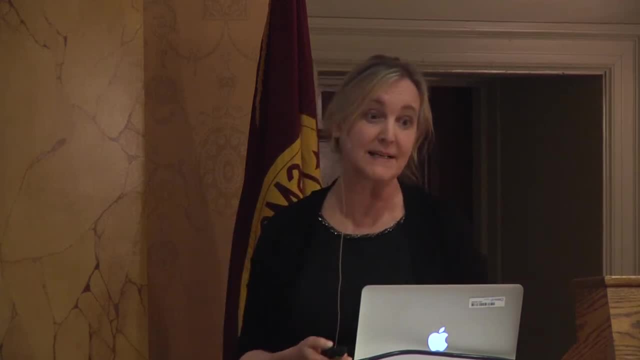 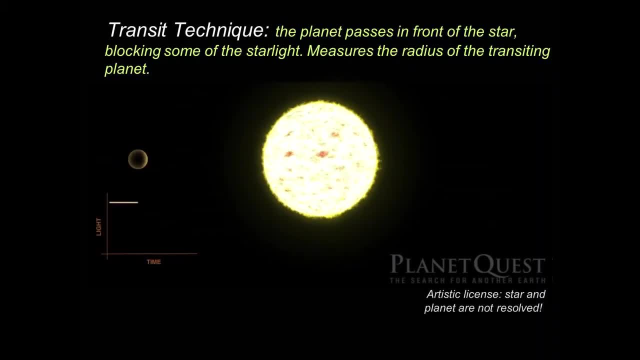 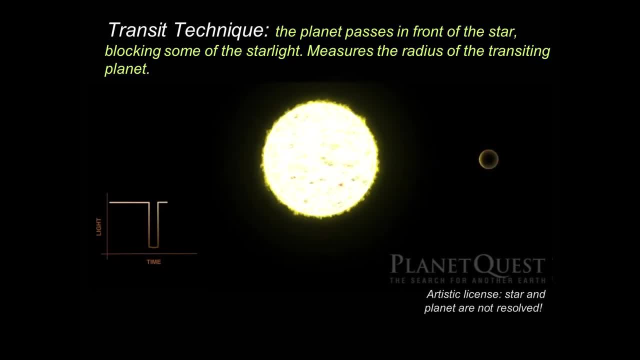 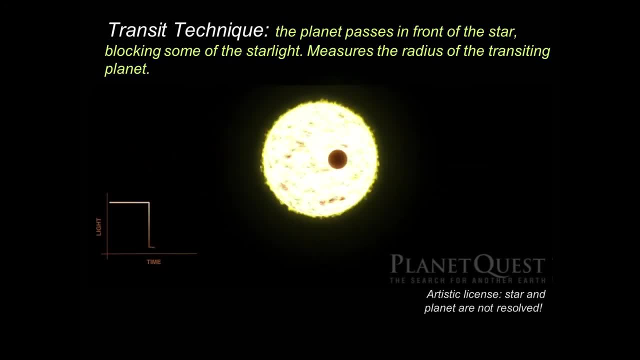 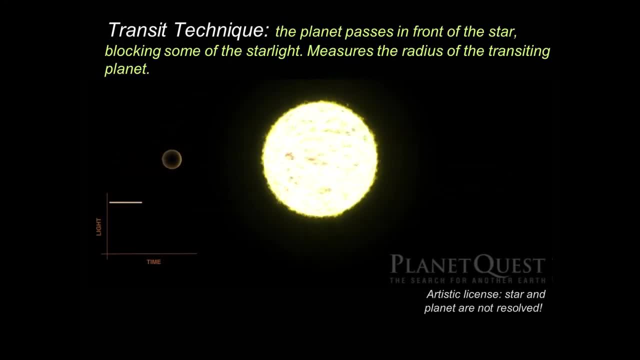 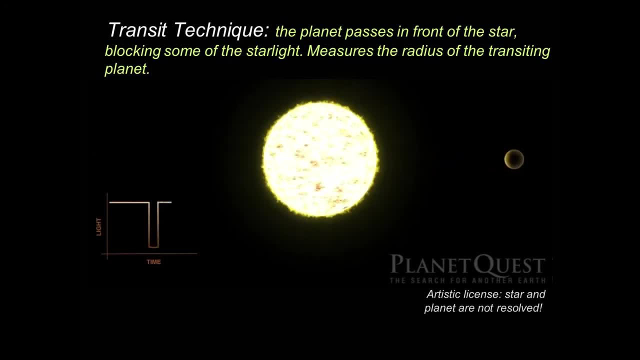 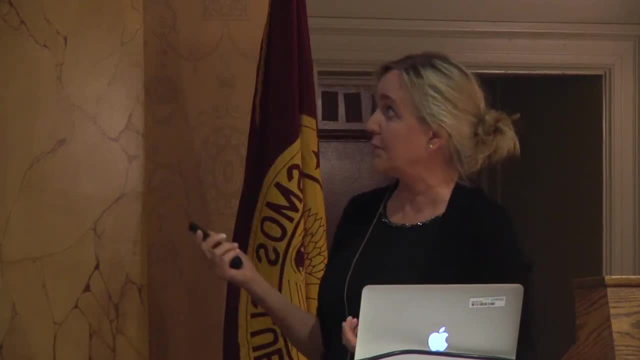 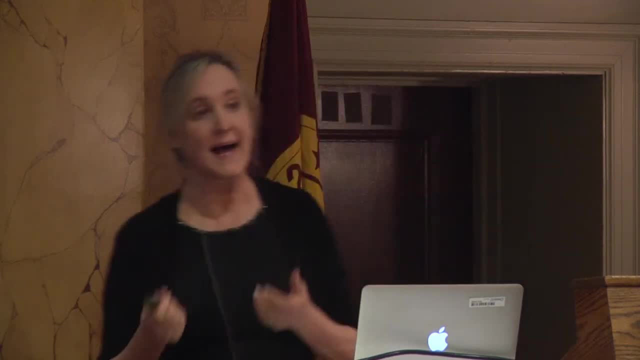 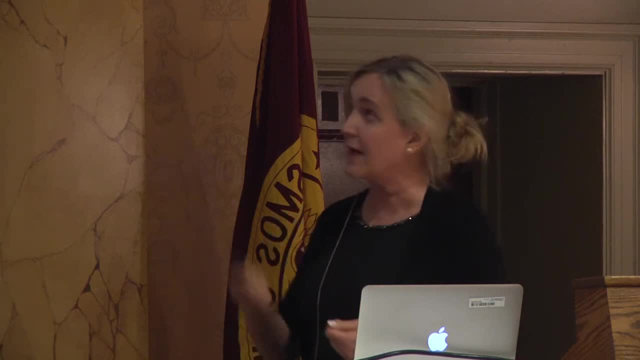 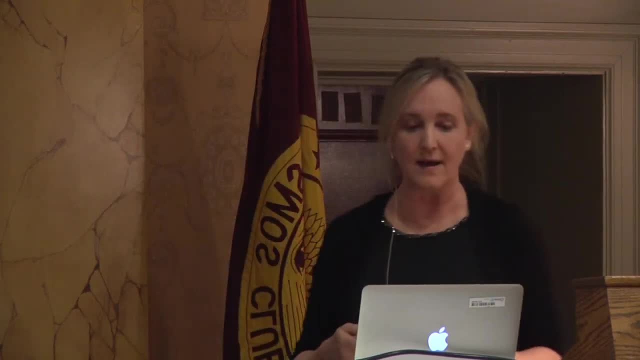 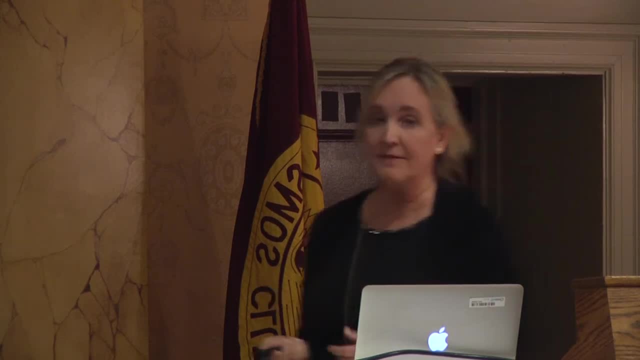 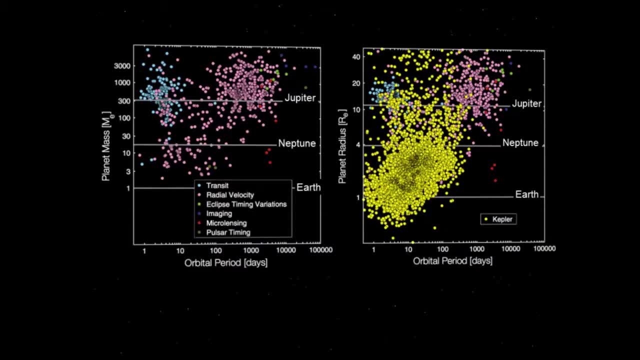 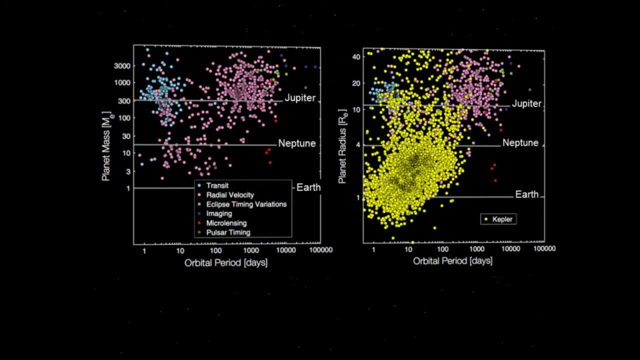 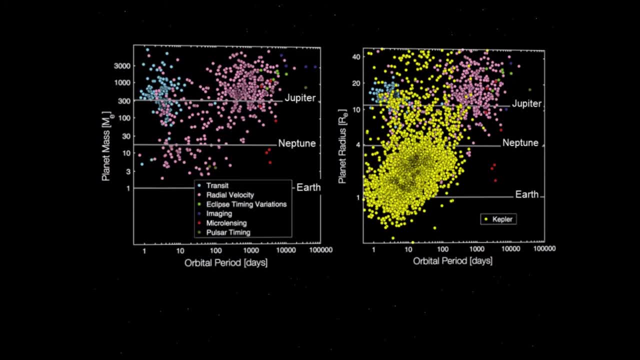 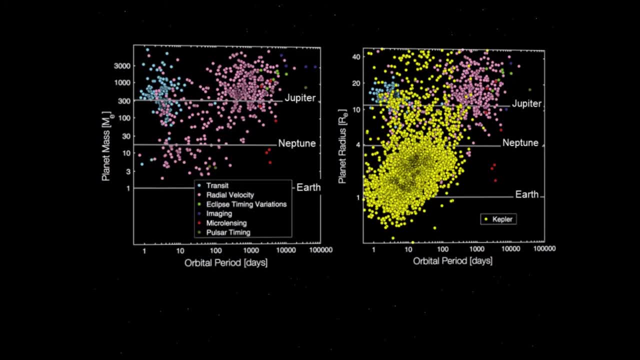 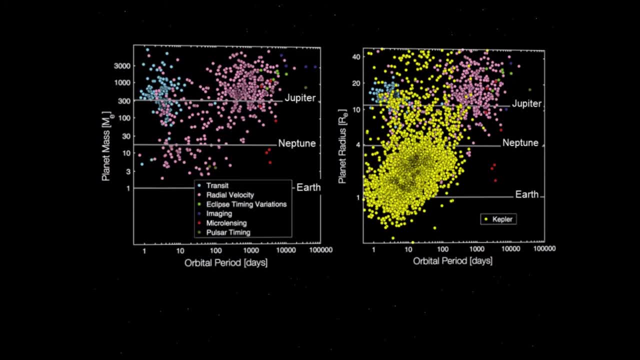 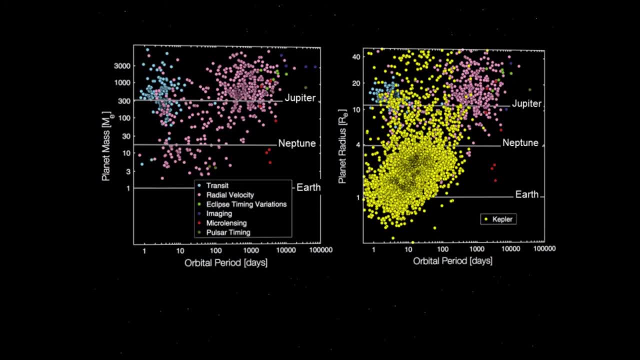 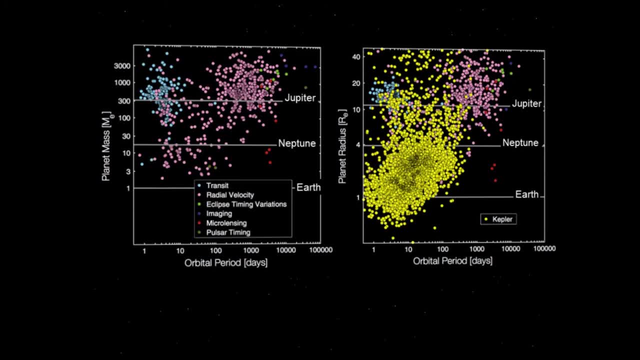 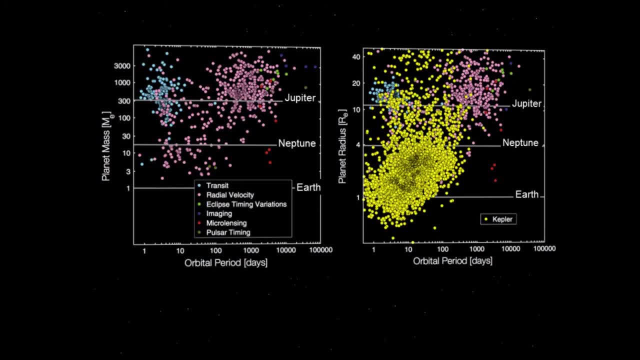 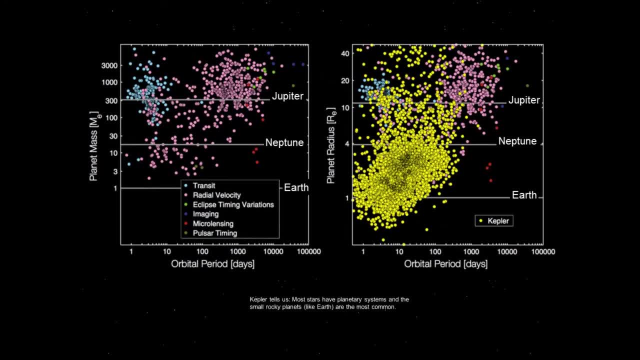 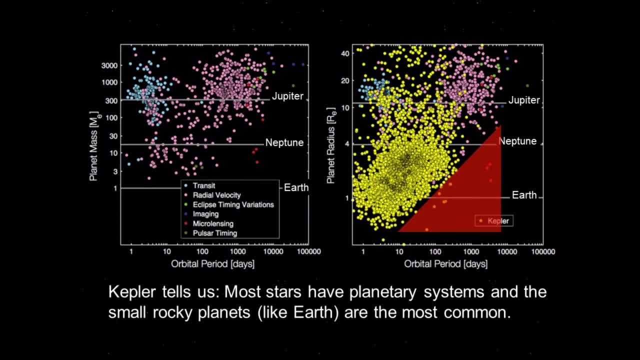 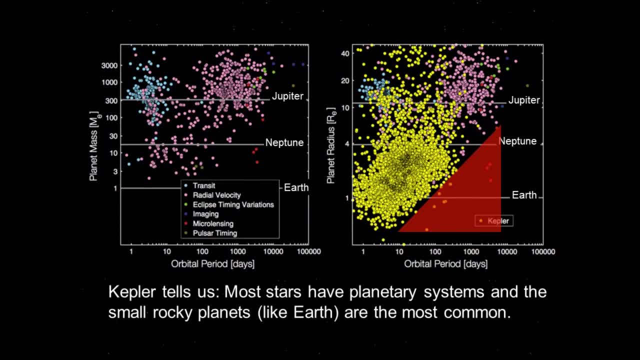 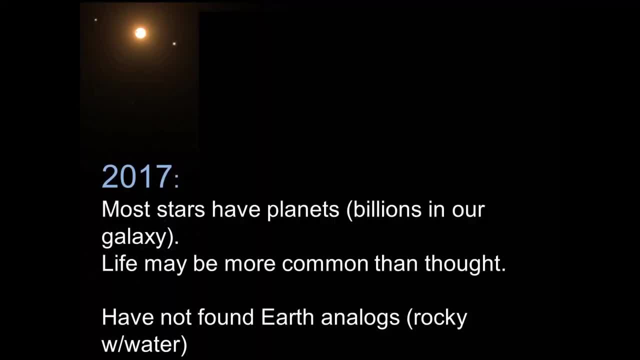 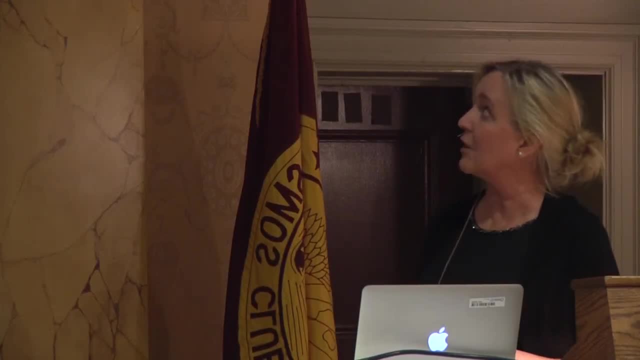 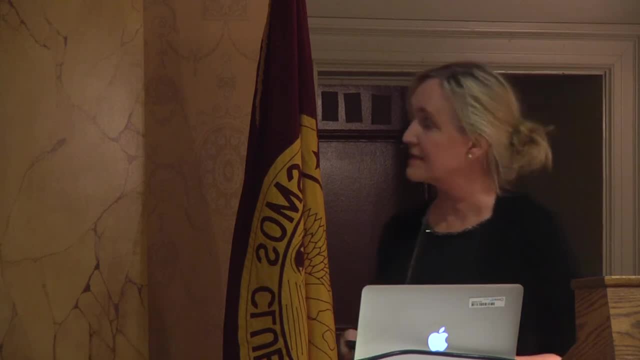 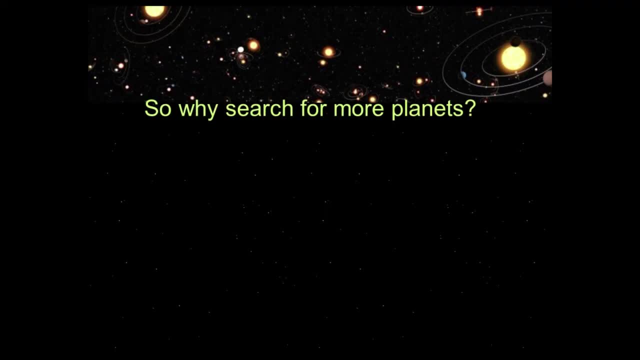 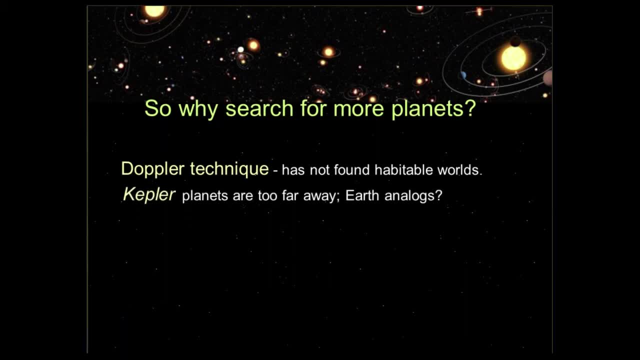 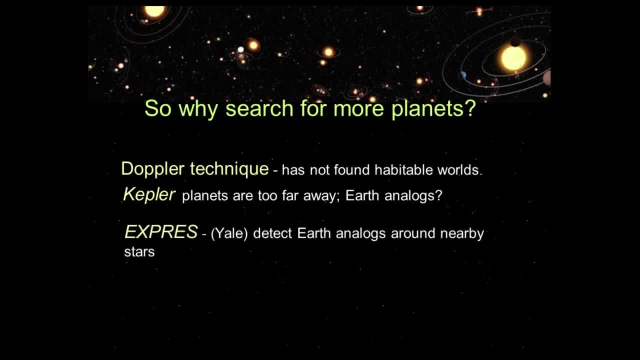 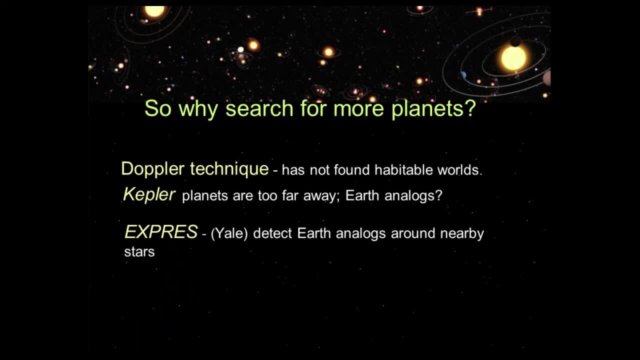 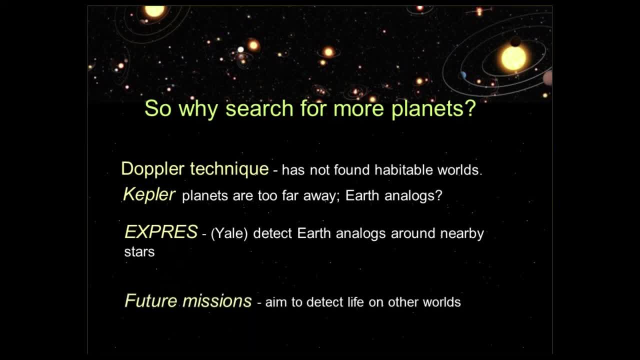 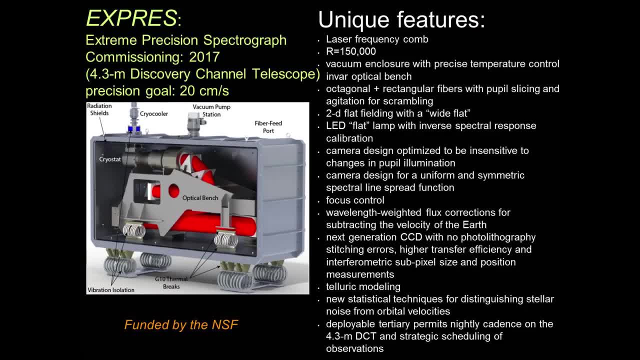 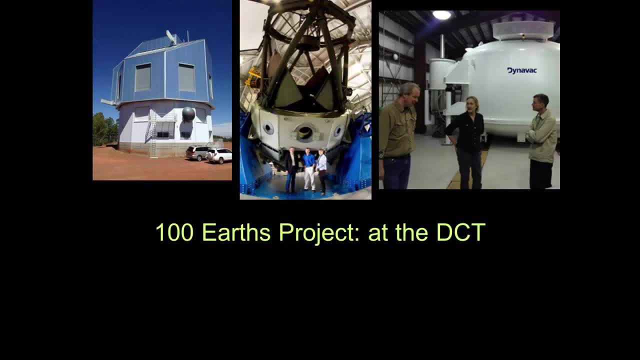 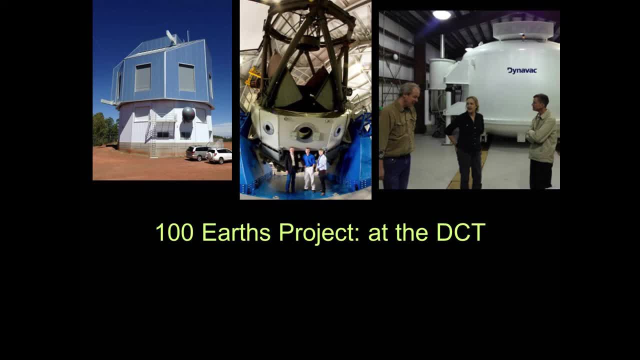 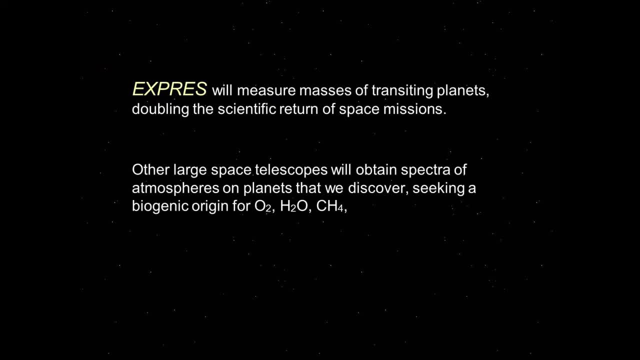 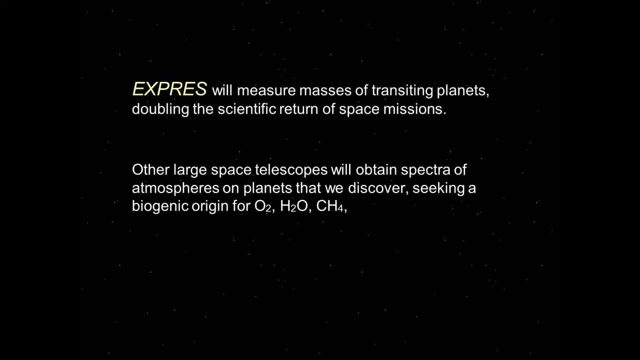 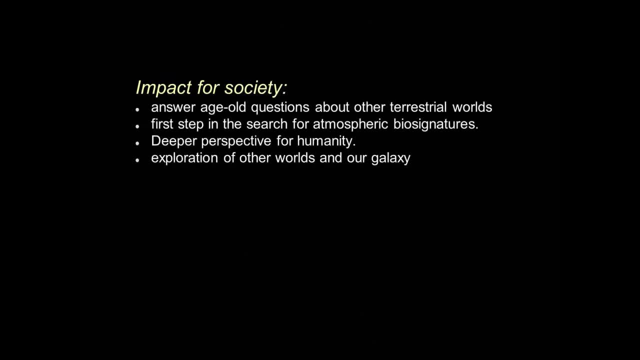 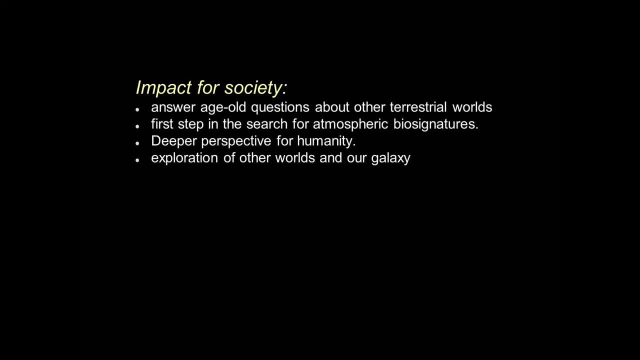 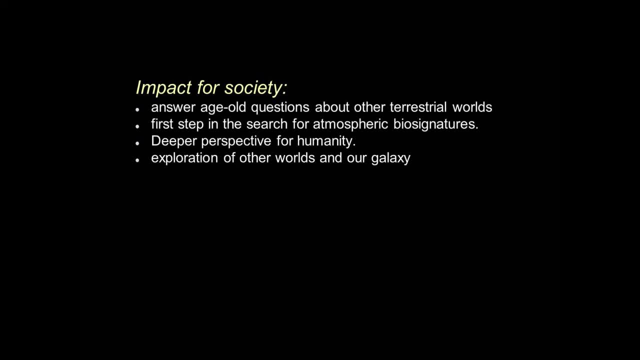 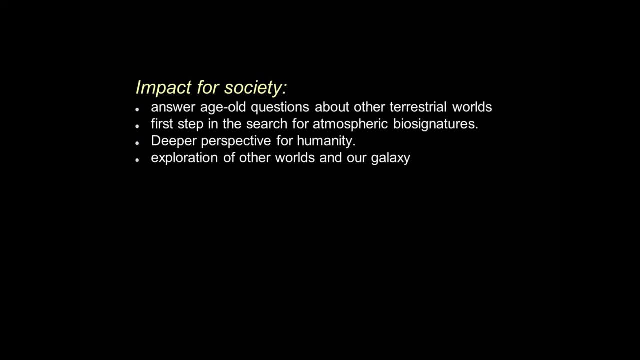 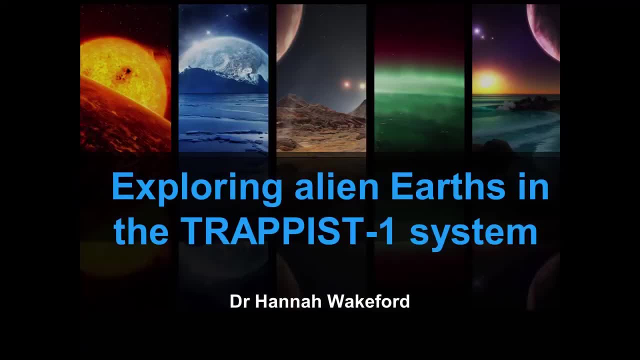 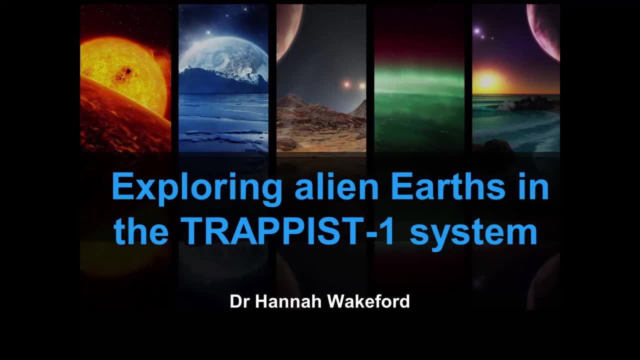 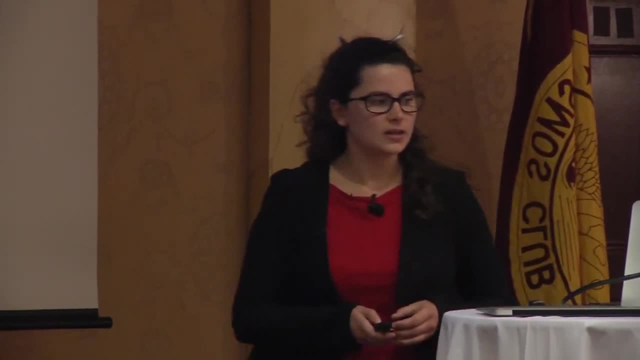 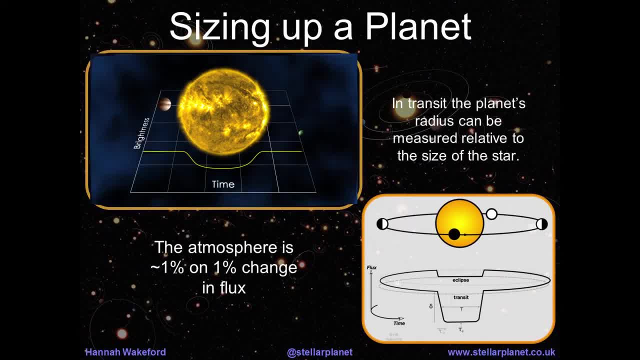 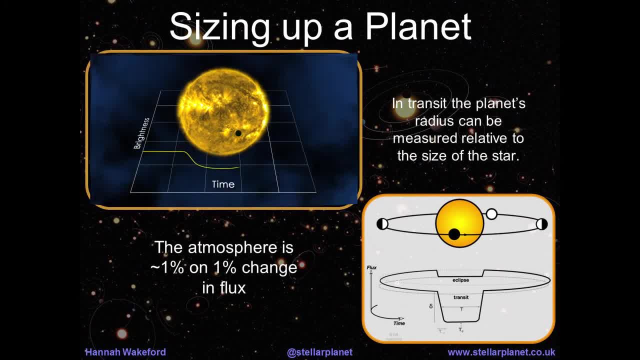 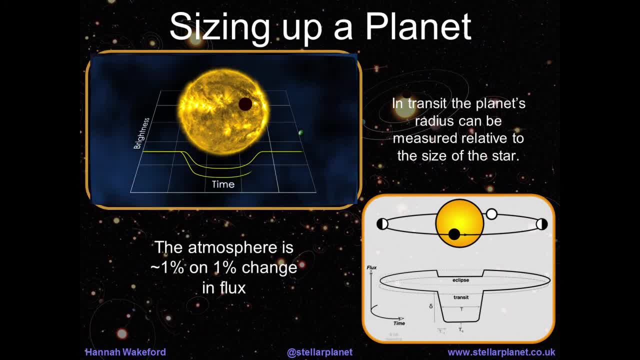 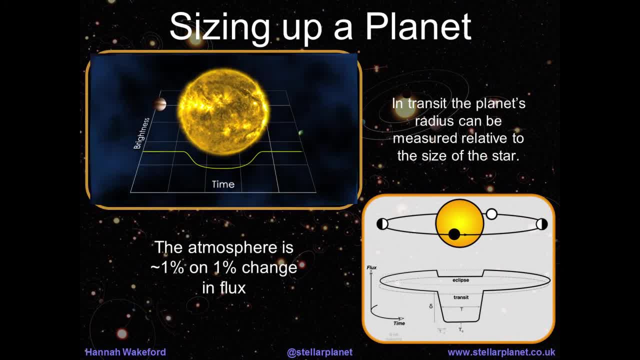 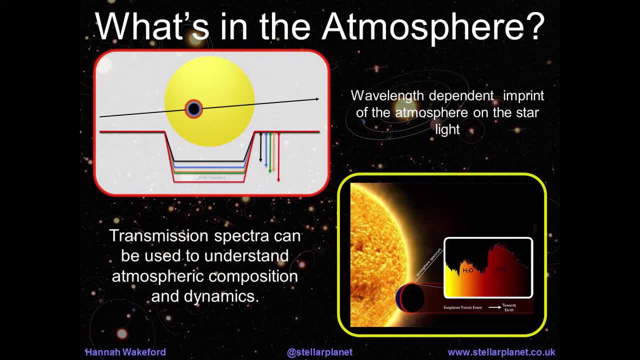 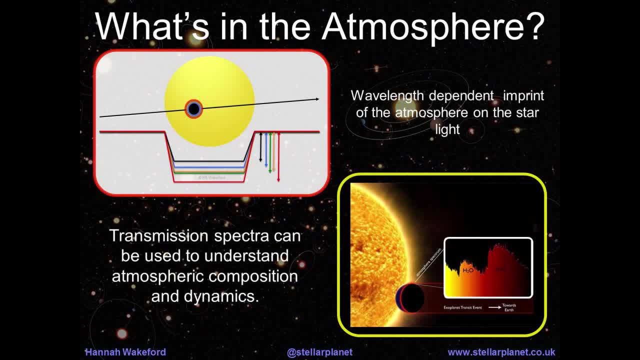 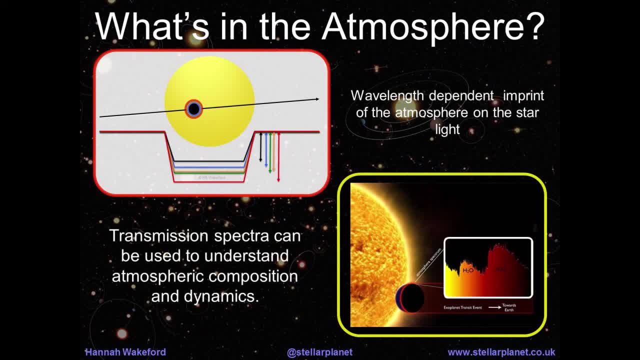 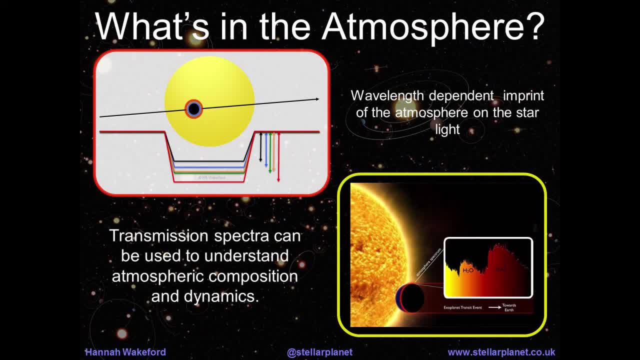 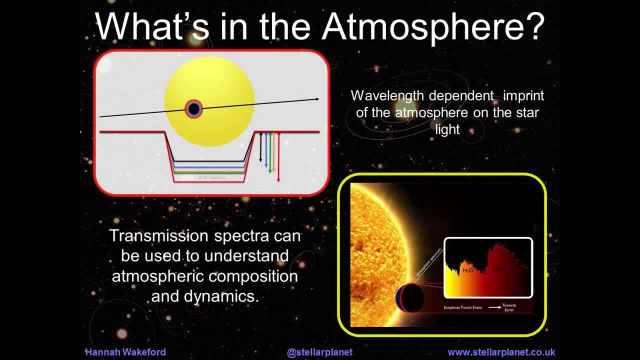 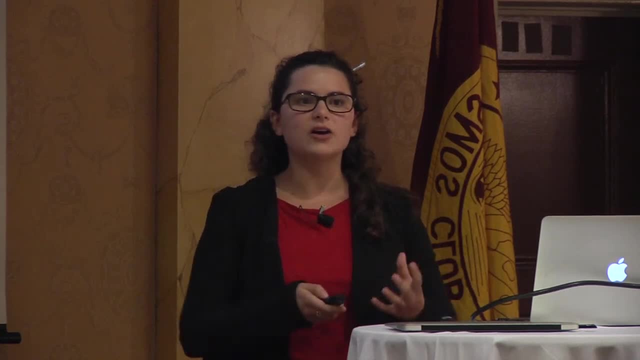 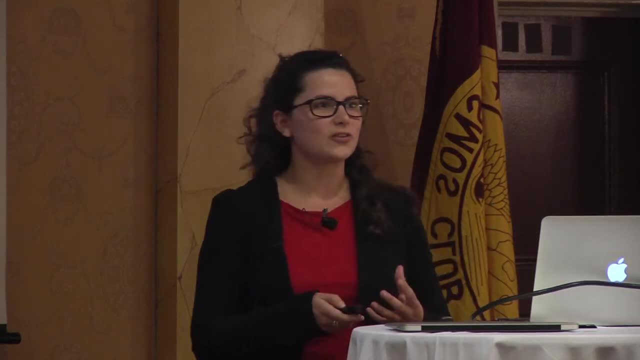 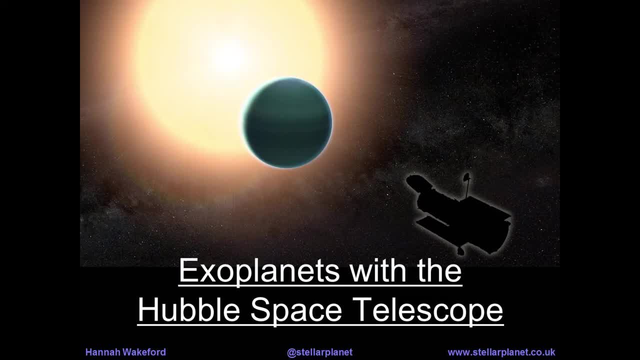 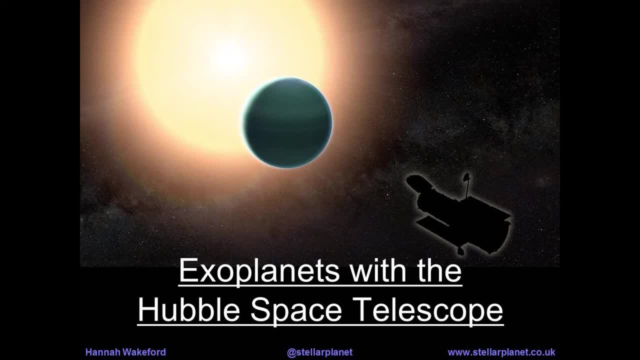 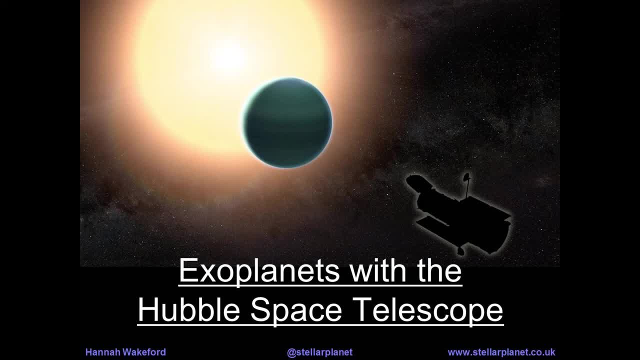 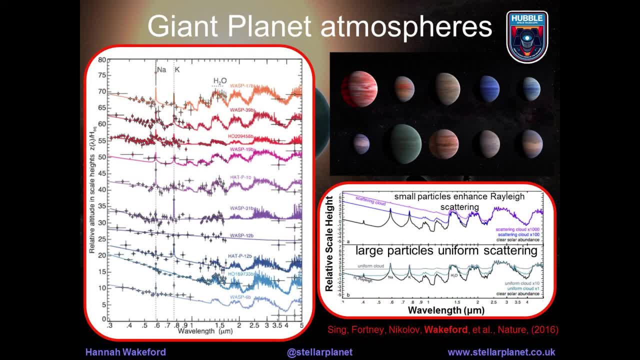 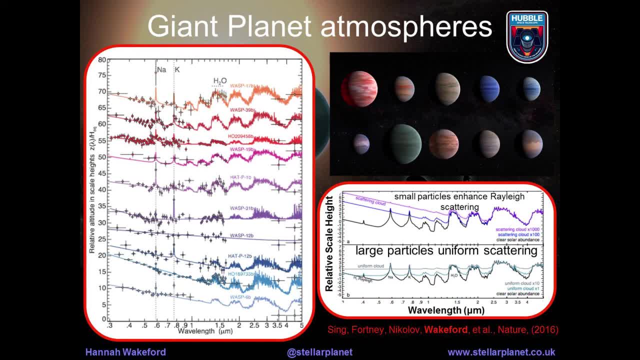 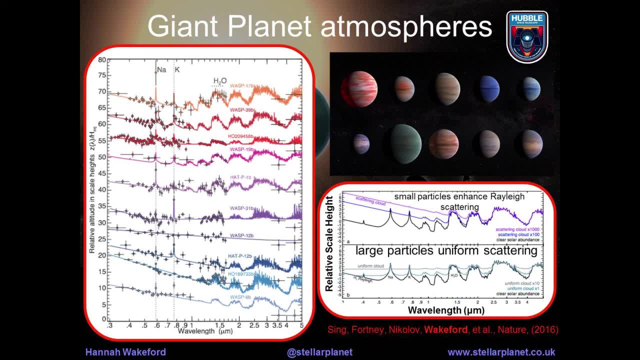 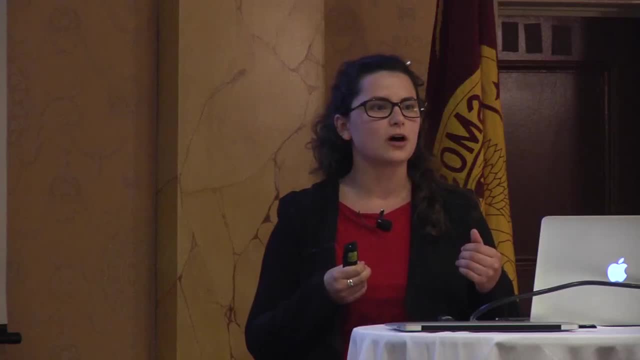 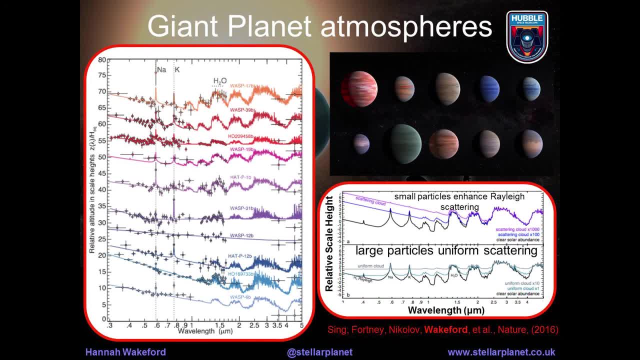 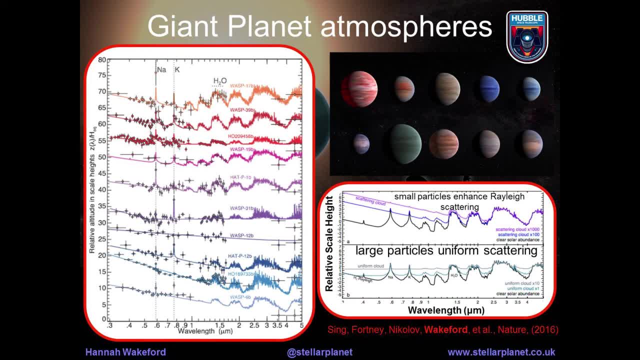 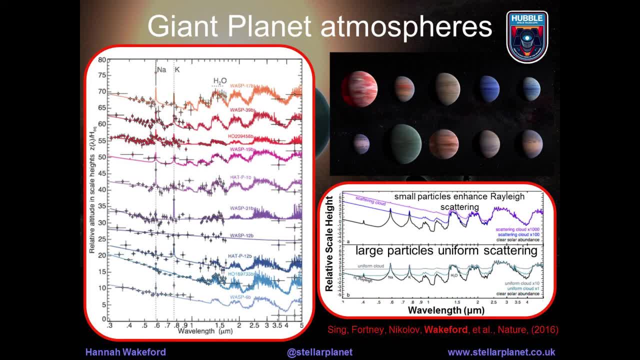 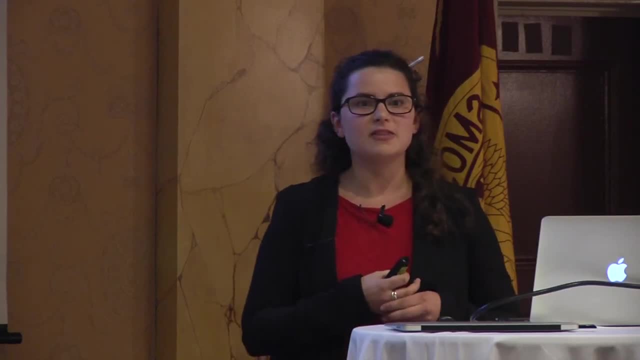 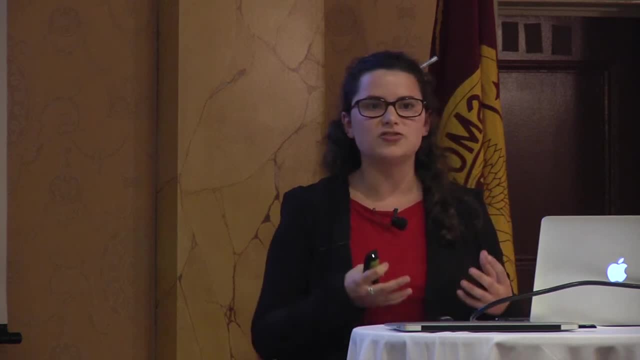 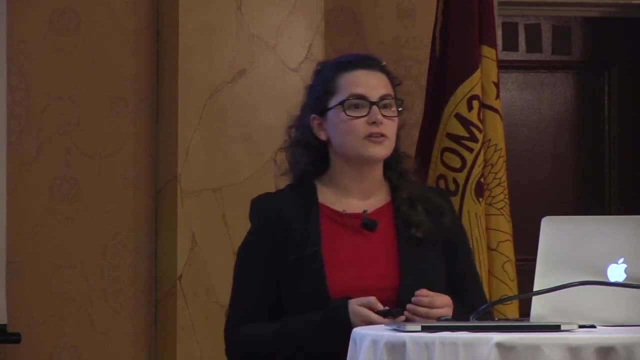 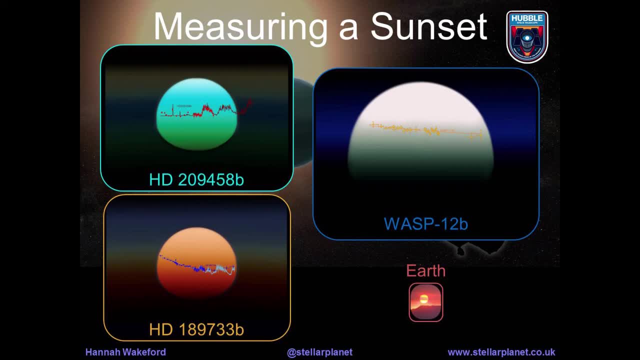 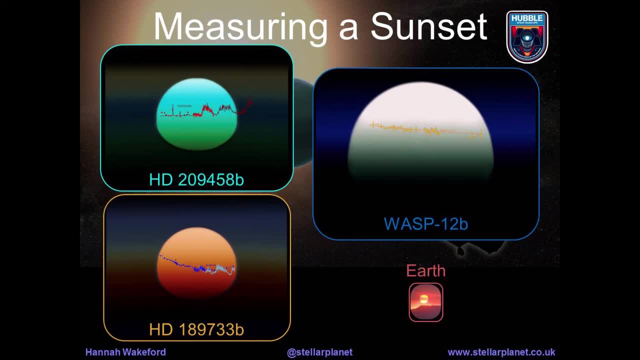 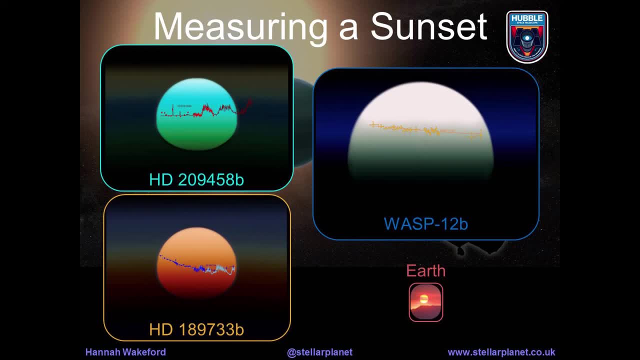 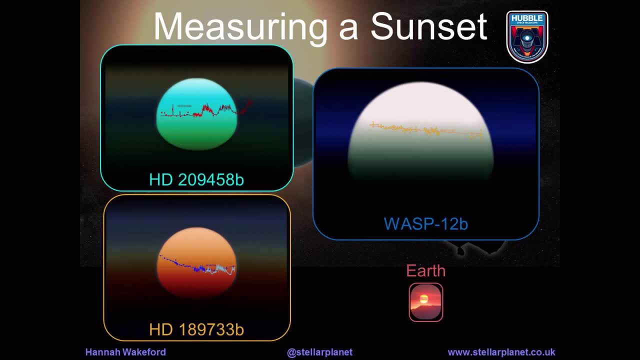 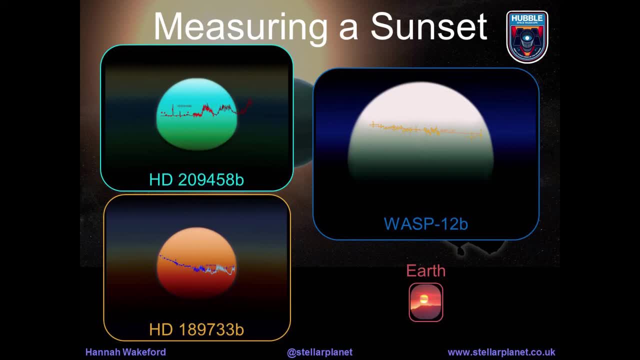 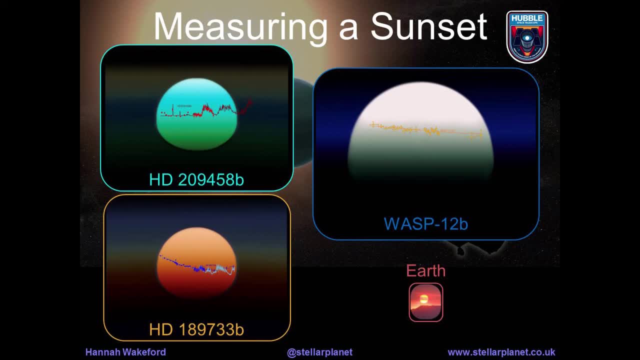 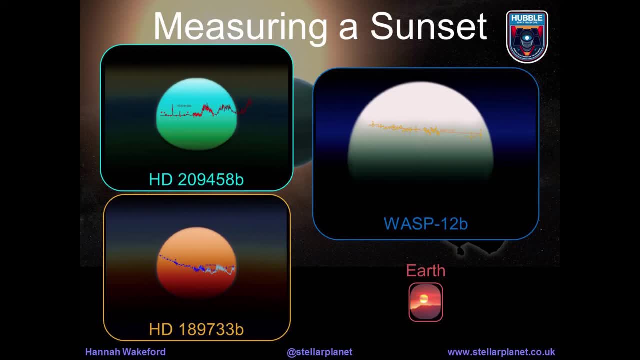 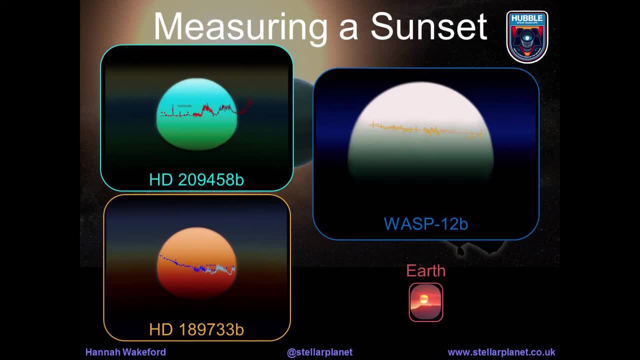 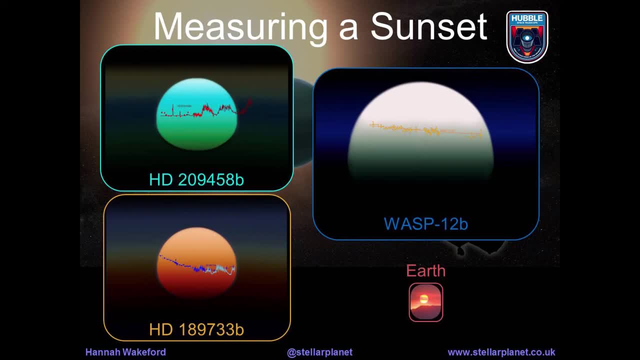 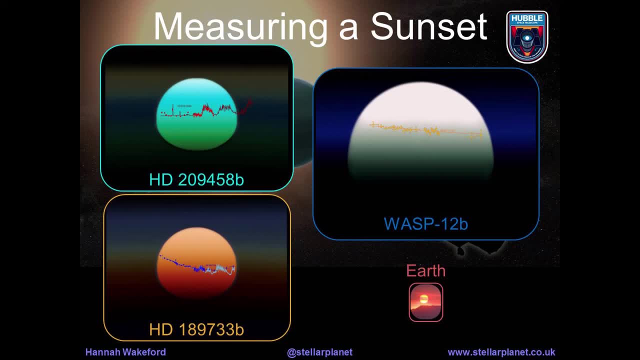 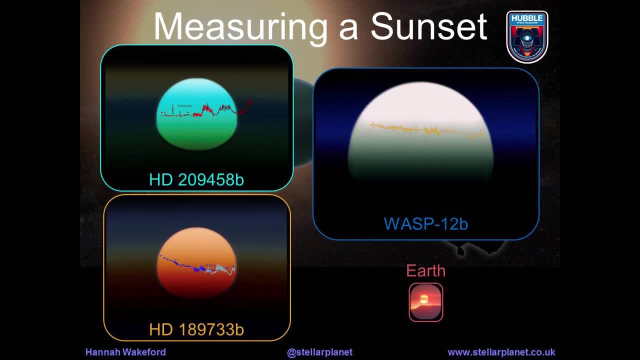 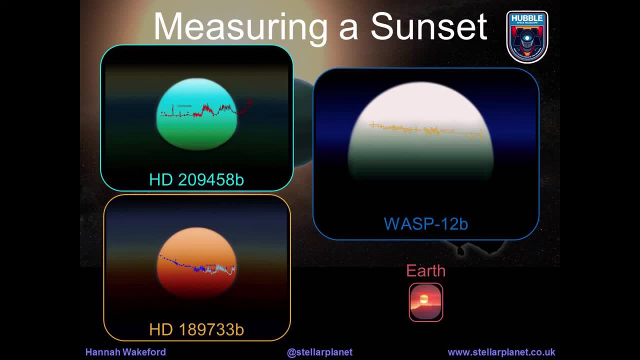 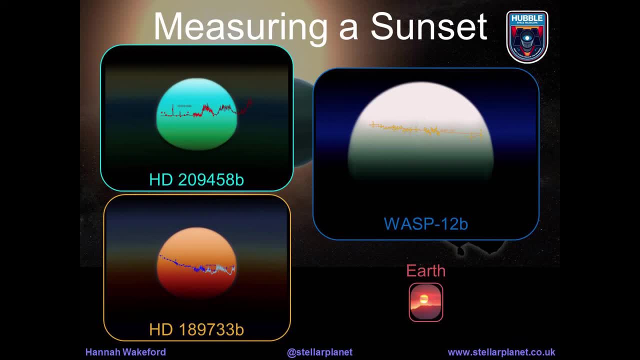 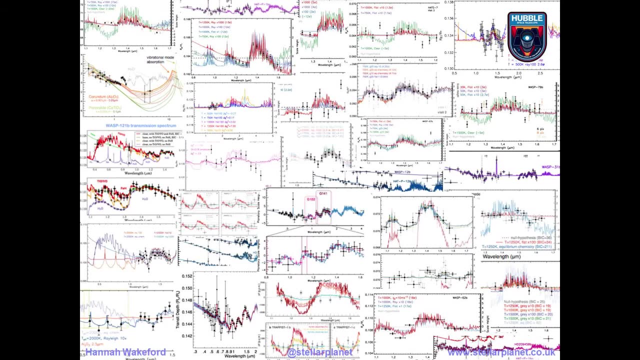 instill exactly what it is I want to really like and what their atmospheres and nature might be like. And this is just a snippet of all of the work that we've been doing with the Hubble Space Telescope. Massive smattering of data for you there. 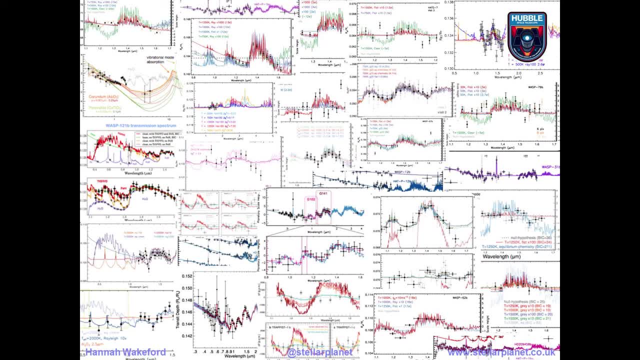 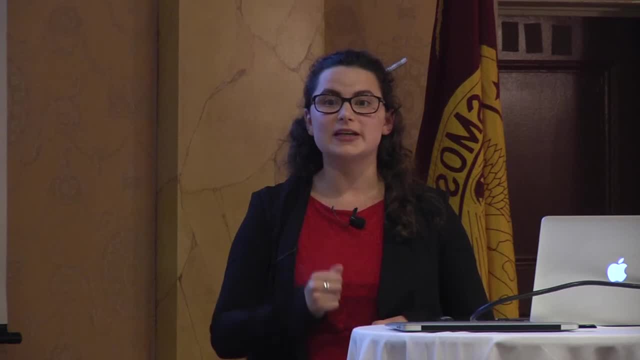 And this represents roughly 40 exoplanets out of the over 3,000 that have been discovered- that we've been able to study their atmospheres, And that is increasing every single year. We have a huge program on the Hubble Space Telescope. to look at 20 more exoplanets. So over the next two years we're going to be getting so much data. But that brings me to. these are giant planets. What about smaller worlds? Now the TRAPPIST-1 system. 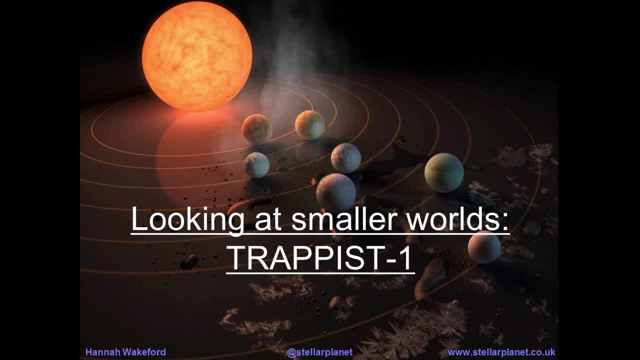 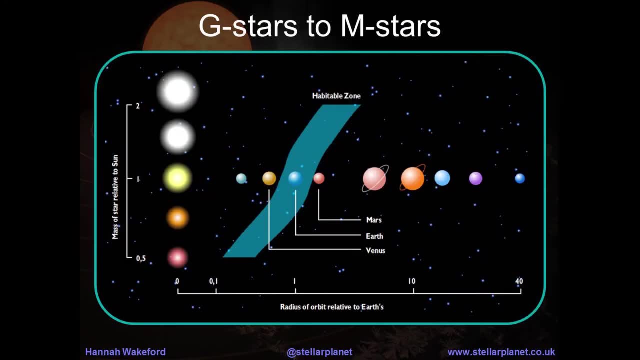 was in the news a lot earlier this year, So I'm going to take you through this really exciting system and hopefully inspire you into learning more about exoplanets. To look at smaller worlds, we need to look at smaller stars And, as Deborah said, 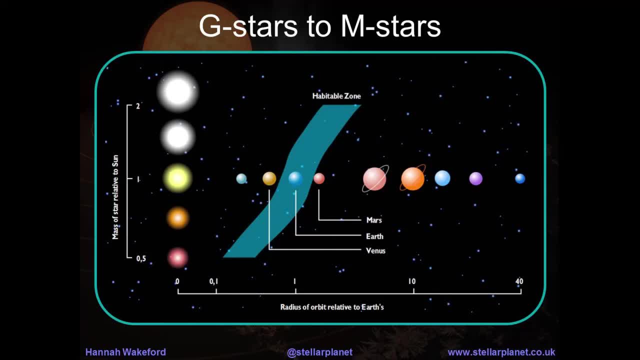 the smaller stars are more abundant in our universe. That's very helpful for us, But they're much harder to look at because they're small and they're faint. They're in the red. But what's also really great about these smaller stars is that as your star gets smaller, it gets colder. 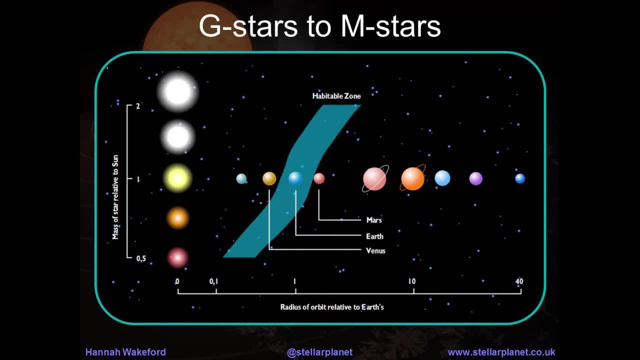 and it pushes this temperate zone, where liquid water can exist, much closer to its star. And the closer the planet is to its star, the easier it is for us to be able to detect multiple transit events And the more transit events we can see. 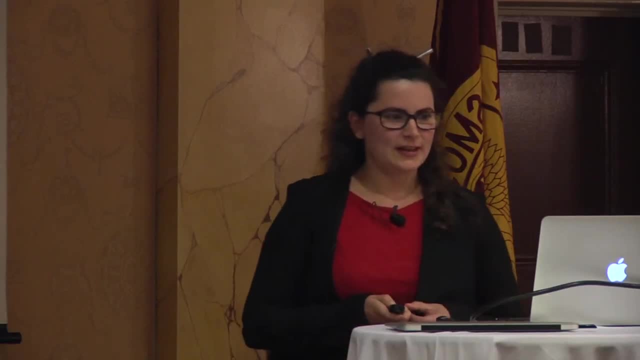 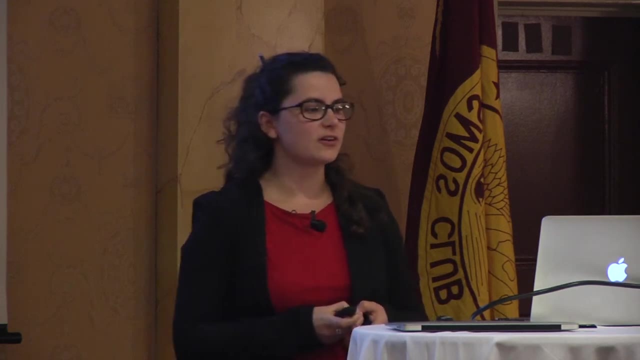 the more times we can try and look at its atmosphere. Now. the beginning for the TRAPPIST-1, the TRAPPIST-1 system was May last year. Just a year ago, this planetary system was announced, where the Belgian telescope TRAPPIST. 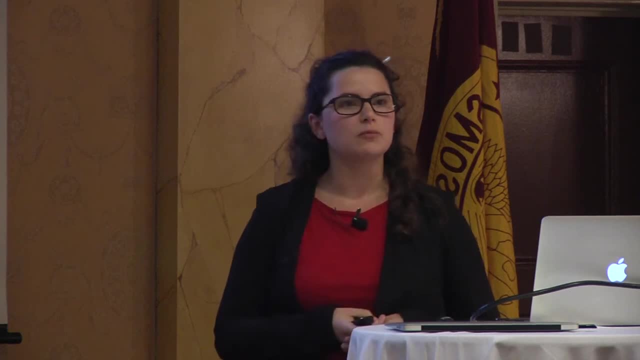 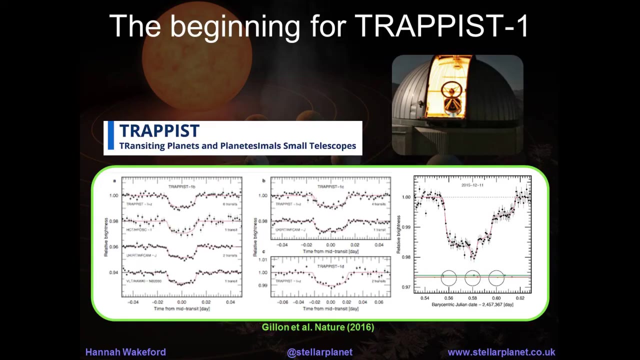 discovered TRAPPIST-1,, a ultra-cool M dwarf with two and possibly a third planet orbiting it, And what you can see here are those detection transits. So TRAPPIST-1b, the largest and innermost planet. 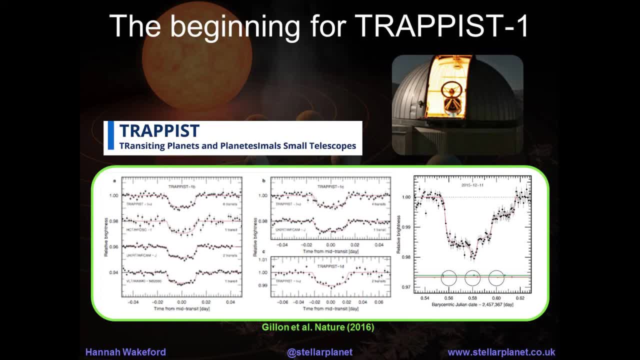 TRAPPIST-1c and then this strange light curve here This is multiple planets passing in front of the star all at the same time, And we took the opportunity on May the 4th last year to point Hubble at an event. 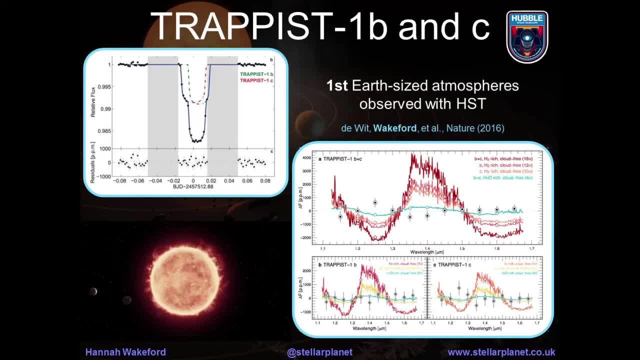 a special event that only occurs every two years. We looked at these two planets, b and c, as they passed in front of that star at the same time, to search for signatures of a large hydrogen envelope around these planets. Now, the reason we're searching for this is because small planets could. 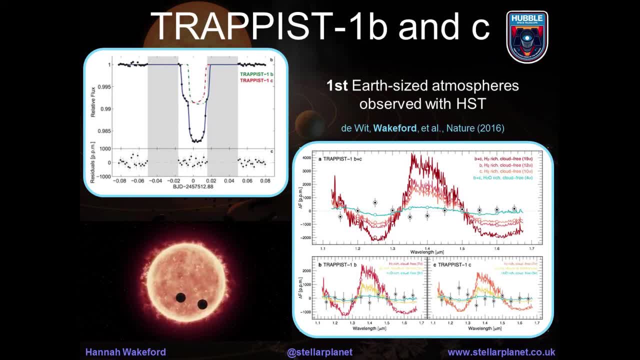 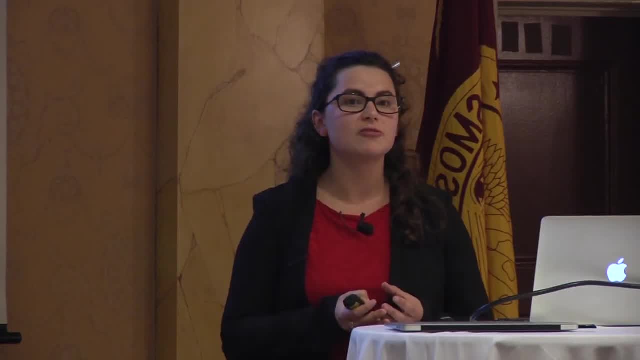 maintain lots of hydrogen around them in an envelope. Hydrogen acts as a greenhouse gas and will change the environment on that planet. So we're trying to understand whether or not these planets have that envelope around them From this observation with the Hubble Space Telescope. 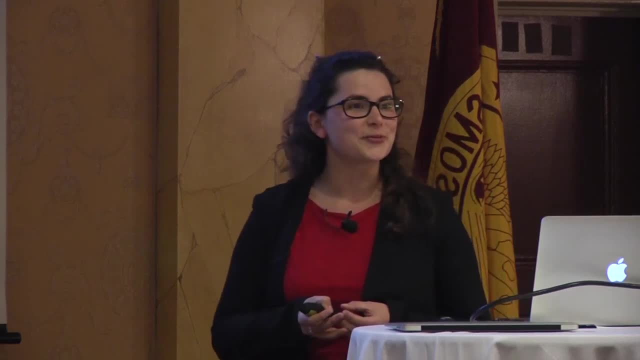 we found that b and c do not have this hydrogen envelope around them, And that's really interesting. That takes us to further studies, trying to understand what their atmospheres are like, And it actually lends. it tells us that these are likely terrestrial. 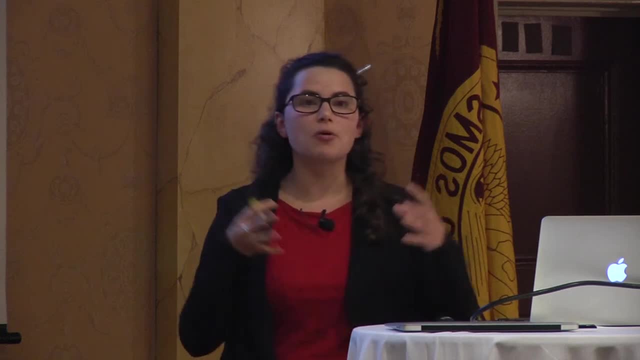 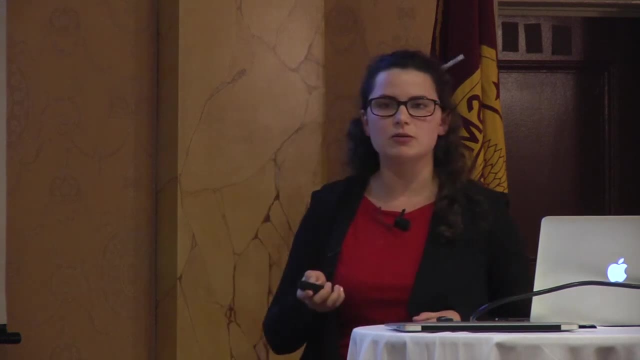 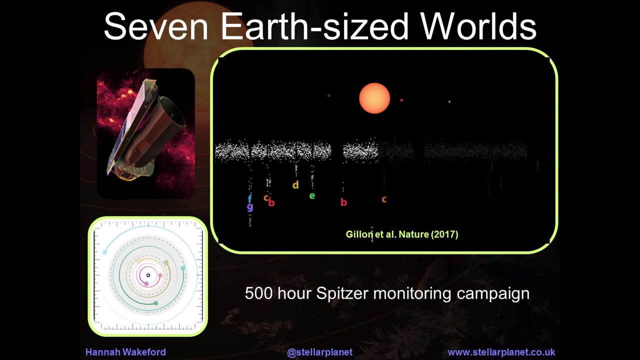 but in nature, ie they are rocky and they have compressed atmospheres. But then we got another exciting thing from the TRAPPIST-1 system: 500 hours of Spitzer Space Telescope time observing this planetary system, And from that we discovered that the third planet in that system 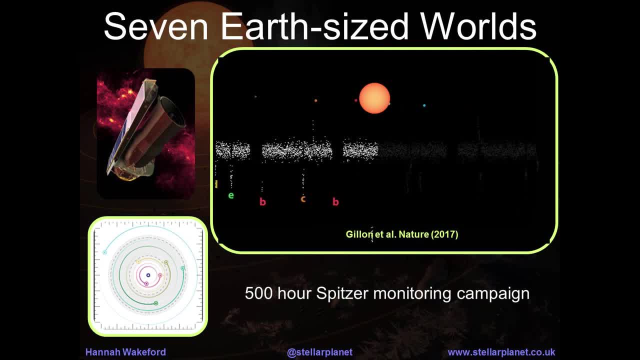 was not one planet, wasn't two planets, it was five planets. Five planets in addition to those two inner ones that we'd already looked at And you can see in this amazing video here. this is the real data from the Spitzer Space Telescope. 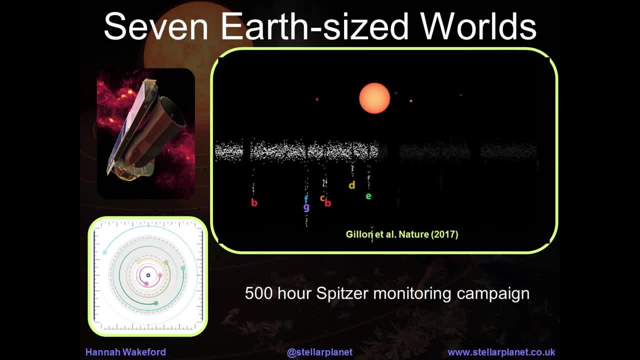 passing underneath And this is a simulation of those planets as they pass in front of that star. So we're able to detect seven planets in this system, Not giant planets, not like our solar system. These are all Earth-sized worlds, Seven Earth-sized worlds orbiting one star. 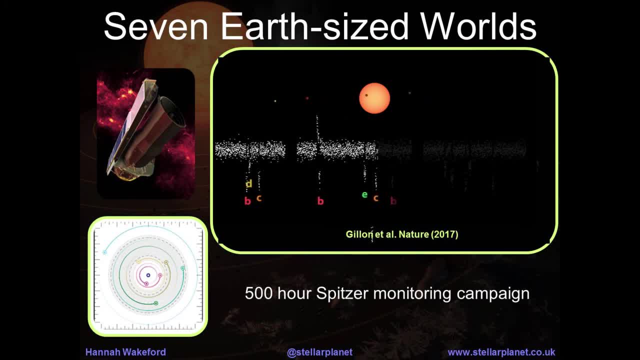 That's a gold mine for the type of work that I'm doing. Seven planets around one star takes the star out of the equation. We're then comparing the planets to each other and comparing the atmospheres to each other. That tells us huge amounts about the impact. 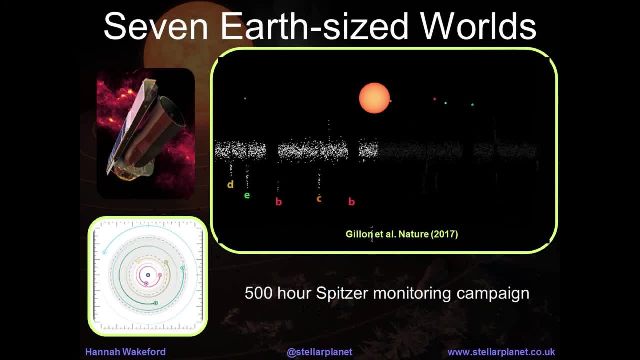 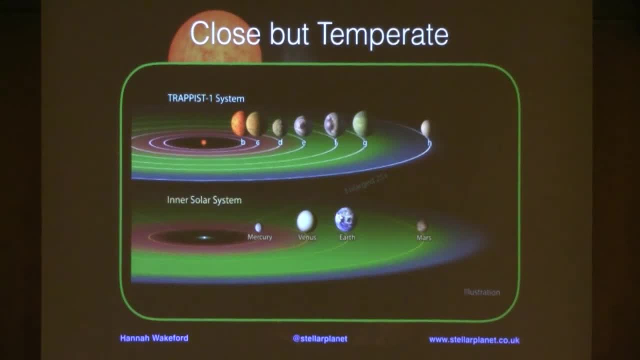 of different planetary interactions and stellar interactions, But also because this star is so small- it's an M-dwarf. This temperate water zone, liquid water zone, is much closer to its star And if you place it in the context of our solar system, 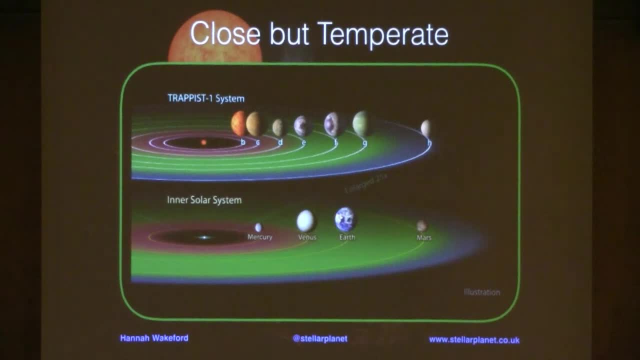 the TRAPPIST-1 system is 40 light-years away, But if you place the planets in the context of the solar system, of our solar system, they all fit inside the orbit of Mercury. So they fit down in this tiny little gap right here. 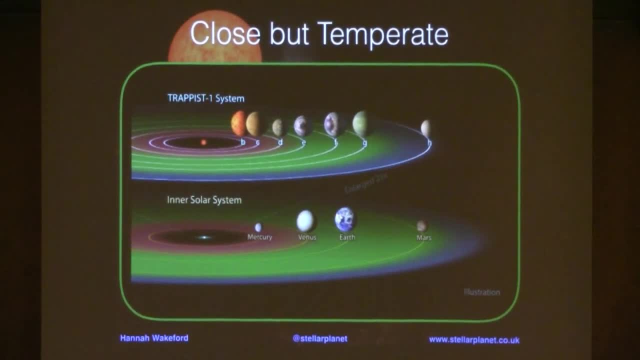 All of the planets, seven Earths that close to the star. And at this distance from the star we see this transition from the hot inner part of the system to the middle temperate part, where the water can turn into a liquid and pool on a surface, if there is a surface. 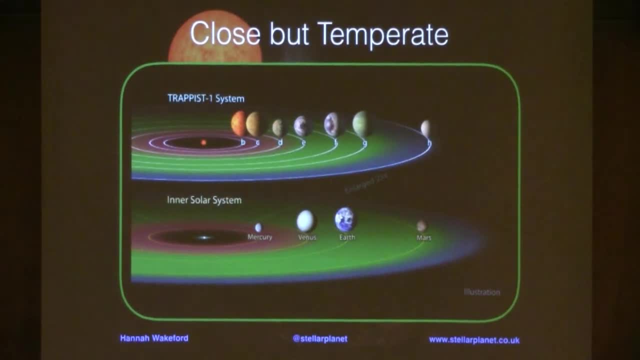 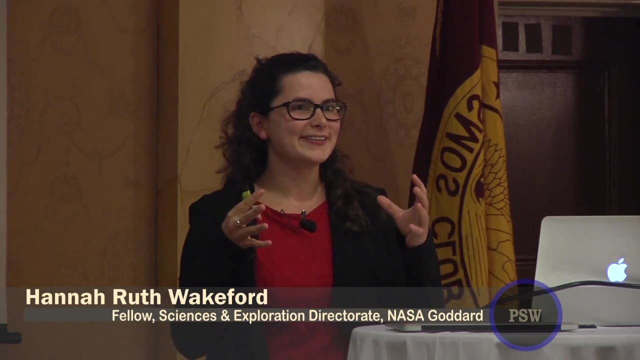 And then further out, where you get the ices forming out by H. So, even though this is much closer to its star, it's actually because the star's cooler. They're in exactly the same zone as our terrestrial planets. Amazing, amazing system. 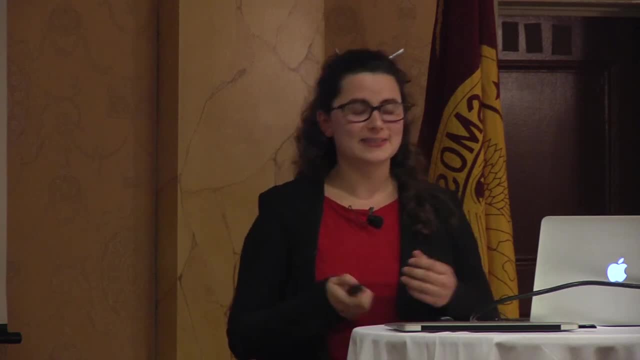 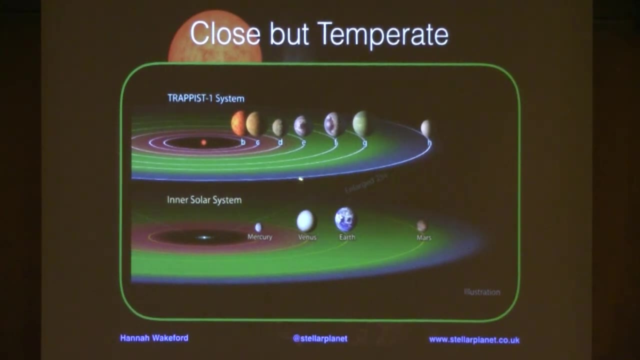 And actually we are currently looking at these four planets here which span this temperate water zone. We're looking at those with the Hubble Space Telescope now to try and determine if they have this hydrogen envelope around it. The further away from the star, the more likely. 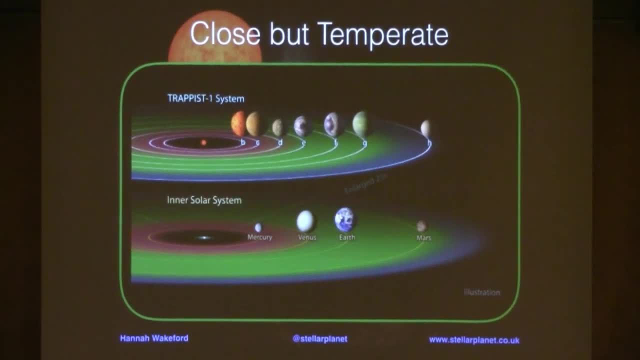 that that planet can maintain that hydrogen envelope. We can learn about that and that process with seven planets roughly the same size, roughly the same mass, all around the same star. It's a fascinating, fascinating puzzle that we are really working to try and figure out. 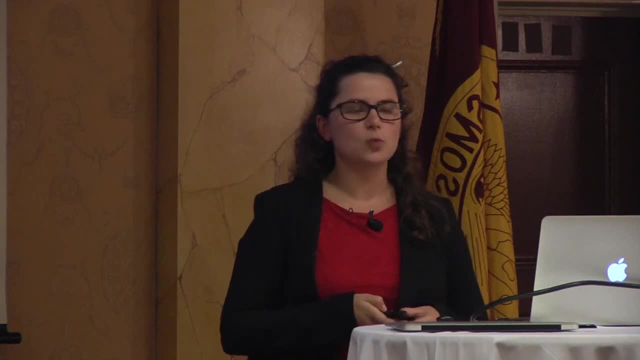 And that takes me forward to the era of the James Webb Space Telescope. And just to give you a little bit of information about the James Webb Space Telescope, we're going to go to the James Webb Space Telescope. It has a 6.5 meter primary mirror. 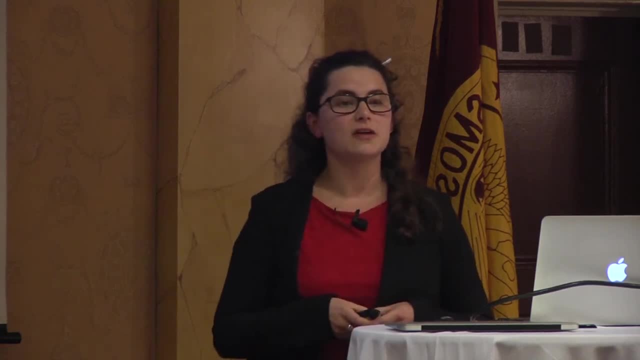 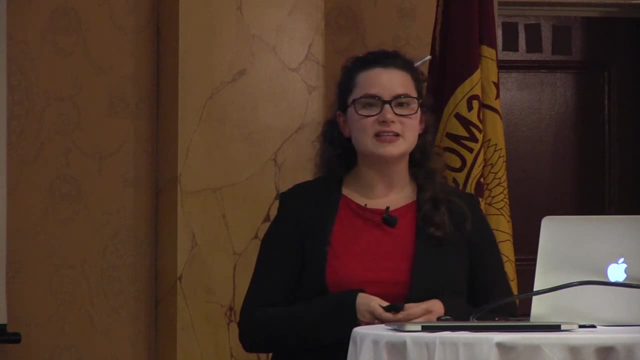 That is the largest telescope that will ever be launched into space. It's so big we don't have a rocket that can take it there. It has to be folded up. So it is made of 18 segments, plated and covered in gold. 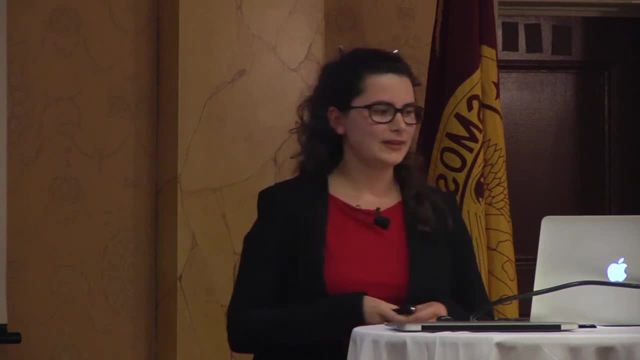 Enough gold to make a nice-sized golf ball. It has seven times the collecting area of the Hubble Space Telescope, And this will allow us to do a lot of work with it, And this will allow us to do a lot of work with it. 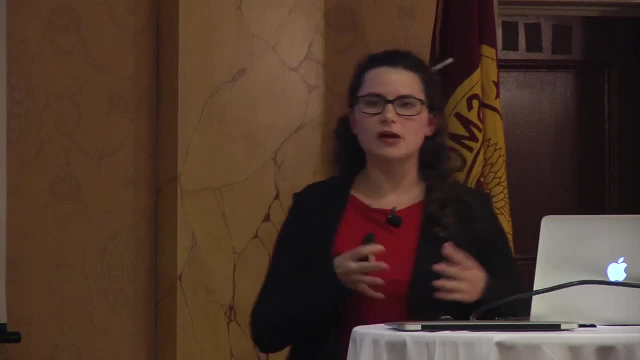 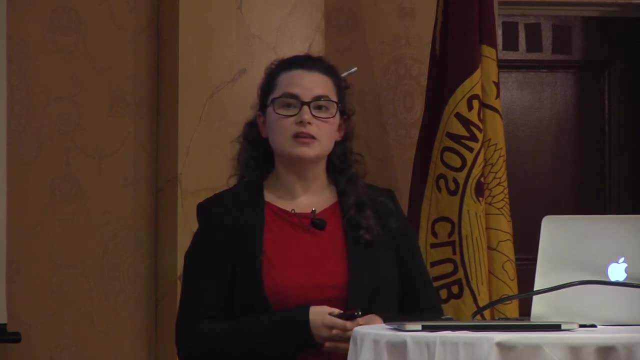 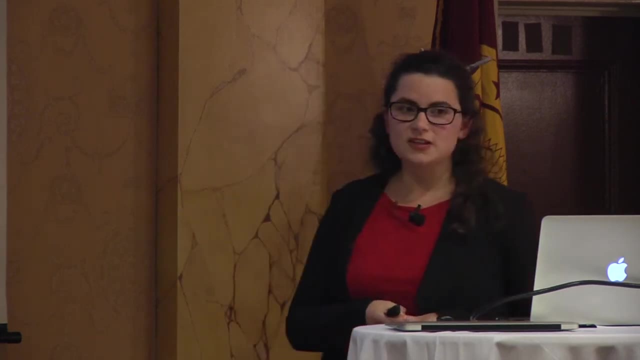 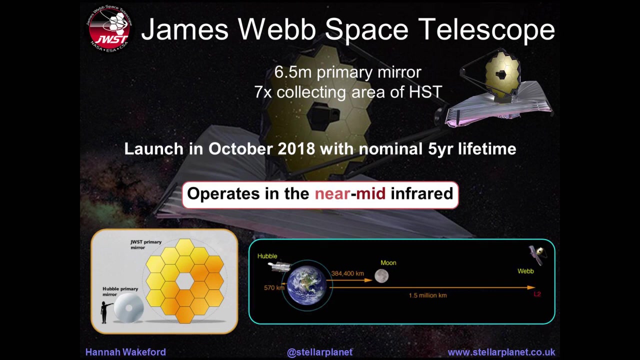 infrared and the mid-infrared, whereas the Hubble Space Telescope operates in the near UV- at the optical mostly- and the near infrared, and you can see in this figure at the bottom here the size of the Hubble Space Telescope's mirror compared to the James Webb Space Telescope. This is an 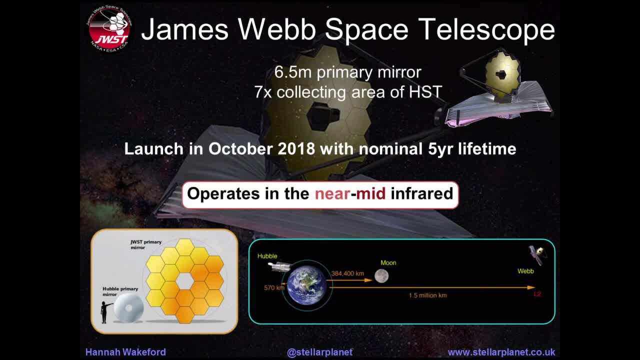 unbelievable feat of engineering, and it happened just near here at the Goddard Space Flight Center, which is unbelievable. It's also not going to be orbiting the Earth like the Hubble Space Telescope. It's going to be a million miles away at the L2 point, and this is a gravitational 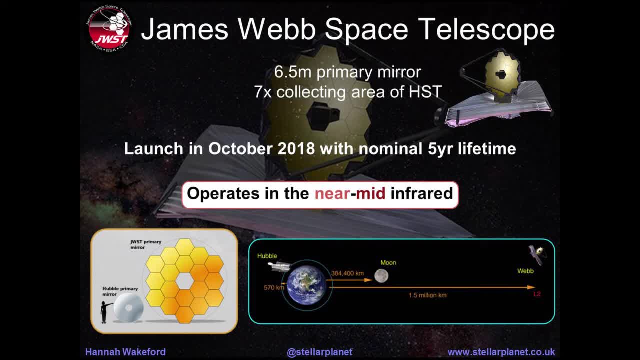 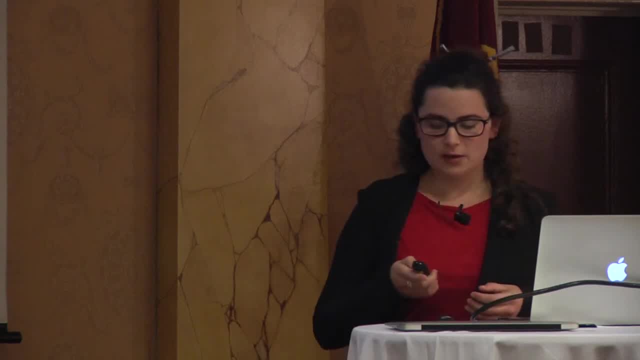 stability point which allows it to be pointed away from the Earth, so we don't have to deal with the Earth's heat and the Earth's light. Now, what is Hubble going to be looking at? Sorry, the James Webb Space Telescope. What is the James Webb Space Telescope going to be looking at? This is a simulation of 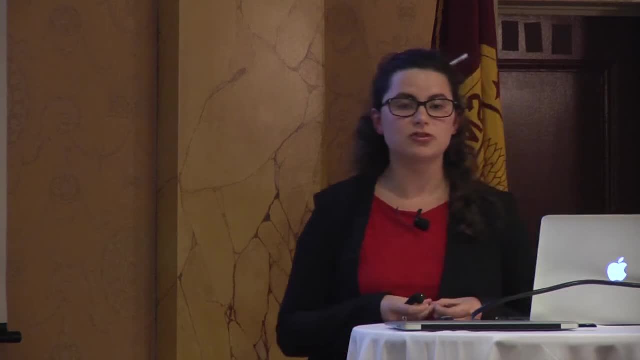 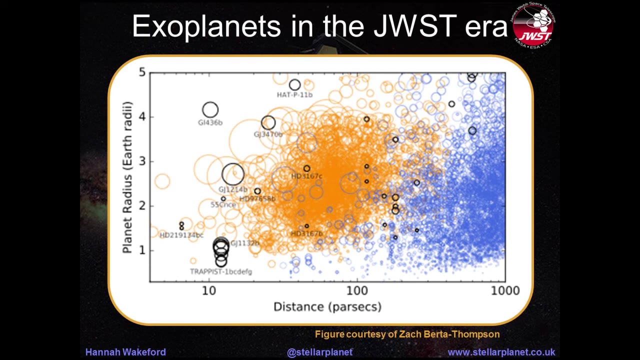 planets that the TESS satellite, which will be launching in March next year. TESS stands for Transiting Exoplanet Survey Satellite and TESS. we expect it to be able to find bright stars with planets that are small around them, and what we can see here is: oh, that was me. 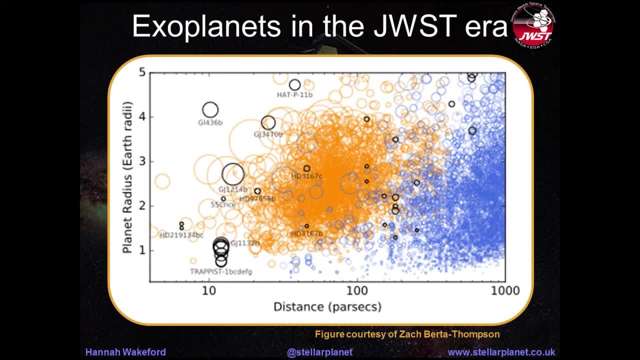 what we can see here is the radius of that planet. so this is using the transiting method. so the radius of that planet- up to five times the radius of the Earth- and the distance that planet will be, that star will be from us. And what you can see down here in orange is 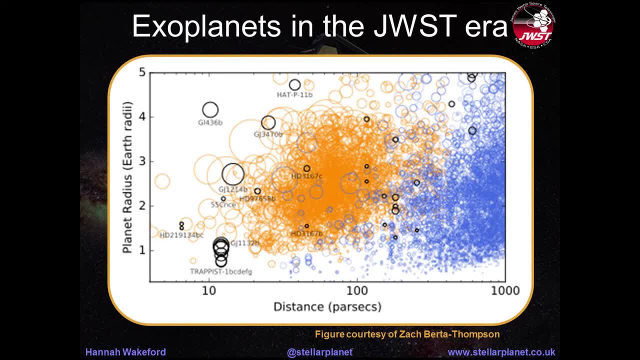 what we expect TESS to be able to discover, for us to explore, and, in blue, what Kepler has discovered. And what is absolutely brilliant about this is right down here, in the best spot, with the largest circles, and the circles mean that it's much easier for us to do this detection. 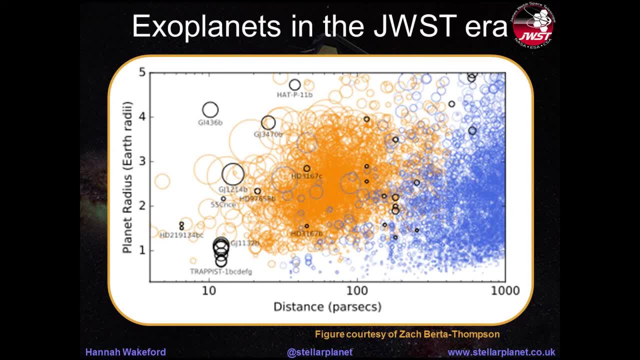 is the TRAPPIST-1 system. They are the perfect candidate for us to point the James Webb Space Telescope at and try and understand their atmospheres. The James Webb Space Telescope is going to give us huge amounts of information, But what also wasn't expected is Hubble to. 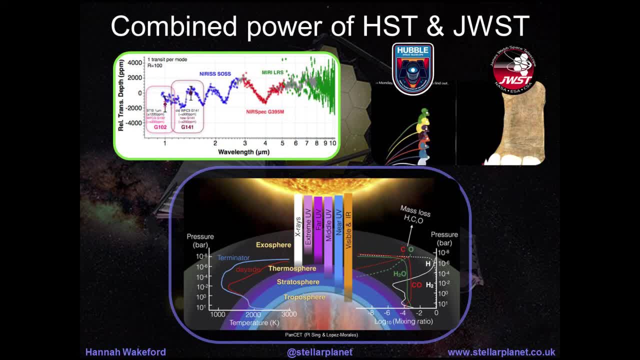 last this long and be such an amazing workhorse for transiting exoplanets. The combined power of the Hubble Space Telescope and the James Webb Space Telescope is going to be a huge advantage for us to be able to explore and try and understand their atmospheres. The 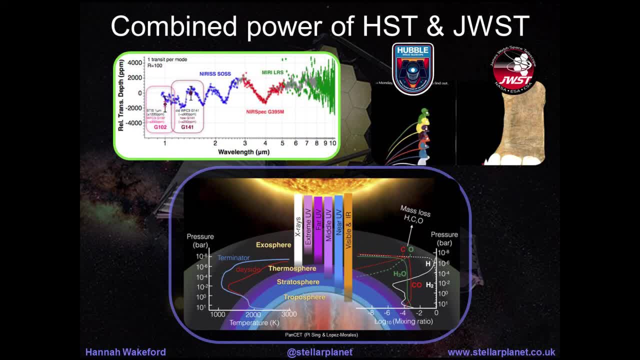 Hubble Space Telescope will get us observations from the UV through the optical all the way out into the mid-infrared. This gives us information on the water content of an atmosphere, the carbon dioxide content of an atmosphere, the carbon monoxide content of an atmosphere. 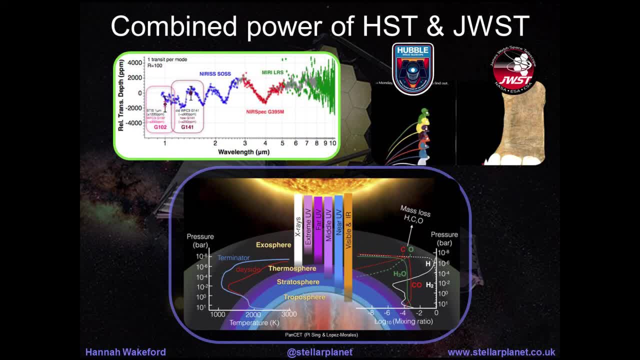 We can understand huge amounts of stuff about a planetary system, And this is just one simulation that we have of a giant exoplanet, with one single observation for each of these colors that you can see here. This is one of the simulations that we're going to be able to get for a giant planet. 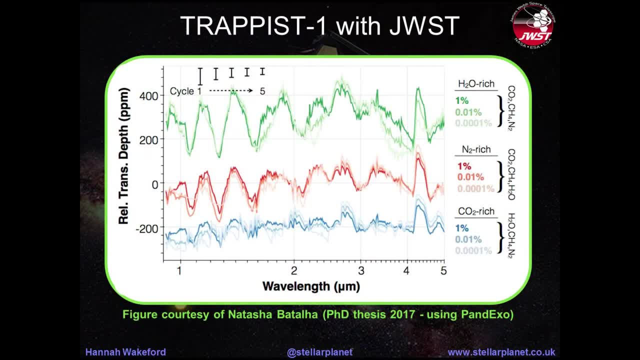 Now what I'm showing you here is simulations by Natasha Batalia, who is also at Goddard Space Flight Center and will be defending her thesis very soon, of the TRAPPIST-1 planet. This is taking an example of TRAPPIST-1F, which sits happily in its temperate water zone. 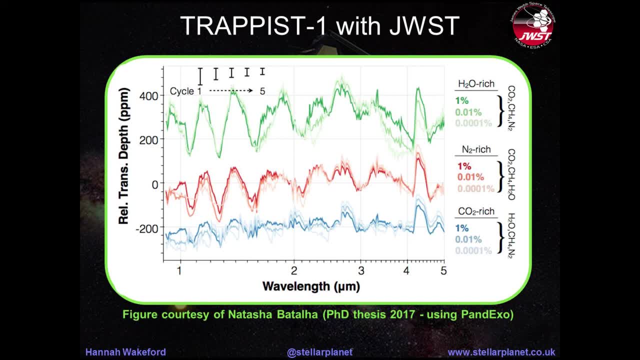 And this is a simulation of water rich atmosphere, a nitrogen rich atmosphere and a carbon dioxide rich atmosphere, And what these little bars at the top are showing is that, quote unquote. there are so many different things at this planet. This is a simulation of both: a water. 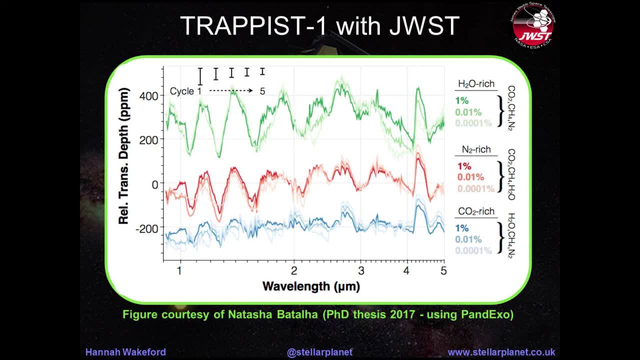 at the top are showing you is after one year of observation, so 10 transits. this is the error bar that you will get with the James Webb Space Telescope And as you go through and get 10 more with each successive year, how the error bar goes down. 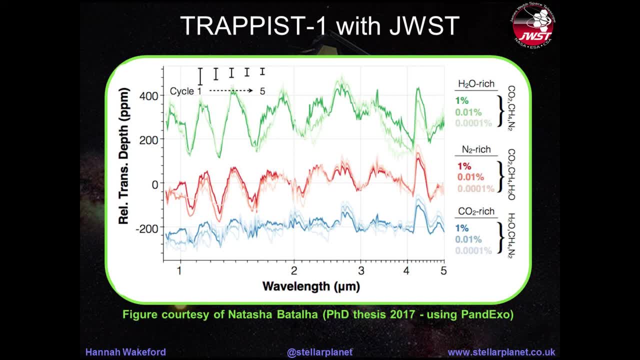 And if you look at the differences between each of these models, you can see that after the second cycle of the Hubble of the James Webb Space Telescope, we'll be able to understand whether or not these planets have a H2O-rich atmosphere. 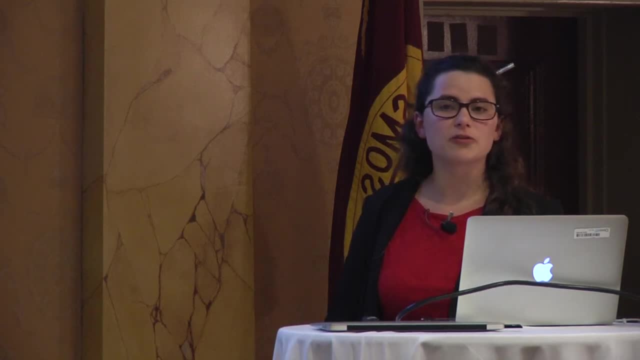 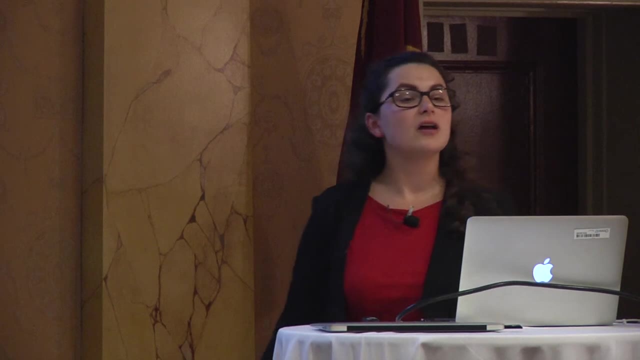 That's something that we never thought was possible, And it wasn't even thought possible when they were designing the James Webb. So this is going to be a fantastic era for exoplanets, our understanding of the environments of other worlds, which gives us the big question we want to answer. 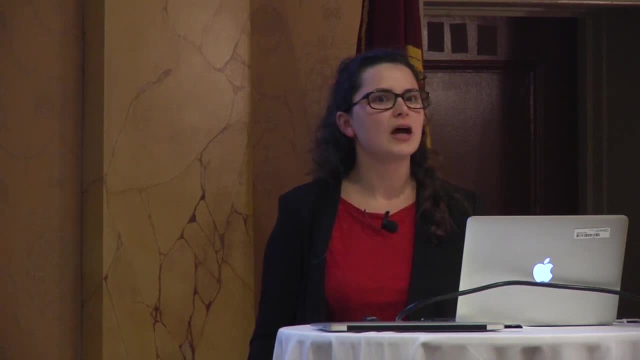 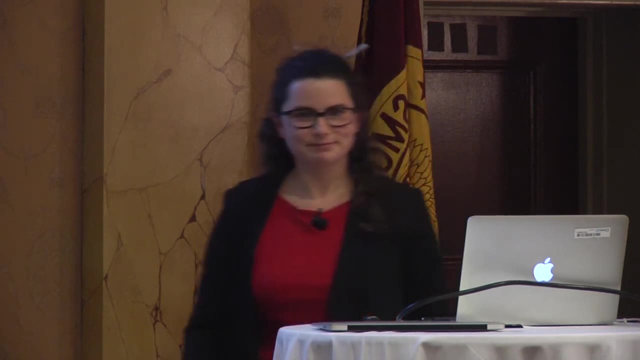 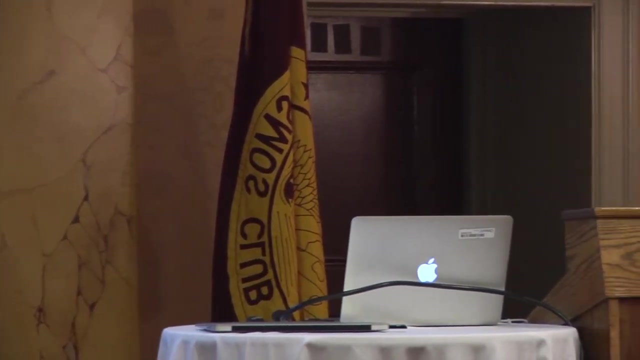 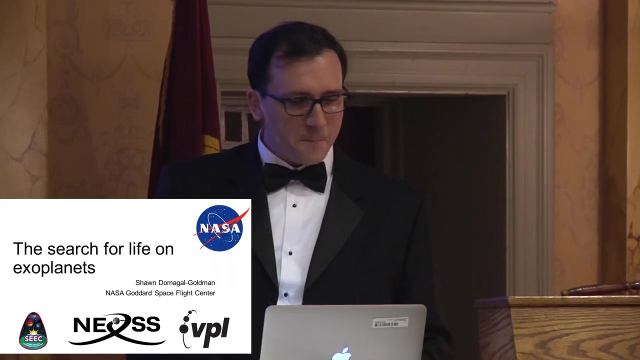 How easy is it to form a solar system like our own and a planet like our own, And what are the environments we should be expecting For other planets? Thank you, Well, thank you for having me here tonight. I'm quite happy to be following that talk by Hannah Dr Wakeford. 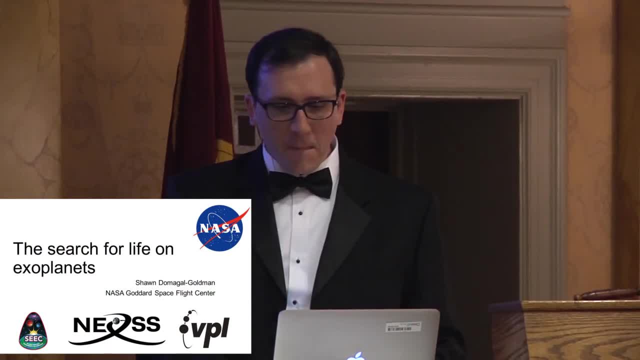 and the previous talk by Dr Fisher, because I've been awed by the ability of my colleagues to understand and characterize the astrophysics and the physical nature of these worlds, as Dr Fisher talked about, and to start to understand their chemical nature. 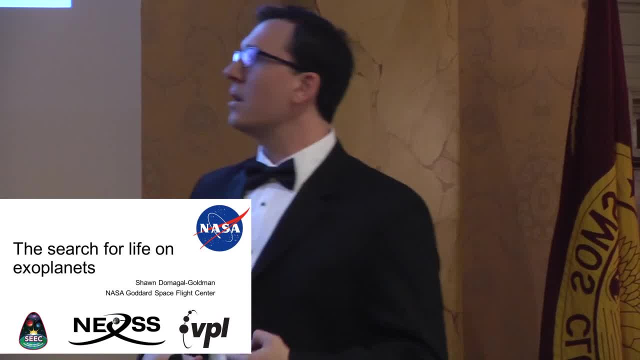 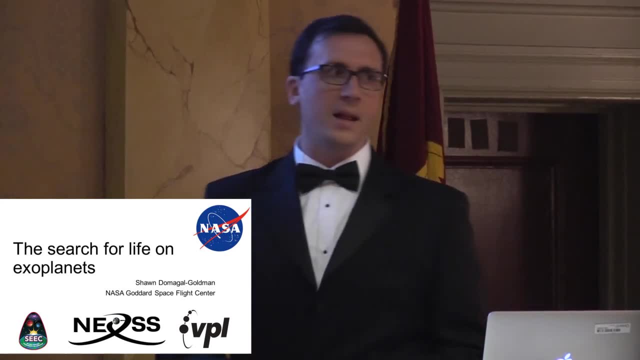 as Dr Wakeford just talked about, And part of what's so exciting about these Trappist worlds is they may provide us with the first opportunity to characterize them from an astrobiological standpoint, to do chemical characterization on worlds that are small enough. 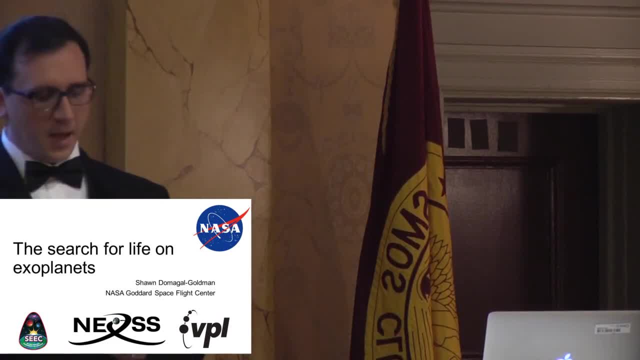 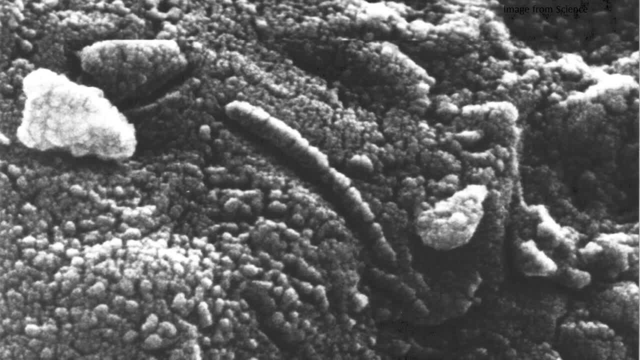 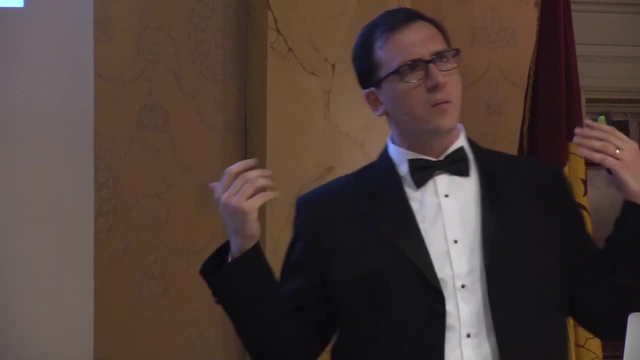 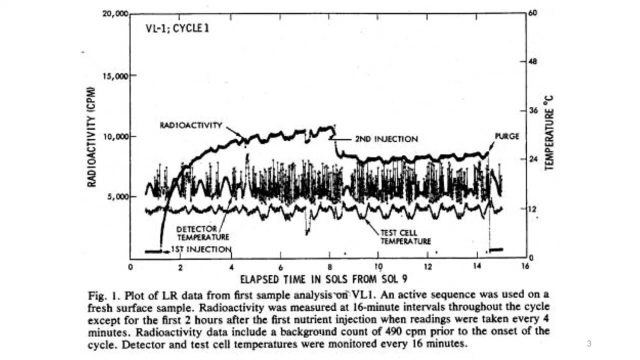 Dr Wakeford, I'll be right back. You can go back to Viking, the first time we did a direct search for life as an agency at NASA, on another planet, And Gil Levin, the person who designed and led the instrument that made this. 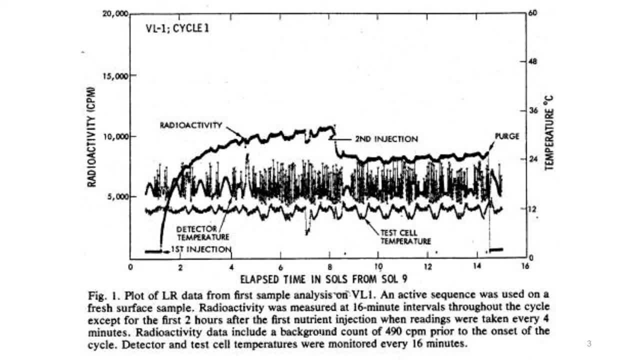 measurement which looked at the radiolytic release of carbon. they basically took radioactive carbon to the surface of Mars and gave that as nutrients to the soil and basically waited to see if that radioactive carbon and the nutrients baked off his gas. and sure enough it did: They got a positive. 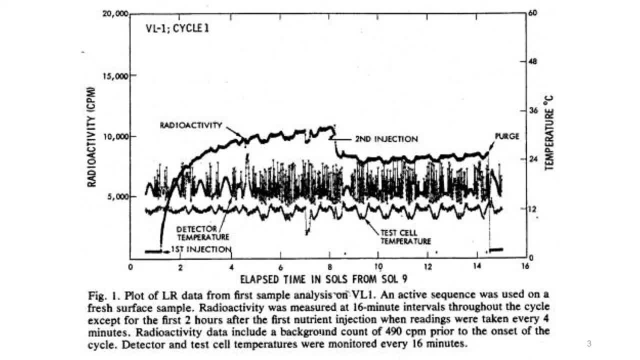 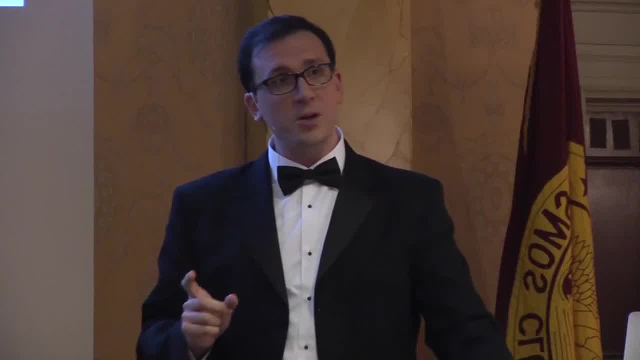 result, And Gil Levin, the PI of this instrument to this day, will tell you that he found the first evidence of life beyond Earth. I will also say that I don't think the astrobiology community in large agrees with his assessment, Unless you think I'm picking on the Martians. 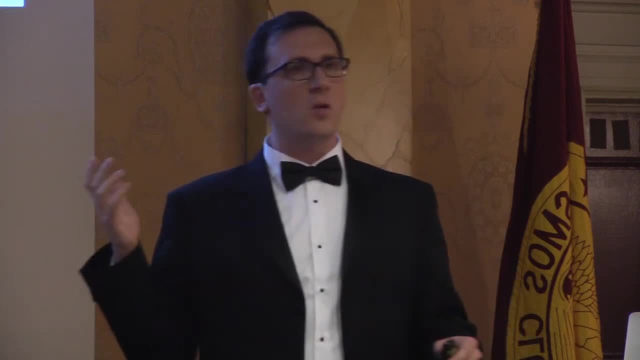 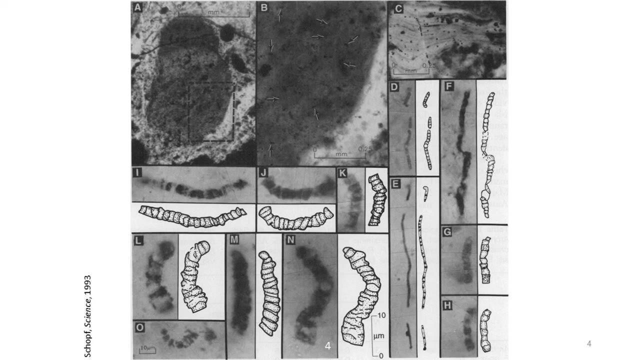 this has also been a problem through Earth history. If you want to know what the earliest signs of life here on Earth are, you could go to the literature. And, by the way, if you want to see outstanding and sometimes pointed scientific debate in the literature, look at the microfossil. 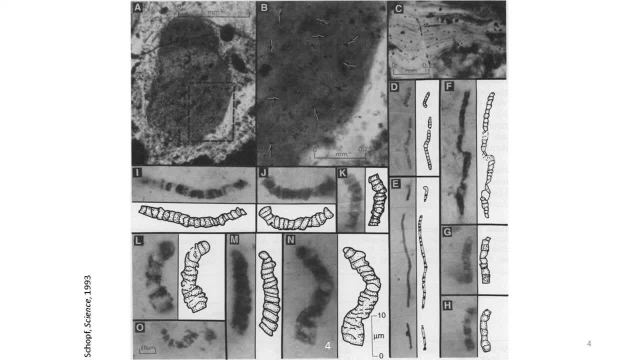 story for the earliest evidence of life on Earth. These are putative microfossils that another researcher called dubiofossils, because they did not believe that they constituted the earliest evidence of life on Earth. So the point to this, before I get into the search for life on exoplanets. 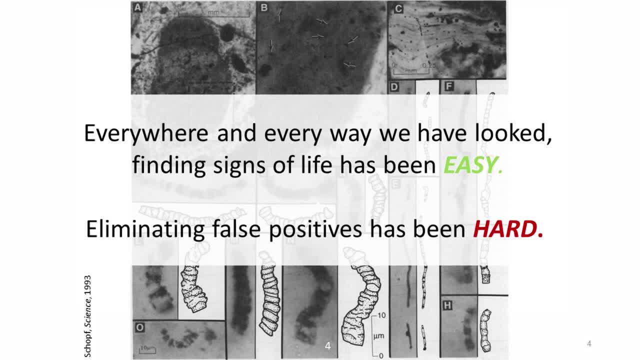 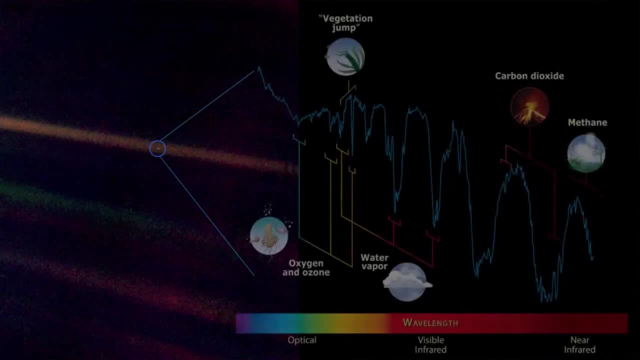 is almost everywhere we've looked and in almost every way we've looked, it's been easy to find signs of life. What's been difficult is to rule out the ways in which non-biological processes can make the things that we're looking for, that we think could only come from life, And so we go to the pale blue. 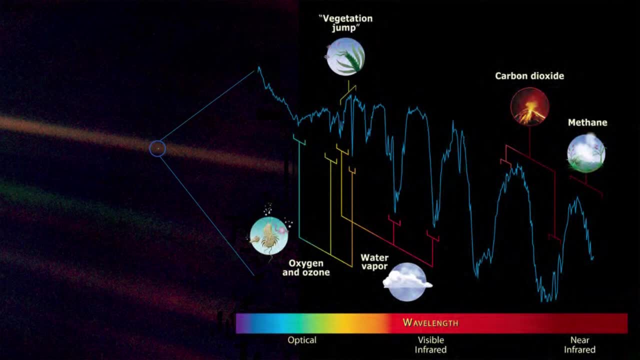 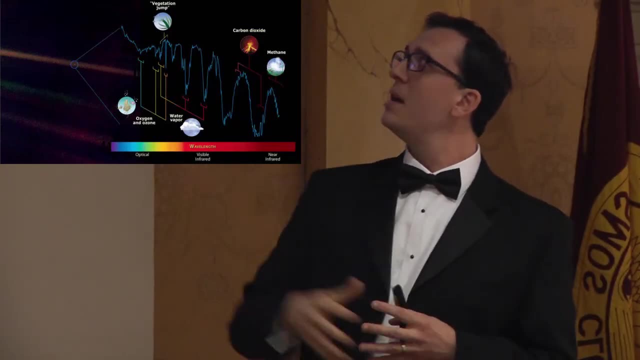 dot that Dr Fisher showed earlier, And this is the data. these are the data that we're talking about getting a spectroscopic signature- okay, just photons from that one pale blue dot. We won't get spatial resolution, at least not with the first generation of telescopes we do this with. 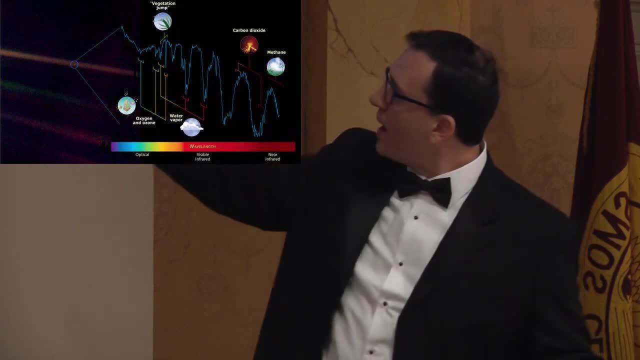 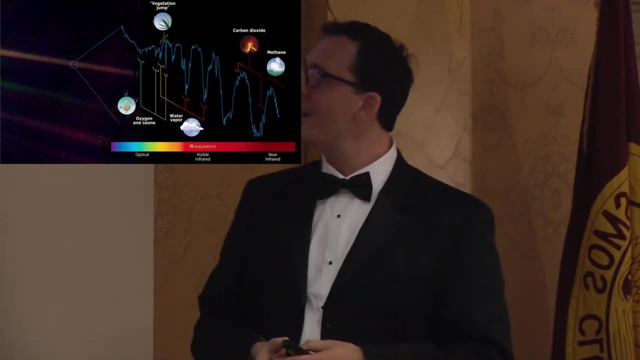 But we will get spectral resolution. We'll be able to spread that pixel of light out on a detector array based on its color, almost like it went through a super high technology prism to see what colors are there and which ones are not. 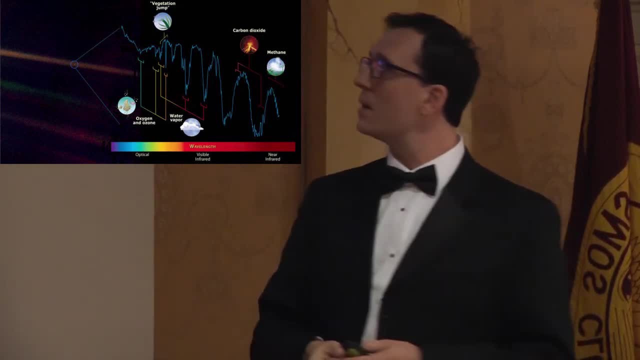 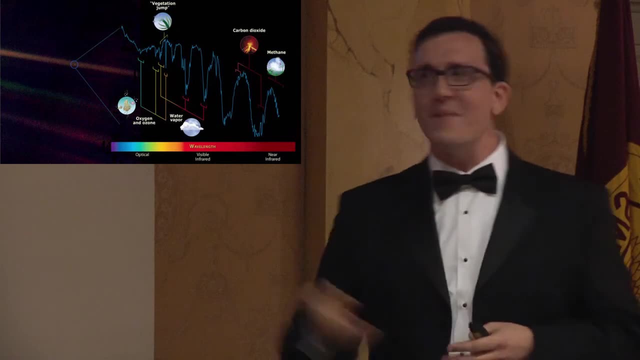 And based on the colors that are absent, we're going to say certain gases are in that planet's atmosphere And if we find oxygen or ozone, and if we find methane, and if we find liquid water, we say okay, there's life there, because life makes oxygen and oxygen does not like to stick. 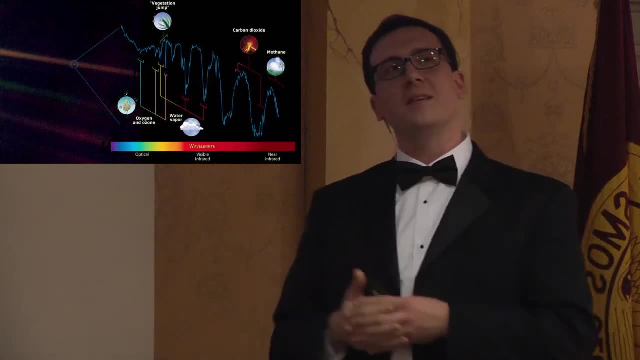 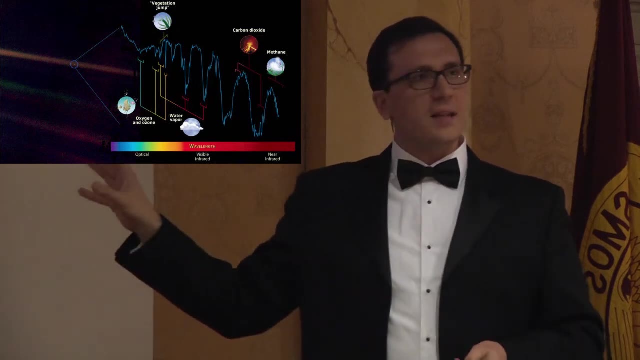 around in the presence of methane, And so you can only replenish that oxygen if there was life on it. You can only have that oxygen there if there was something like life replenishing it rapidly. Now I still think that story stands, but when we talk as astrobiologists to instrument designers, 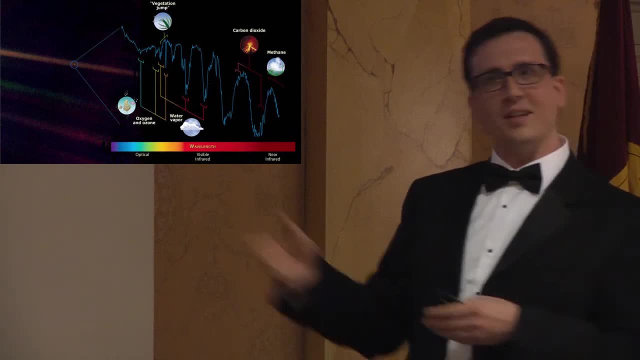 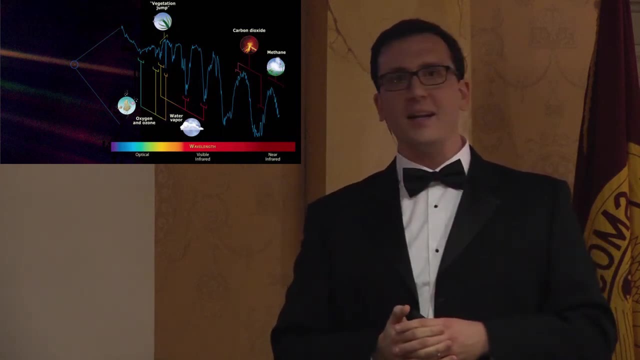 or engineers. they might say: well, just tell us what wavelength you want to find the oxygen and we'll design an instrument to go and get that wavelength of light. And so, just you know, give me your two gases and the wavelength range that I need for them. 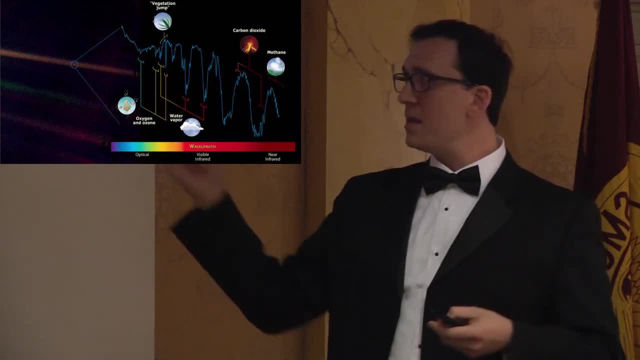 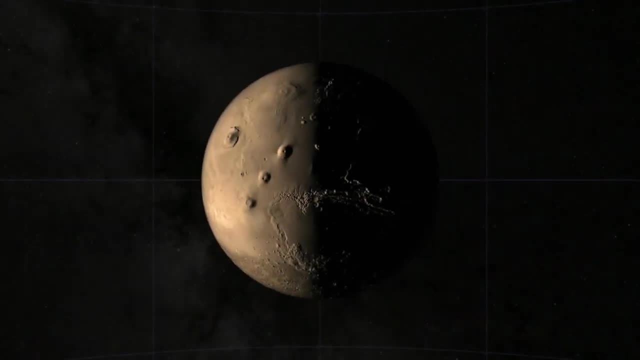 and then I'm going to go design an instrument to see them. As an earth scientist and someone that knows that story of the false positives, I think, well, it's not that simple context, So I'll come back to this a bit later. And I think about the TRAPPIST systems when I 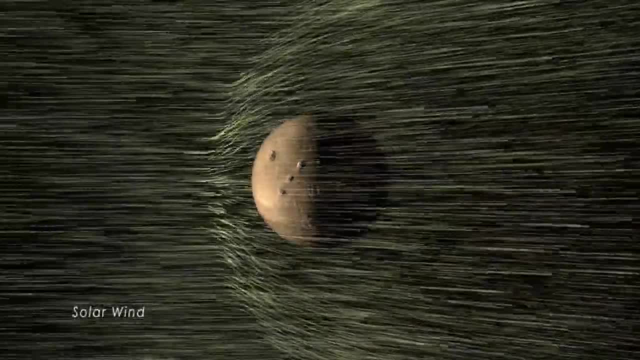 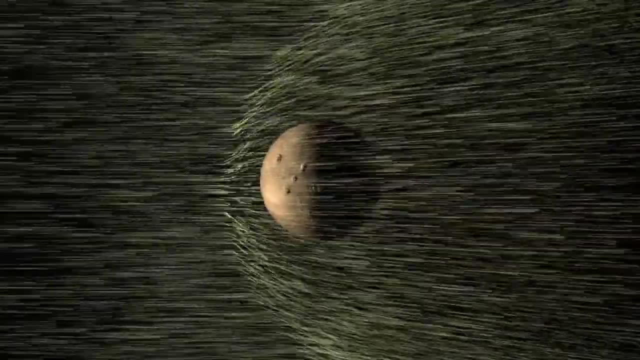 think about context as well, because if we want to do a search for life, the lesson for me from the Ellen Hills meteorite on Mars is that you had to interpret the data, those fossils and the mineralogical data and the isotopic data in the context of the rock. Well, for exoplanets, our 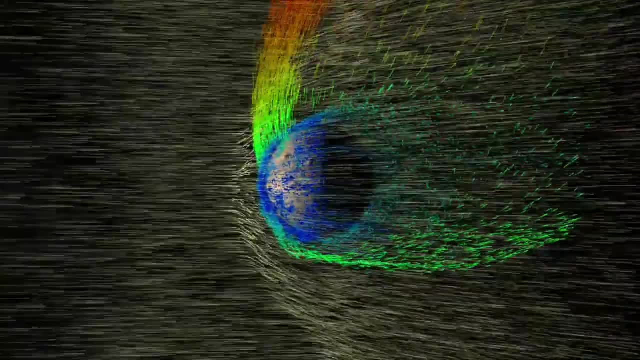 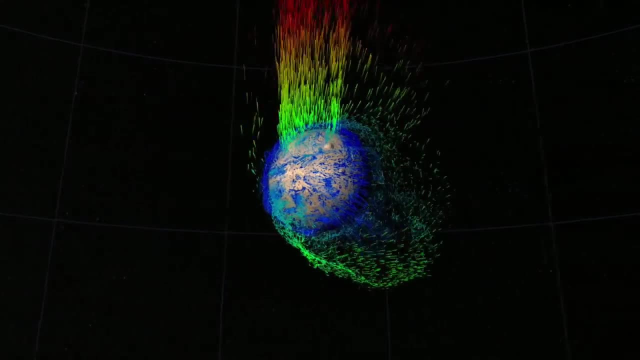 context is going to be the entire atmosphere. It's going to be the entire planet. in a sense, This is a simulation of real data from the MAVEN spacecraft that's in orbit around Mars right now And it's in a special orbit where it can look at things escaping from the Martian atmosphere. 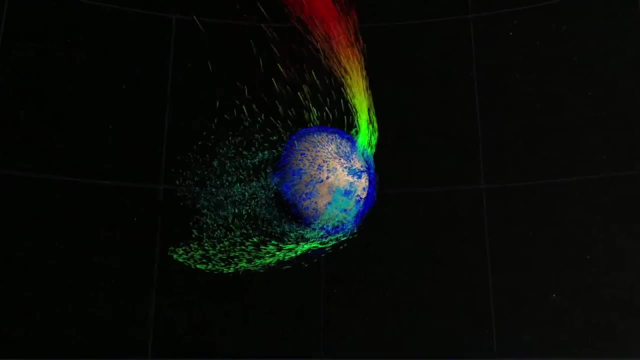 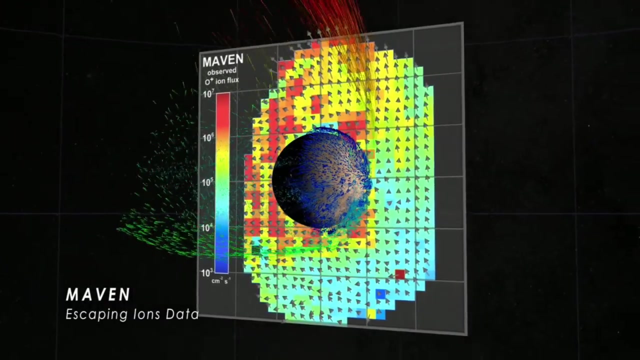 specifically ions of many things. This is a map of oxygen And what happens is, as Mars gets hit by a stellar wind, by the high energy radiation released from the sun, that can ionize the molecules in Mars's atmosphere and lead them to be stripped away along magnetic field lines. And 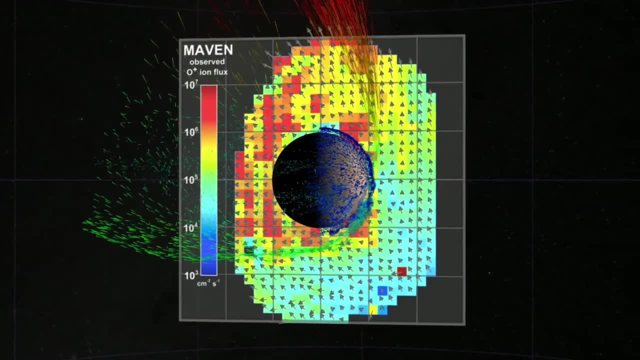 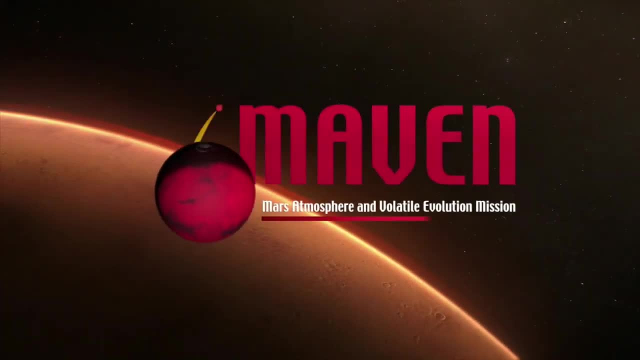 it can also impact the magnetic field lines. And it can also impact the magnetic field lines Which can accentuate that process. And I point this out because habitability is going to be something for exoplanets, where the context of it is not some rock, It is the entire planet in the 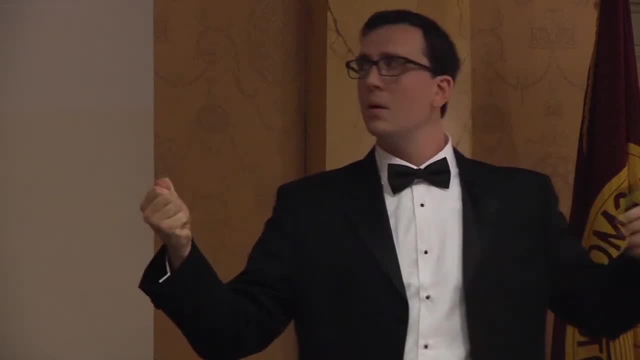 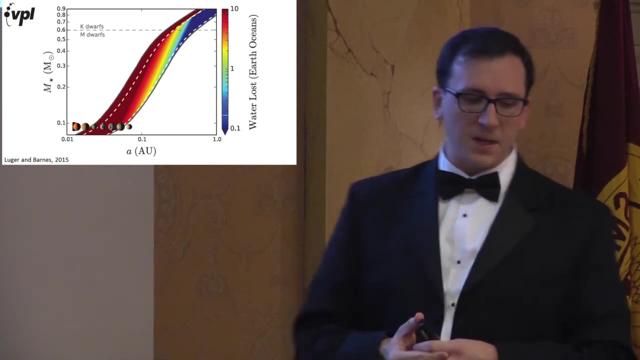 context of its star and also the neighbor planets. So I worry about this process, in particular for the Trappist worlds and other worlds we're going to look at soon for signs of life with the James Webb Space Telescope, because that process might be more efficient on planets around the world. 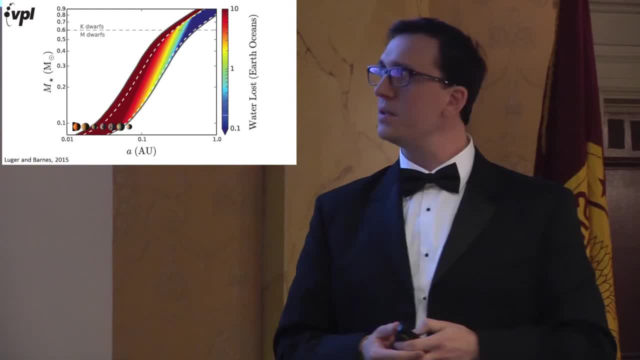 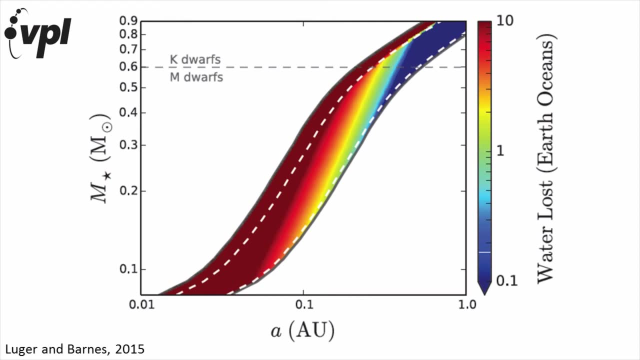 So this is a map or a diagram of this is the mass of a star on the vertical axis and the distance of a planet from that star on the horizontal axis, And the colors represent how efficient we think atmospheric loss might be for a planet with a given orbiting distance from a different star type. 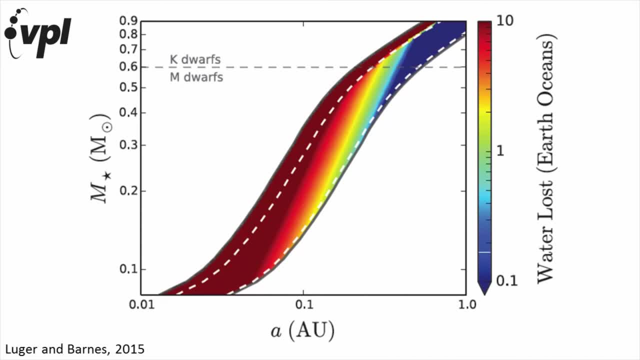 And as you move to the lower left, you get towards hotter and hotter colors. The white space is stuff that's just dead to begin with, right? So it's outside the habitable zone because that planet's either too close to the planet or it's just dead to begin with. So it's outside the habitable zone because that planet's either too close to the planet or it's just dead to begin with. 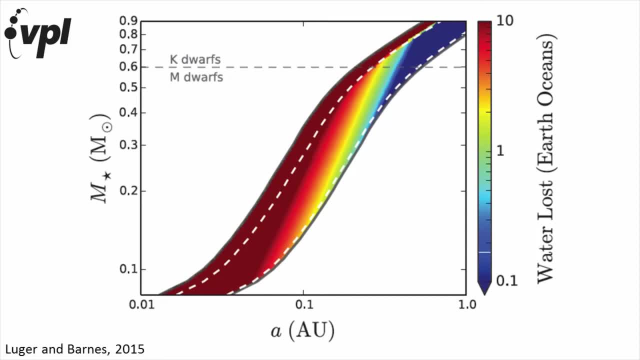 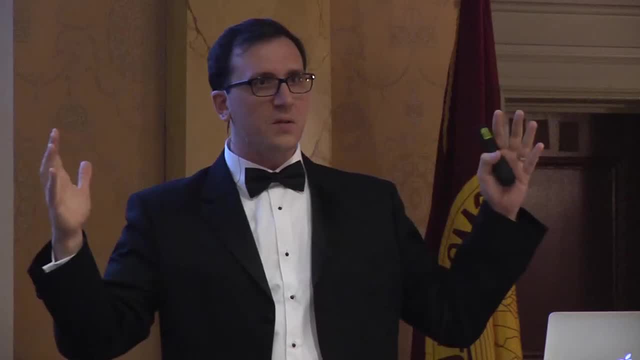 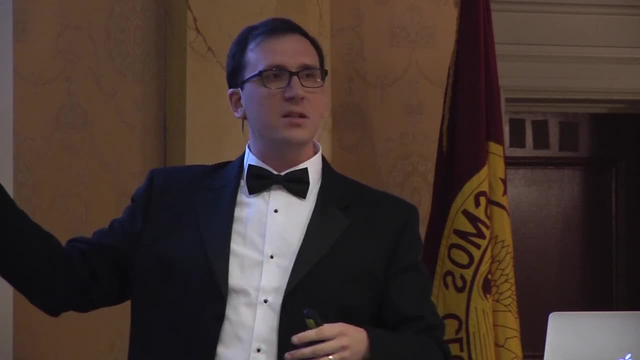 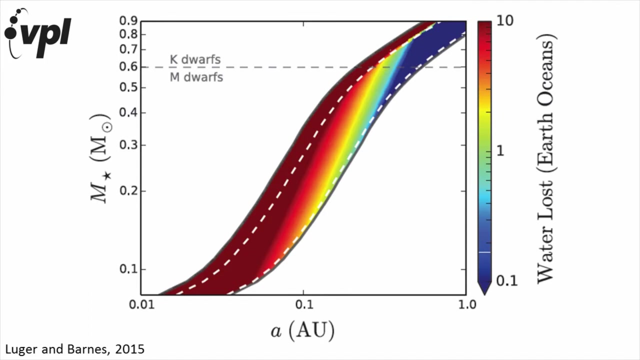 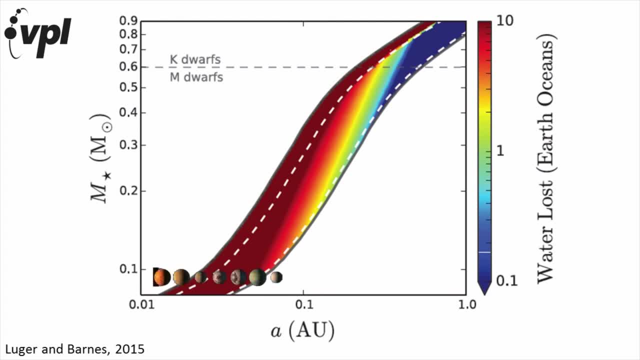 diagram. So there's the Trappist worlds that we're just talking about. The ones in the habitables are sitting right in that red area, and red means atmospheric loss should be quite effective. Now, I'm not saying we should not look at those worlds. In fact, the nerd in me wants to look at these worlds specifically to test this theory. because this is all. everything on this diagram now is a model and this is an artist's interpretation of data. okay, 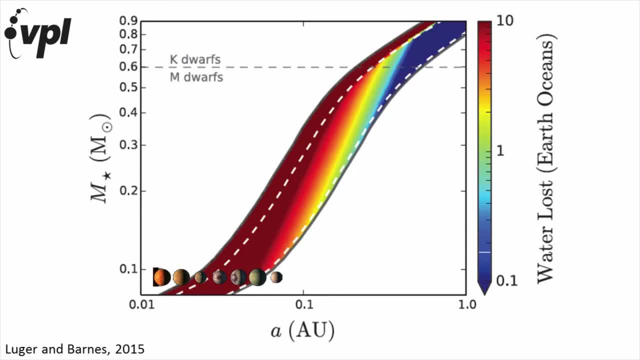 And so, if for no other reason, I want to test the theory that goes into that model by looking at these Trappist worlds, even if they don't have atmospheres. to me that's fascinating. And if they do have atmospheres and our models are wrong, then we've got a chance. that's. 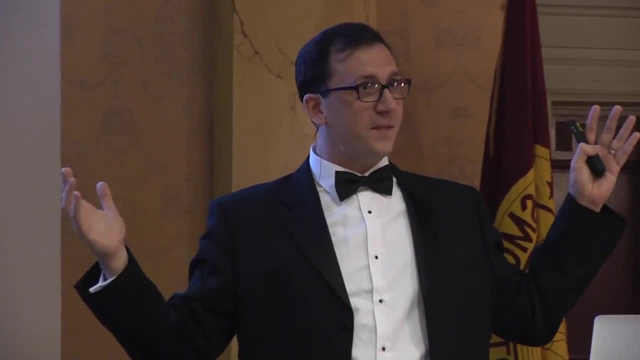 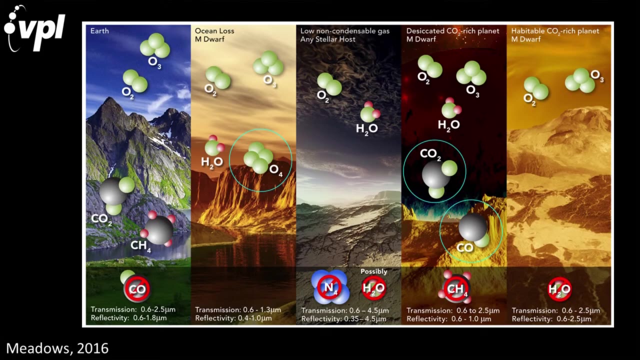 a lottery ticket right, We might be able to actually search for life in the next five years. if that's the case, Now there's another caveat, which is, even if the atmosphere is retained, these cooler type stars, because the energy distribution of photons from the host star is different. 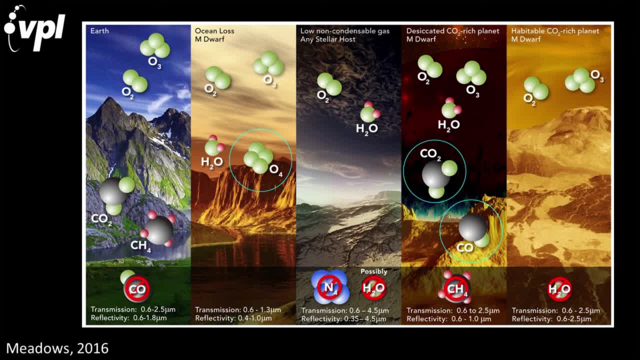 and weighted towards the higher energy regime. it also affects the chemistry inside the atmosphere, And it does it in a way that could lead to the buildup of oxygen and ozone in the atmosphere without any biological flux of oxygen into the atmosphere, And there's two reasons for that. 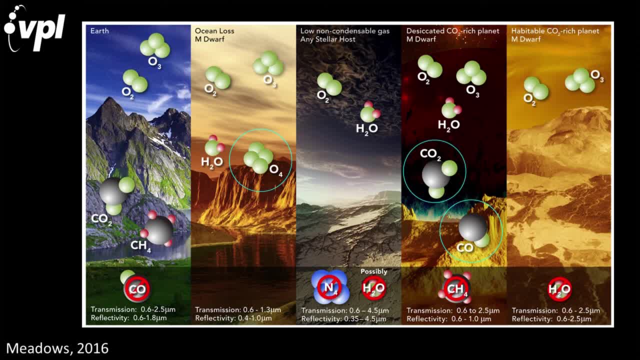 The first is that high energy radiation that I showed stripping away the Maven atmosphere. if it doesn't strip away all of the atmosphere from one of these worlds, it's going to strip away the lightest atoms in the atmosphere, And the lightest atom is hydrogen. 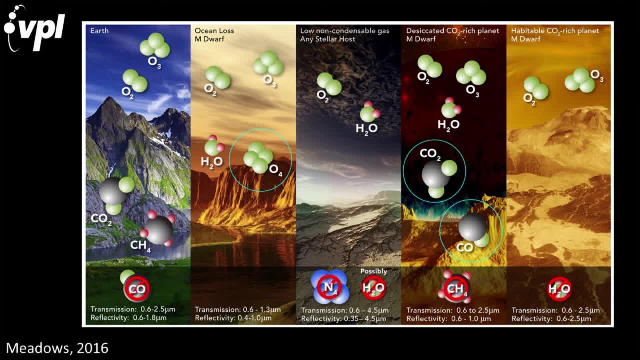 Now hydrogen and oxygen are kind of like the moral combatants in chemistry, at least in terms of atmospheric chemistry. If you look at the history of our atmosphere's chemistry over the entire history of Earth, it's a story of the redox state, of essentially the balance between oxygen atoms and hydrogen. 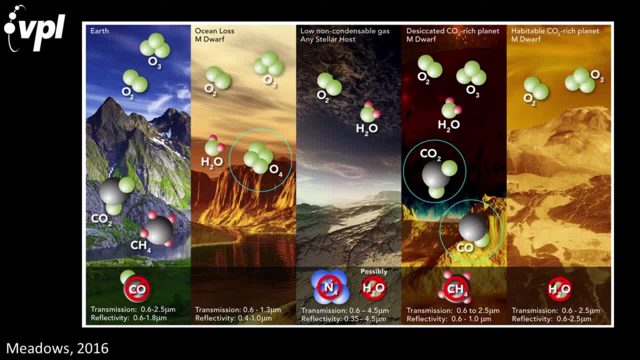 atoms. If you get rid of all the hydrogen atoms but not the entire atmosphere, you're going to end up with an oxygenated atmosphere. So if you get rid of all the hydrogen atoms but not the entire atmosphere, you're basically 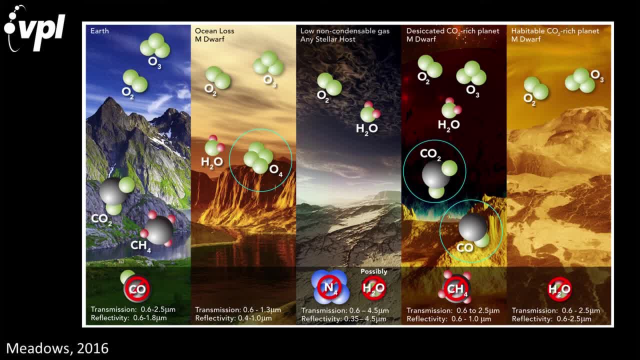 left with oxygen atoms to dictate the chemistry, You'll end up with an oxygenated atmosphere And I worry about that. so it's because, So if the atmosphere is not lost and you just lose part of it, you're preferentially going to lose the things that would lead to an accumulation of the thing that you think is a biosignature. 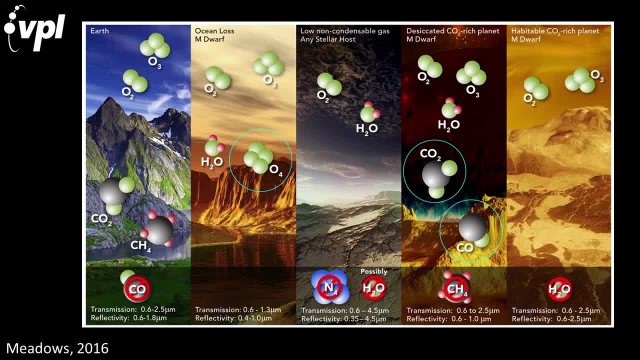 And the other reason is those photons are also really good at splitting up carbon dioxide molecules. If you split up CO2, you strip away an oxygen and you let that oxygen hang out free, not seeing any hydrogens in the way to combine with another oxygen to form O2 and O3.. 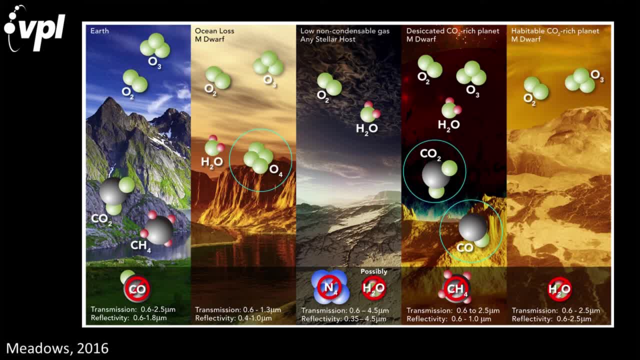 And the other reason is those photons are also really good at splitting up carbon dioxide molecules- an accumulation of the thing that you think is a biosignature. And the other reason is those photons are also really good at splitting up carbon dioxide molecules. If you split up CO2, you strip away an oxygen and you let that oxygen hang out free, not. 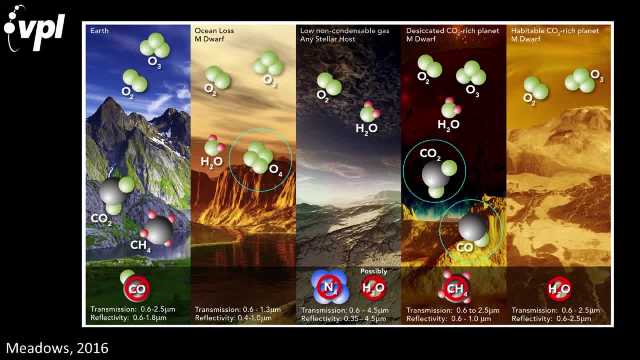 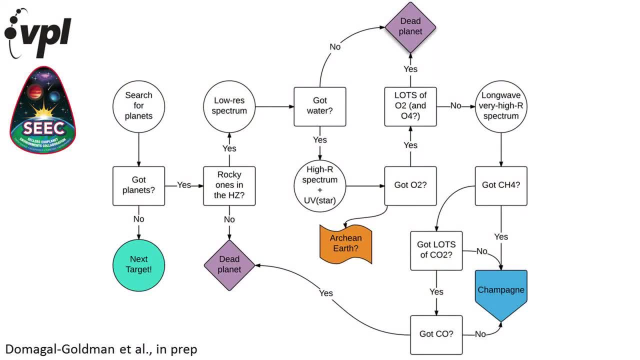 seeing any hydrogens in the way to combine with another oxygen to form O2 and O3. So I worry about this from the- let's call it the Allen Hills perspective. So we've taken this into account over the last. I mean, really this stuff goes way back. 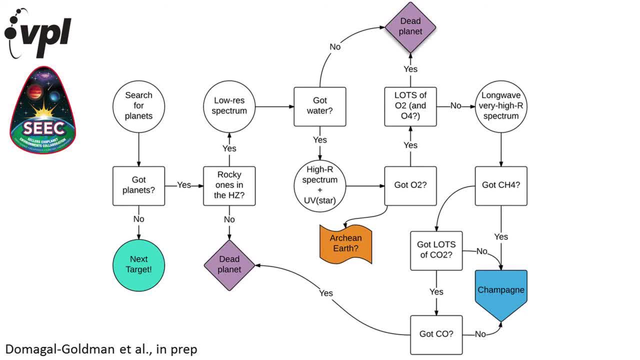 you know, decades. But what we've been doing lately is trying to come up with an observational strategy that accounts for not just the false positives I just talked about here, but all the false positives for life that we've thought of to date. And the end of the day it comes back to the same story. 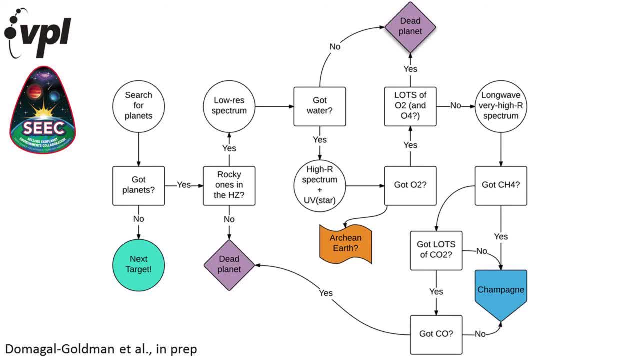 If you want something which has been called thermodynamic disequilibrium in the atmosphere, I actually think it's better described as kinetic disequilibrium. In some ways, thermodynamic disequilibrium is bad. I think of that as a free lunch. 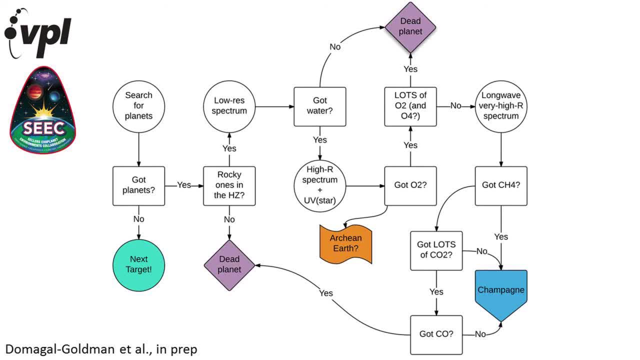 If you've got too much energy sitting out there. the analogy of one of my colleagues uses is: If you've got a dish of candy outside your office at a university and it's not eaten, it's probably summer and the students are gone right. Free lunch is something students don't pass up, and free lunch is not something that life passes up either. What you really want to look at is how is it that that gas is retained in the atmosphere? Does it require life? And would you predict life would generate that gas at those rates? 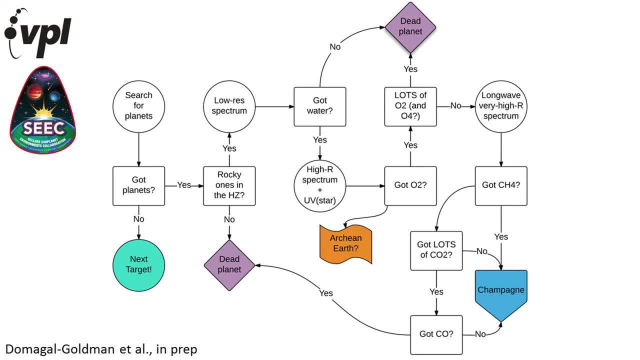 And this is our observational strategy. I won't go through the whole thing, but it starts off by saying: do you have planets there? If so, are they in the right place to have life? If so, is there water there? We do the water first, in part because it's easy to see. 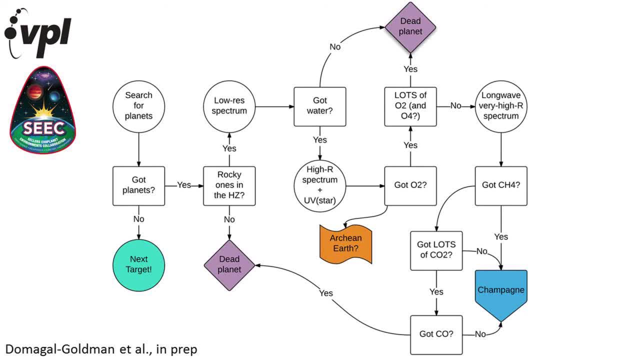 It's got big spectral features. If you've got water, you start to look for the oxygen. You start to rule out the false positives And it ends here: Do you have methane? If you have methane and oxygen, that's critical. 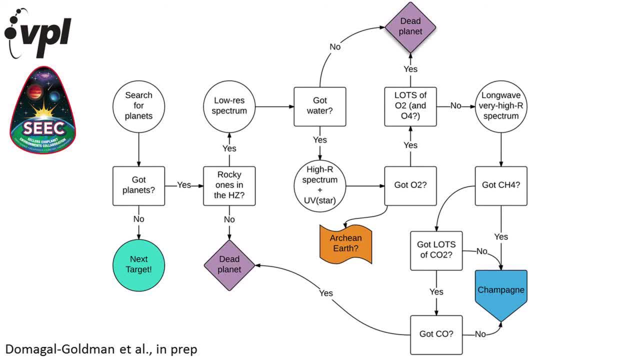 And it's not to me a thermodynamic disequilibrium, It's more, in my mind, a kinetic one. The analogy I use here is if I see pizza in a room full of those same college students. I know there's a pizza delivery restaurant nearby. 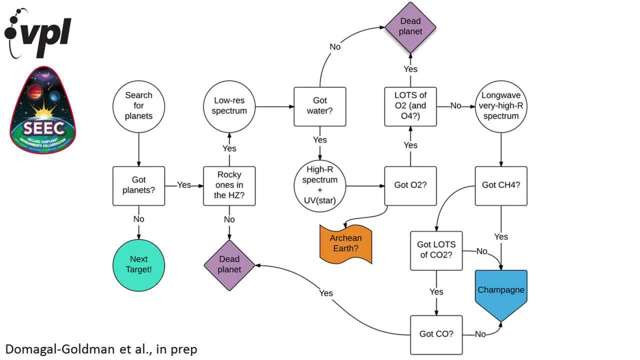 And the reason is college students eat pizza. So if that pizza's there and it's in significant quantities and there's a significant quantity of college students around, you know there has to be a rapid pizza delivery mechanism. At least, when I was in college I wasn't making that much pizza, at least not in large quantities. 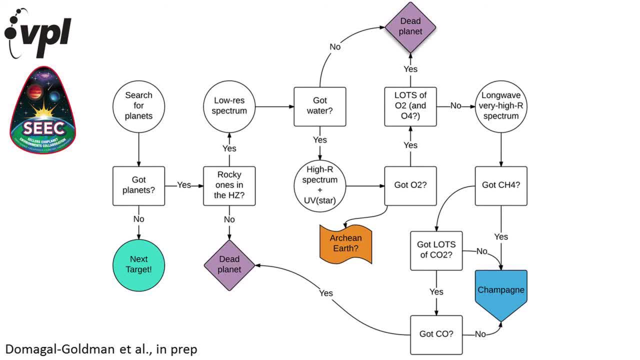 Actually I wasn't making pizza. I make pizza now, but I didn't make pizza when I was in college. I didn't have that skill set. So by the presence of the quantity of pizza and students in the same room you can ascertain. a pizza delivery mechanism which is a pizza restaurant. It's the same thing. But oxygen and methane destroy each other. You can only keep them in the atmosphere together if you're replenishing them at very rapid rates, And those rates are orders of magnitude larger than any non-biological process. And all the non-biological accumulation and ways to accumulate oxygen we know of actually work. on the other end, They work on slowing down the destruction of oxygen so that it's slow enough that these slow abiotic production rates can maintain it in the atmosphere. 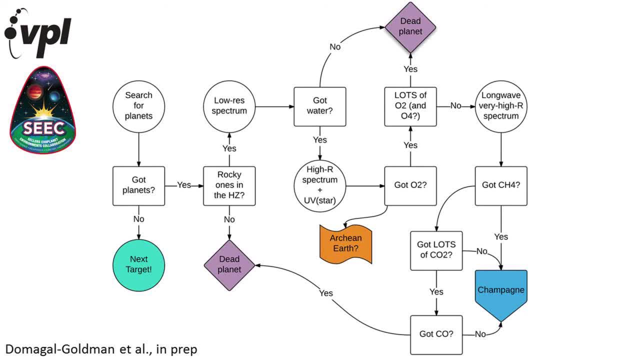 So to me the biosignature is about the fluxes, And to get the fluxes you can't just make the measurement of the one gas you're worried about. You have to measure the entire atmospheric chemistry as well as you can. 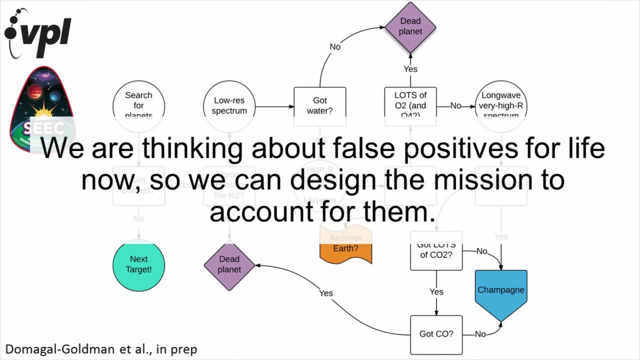 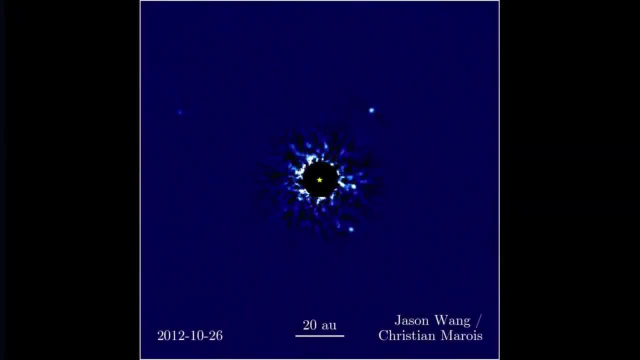 So we're thinking about these false positives And we're thinking about what you would need to do to actually make the measurements to rule out the false positives, And one of the things that's quite powerful is to- and the transit spectroscopy technique is absolutely tremendous and it's going to tell us a lot about the chemistry of worlds. 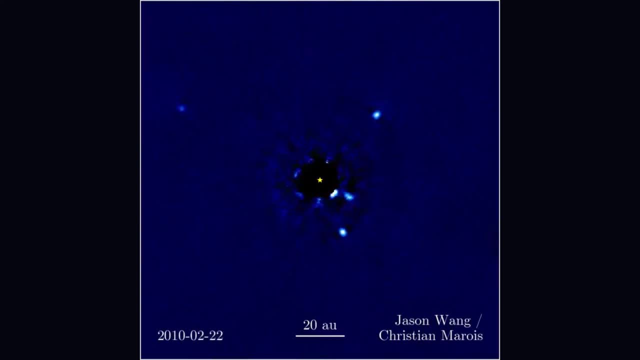 in the near term, But eventually you want to do something like this. This is a wonderful movie that's a stitched together, an interpolated set of images of uninhabitable worlds made from a ground based telescope by Wang and Marois Marois. 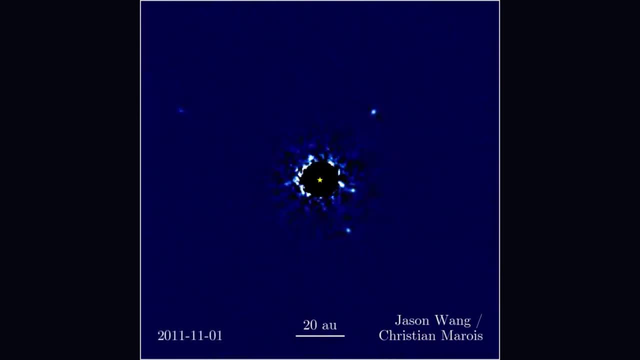 And we want to do a movie like this for potentially habitable planets around other stars, Because if we directly- this is, if we do this- we're getting planet that's coming from the star bouncing off the planet and coming back to our telescopes instead of seeing the 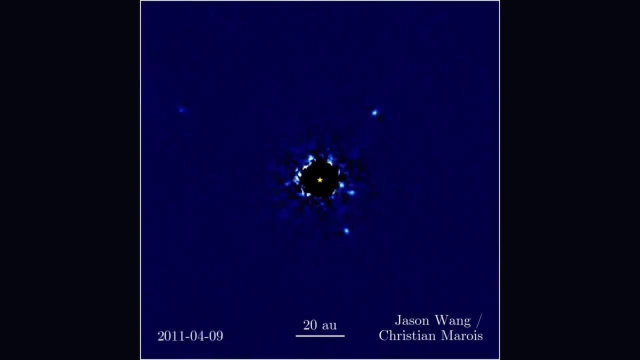 planet pass in front of the star, And what that means is we get to see deeper into the planetary atmosphere, because, instead of glancing through the top of the atmosphere, it's penetrating deep into the atmosphere before those photons, And that's how we return to our cameras. 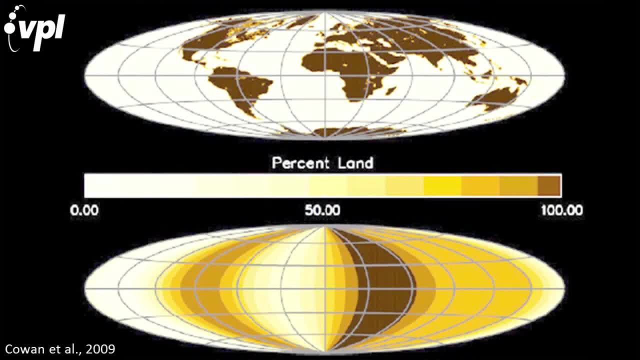 And what that'll let us do is it'll let us not just see deeper into the atmosphere, but also, hopefully, to the surface. If you have a big enough telescope and you look a long enough time with it, you can start to see the spectral features from the surface associated with oceans and continents. 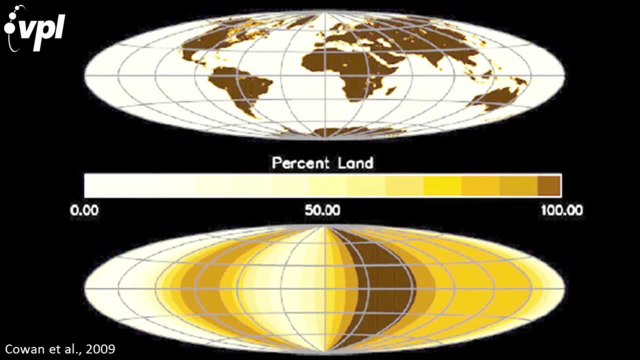 And if you stare at that planet, as the planet spins underneath, the telescope, the planet's going to be giving you different sides of it as it rotates. And this is an experiment by Nick Cowan, who's now up in Canada. He was at the University of Washington at the time where he took a planetary spacecraft. 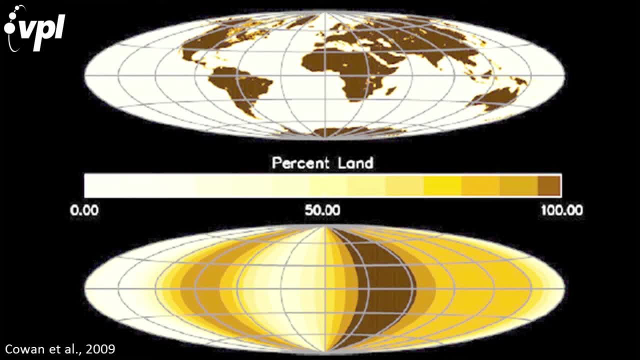 pointed it back at Earth from further out in the solar system, basically convolved the data back down to a single pixel and then looked at the pixel change over time And he was able to tease out from the one pixel of light and its colors where continents 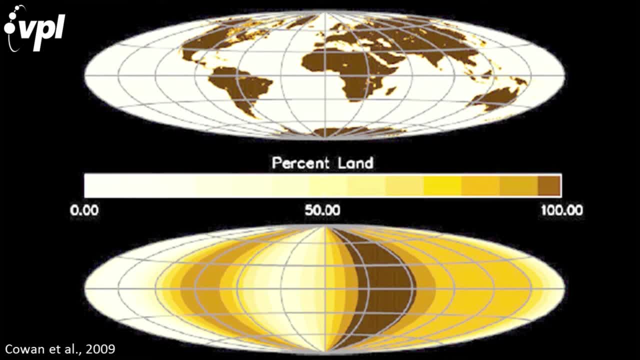 and oceans were on Earth because the Earth was spinning underneath that spacecraft and presenting different faces of the Earth over time. So he did it. the technique he used was a principal component analysis, and now we're looking at what we could do In terms of a principal component analysis for exoplanets. it's sort of a proof of concept. 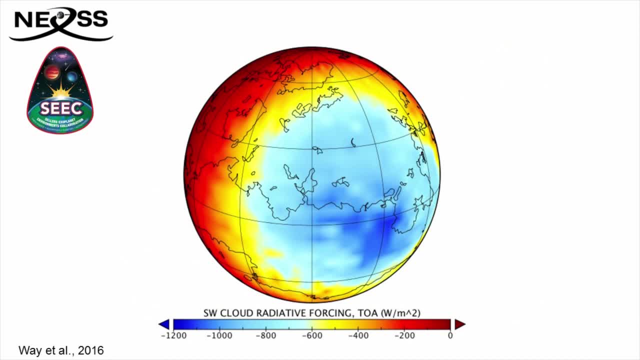 Now, to do this really well, it's going to take more than just a brilliant scientist or even a couple brilliant scientists. this is really going to take a whole community of people. I talked about what we've learned from the MAVEN mission, which is a planetary mission. 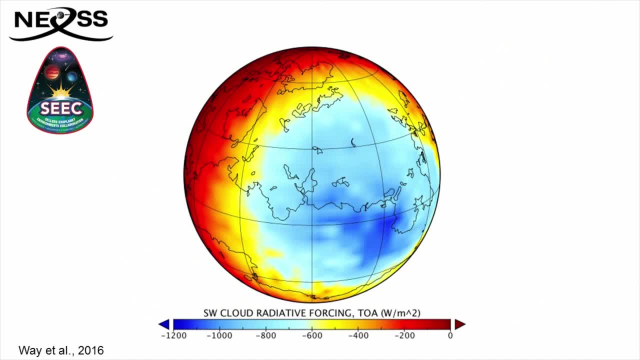 It's really a heliophysics process, that's the loss of this atmosphere through the top. We have to think about these things in a system science context, which is something that the Earth scientists are teaching us, because you have to think about that biosignature. 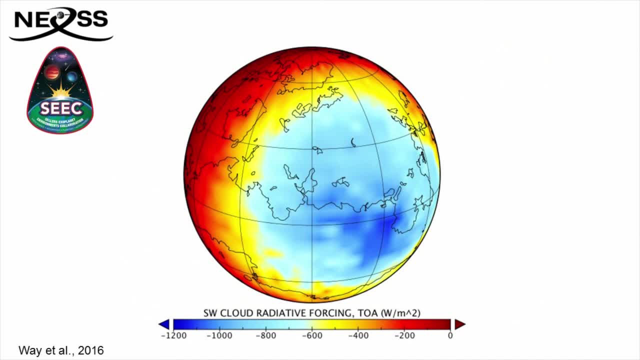 volcanic production in the context of oceans and continents, And this is where I have a lot of hope for our ability to do that. So this is a paper that just came out this year, where colleagues at NASA up at the Goddard Institute for Space Studies in New York City took an Earth climate change model. the same 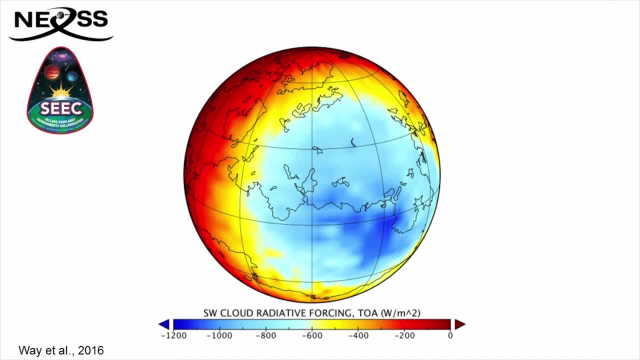 kinds of global climate models we use to predict anthropogenic climate change here on Earth, and they changed the inputs to that model to make it for to simulate Venus. And they did: This isn't modern Venus, This is an ancient Venus. They've also done modern Mars. 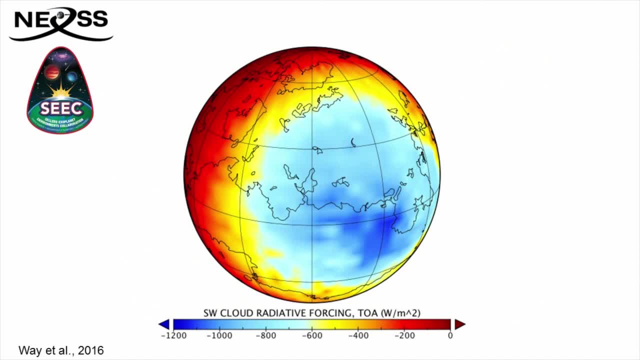 But that tells me two things. One, the models are good. They're not overly tuned to Earth. But two, we have models that work out of the box, that come with all that system complexity. we need to treat these biosignatures in their planetary context. 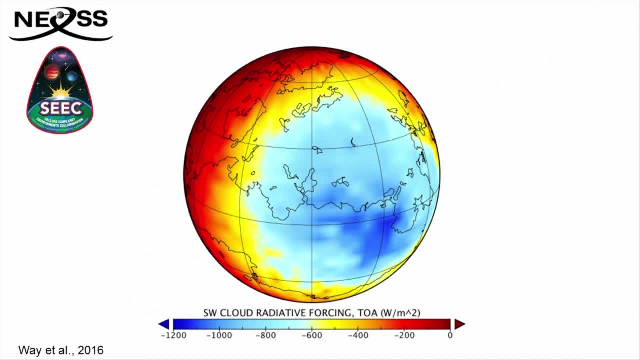 Unless you think this is just about NASA. we've actually got a whole community of scientists on board from universities and from across the country and we're expanding this throughout the world. This is the Nexus Exoplanet Systems Science Group. We're bringing this to NASA. 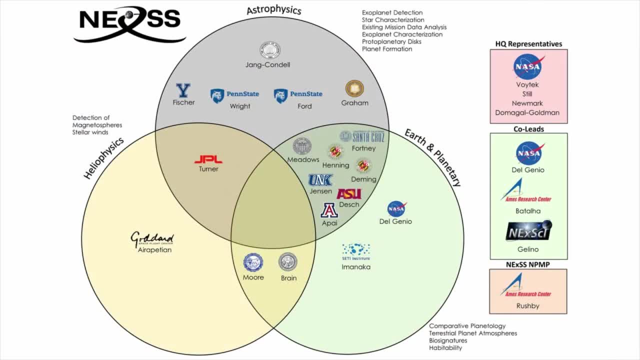 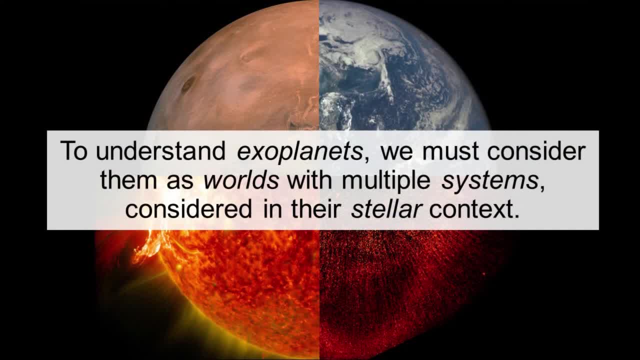 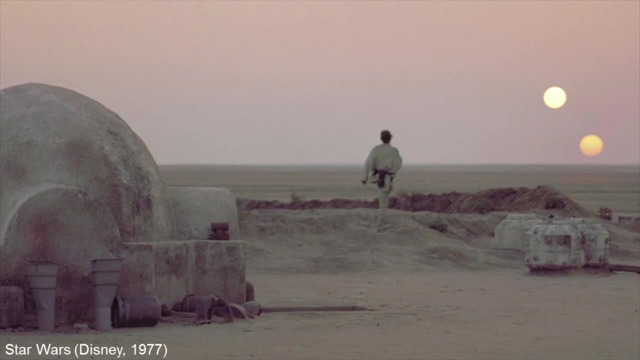 We're bringing all this science to bear on a single topic across all four divisions at NASA, Because to understand this, we really need to think about these things as systems with multiple components interacting. And I like to close here for two reasons. One is I'm a geologist and there's a history in geology seminars. to close with a picture: 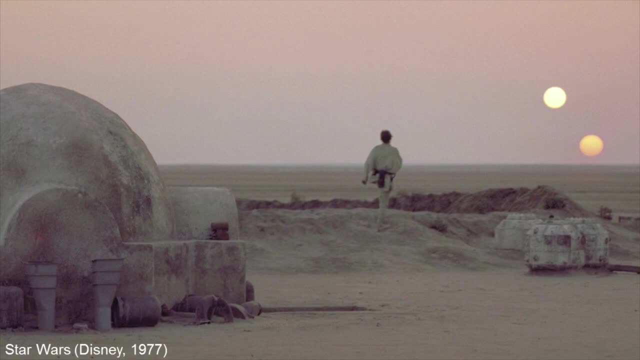 of a sunset And outside of… Dr Wakeford's talk, this is the best thing I can do for an exoplanet sunset. but I also like to close here, because when this movie was made, the astrophysicist said: well, that's nice and poetic, but that's impossible. and what? 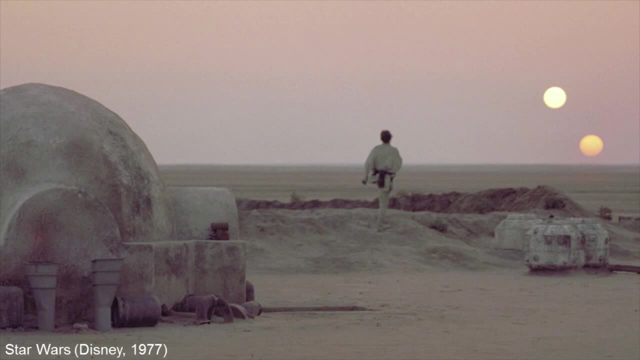 folks like Dr Fisher have found out is: you can have planets around double star systems like this. they exist, we've found them, and we found a lot of other surprises too. we're going to continue to find them in the near future. on the chemistry of these worlds. what I want to spend the next 20 years of my life. 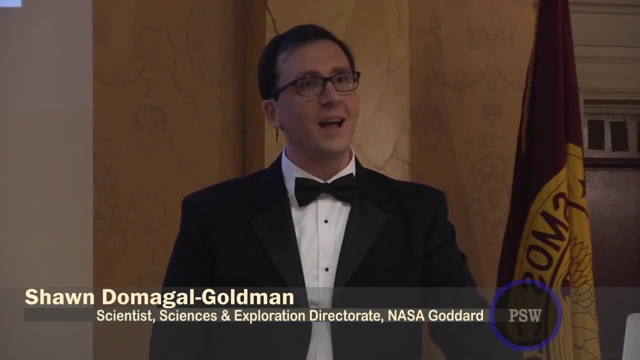 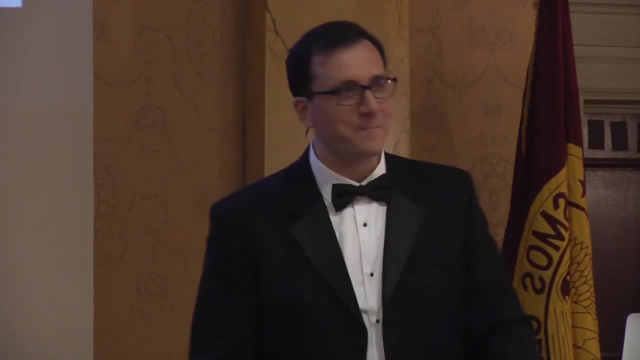 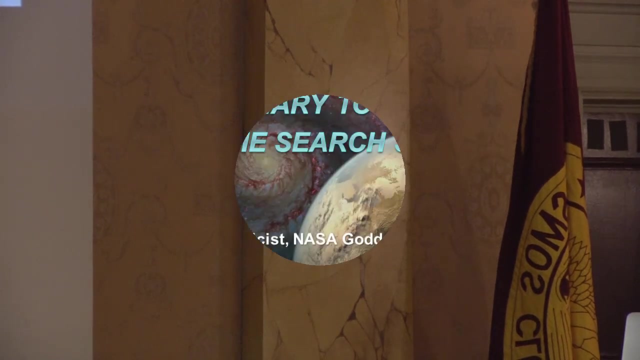 working on is working on the telescopes that'll get us biological signals from these planets so we can be surprised and rewrite the textbooks on how life interacts with its host planet. thank you, okay, but also the thing that Sean did, which I hope you got was, I think he made 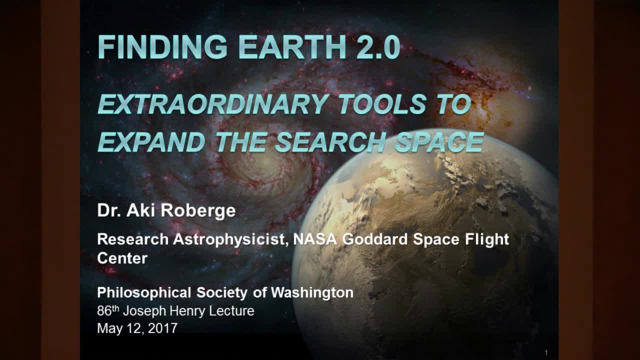 a very compelling case for investigating planets in a range of stellar environments, including the solar system, and the solar system and the solar system including ones that are more like the Sun Earth system that we know so well. so now I'm going to talk about what will be needed to actually achieve those goals. 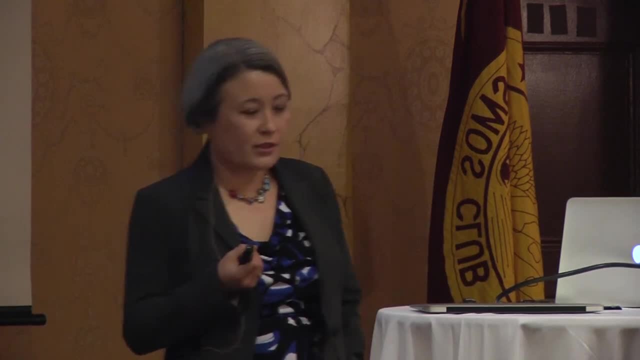 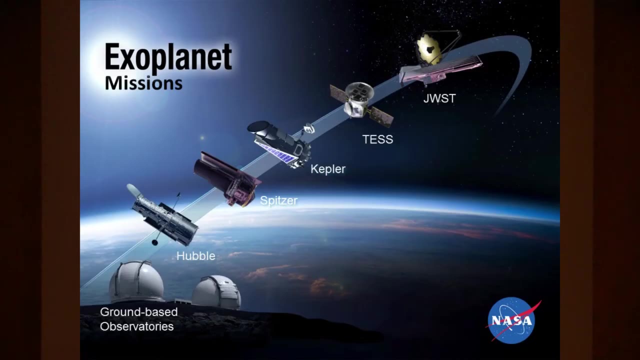 so we are advancing different observational techniques and developing new technologies to get there. this graphic shows the arc of the past and near future facilities for use for exoplanet studies and I think every single one of them has been mentioned in the previous talks. and just a recap, the 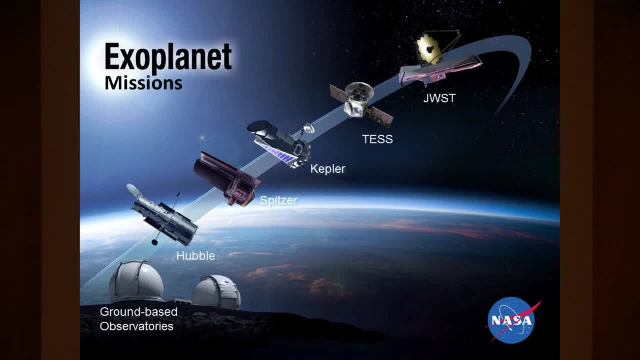 story started with the discovery of exoplanets using ground-based observatories, and Deborah was part of that in the early days still is. Those ground-based observatories are still critically important even today, producing more and more discoveries. So then, Hubble made the first discovery of 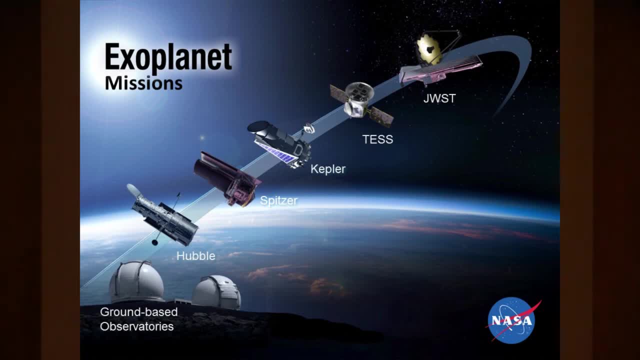 an exoplanet atmosphere. then Spitzer and Kepler. well, Spitzer started characterizing the atmospheres further and then Kepler just led to like an enormous explosion and a huge numbers of transiting exoplanets discovered and really showed the huge range and diversity of their masses and their 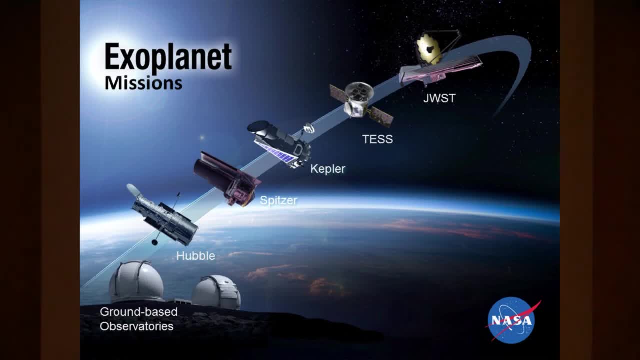 orbits. Okay, so then, as Hannah said, moving into the near future, the Transiting Exoplanet Survey Satellite will discover more small transiting planets, but this time they'll be orbiting stars that are closer to us, making them much easier for follow-up observations, which will be done with the 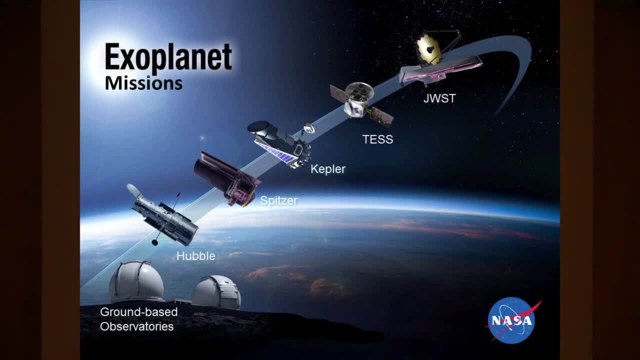 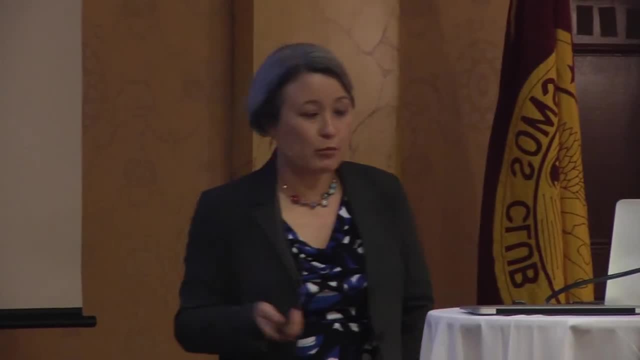 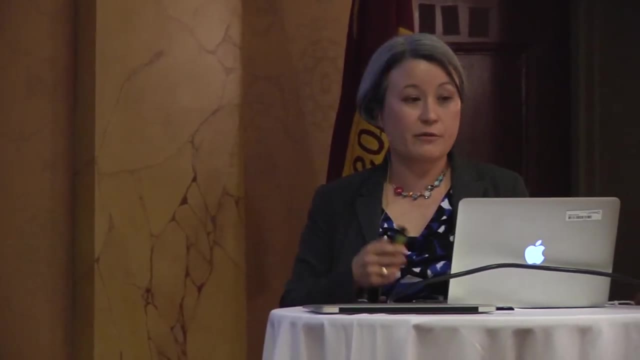 James Webb Space Telescope, which should really knock it out of the park for giant spectroscopy, actually doing spectroscopy to characterize the atmospheres of giant planets and for some small planets around small stars. Okay, however, so we've done all that. that's. that's what we've done, that's. 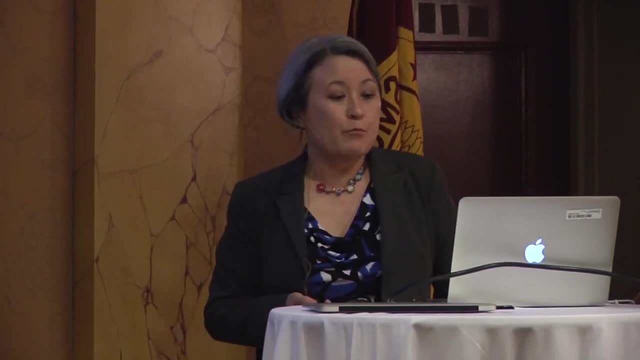 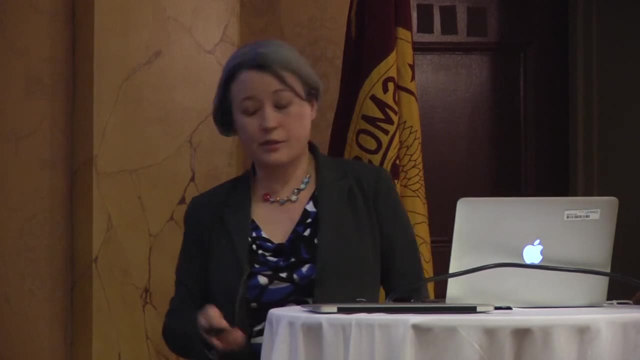 what's coming in the near in the next five years ish. but there's still an exoplanet parameter, space that we have not, cannot yet reach for atmosphere studies, And I'm gonna explain it. talk about that a bit next. Okay, so again, just recapping. 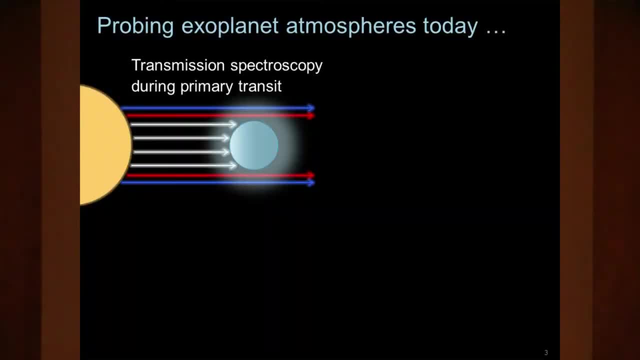 again what Hannah said and what Sean said: searching for life on exoplanets is really a search for atmospheric molecules, atmospheric biosignatures. So we need to probe the atmospheres. Today we're doing that for giant planets with transmission spectroscopy, as in this cartoon light from the star, some of it. 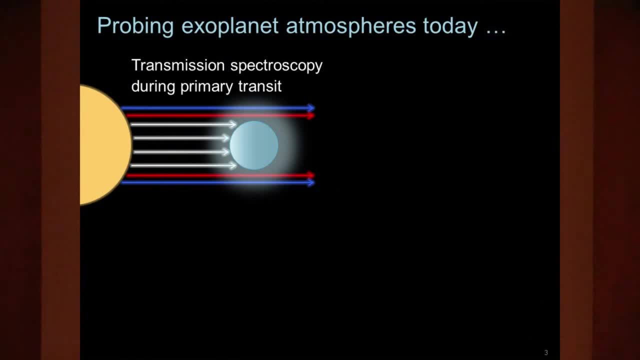 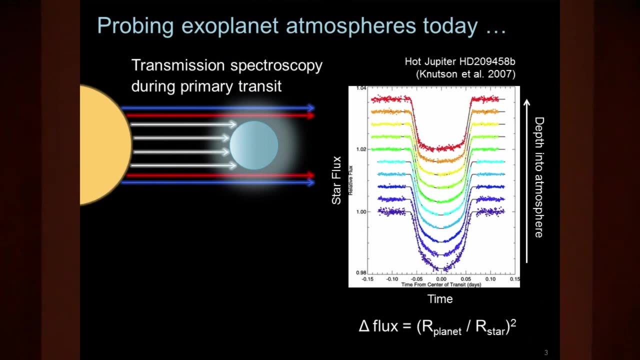 is blocked by the solid surface, and some of it is blocked by the solid surface. Some of it passes through the atmosphere. If you obtain light curves at different wavelengths, as Hannah also said, you can recover the spectrum of the planet. So the point here is that different wavelengths of light penetrate more or 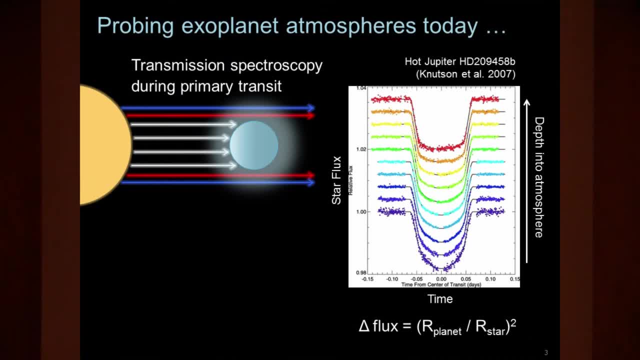 less deeply into the atmosphere. So for example, here the blue light ends up getting absorbed higher in the atmosphere and it the planet looks bigger, so you get a deeper transit depth. Then the red light penetrates more deeply Into the atmosphere. the planet looks smaller and you get a shallower. 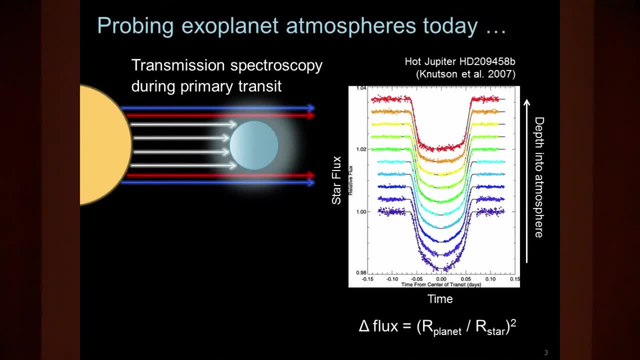 transit depth And if you do this for a bunch of wavelengths, you probe the depth into the atmosphere. So, and doing this, you can recover the wavelength dependent atmospheric absorption spectrum of the planet. However, as you can see this change in flux here, the relative change in flux is proportional. 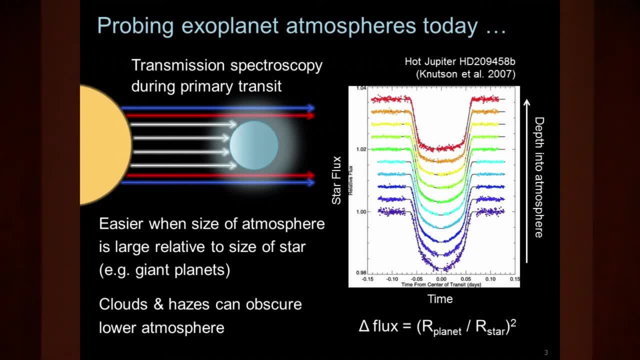 to the area of the planet over the area of the star, And so you can imagine, this is much easier when the size of the atmosphere is large Relative to the size of the star, like for a gas giant planet. The other issue with this technique is, as Hannah also mentioned, that clouds and hazes, as 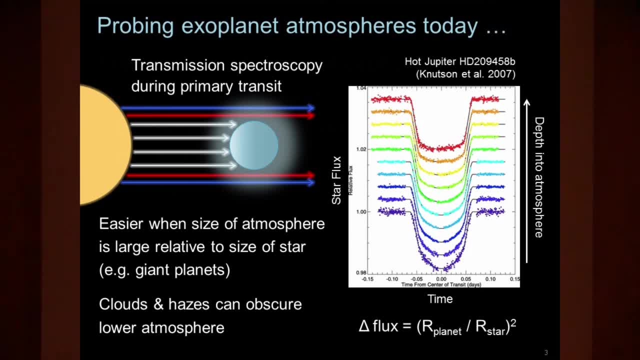 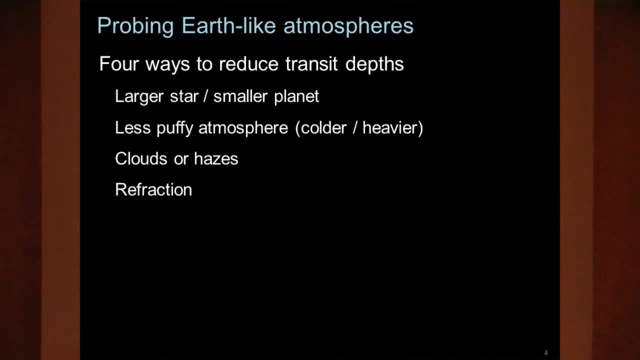 interesting as they are for their own sake, can obscure the lower atmosphere of the planet, and there's actually an interesting illustration. Actually, no, sorry, first I'm going to do this. Ok, so if we want to push this technique, So why can't we use this technique to do? 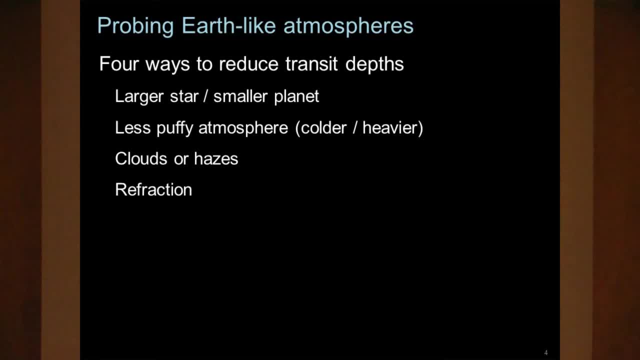 true, Earth's around Sun like stars, and here's why there are four ways to reduce the size of that transit signal. you're actually trying to measure that dip in light. you can have a larger star slash smaller planet. you can have a less puffy atmosphere, one that was colder or heavier- clouds and hazes, as I mentioned. 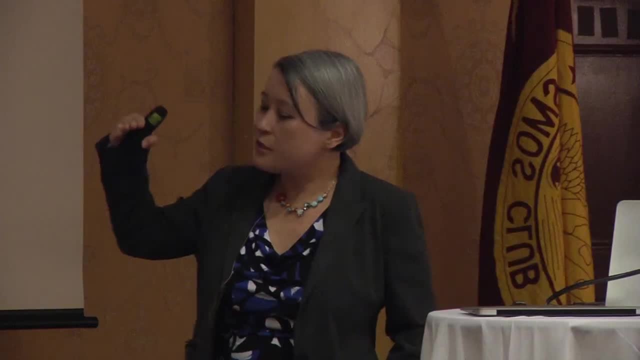 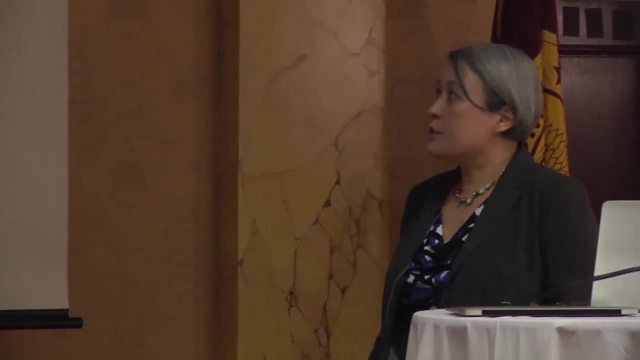 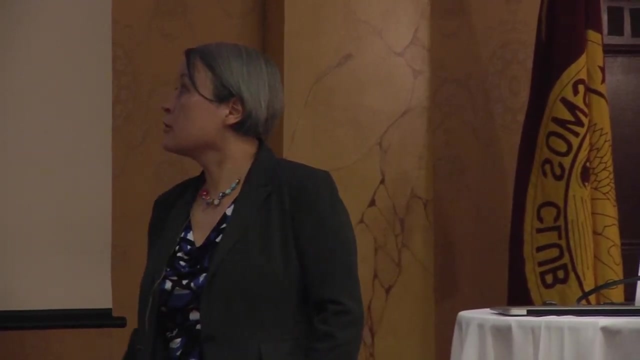 and then also refraction, just as the light just skims through the surface of the atmosphere and bounces off like a like bouncing off pond. all of these ways to reduce the transit signal, they all apply for Earth, like atmospheres around you know. for for Earth, Earth, like atmospheres on Earth sized planets. 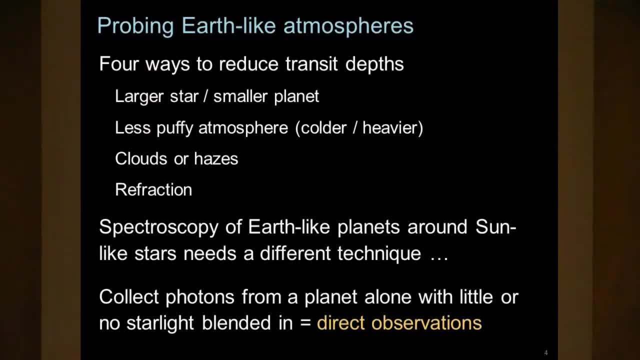 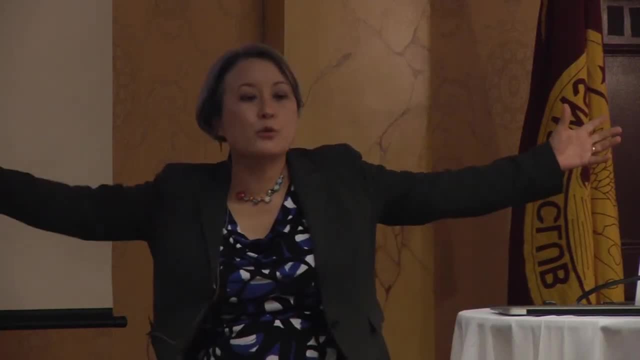 around Sun like stars. so, in some, the spectroscopy of Earth like planets, the ones that we, the ones that are more like us. we really need a different technique. in particular, what we need to do is we need to collect photons from the planet alone this time, not the, not a huge bucket of star photons with a tiny 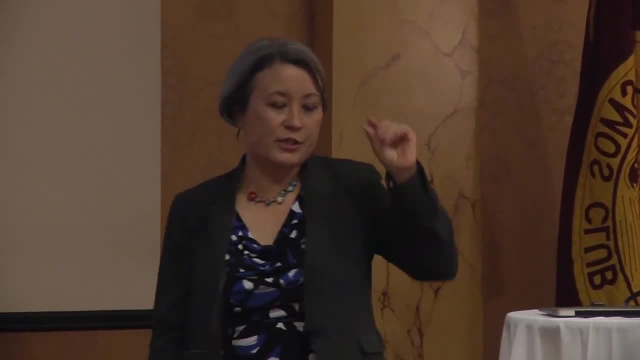 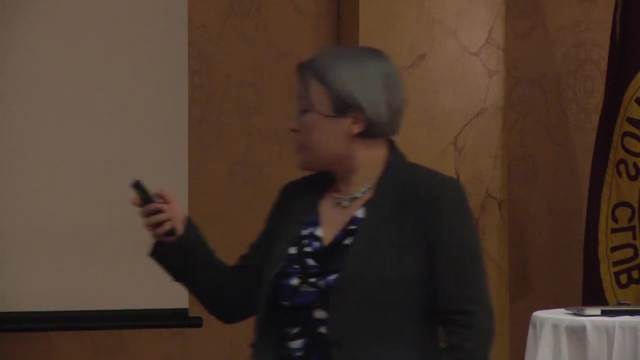 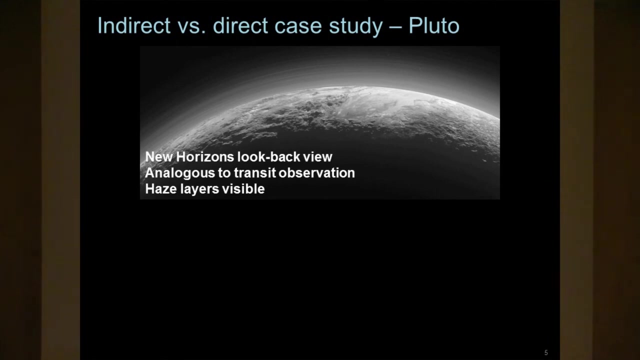 little signal of planet buried in it. we want to just suppress this. we want to suppress the stars and actually just observe the planet itself. so actually there's a kind of an interesting illustration of this that we just got from the New Horizons mission to Pluto. that shows kind of what I'm talking. 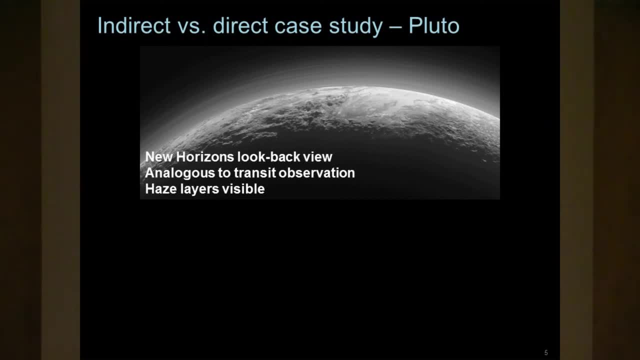 about here, I realized. so this is view of Pluto's limb. New Horizons was looking, had passed, Pluto was looking back towards the Sun, much like transit observation, and it was actually super interesting because they saw for the first time, unexpectedly, this, this very extended haze layers, many of them reaching up in the atmosphere, which was 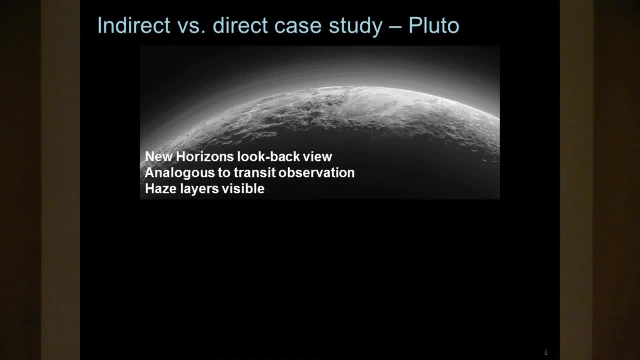 actually very interesting, but for our purposes haze is bad and an observation like this is extremely sensitive to haze and cloud. of course, Pluto's atmosphere is extremely tenuous, so you can still see the surface of the planet, but still this particular observation was sort of, in a way, dominated by the haze layers. On the other hand- this is New- 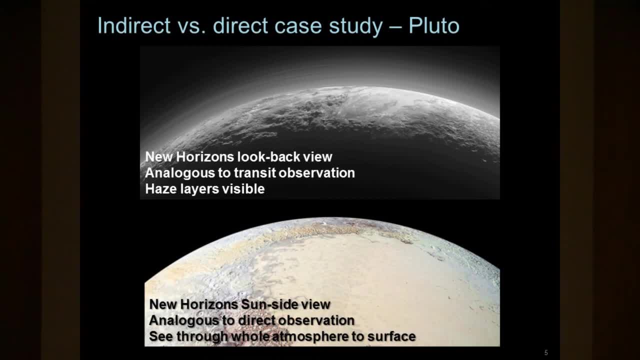 Horizons when it was on its way to Pluto, approaching Pluto. This is the sun's side view and this is analogous to a direct observation where the sunlight hit the planet and bounced, gone all the way down through the whole atmosphere, bounced off the surface and come all the way back. 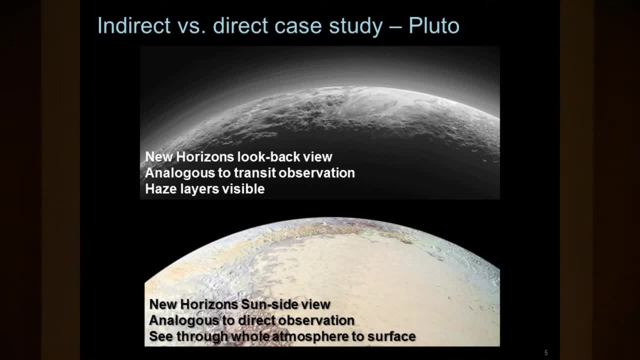 out again, And this is more like what we would do. this is more like what we would want to do for exoplanets, what we'll need to do Because, as I think Sean mentioned also as well, we actually do want to be able to probe all the way through the atmosphere, all the way down to the lower. 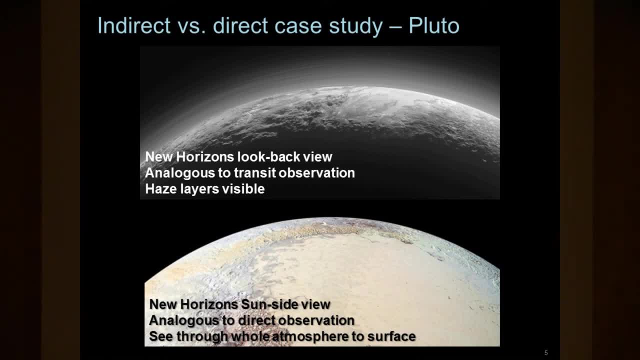 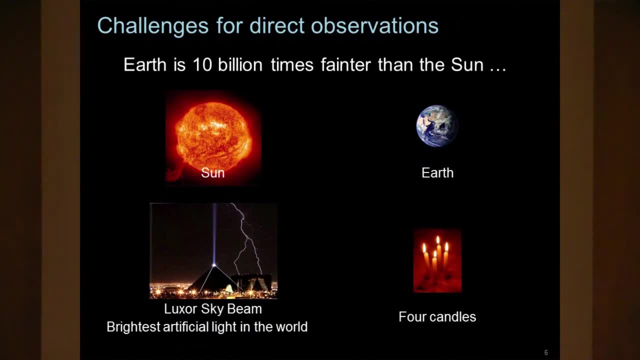 atmosphere and actually try to get a hint of what the surface features might be. Okay, so why aren't we doing this? Why aren't we taking pictures of exoplanets around sun-like stars right now? Okay, because it's really bloody hard, and let's just try to. 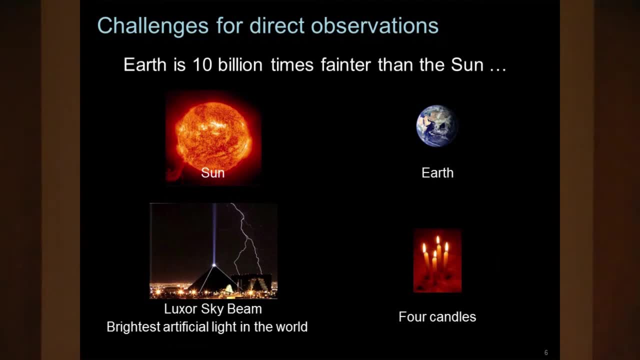 wrap our heads around exactly how bar-hard it is to take a direct picture of an Earth around a sun. Okay, so this is Earth is 10 billion times fainter than the sun, So I tried to come up with an actually mathematically accurate analogy for that And actually the traditional firefly. 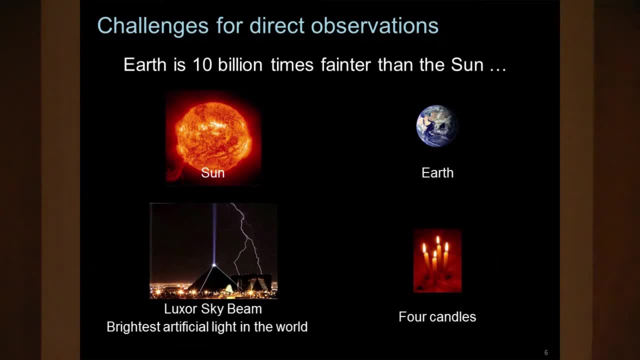 next to the searchlight. not faint enough. Firefly is too bright, So the Luxor sky beam is the largest, is the brightest artificial light in the world coming out of this hotel in Las Vegas? If that's the sun, then the Earth is four lumens. 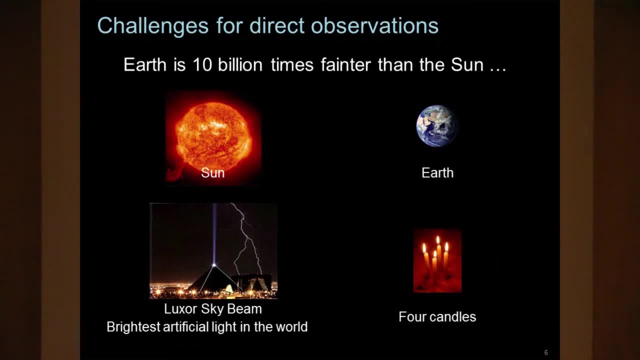 four standard dinner table candles. But astronomers actually observe things fainter than that. We've done that all the time. we do that all the time. we've done that before. That's not the really hard problem. The really hard problem is that those four candles are right next to the bright source. 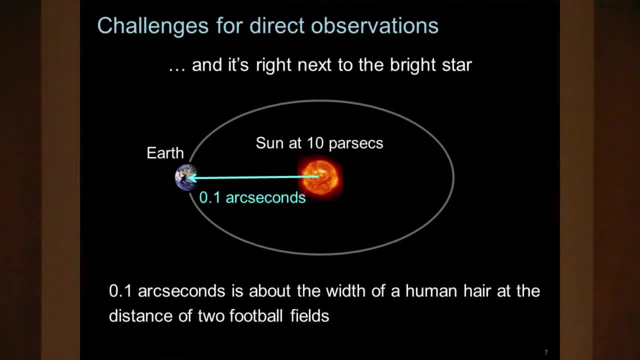 So for the Earth-Sun system at a distance of 10 parsecs, which is not very far away, the maximum angular separation, apparent separation between these sources is 0.1 arcseconds, And that is about the width of a human hair at the distance of two football fields. 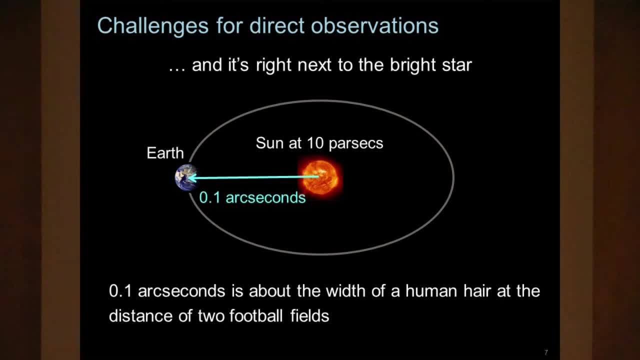 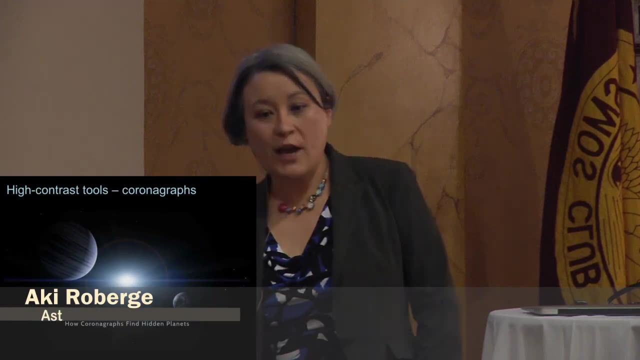 Okay, so now imagine the difficulty of trying to get the light just from those four dinner table candles when they were sitting right on top of the Luxor sky pyramid thing. Okay, so how can we do this? We need to dramatically suppress the light from the star so that we can see. 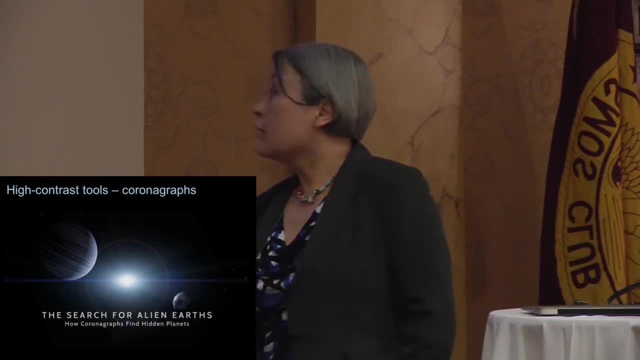 the pale blue dots next to them. And there are at least two different ways, technological ways, that people have thought of doing this. Okay so, and here is the first one I'm going to go over. So this is a movie that shows how a high-contrast instrument called a coronagraph works. Now 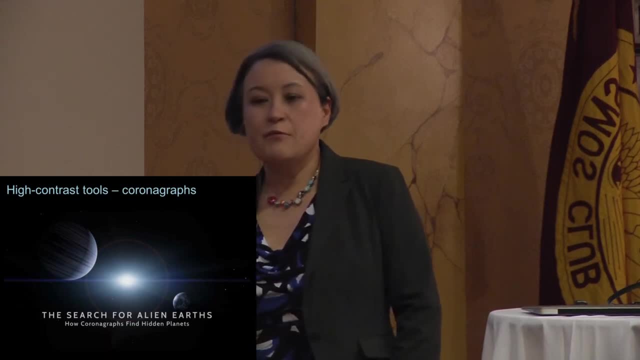 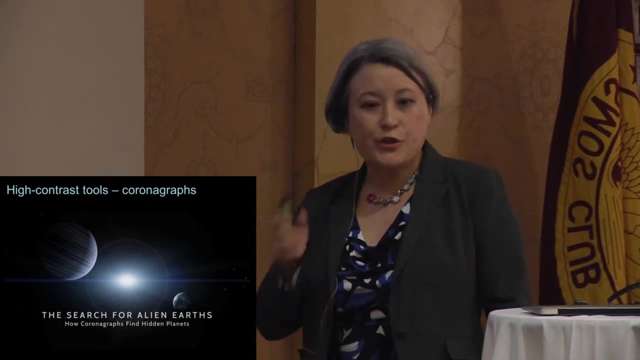 these aren't new. We've had coronagraphs for many decades. They were originally in the early 80s, invented to study the sun's corona, And they are used now already to take direct pictures, direct observations of exoplanets, Those four super Jupiters that Sean showed orbiting their 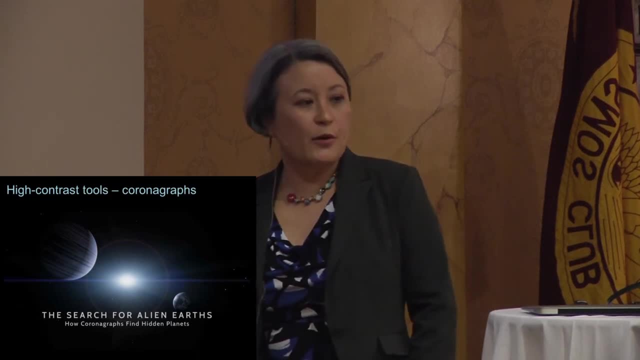 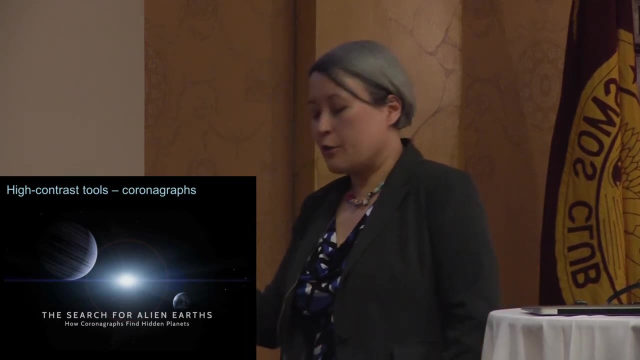 star. those were done with a coronagraphic instrument on a ground-based telescope. But we need to push this technology a good deal before we can actually do Earths around suns. So let's see, Let's watch this movie, that very nice one that JPL made. 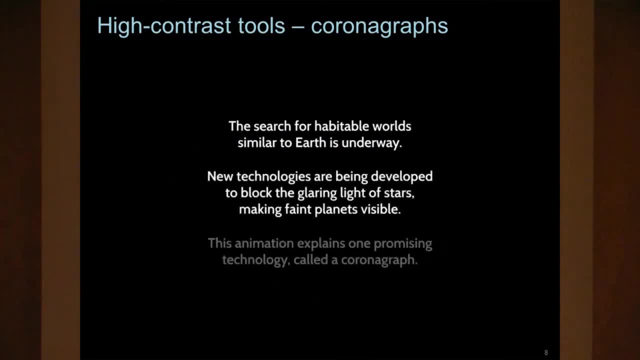 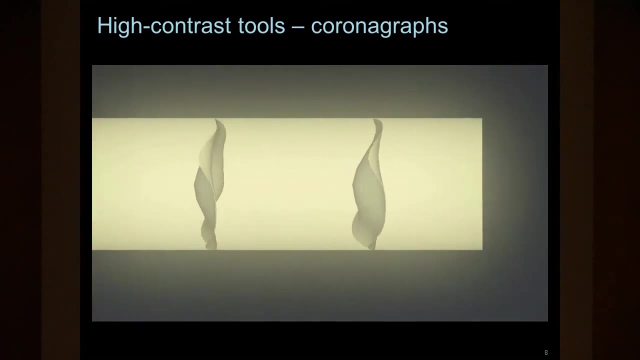 With a bit of an intro that says everything I already just said. Okay, now we go. Okay, so there's a telescope, There's light from the star coming in And the wavefront is coming in and it hits a number of optics, And if you don't do anything, that's what you see. 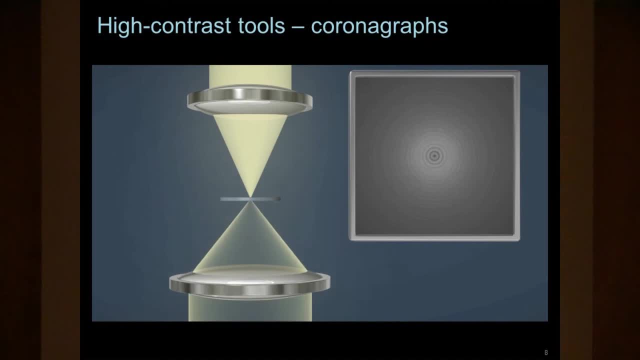 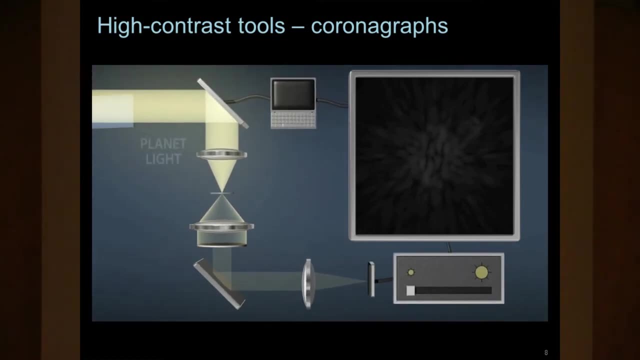 an airy diffraction pattern. If you put in an occulting spot, basically a little shaped mask, you suppress, Okay, and then a LEO stop. Okay, it's better. And now you see: okay, nothing, All right, let's change the contract. First of all, 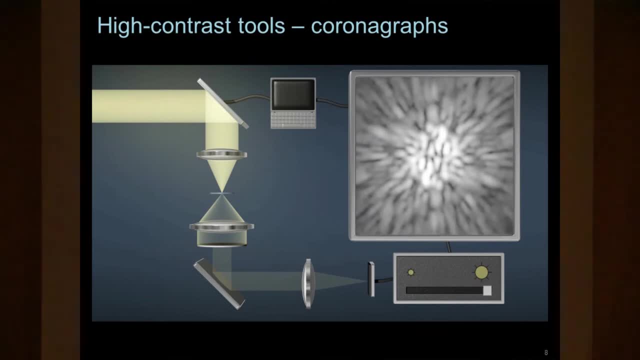 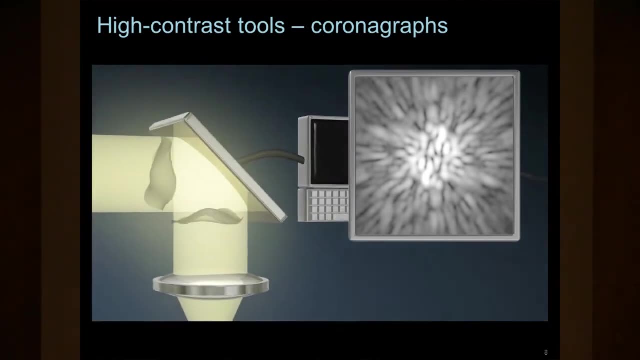 imagine that there was a planet actually in there and it's coming at a slightly different angle And now we change the contrast and we still see nothing. It's still just a bunch of residual speckles of starlight. So what really needs to happen is if you notice here that the shape 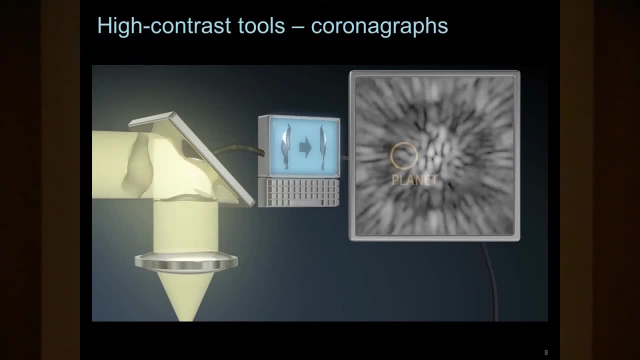 of the wavefront coming in from the telescope is distorted. It's not flat like it's supposed to be. So this is the new innovation here would be adding what's called a deformable mirror that actually changes its shape to correct for the distortions that were. 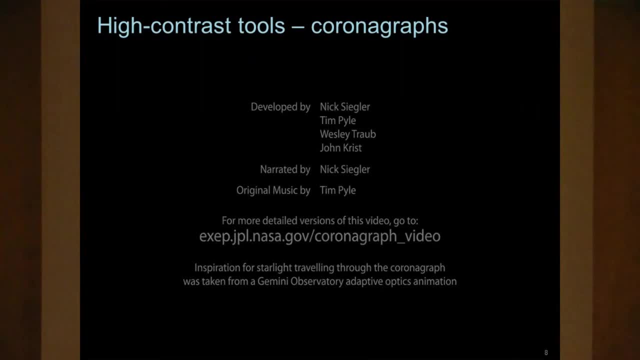 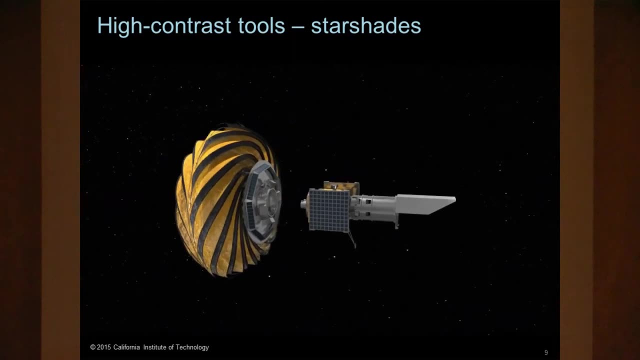 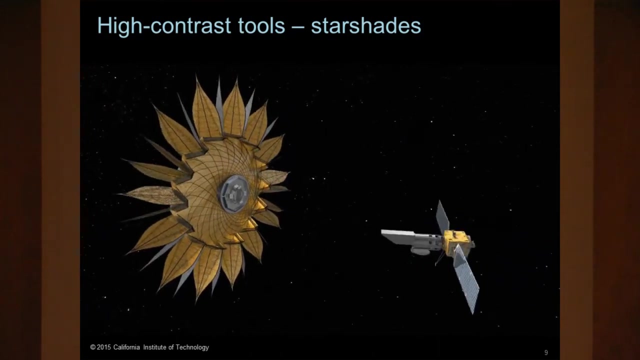 introduced by the primary telescope, and then flatten the wavefront so that you can actually get good contrast and start to pick out the planets from the residual starlight. Okay, so that's one notion. Okay, here's another one. This one is intuitive and 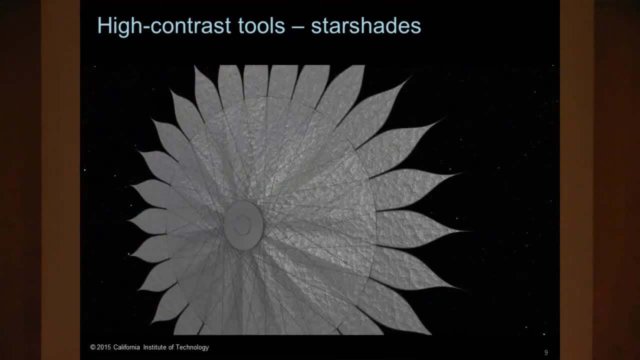 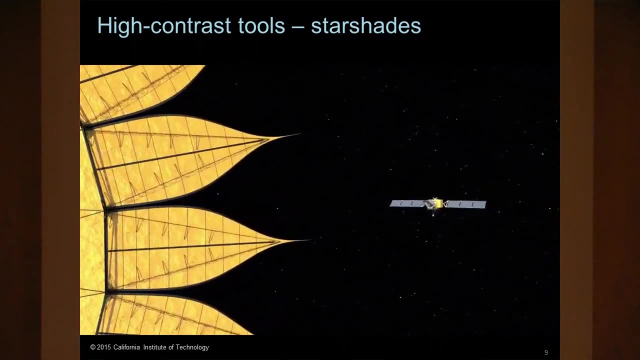 seems a lot easier. It's called a starshade, Unlike the chronographs. these have never been used before, and this movie will actually kind of probably show you why. But in a simple sense it's blocking the light from the star again, but this time the thing you're using to block the 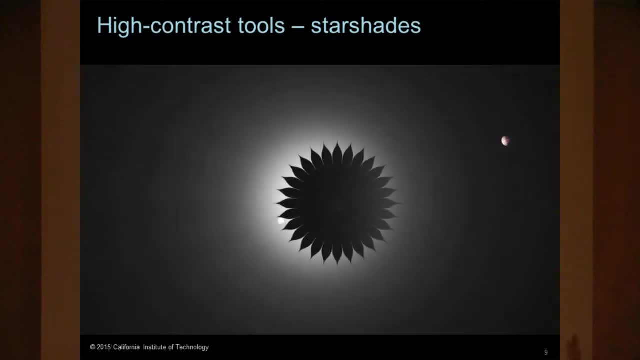 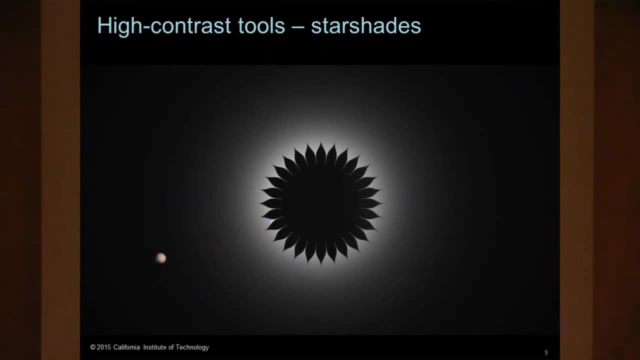 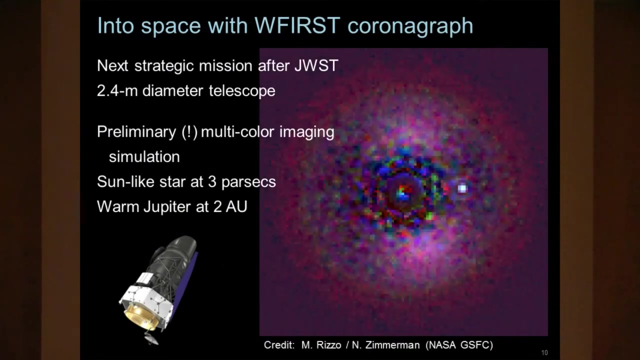 light outside the telescope, Way, way outside the telescope. All right, so let's watch. Okay, so the starshade unfurls and deploys for this particular configuration. This is a fairly small telescope, maybe one meter, and this thing is about 40-ish meters in diameter. So starshades are many in general, several tens of 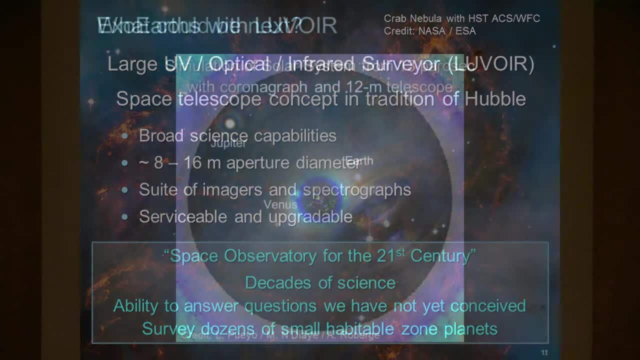 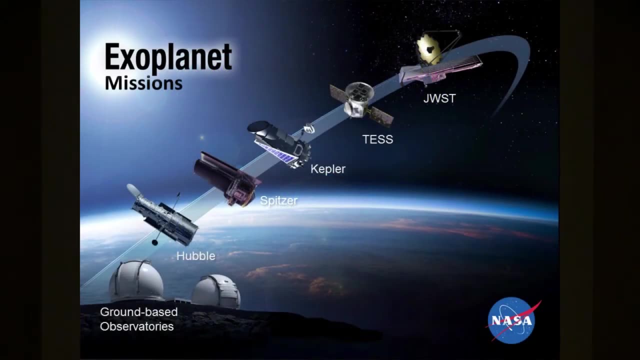 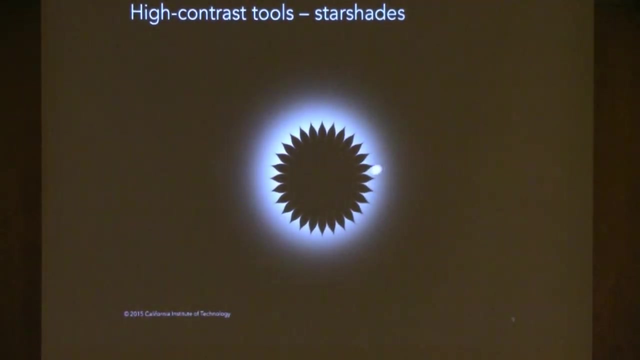 meters in diameter. Then it unfurls, it flies away. It flies away from the telescope in order to make it so that you could see the habitable zones of you know planets and the habitable zones of nearby stars. The planet starshade separation has to be something on the order of tens of thousands. 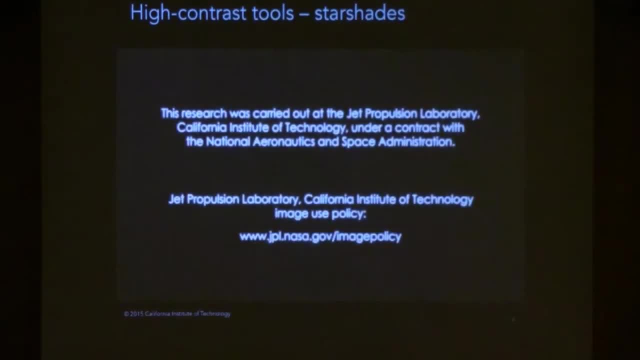 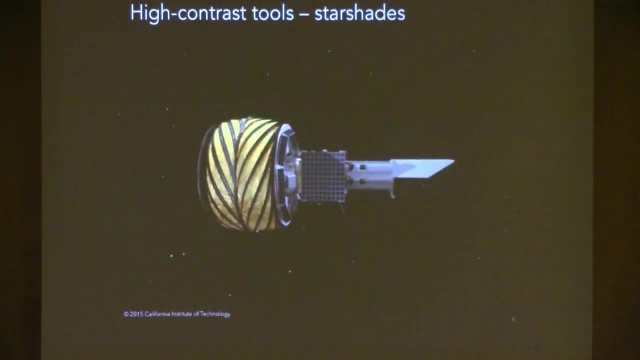 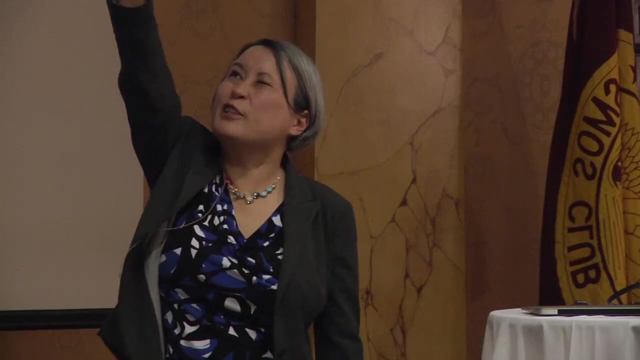 of kilometers, significant fractions of the Earth-Moon separation. Okay so, but still, though it looks very intuitive, because it's actually much more like what we do every day, when we are trying to make a high-contrast observation like, oh, like- an airplane flying by the sun. Block the sun with. 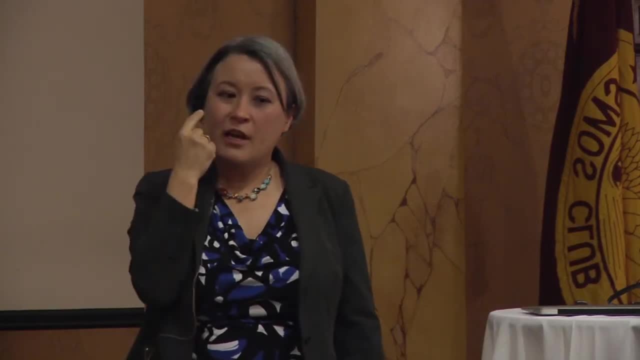 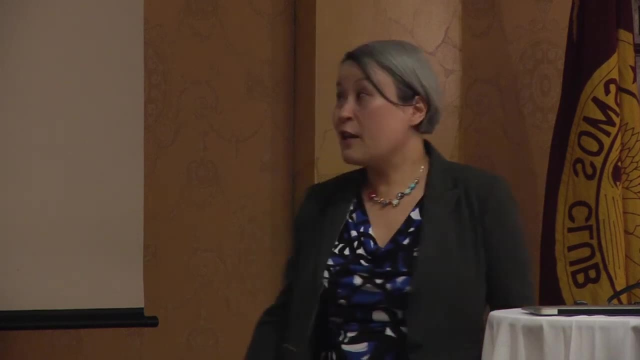 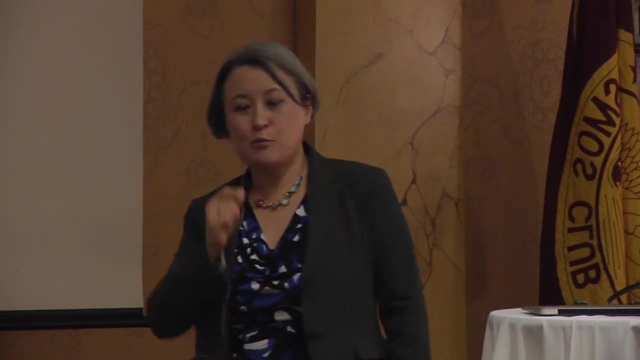 your hand In the starshade, your hand is outside of your camera, the eye, and it's actually, you know, much more like what we do, And that movie makes it look pretty easy. However, that shape, the shape of that starshade, is critical. It has to be exactly precise and correct. Furthermore, if you want to retarget this thing to observe another star, you have to move it over an arc that's tens of thousands of kilometers long. So, as you can imagine, the retargeting times are extremely long and they take a lot of fuel, On top of which they can't really be tested. 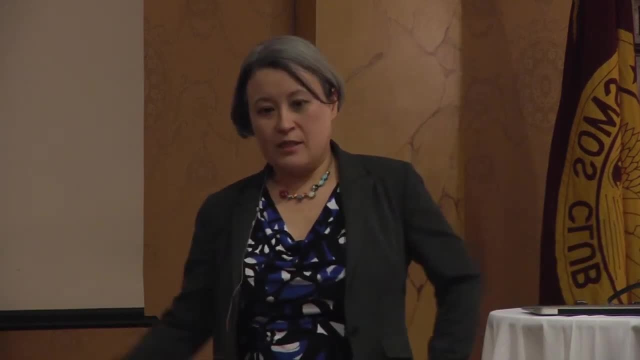 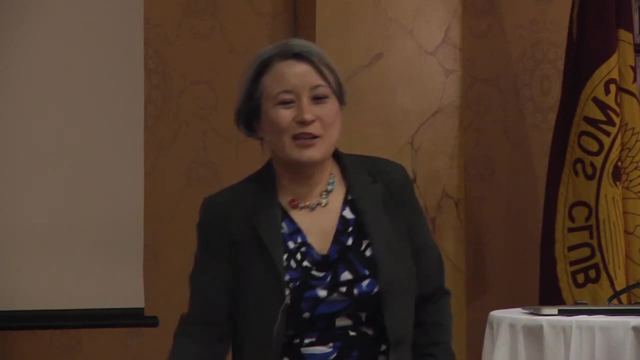 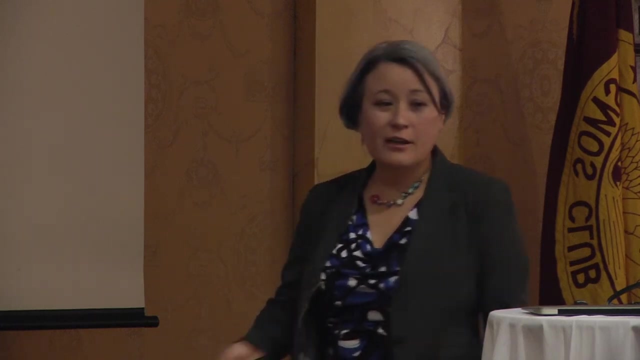 properly on the ground. I mean, the thing is, you know, tens of meters, tens of kilometers, tens of liters in diameter and a full-scale, your full-scale lab would have to be out at the moon, I guess. So anyway, so they have their challenges, They have their development challenges, but in principle they 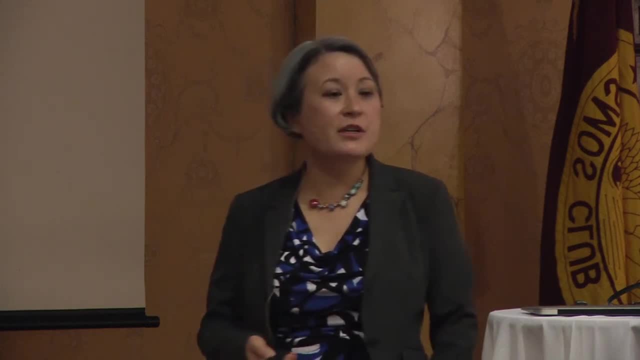 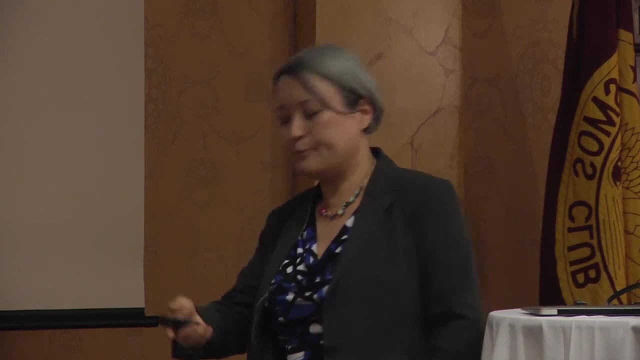 actually are very nice In principle. they can achieve higher contrast than coronagraphs can at smaller separations from the star. We just at the moment it's still kind of like in principle, Okay. so where are we going to develop these two technologies to the point? 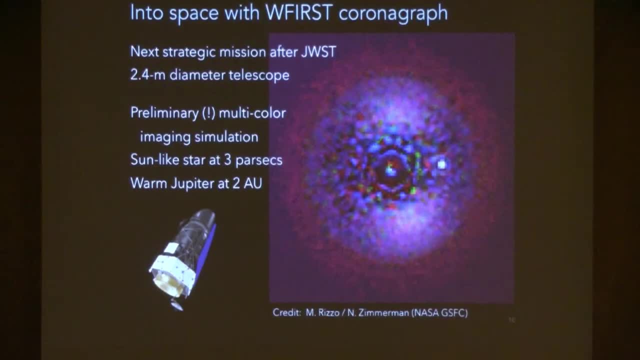 where we actually need them to be. So the first is well, the next step is to go into space with a really the first, really advanced coronagraph, and that will be done with on the WFIRST mission. So WFIRST is the next NASA's. 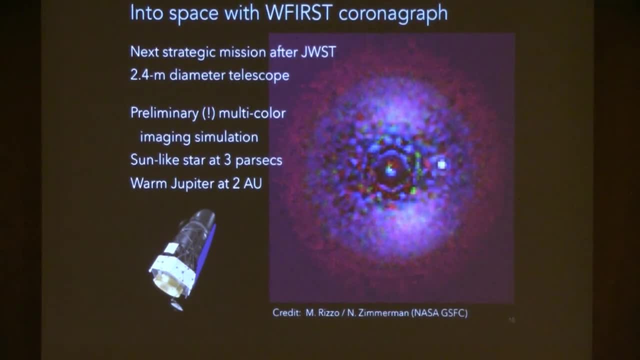 next strategic mission after the James Webb Space Telescope. It's a 2.4-meter diameter telescope with wide-field imaging. It's primarily actually focused on dark energy studies, but in addition it will also carry a first really advanced coronagraph that actually incorporates those deformable mirrors that I showed. 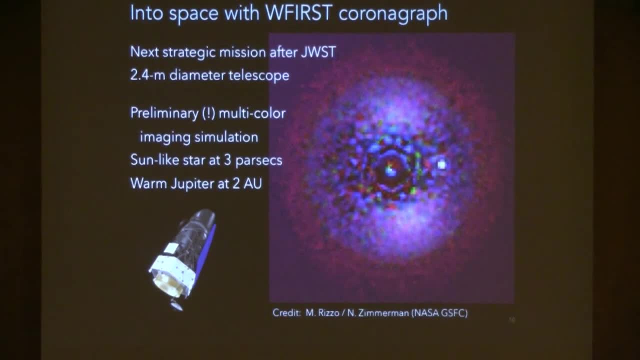 And that. but it is a technology demonstration instrument so it is not at the performance level that, anywhere close to the performance level, that we'd need to do true Earths around suns. but it would greatly advance direct imaging from space And this is a preliminary multicolor imaging simulation of what WFIRST would see, for let's see a sun-like star at 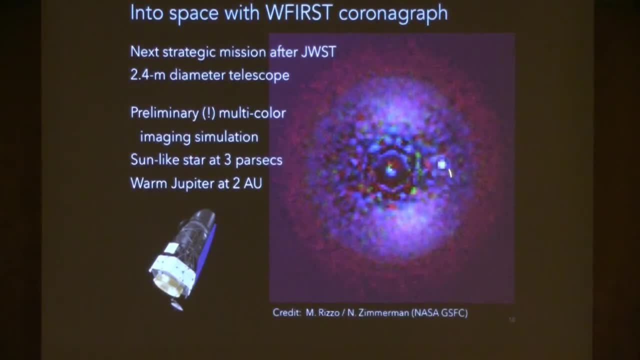 three parsecs pretty close, with a warm Jupiter at 2 AU from the star. And actually all of this haze of light here is light reflected off interplanetary dust in the system which is coming from asteroids. actually It's expected to be there anyway. 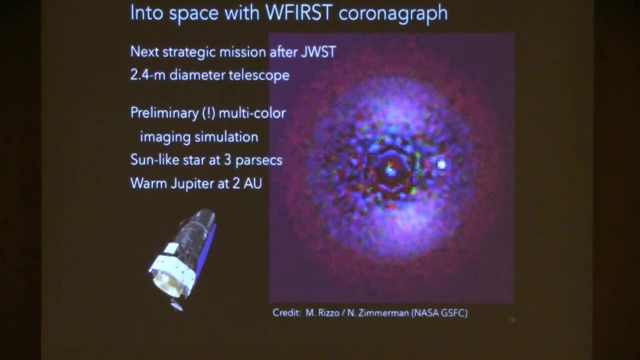 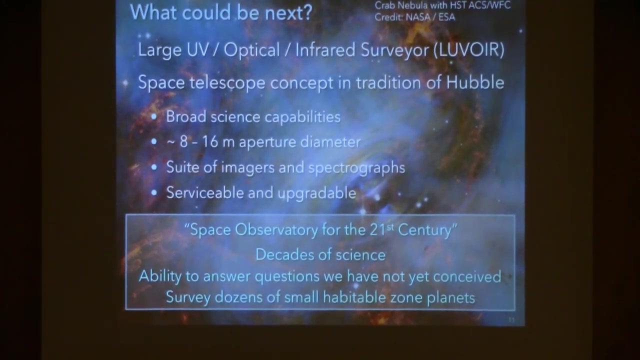 And just as a shout-out here, the simulation was made by Neil Zimmerman at Goddard and Maxime Rizzo, my postdoc, who's right over there. So Okay, but like I said, so WFIRST coronagraph should greatly advance the coronagraph technology. 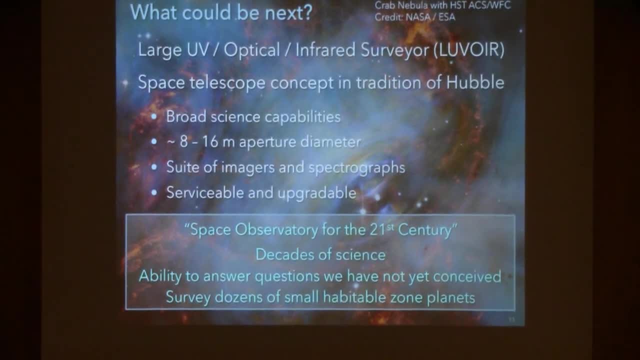 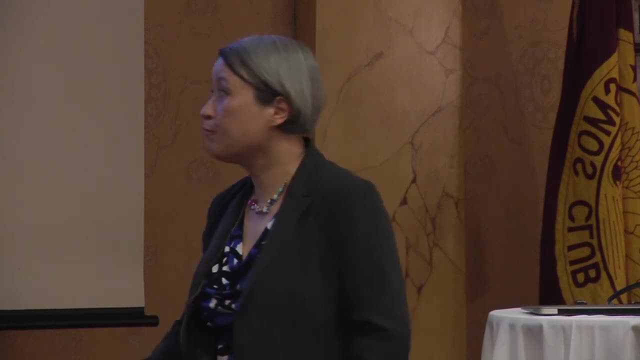 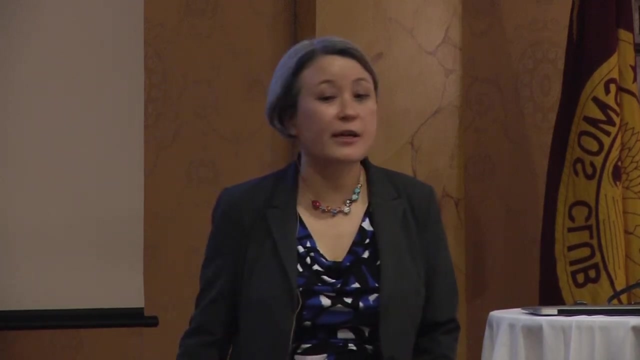 I should. yeah, also I should say there is some talk about possibly flying a technology demonstration starshade with WFIRST as well as sort of like, as a follow-on towards the end of the mission. But again, neither of those devices paired with the WFIRST telescope are going to get us there and, to be blunt, the telescope is just too small. 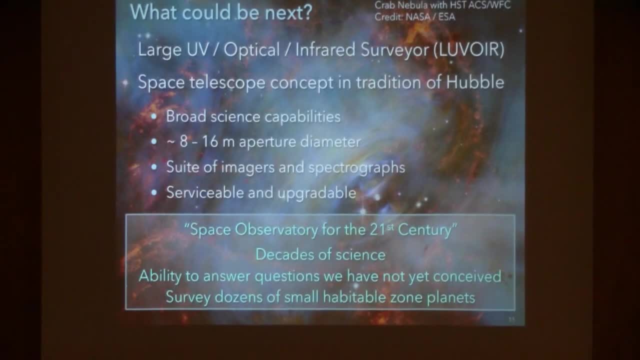 So what? What do we want to really do? So NASA started a study, a three-year study, of a concept for another strategic mission that would come even after WFIRST. So it's called Large UV Optical Infrared Surveyor, or LUVOIR. 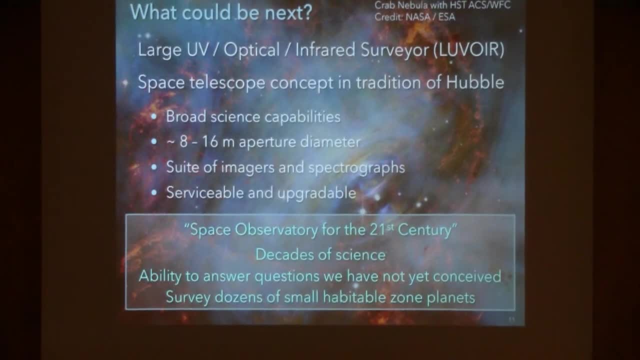 Not the catchiest title, but it's just a working title And this is a concept for a space telescope in the tradition of Hubble. So a truly multi-wavelength facility, A facility with broad science capabilities. Its aperture will be in the 8 to 16 meter diameter range. is what we're studying. 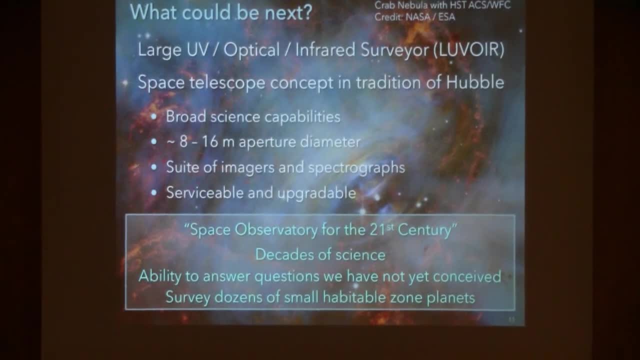 Full disclosure. I'm the study scientist for this effort and Debra is the co-lead of the science team and Sean is the deputy study scientist. So we also envision it would have like a whole suite of imagers and spectrographs, a very diverse toolkit, like Hubble does. 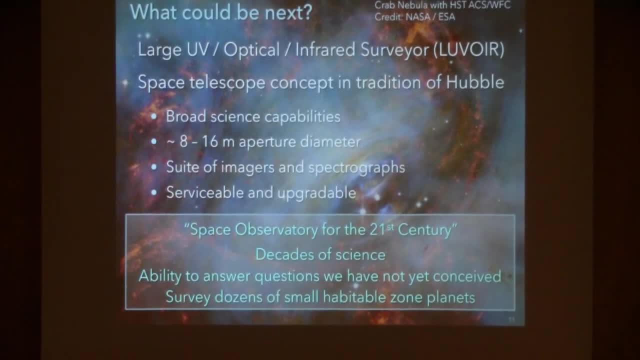 And also, too, it's planned to be serviceable and upgradable from the get-go. We want it to last for decades and carry Have the ability to answer questions 25 years from now. that we haven't thought of right now when we're designing it, which was key for Hubble. 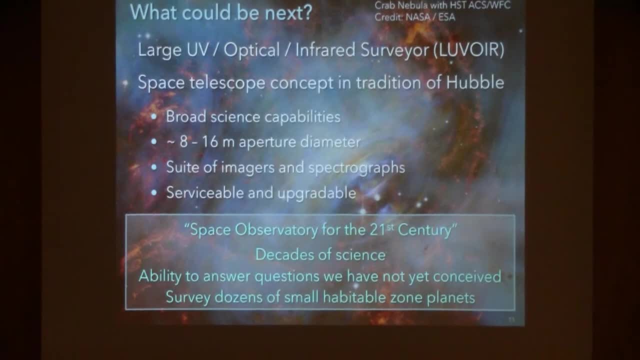 But on top of that its probably key science goal would be to really survey spectroscopically, survey dozens of small habitable zone planets, Actually probe their atmospheres and see if any of them Have show signs of atmospheric biosignatures. 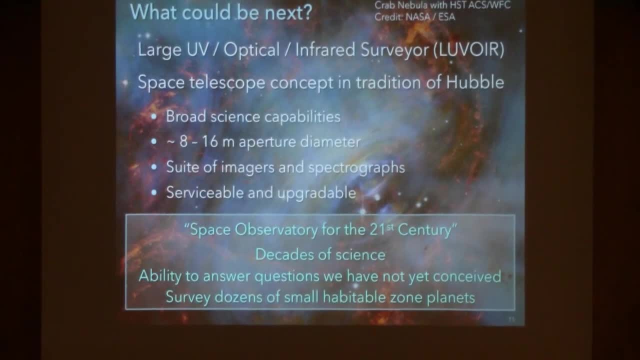 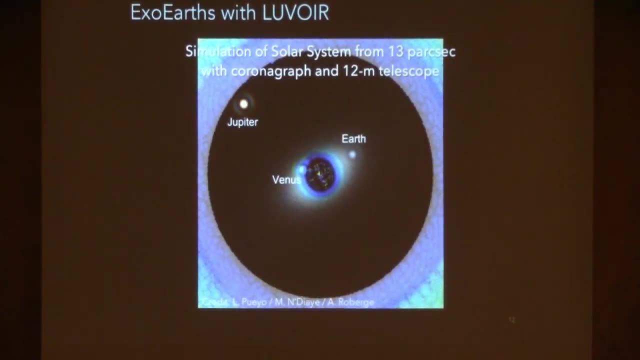 Habitable zone, oh, in particular, habitable zone planets around a wide range of stars, including sun-like stars. Okay so, and this is a simulation of what LUVOIR- preliminary simulation of what LUVOIR would see, This is the solar system from 13 parsecs, with a chronograph and a 12 meter telescope: Jupiter, Venus and there, the pale blue dot that we're actually hunting for. 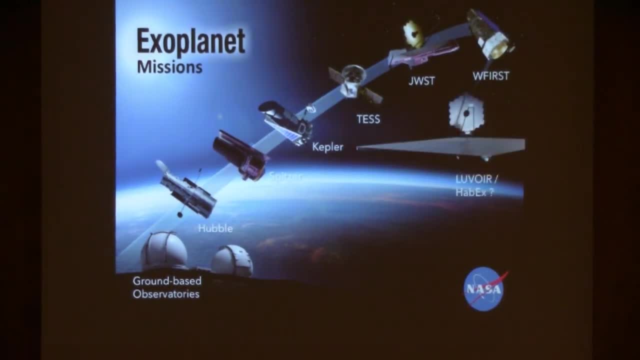 Okay, so just to wrap up, we'll fill out the rest of the NASA mission swoosh here. So moving forward to WFIRST and then hopefully to LUVOIR, or a different concept that's quite similar to LUVOIR, that's called HABEX. 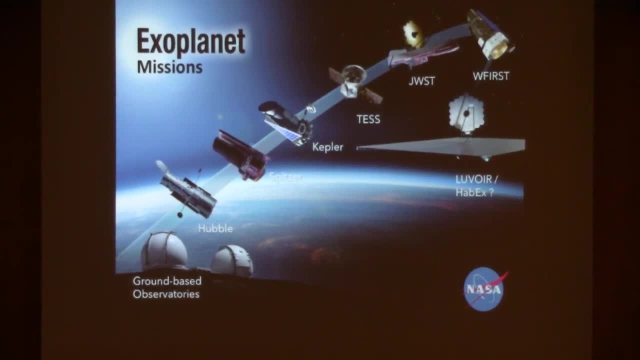 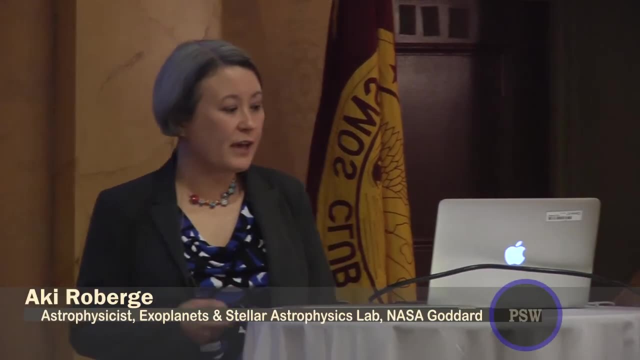 So there is a possible path stretching out over the next decades that leads to the first survey for planets that could actually be hospitable for Earth life, And, furthermore, if that kind of life is not extremely rare, then we'll have a fighting chance of finding some. 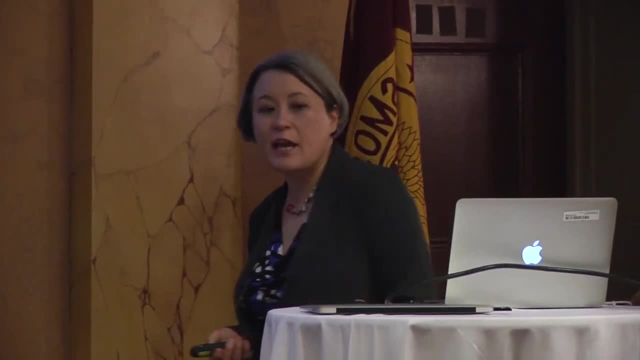 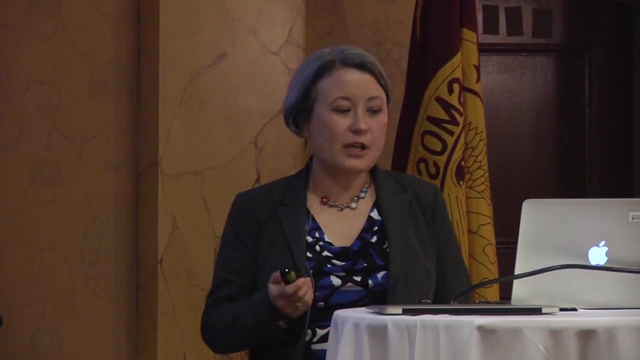 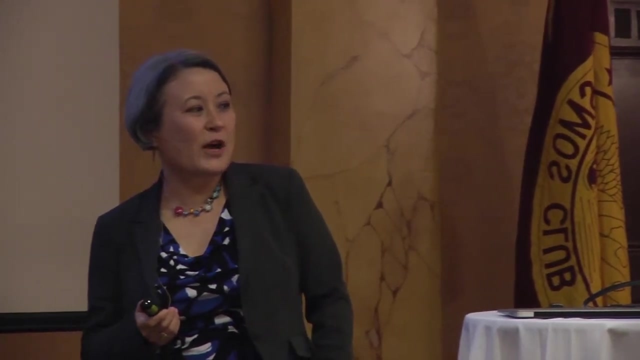 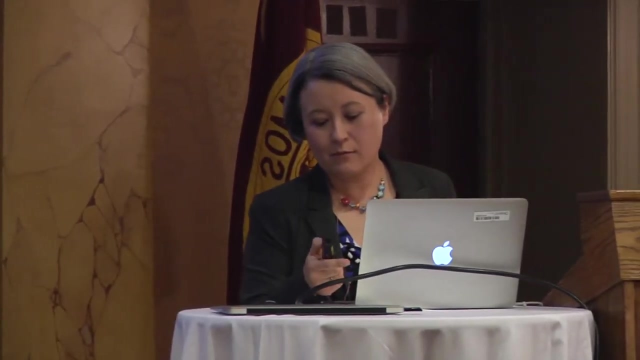 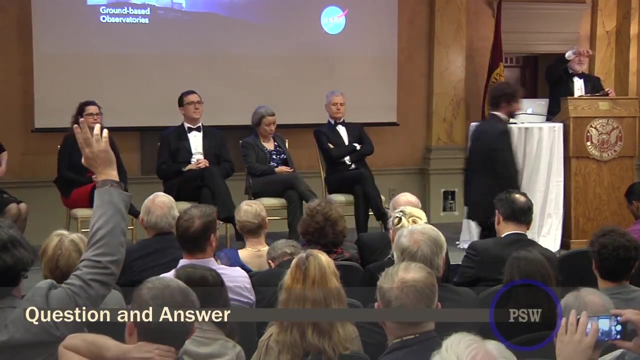 And so I'd say we're really in the exciting position of possibly answering an ages-old question about our uniqueness in the universe, Or perhaps actually, even more likely, finding out if we're actually asking the right questions. So okay, When you have a question, put your hand up in the air and a microphone comes to you and I will point to you and call your name. 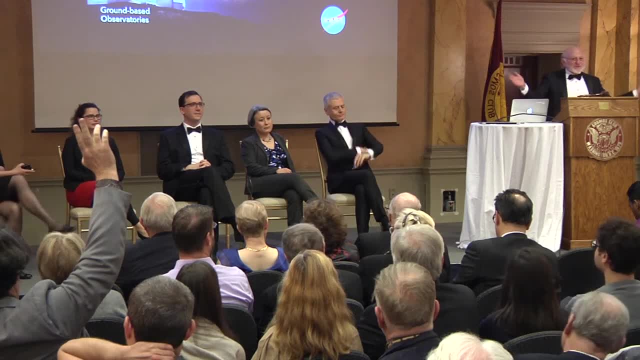 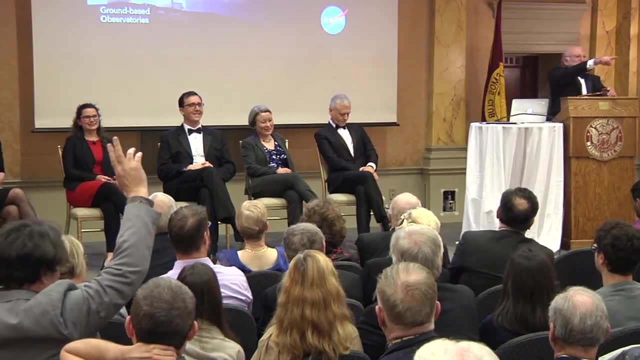 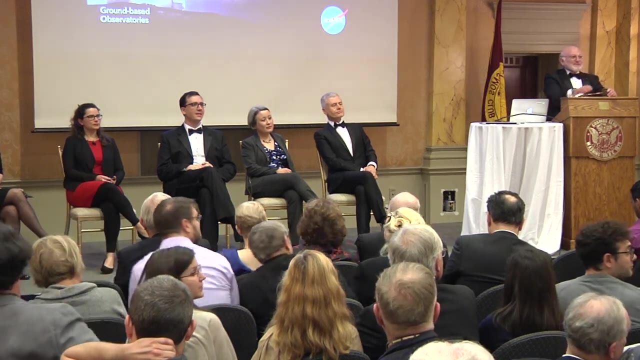 Stand up, tell us your name and ask a question. No speeches, just questions. Speeches come in the social hour. Okay, so there's a question in the back there You have to hold it close to your mouth. Hi, I'm Joseph Powers. 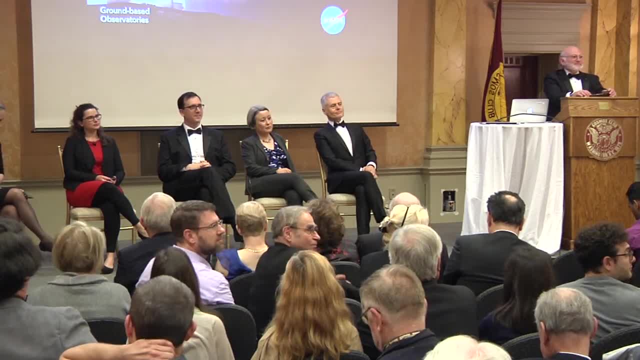 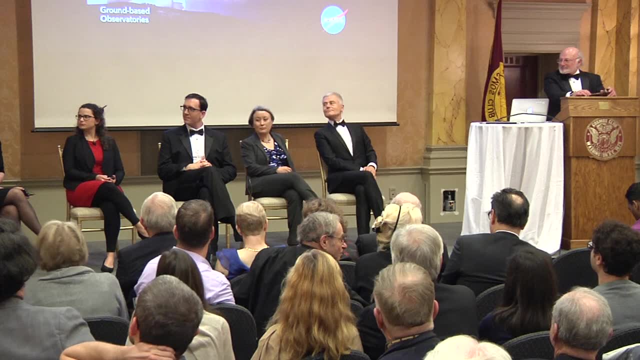 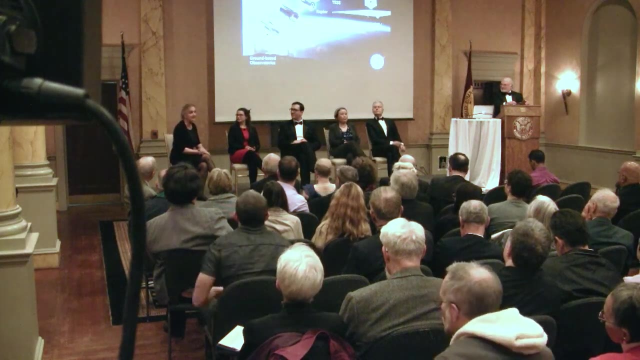 My question was: I see that it's just groundbreaking. There are ground-based observatories there, So where do next generation ground observatories like the 30-meter telescope and the giant Magellan telescope fit into this scheme? Okay, yeah, Right, so that's an exciting question. 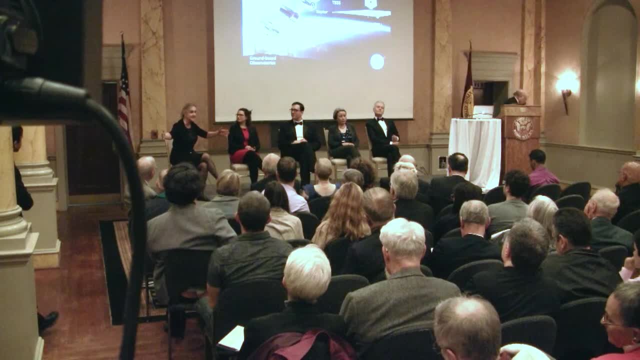 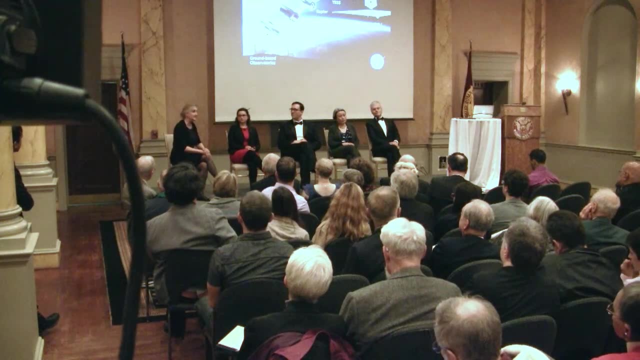 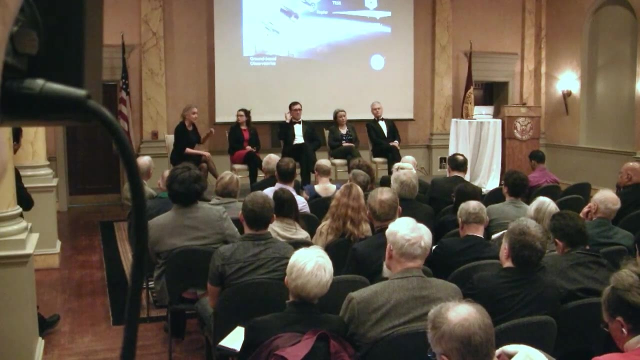 As these giant telescopes- 30-meter class telescopes- are built on the ground, they'll need to correct for the Earth's atmosphere, atmospheric distortions, And so fancy AO systems are being developed And I expect that there's going to be a lot of progress with those telescopes. 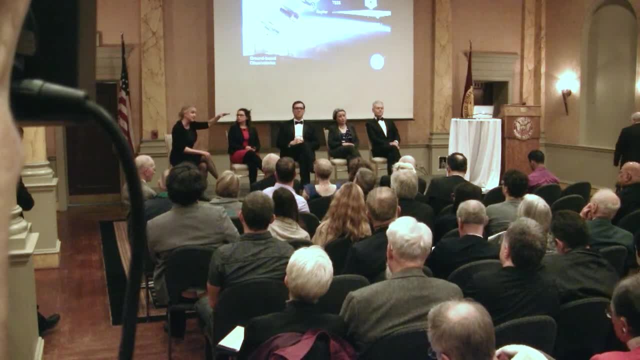 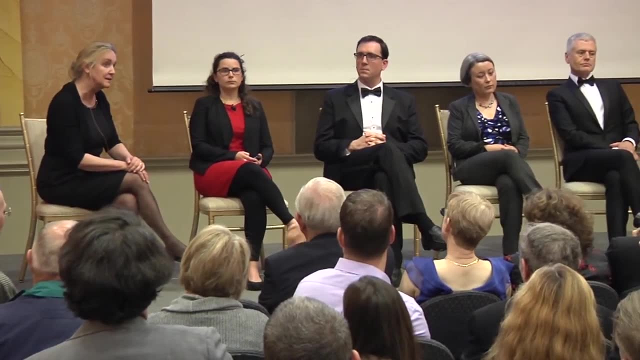 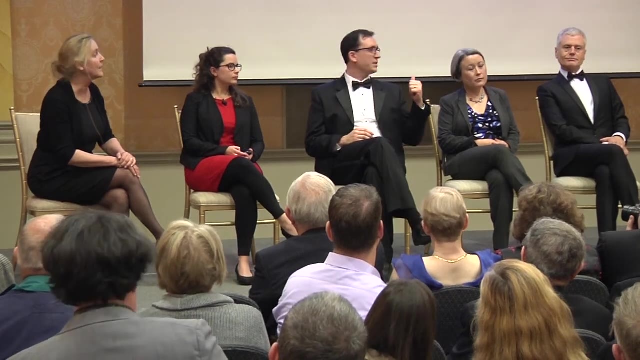 But I see those telescopes as providing a bridge to the space-based telescopes. It's just impossible, I think, to beat the resolution that you can get from space. One of the first questions we ask ourselves when we design one of the next generation missions is: 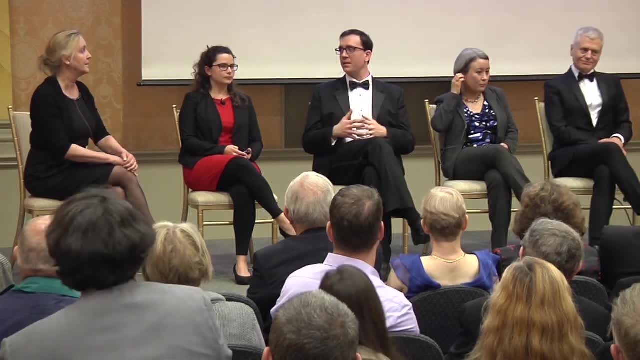 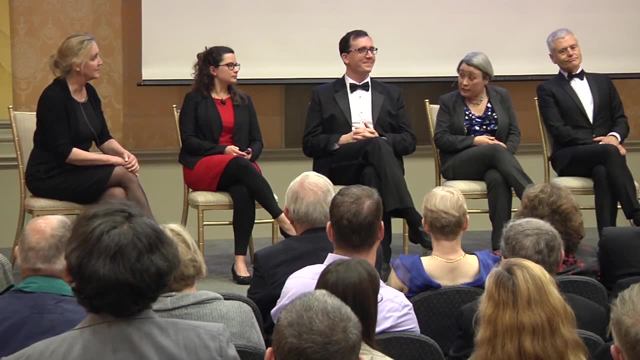 what do we think the ground's going to be doing? Let's not duplicate that effort, let's complement it. Yeah, exactly, Absolutely. If we can do it from the ground, we don't do it from space. But what, I guess I would add though? 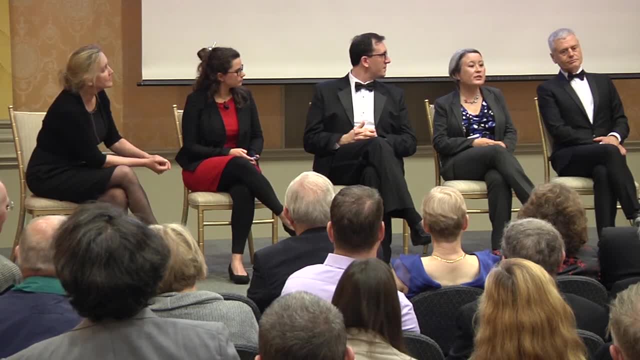 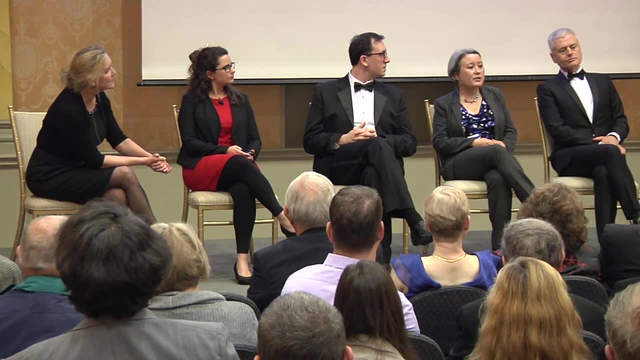 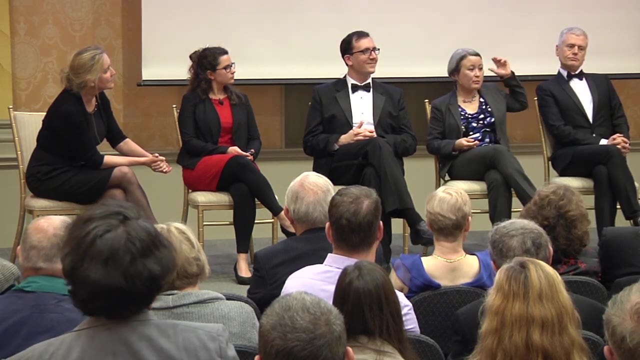 what I think the ground-based extremely large telescopes, or ELTs, that are coming. they should be able to do direct observations of Earth-like planets in the habitable zones of M dwarf stars. So in that sense it's very complementary to a space mission like LUVOIR or HABEX. 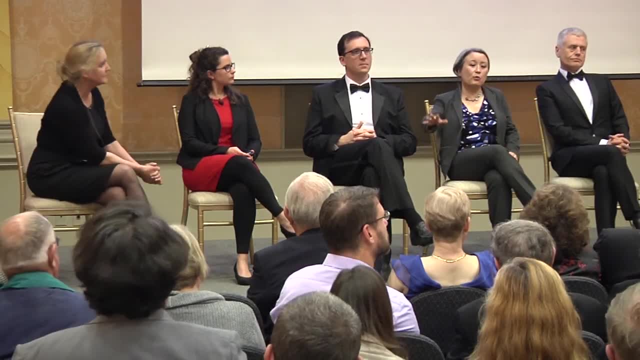 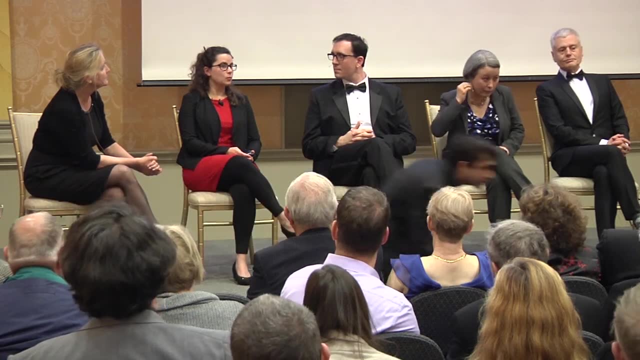 LUVOIR and HABEX would focus on the sun-like stars, and the ground-based facilities will focus on the sun-like stars And the ground-based facilities will focus on the low-mass red dwarf stars. Of course, there are problems with the Earth's atmosphere and what it's made up of. 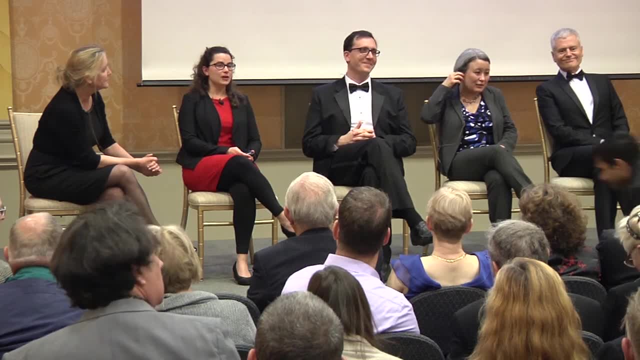 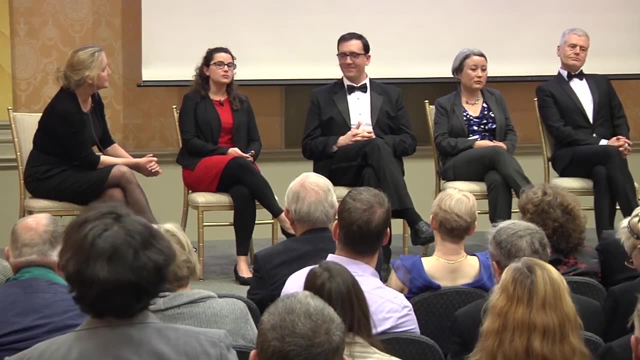 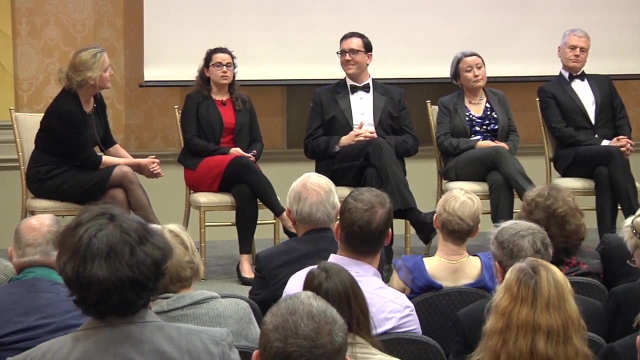 We have a huge amount of water vapor in our Earth's atmosphere That absorbs the wavelengths where we're looking for water absorption in these alien planet atmospheres. The same thing for sodium, the same thing for potassium, ozone, CO2.. Huge amounts of things in the Earth's atmosphere that need to be corrected and monitored over the course of the night. 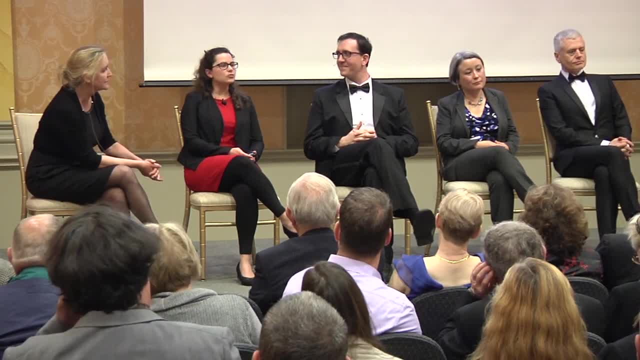 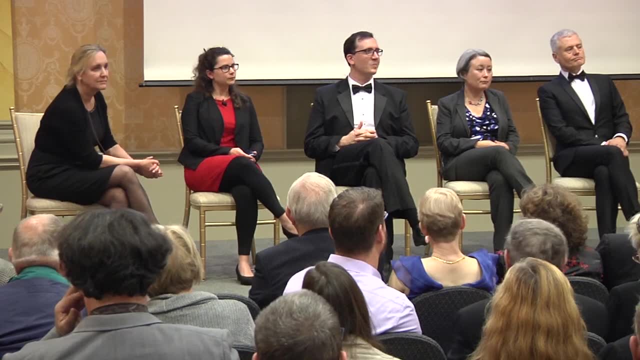 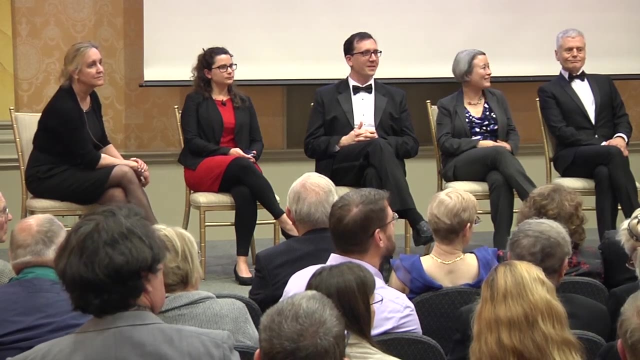 how those column densities are changing. So when we're trying to understand the atmospheres and the environments of these worlds, we really have to consider those when looking from the ground as well. Okay, next question. right here I am Chris, I am a guest here. 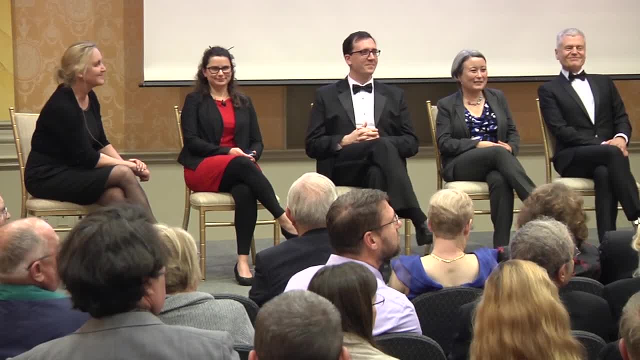 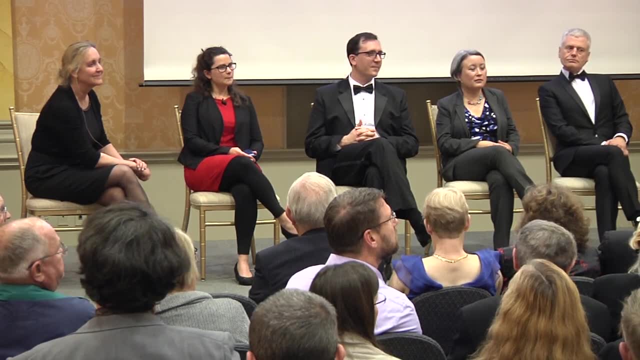 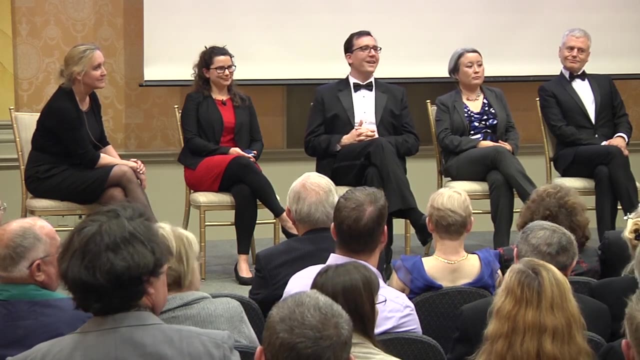 Oh, can you hear me better now? I know you are very confident of finding a planet and some life on it. Is there any way to calculate the age of that exoplanet, Because Earth took about 4 billion years to evolve to what we have today? 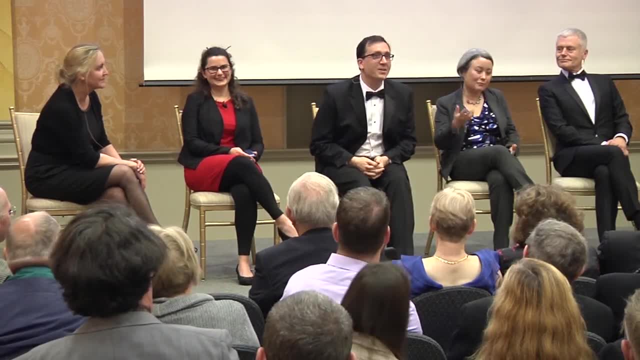 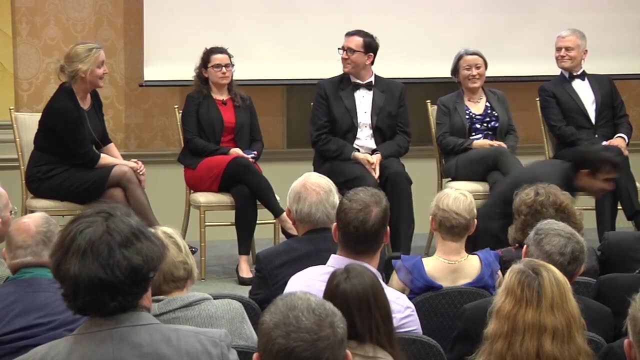 So the answer for the planet is no. And then I'll turn to any of my colleagues, because our best guess is going to be from measuring the age of the star, And they know more about that than I do. Yeah, the planets form with the stars, no question. 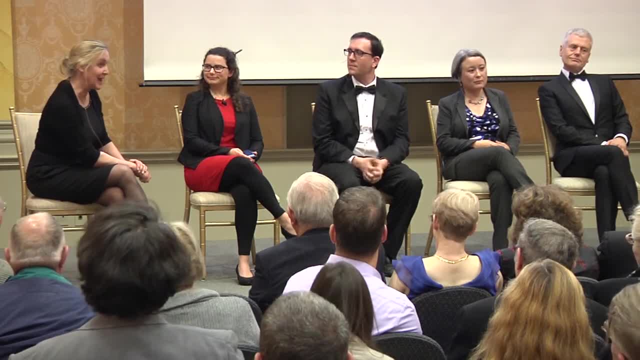 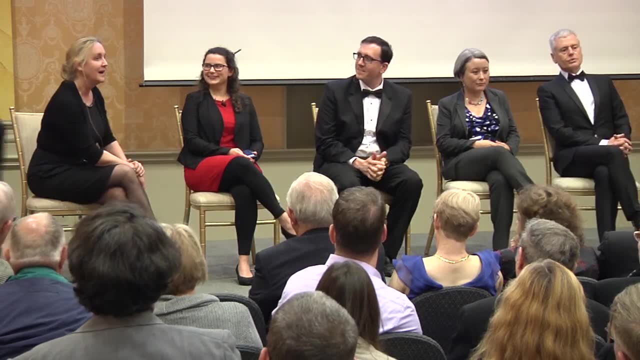 And we're getting pretty good at dating stars now, Figuring out at least if stars are very young, middle-aged or very old. We can at least classify them that way- And most of the stars in the solar neighborhood have ages that are not so different from the sun. 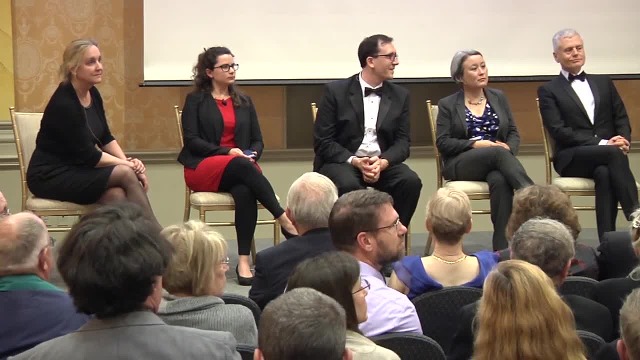 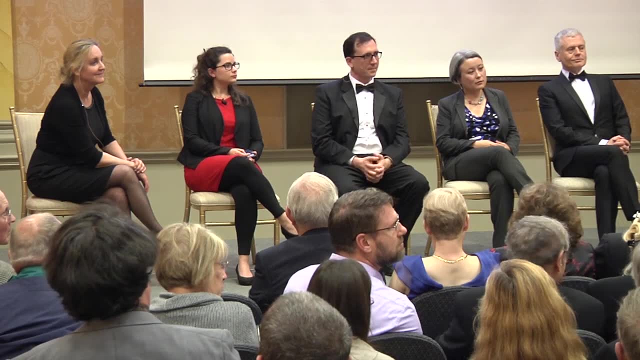 Dr Roberge, you mentioned moving star shields around potentially, And I wondered: you said that it's difficult to do because it's first of all it takes a lot of fuel And also it's moving them large distances. How do you even begin to do that? 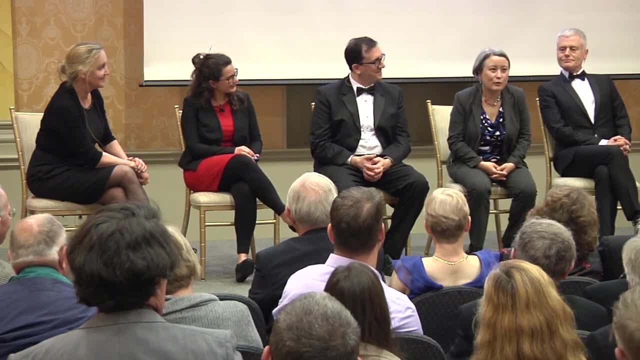 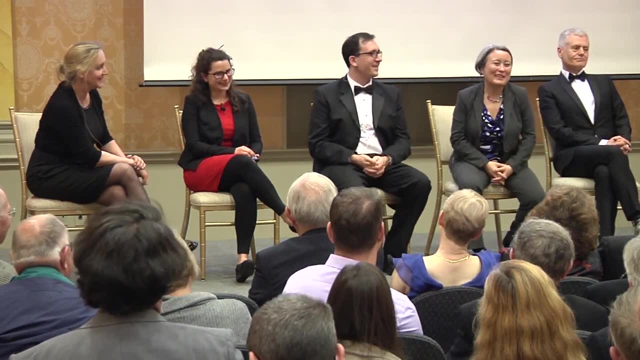 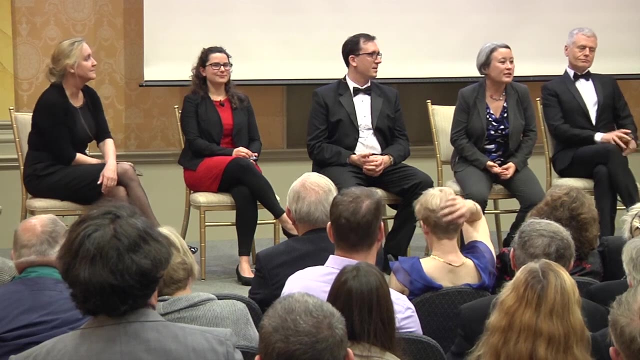 Well, You put little engines on the star shade, Little jets Actually, I suppose ion-electric propulsion, I suppose, would probably be the first thing to do. But any way you slice it, it's sort of a fuel-limited problem. 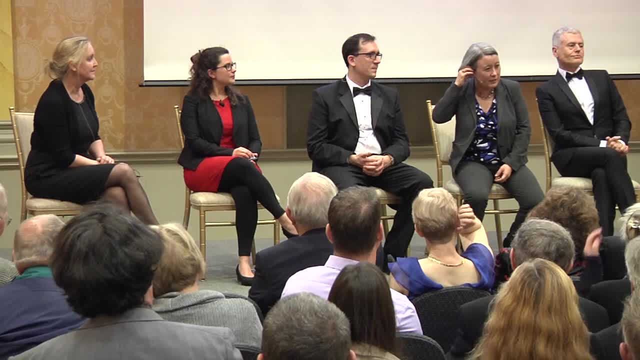 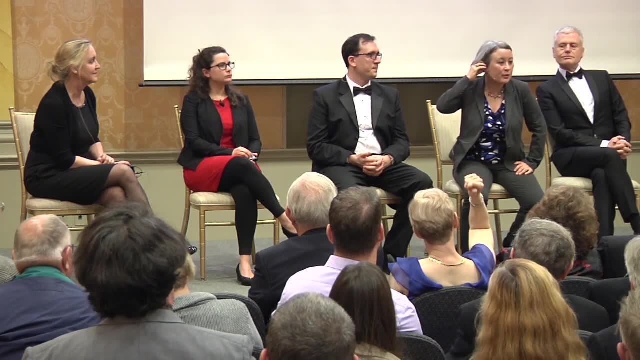 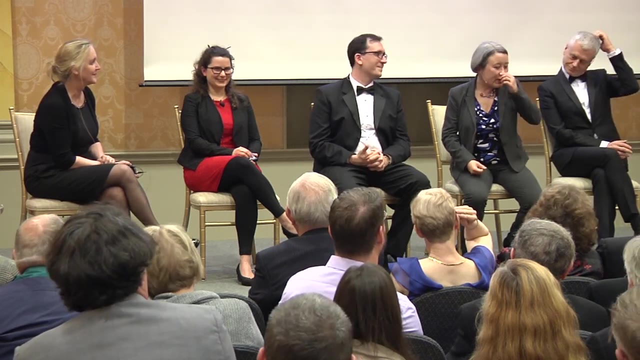 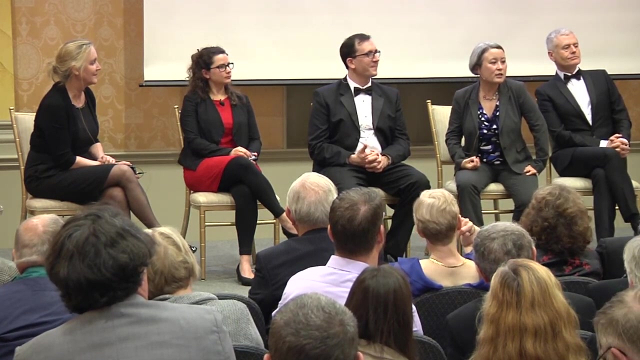 But as you can, I don't know. I mean, I think moving a star shade all over the sky is not insurmountable. That is an engineering problem that can be solved. But the real challenges, I think, are making it, figuring out how to, if it works as a system, making sure that it deploys to the precision that it needs to deploy. 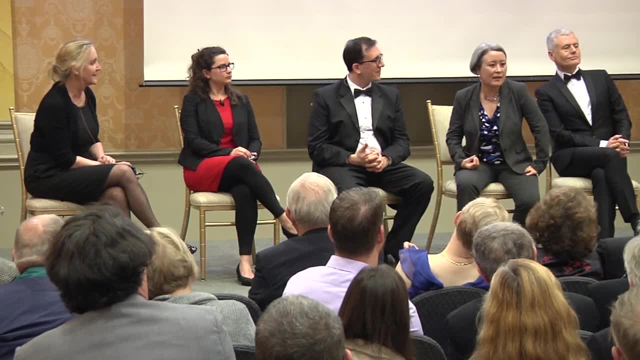 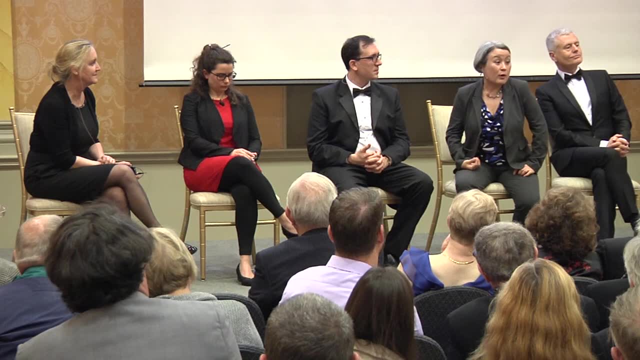 That shape of that star shade is no accident. It must be exactly right And it needs to be. you need to basically deploy to- I don't know, maybe tens to hundreds of micron precision over a thing that's 50 or 60 meters in diameter. 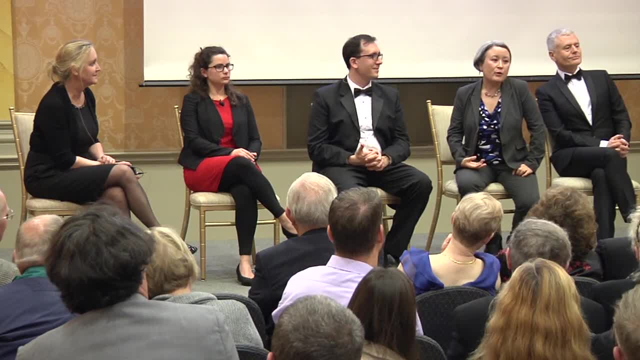 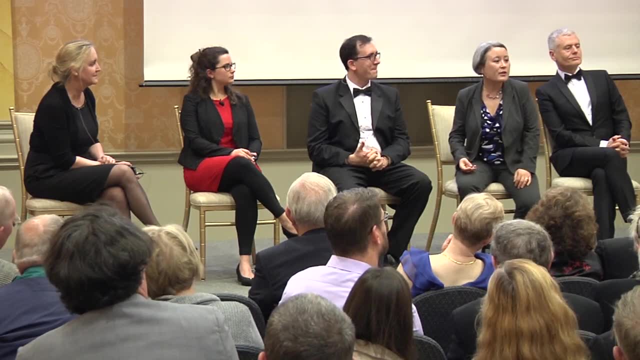 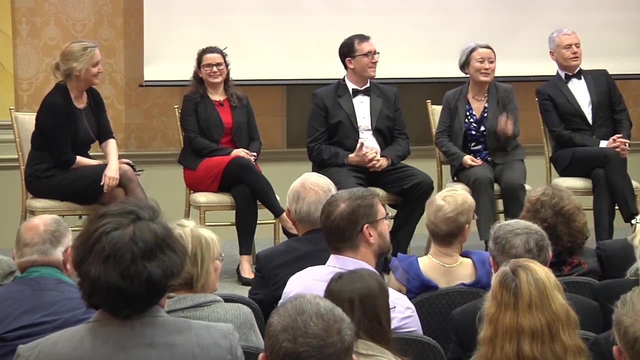 That is no joke. So there are some other issues about how they will work as systems that haven't been investigated yet as well, I would say, because it's really hard to test and study this thing on the ground. Not that Northrop Grumman isn't trying, but shout out there for Albert. 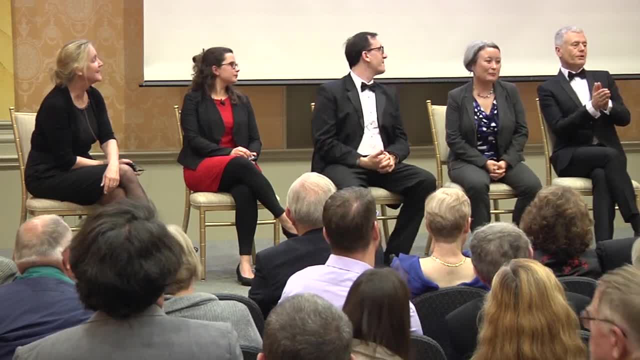 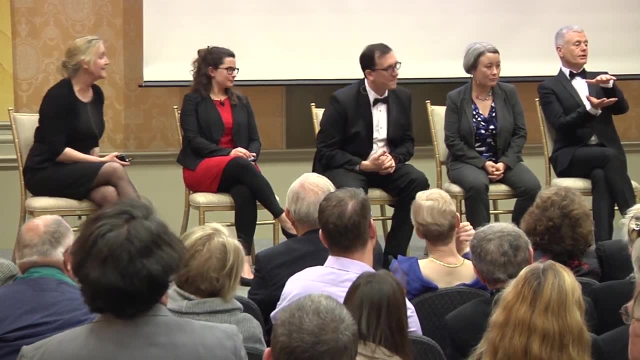 And just to give you an example of how hard that is: on the James Webb Space Telescope you saw the five sunshield layers. We have to align those because you don't want the telescope seeing the layer at the bottom which is facing the sun. 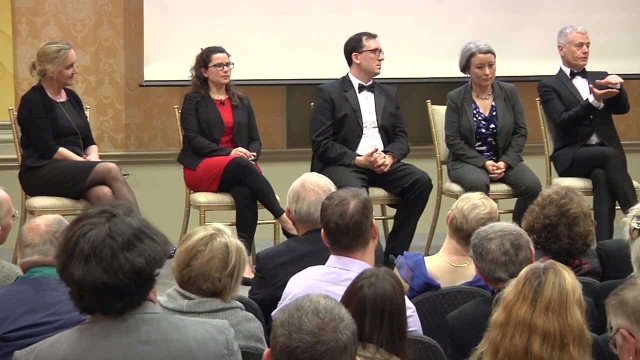 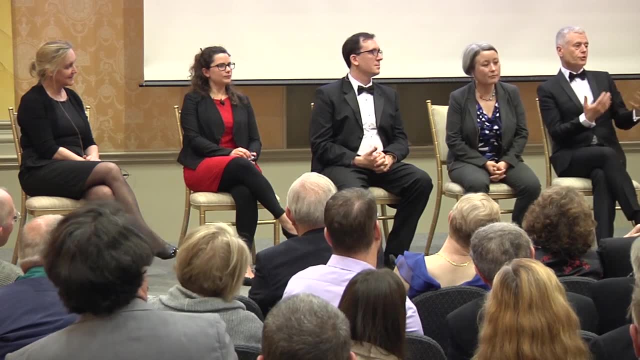 It's therefore warm And that kind of alignment is around, you know, a few centimeter kind of tolerance for each of the layers. So you're talking about, you know, many orders of magnitude improvement in being able to predict where everything will be when you deploy it. 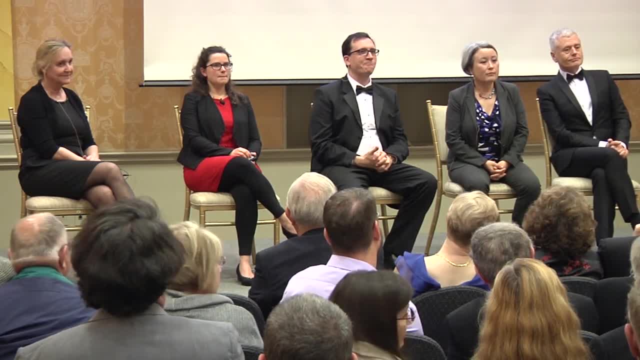 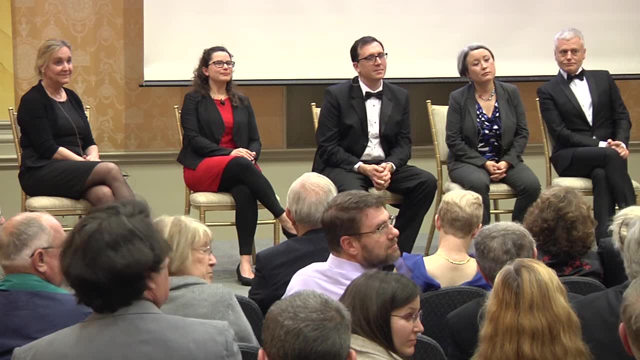 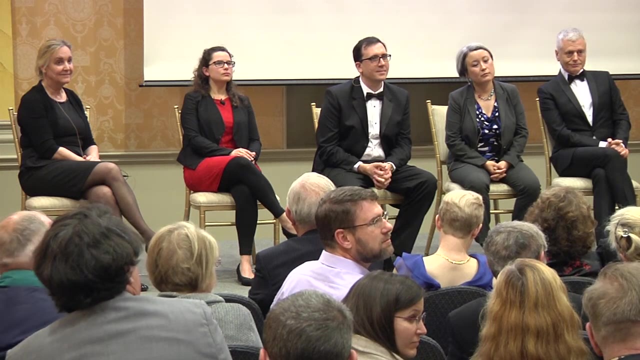 Yeah, Hello, my name is Alon Lanier. I do not work in the field of astronomy, but I did read a little bit about the coronagraph And I did. I do know that James Webb Space Telescope, as you mentioned, will have a coronagraph. 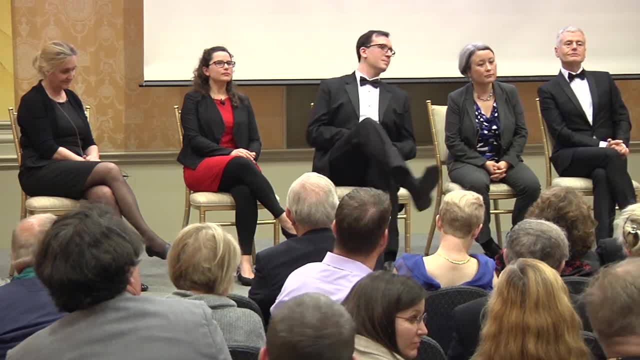 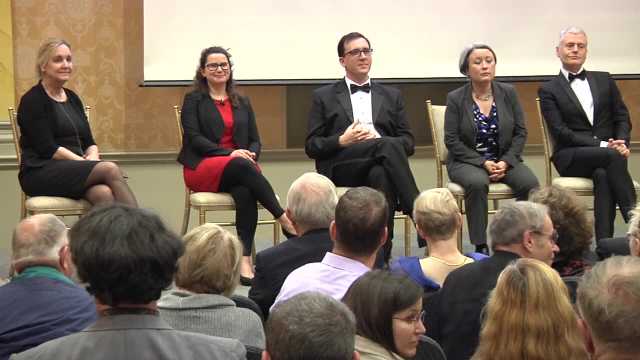 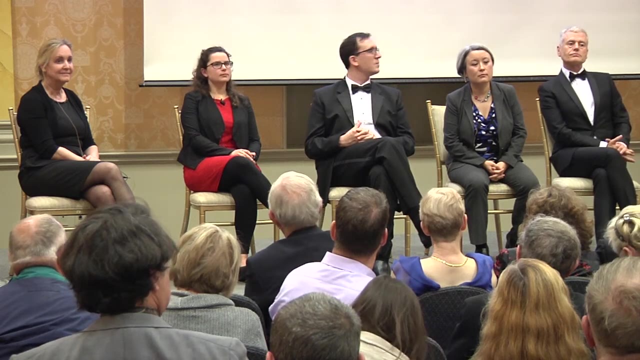 Like: what kind of capabilities will that coronagraph have regarding exoplanets? And second, I've read about other things like that the Subaru Telescope just had a coronagraph And this university in Caltech. they developed what is called high resolution spectronomy. 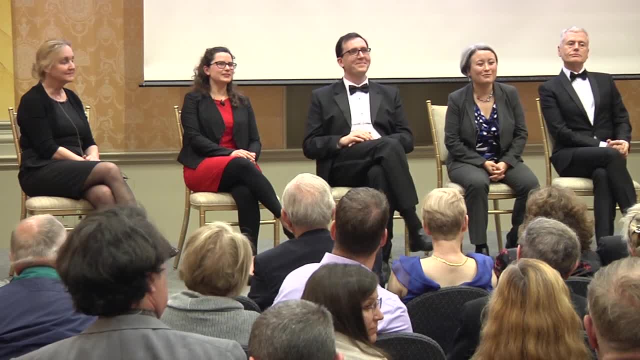 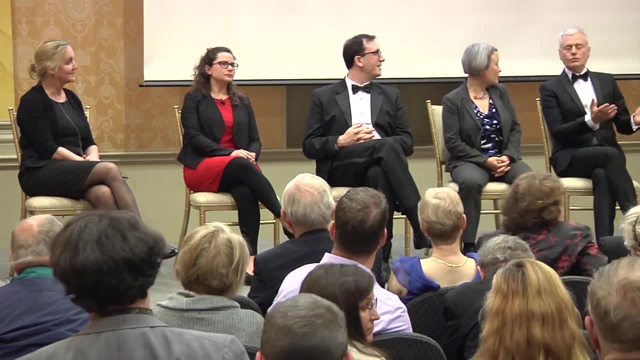 And really I don't know anything about these technologies, But if you can explain how they, a little bit about those and how they might affect the search for exoplanets. So the James Webb Space Telescope coronagraphs were designed some time ago. 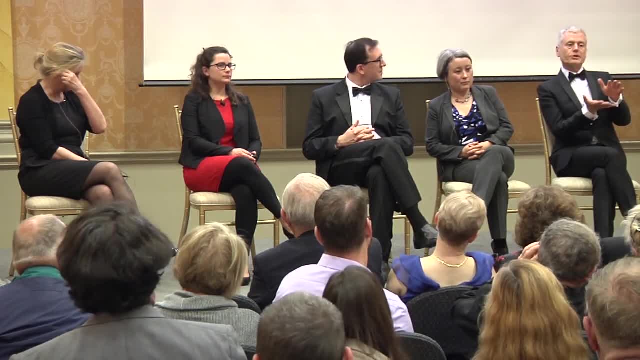 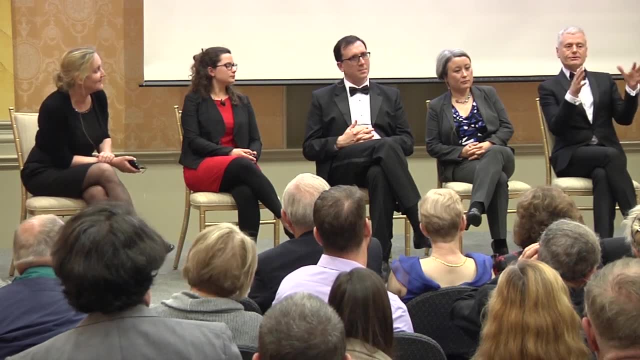 And we measure the performance of coronagraphs in terms of their contrast. So, as you heard from Aki, to see Earth-like planets around you know sun-like stars, you need to be getting to contrast levels of around you know 10 billion. 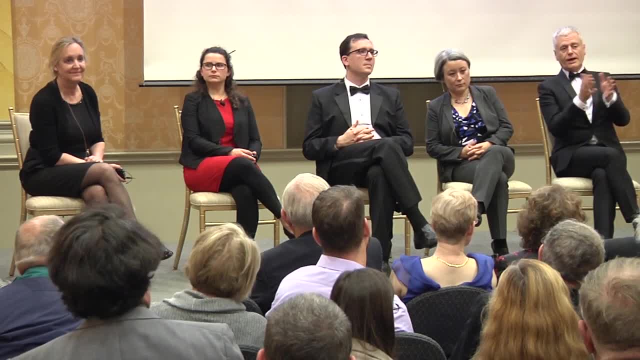 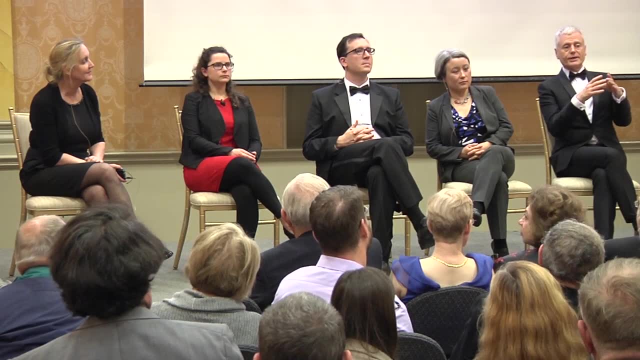 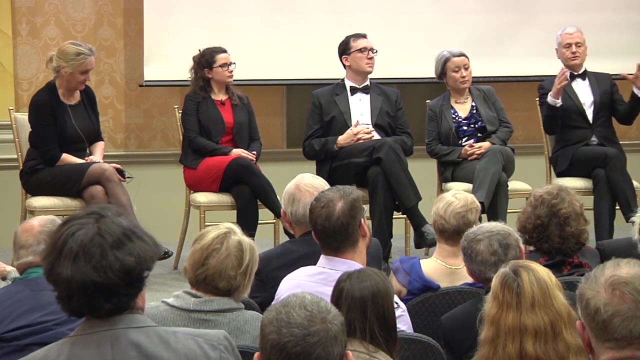 The James Webb Space Telescope, contrast is around 10 to the sixth, possibly 10 to the seventh, And we're working in the infrared so we cannot see that close in And it's really designed to do observations of gas giant planets at fairly significant distances from the stars. 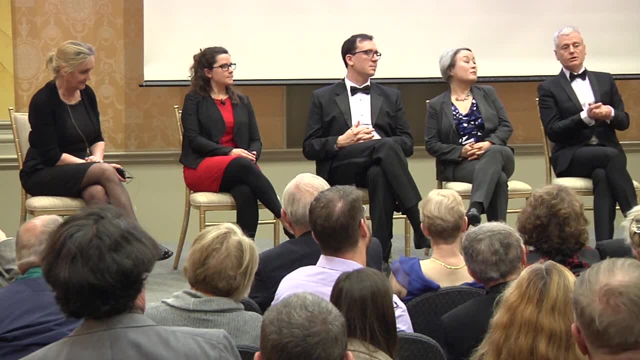 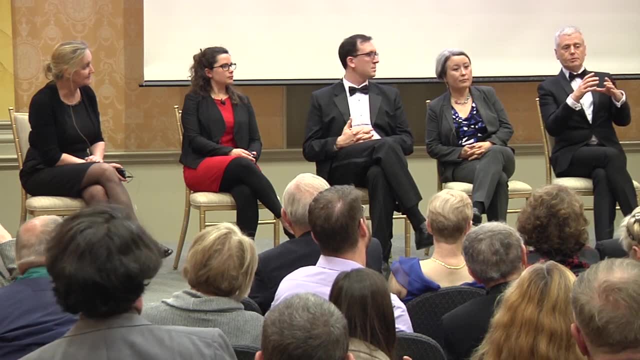 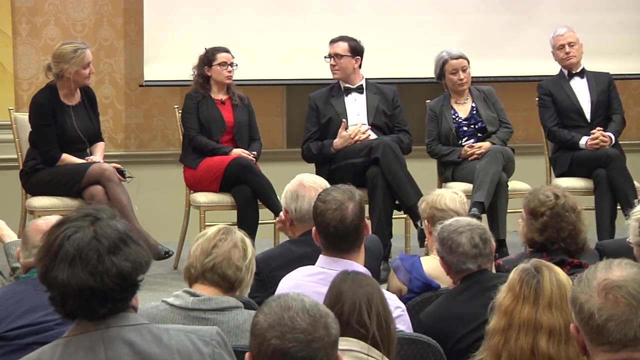 like Jupiter and Saturn in their own solar system? Yes, But for the problem it was designed for. it wasn't designed to do this really tough problem of imaging Earths. One thing I will say about the coronagraph from James Webb is these Jupiter-Saturn-sized worlds. 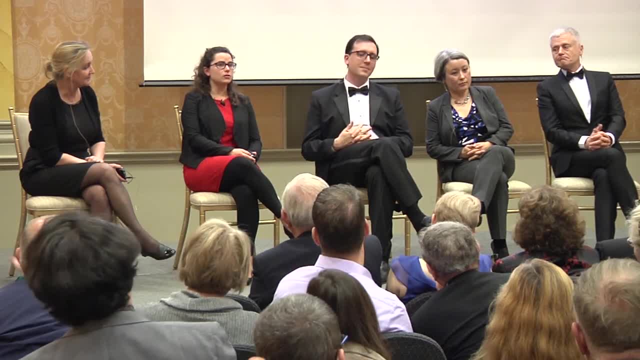 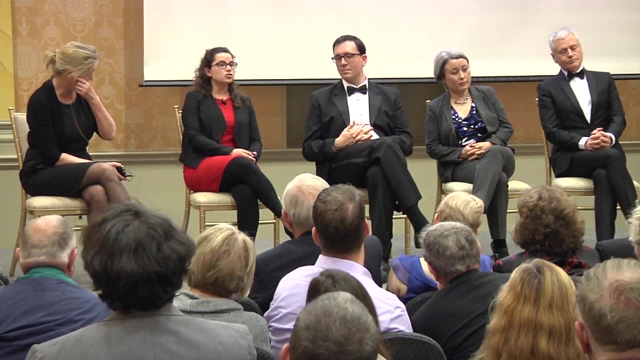 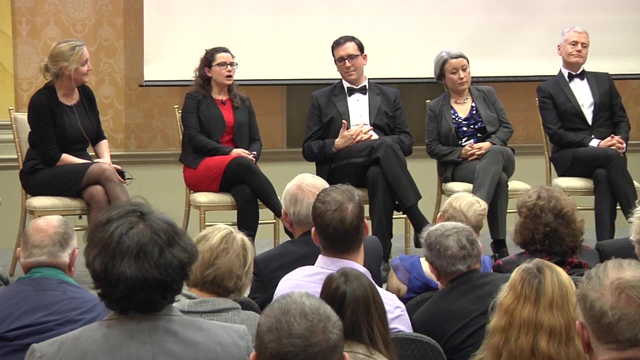 those kinds of distances are very important for our understanding of our solar system, our terrestrial planets and our habitability. So understanding how those objects are shaped in other solar systems is really key for a full and complete picture of our own solar system, And that's why studying and understanding the atmospheres 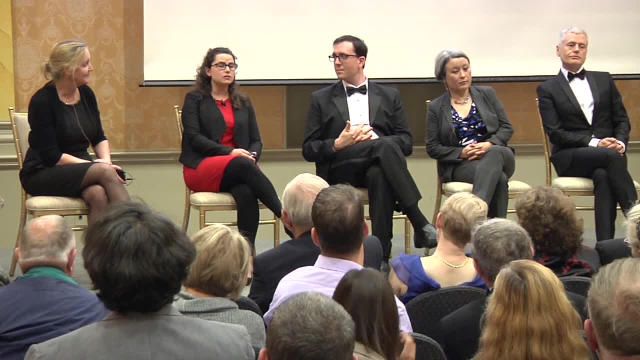 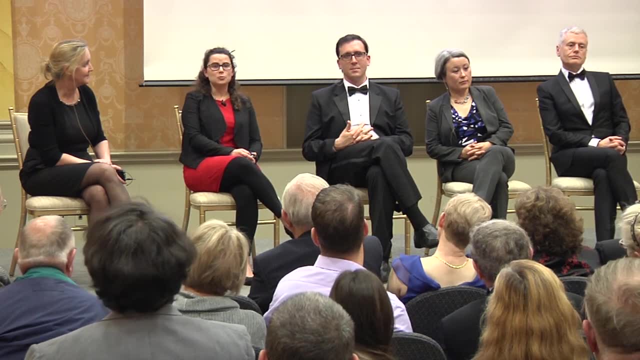 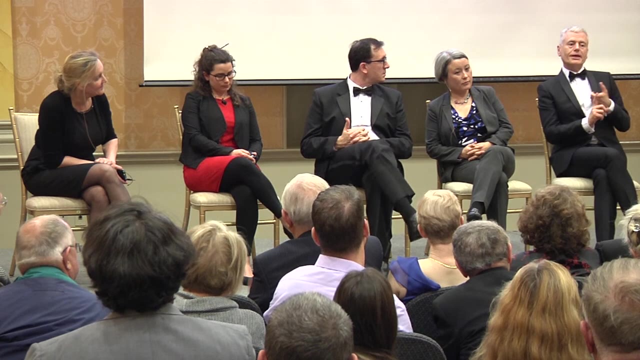 the constituents of these giant planets, the dynamics in those atmospheres is really, really important because it really does lead back to our own planet and our ability to live here. And I'll just add one other thing real quickly: The other unique capability that the James Webb coronagraphs have. 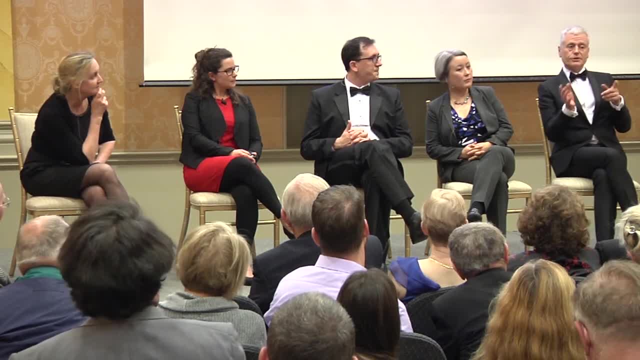 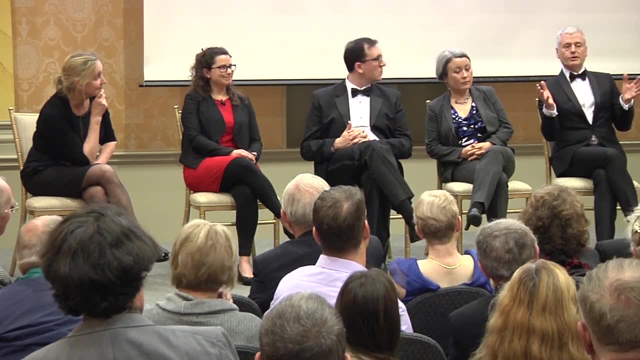 are the mid-infrared imaging from 5 to, you know, just about 30 microns. That we've never been able to do before, So that's a really new capability. It opens up a lot of molecular lines that we haven't really studied before. 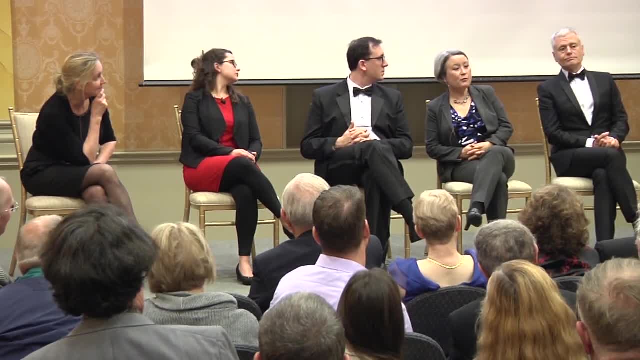 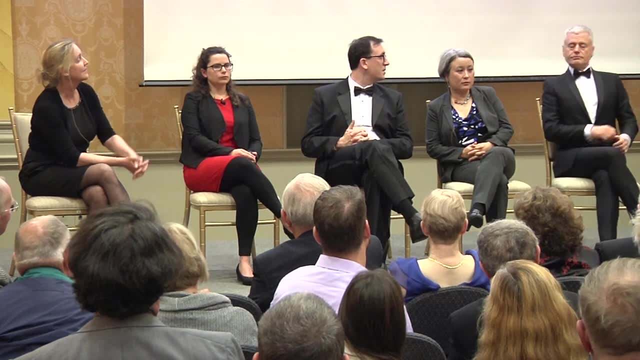 Yeah, but as you said, those coronagraphs don't have deformable mirrors. The high-resolution spectrograph technique you mentioned, that's mostly being developed for the ground at first, Except the high-resolution cross-dispassion. Yeah, the Dimitri stuff. 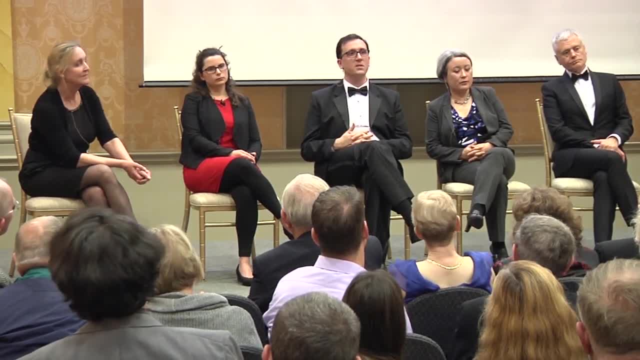 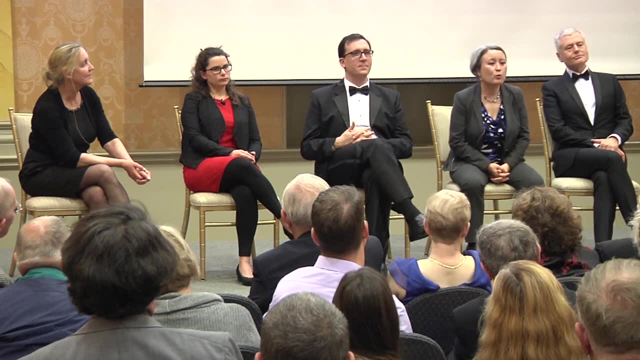 But we are looking at incorporating that into these future telescopes as well. That's a new technique that there's some things to still figure out, actually on how to make that technique work at the really really sensitive levels that you need for Earths around the Suns. 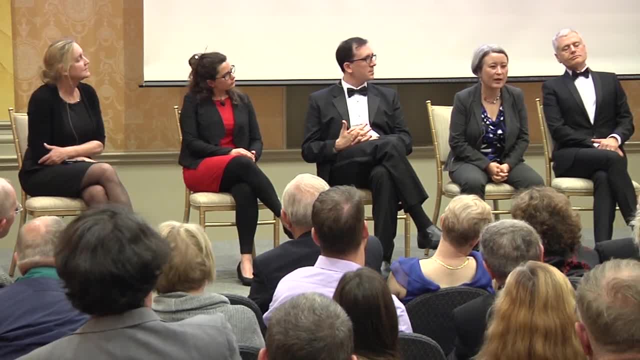 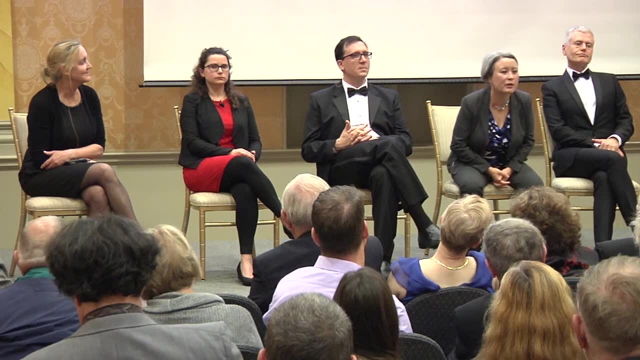 Probably it can't do it by itself, but it might. combined with the coronagraph it might actually give it a little extra oomph. But there's a lot still to study about that particular technique, the one that you mentioned, the high-resolution technique. 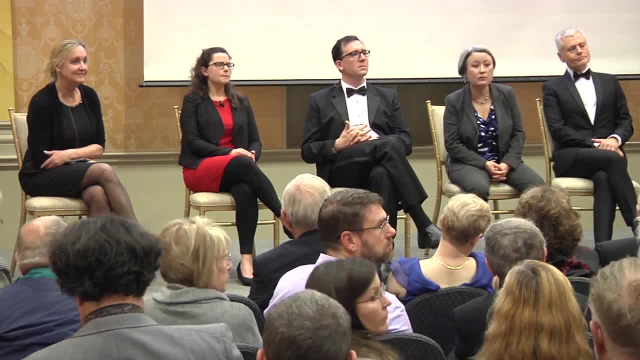 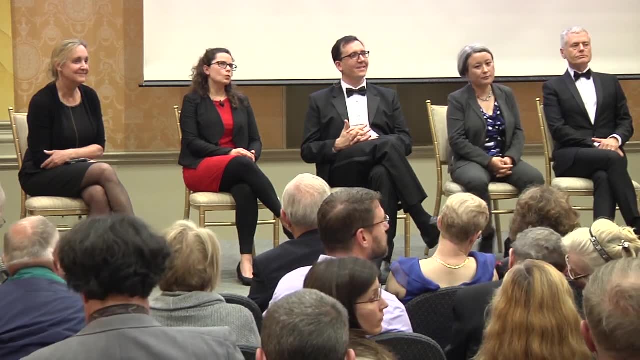 I wonder if you could say something about a different concept of a telescope, where instead- Yeah, it's me again- Instead of these telescopes where you can just reuse it and point it at different stars, if you had something more like a sacrificial telescope. 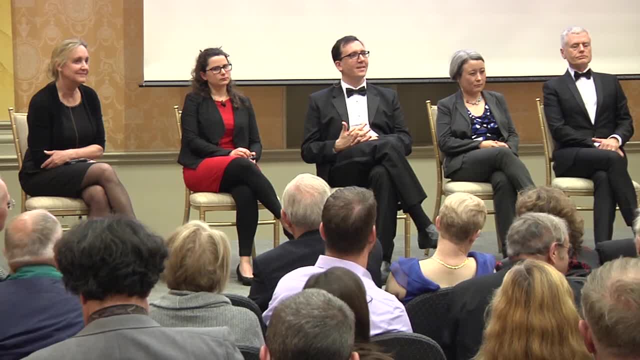 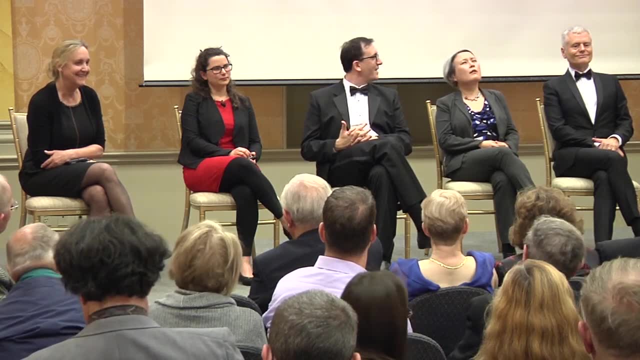 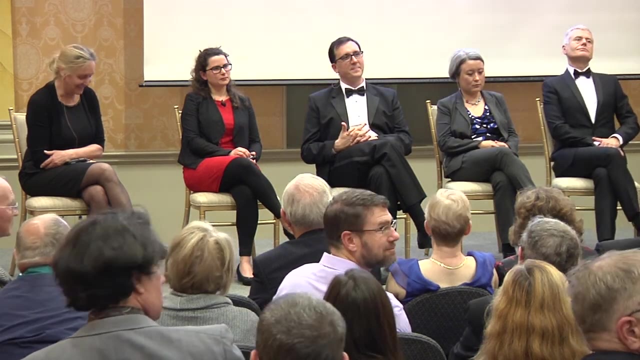 that you send out to the extreme edge of the Solar System and use the mass of the Solar System as your lens with gravitational lensing. if you had one target that you really wanted to look at very closely in terms of the feasible technologies, what could you see with gravitational lensing? 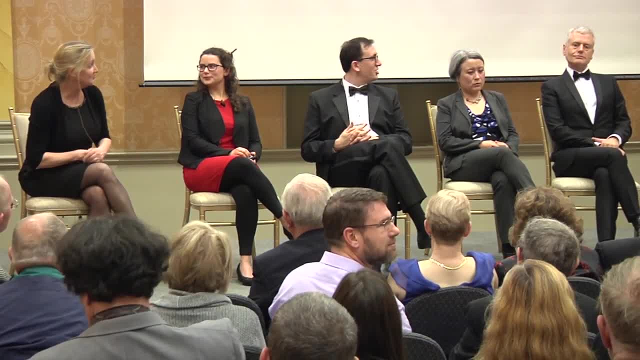 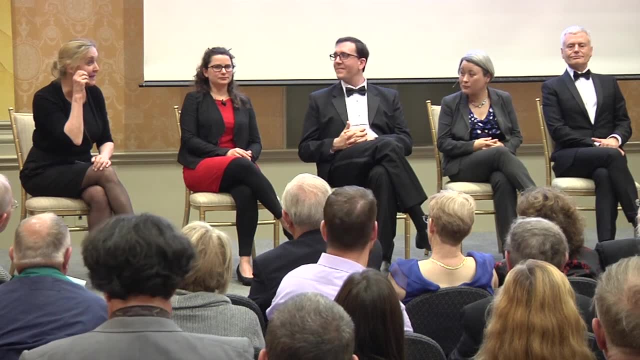 The telescope, aside from the politics of needing to send an actual nuclear reactor and not rely on space probe-grade plutonium. but put that aside, I can say a little bit about that. I was talking to some of my colleagues at Caltech who were talking about that idea. 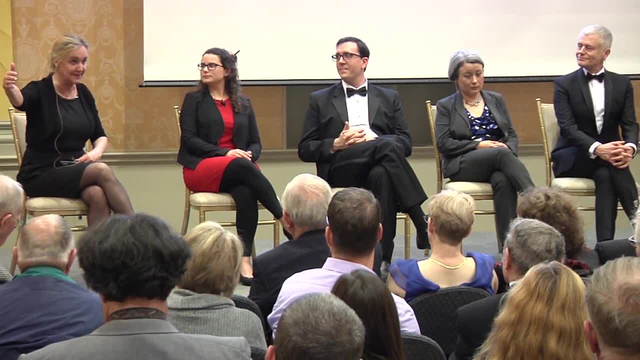 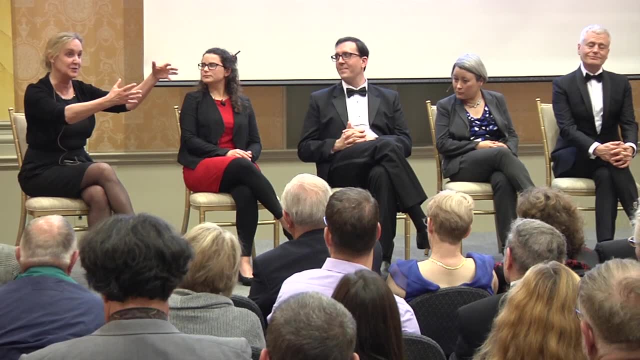 Yeah, so you send a spacecraft out to, as you said, to the outer part of the Solar System. Then you look back towards the Sun and- because the Sun has quite more mass than anything else in our Solar System- as a star behind the Sun, 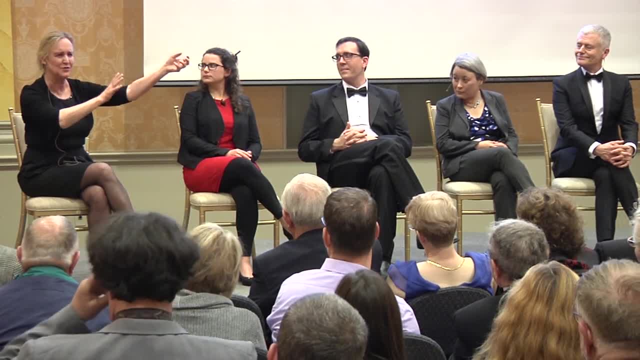 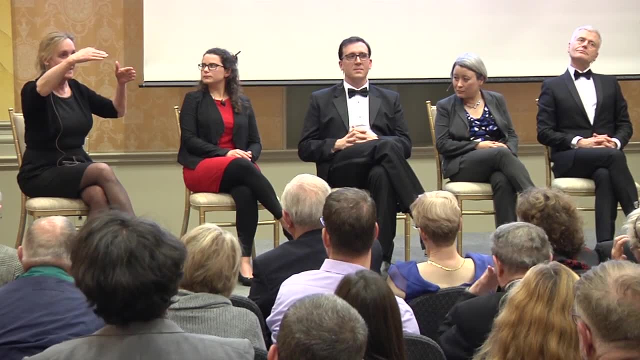 as that light's coming towards us. normally you might think, ah, the Sun will just block it out. But in fact some rays of light from that background object are bending. We would have missed them, But the mass of the Sun warps the space-time continuum. 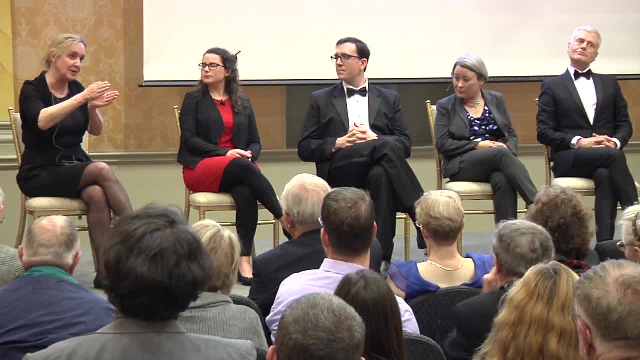 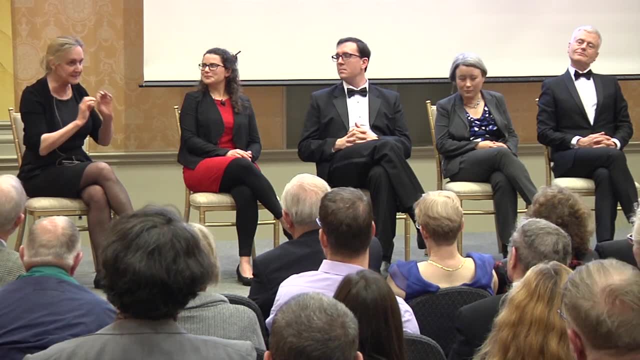 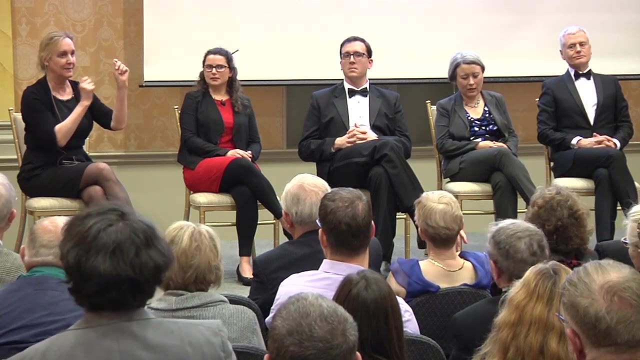 bends the light back to us and focuses it so that we could actually for the right alignment, and it would be totally serendipitous- It's difficult to plan this. You would be able to see with incredible brightness, a planet orbiting a star that's behind the Sun. 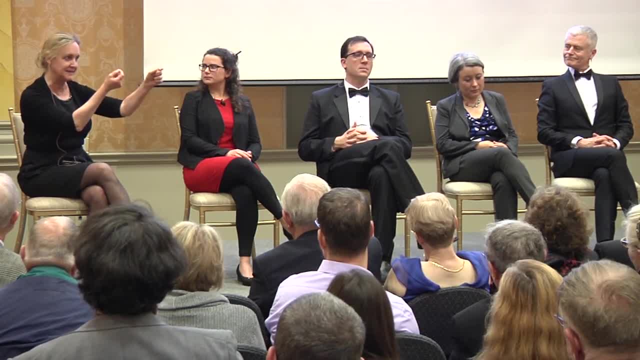 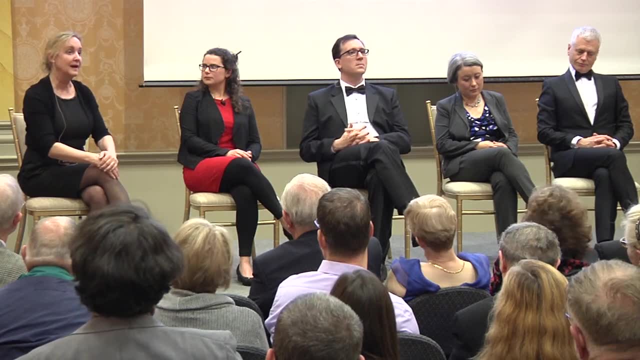 You have to have exact, you know sort of the distances between the Sun and that background object are important and the distance of you to your spacecraft and the outer Solar System are all important. But it does have the potential right to hit the jackpot. 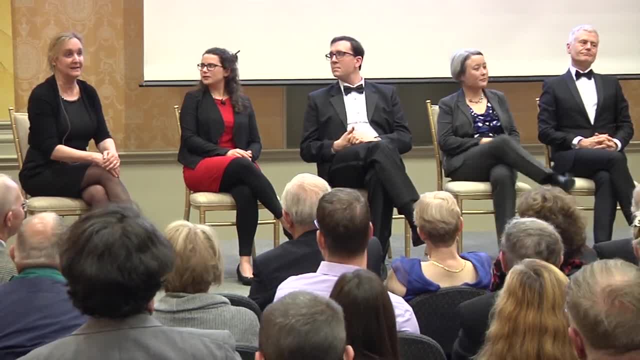 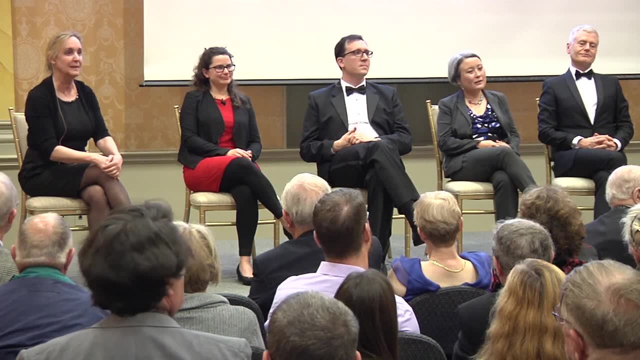 What would you see? Oh, you would see. you would be able to get spectra. You might even see a bright enough image of a planet to see clouds rotating on the surface of the planet. It's a Hail Mary, Hail Mary. Invest in study. 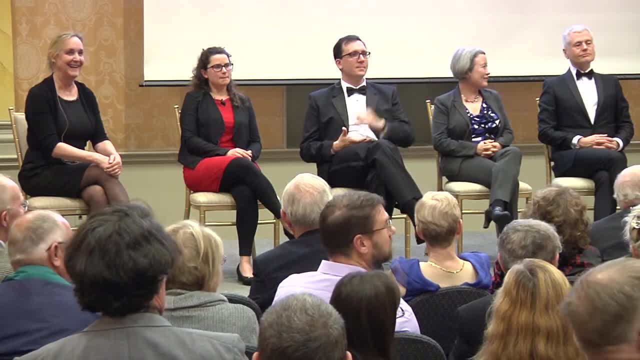 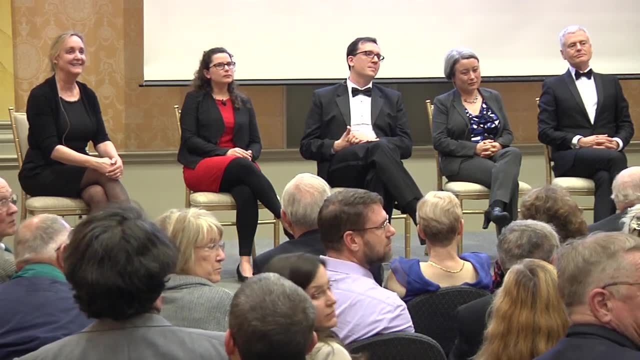 Hi, I'm Patrick Alsup and I've got a couple questions. One of the things I've read repeatedly about affecting the suitability of Earth for life is its rotation rate, and the presence of a large moon Is either of those, and actually I suspect that you probably can detect. 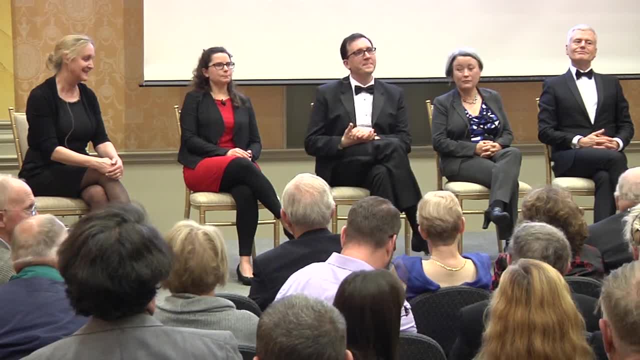 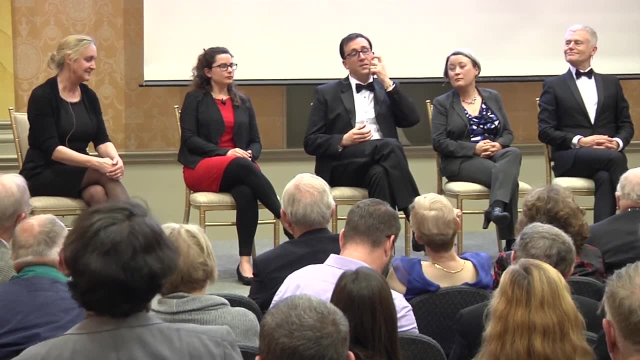 something like the rotation rate of the planet based on that surface survey. but could you detect a large moon or other characteristics that might contribute to the suitability? The answer is yes, although it's going to be easier to do it at some wavelengths than others. Actually, if you look at the wavelengths at which carbon dioxide absorbs or water absorbs, which our atmosphere is full of, the Earth can become quite dark and the moon, because it doesn't have an atmosphere, retains its brightness In the Earth-moon system- the moon, I think. 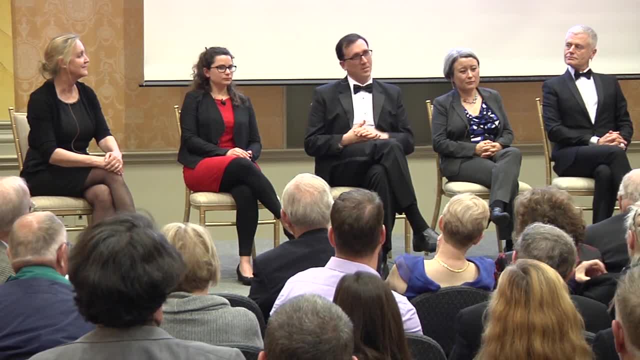 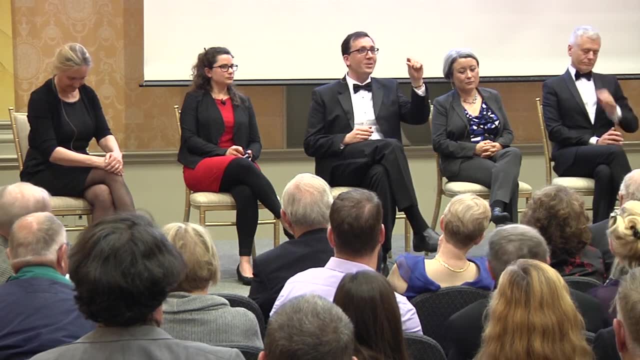 is about 10 to 20% of the total brightness of the Earth-moon system, So the pixel would get very dim at those wavelengths that water and carbon dioxide have deep absorption features And at that point you would actually be able to be getting, essentially, a spectrum of the moon. 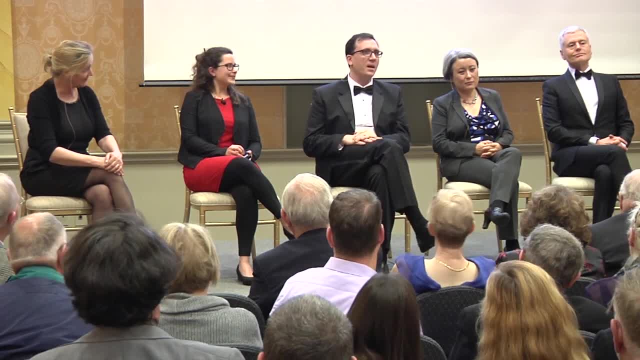 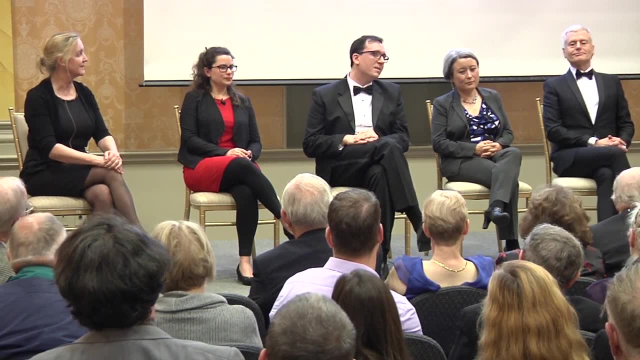 around that planet. If you're interested in this, there's work by Ty Robinson and colleagues that came out a few years ago. So again, looking at the time-resolve thing and looking at the right wavelengths, you could probably tease that out of the data. 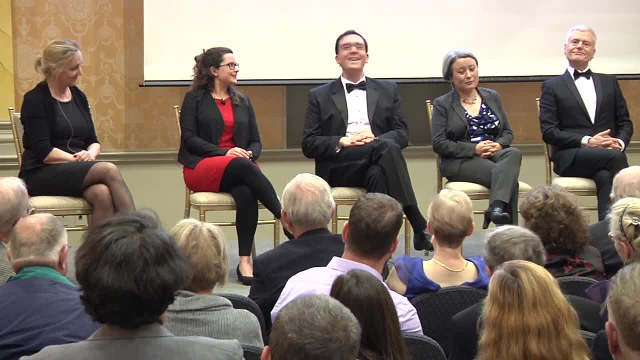 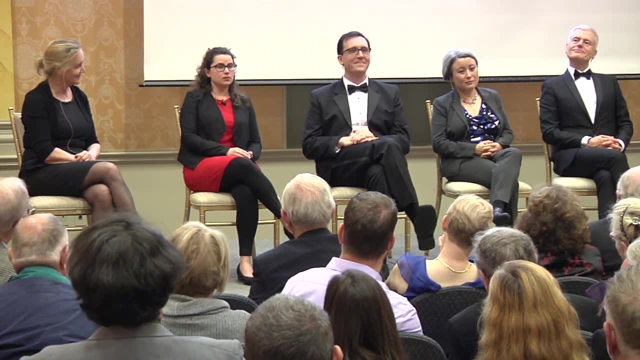 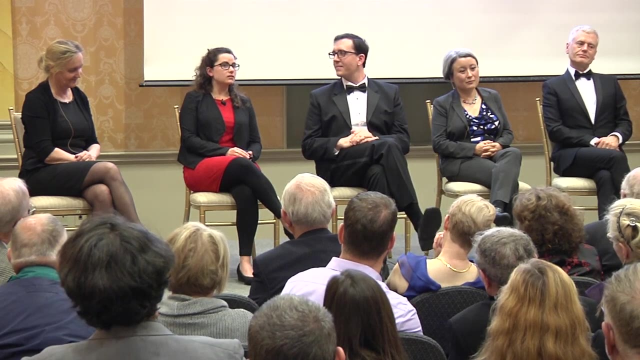 The problem is, of course, the moon is airless. That's great. If you've got anything else, then we're very much based in that simulation situation on what we know here. Anything else will result in different patterns that you would see. amplification of signals. 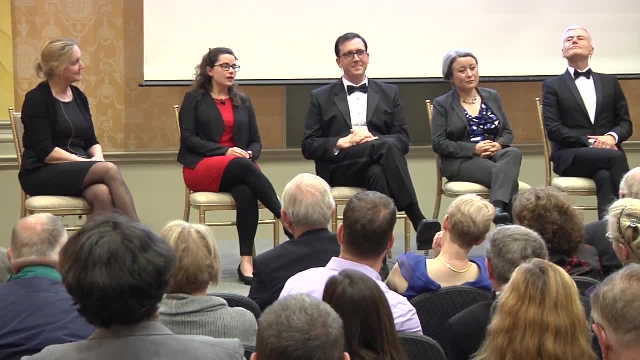 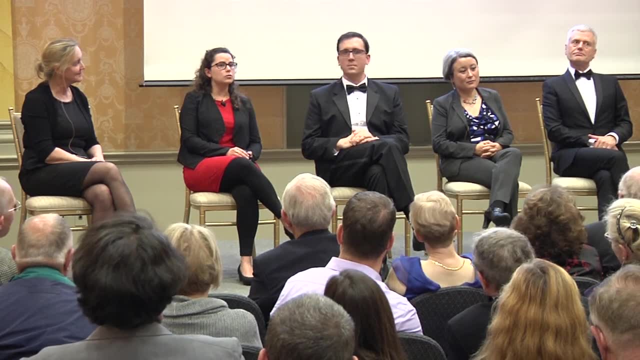 at different wavelengths based on separate atmospheres, And that's certainly an area that people are exploring, because it's really an interesting concept of whether or not we can discover and analyze moons around planets, including moons around giant planets as we have around our giant planets. in our solar system. So it's a tough question, but it's not without possibility. Actually, I guess I would make one more comment too. I think the problem is maybe, perhaps a bit backwards. I think we'll need to find the habitable planets. characterize them, see if they have liquid water, and then see if it matters whether they have a moon or not, because the importance or influence of the moon on our planet is a data point of one and it's all a bunch of theory anyway, But now it's a testable hypothesis. 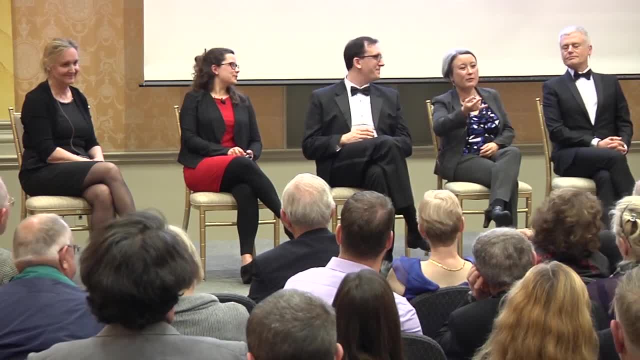 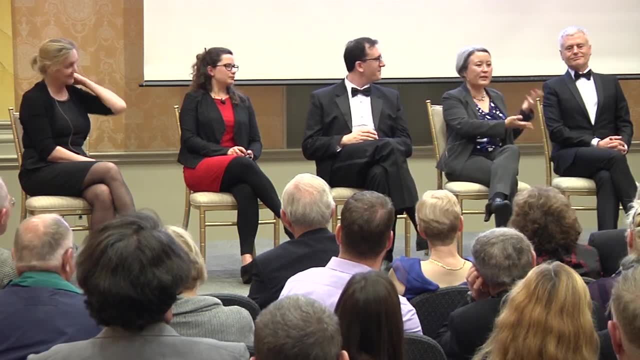 We want to make it a testable hypothesis. It's a testable hypothesis, but I think it's the other way around: Find the habitable conditions first and then figure out well, what are the factors that affect whether this planet is habitable. 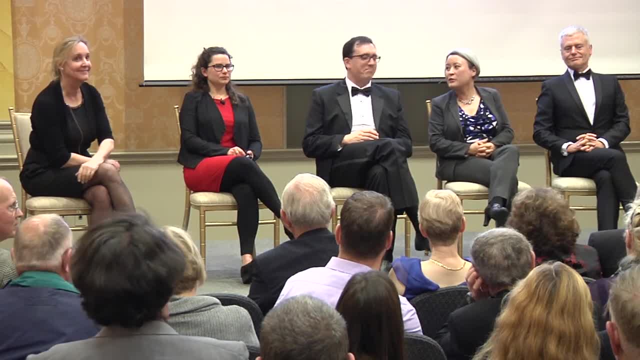 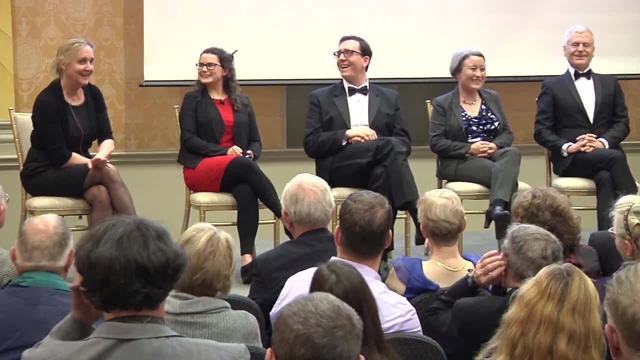 or not, that one or something Moons may be a factor, but I doubt it's the most important one. Yeah, I think exoplanets has been astonishing. Theory has been wrong almost all the time And it's really the empirical evidence. 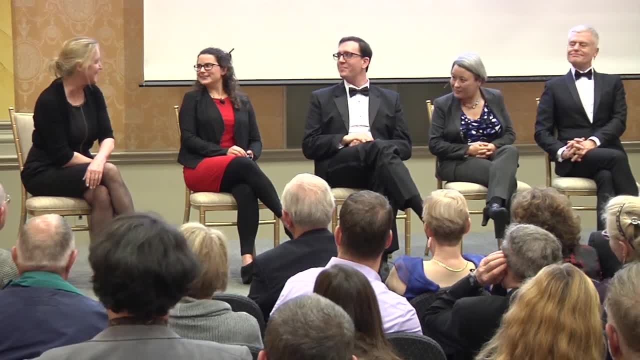 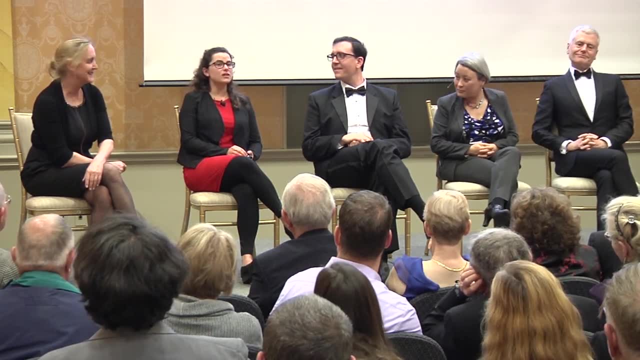 that just has left us saying what, How can that be? Yeah, it's not even just scientific theory, It's: our imaginations aren't as good as nature's imagination, They're just not. Science fiction did not project the presence of giant Jupiter-sized. worlds so close to their star, 20 times closer than we are to the sun. Yeah, even sci-fi didn't. Sci-fi couldn't work it out. Our imaginations aren't as good as nature, and we're going to be finding out. 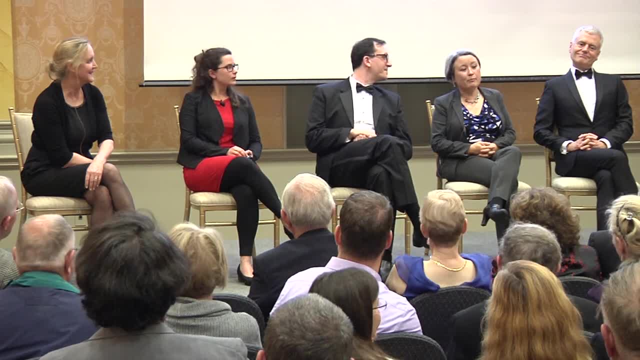 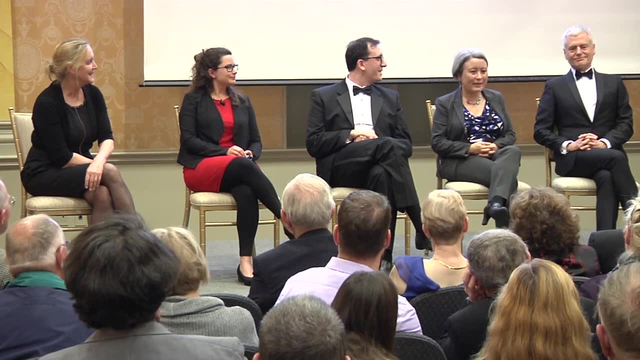 exactly how far that goes over the next couple of decades. Yeah, and I mean my personal research is in planet formation. Off the top of my head, I can think of four different ways to prove from theory that planets cannot form Right. 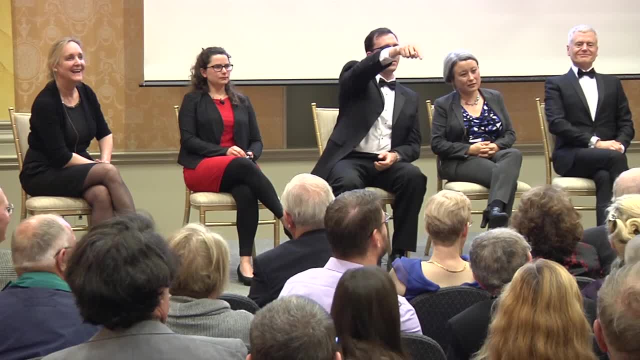 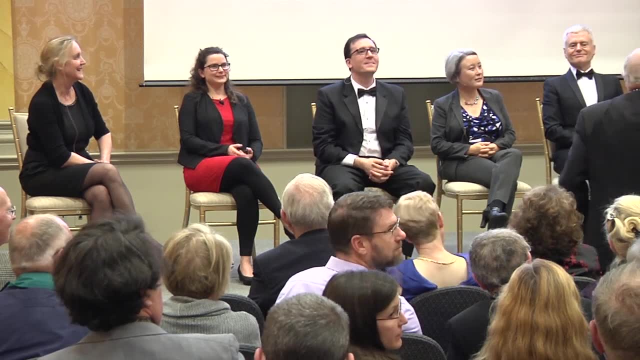 There are three microphones. If you have a microphone in your hand, you hold it up, so I know where they are. Okay, Carl, you have the next question. And then you have the next question And if you have a question, 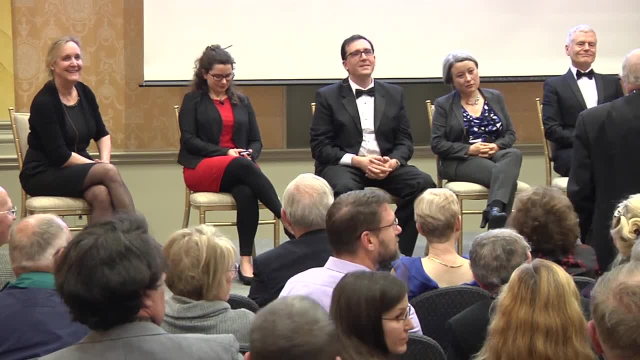 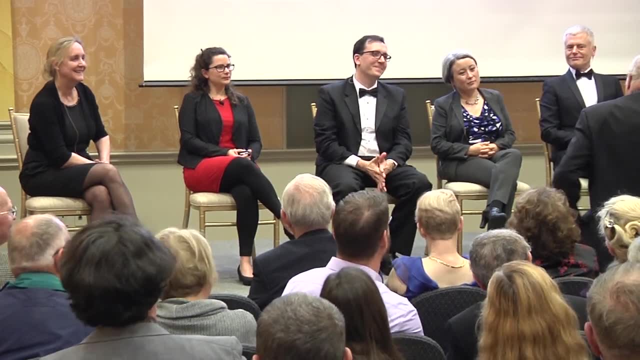 you hold your hand up long enough for the other guy with the microphone to find you. Yes, there's a question there, Okay. Okay, Carl Merrill, I'm a member of the Society. Could you clarify what you think would be a real signal of life? 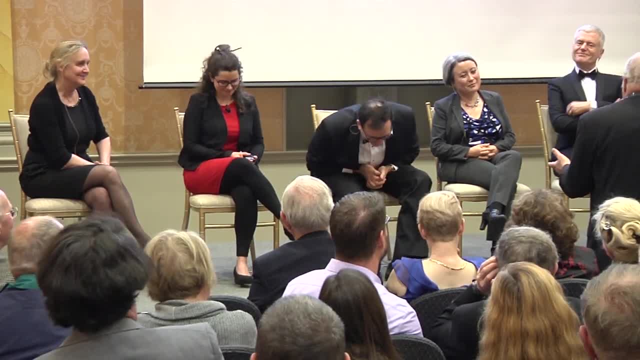 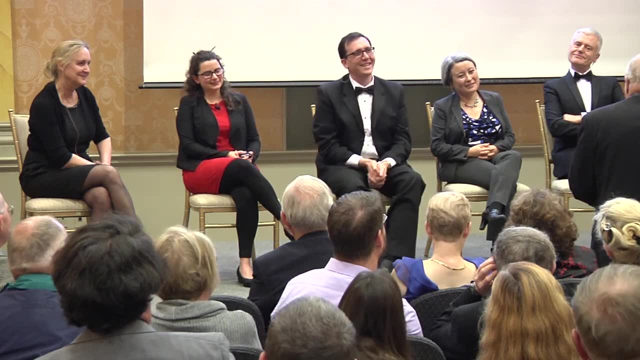 Because, on one hand, I thought oxygen was a signal. On the other hand, you said: well, oxygen could be formed without any life. On the other hand, we know on this planet there was life before there was oxygen, before the cyanobacter started. 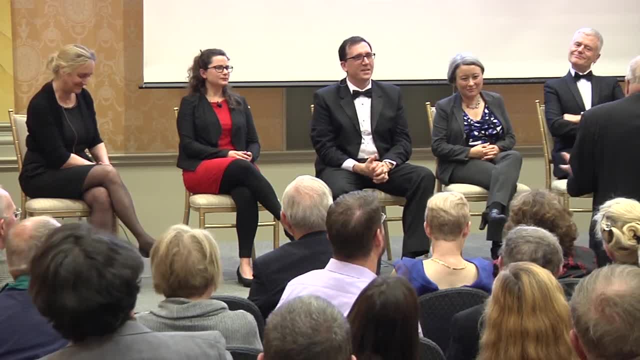 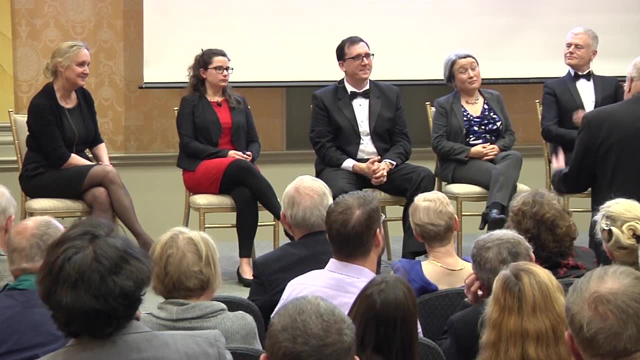 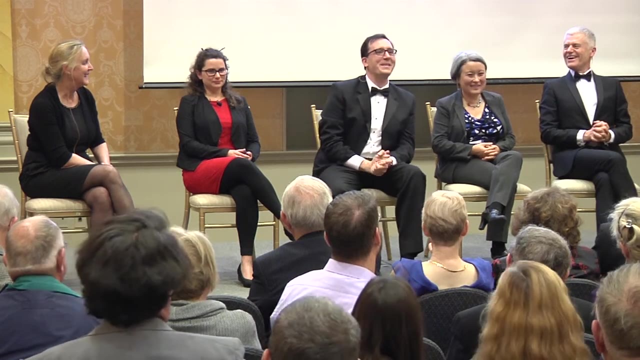 making all this extra oxygen? I'm not really sure. And then the other question along the same lines is: could we get a signal from complex organic molecules? when we're doing the spectrum, Always soft volumes. So apologies for muddying that one up a bit. Both in the literature and in this talk, actually. So let me give the specific answer and then the general one. For modern-day Earth, the best biosignature is still oxygen and methane together in the presence of liquid water. I think myself as a scientist. that's the point at which. 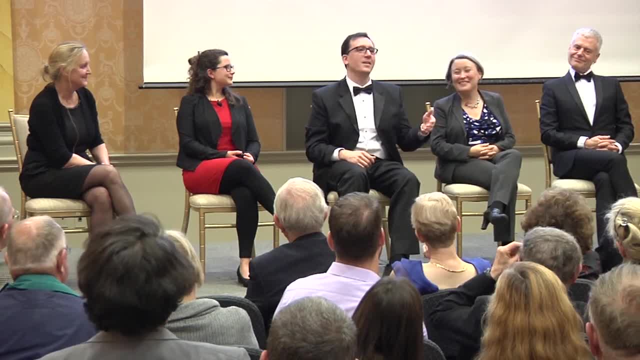 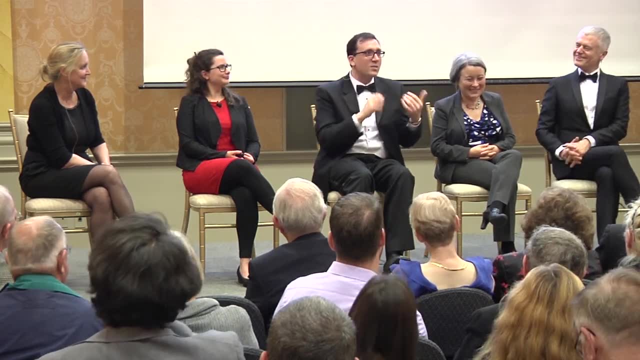 I'm willing to call the president, call the press conference, write the paper and go forward. You know, if the rest of the scientific community disagrees at that point, that's on them, That's between me and them. But that's when I'm willing to put my name on the paper. 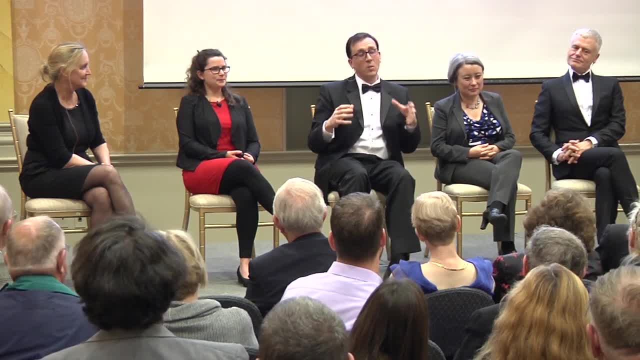 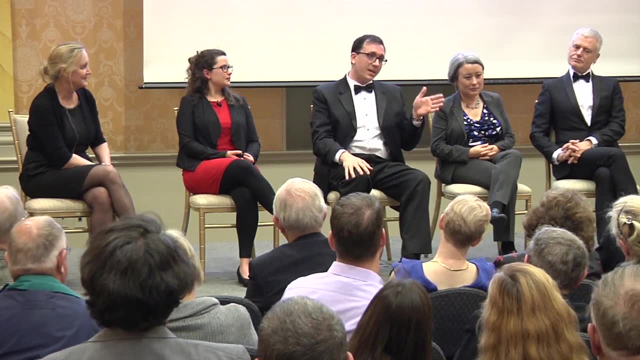 that says, yeah, we found evidence of life elsewhere More generally, and we're working. actually, there's going to be papers coming out next week that suggest that we actually turn to a more quantitative approach using Bayes' theorem, And to do that you need the prior. 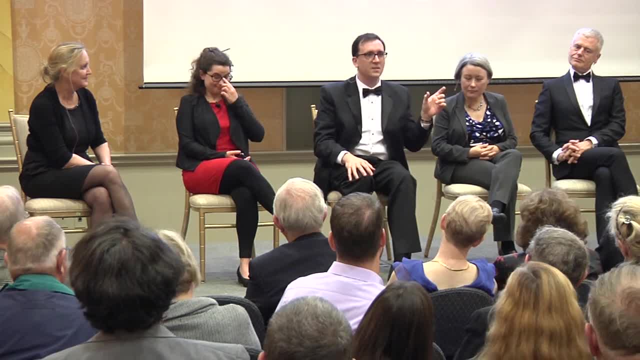 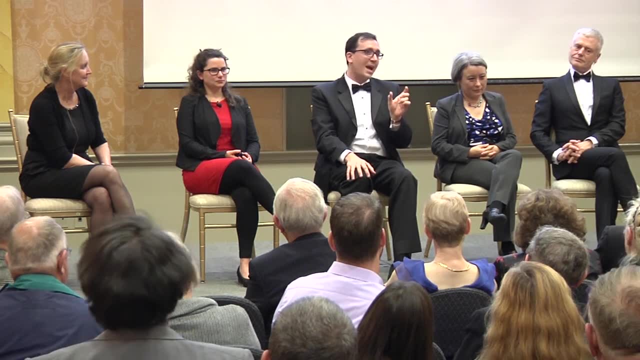 which is the whole point of doing the mission in the first place. But you also have essentially, the ratio of the probability the data arise that you see from a living planet versus one that is habitable but not alive, And to get that ratio we actually have to build. 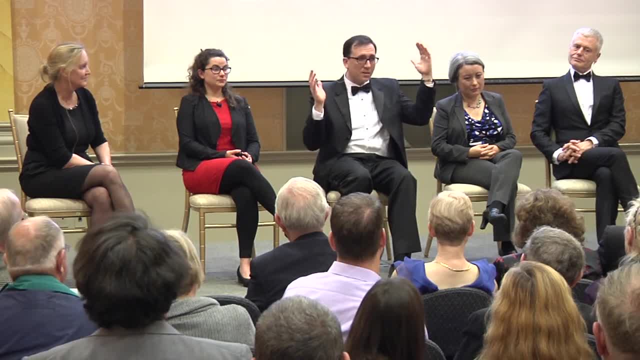 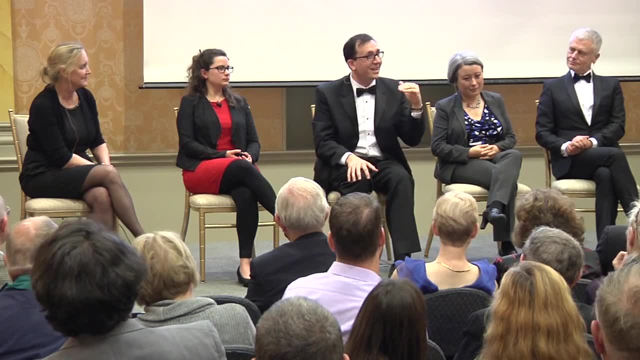 really good models of planets that are alive, Like we have those. actually, Our GCMs are great models of planets that are alive. We also need to develop really good models of planets that could be alive but are not, And that's actually. 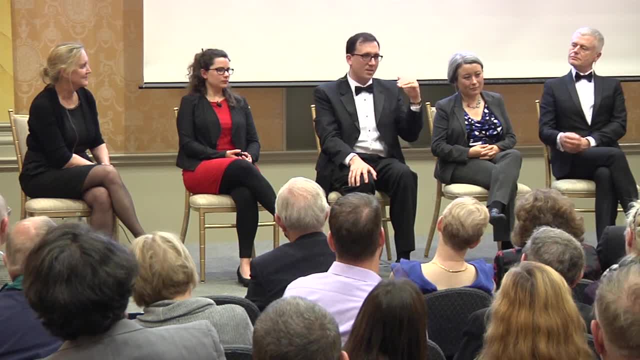 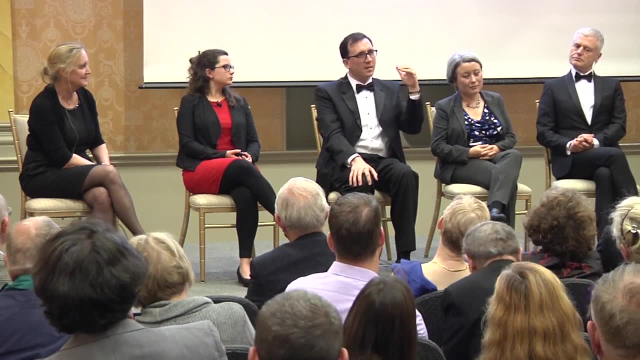 I think we're actually behind on that one. That one's actually more difficult to do because life is so intertwined with the one planet that we know that has the conditions for life. That'll allow us more quantitative assessment. I think there's other things I could say. 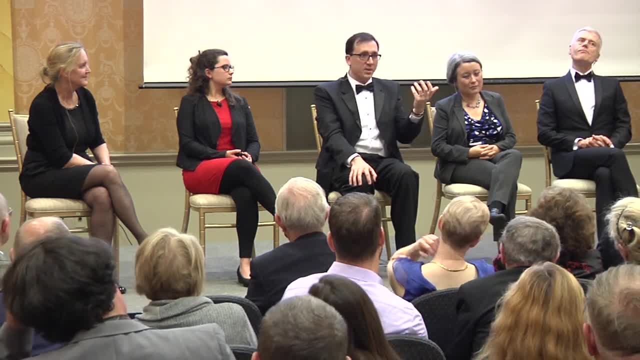 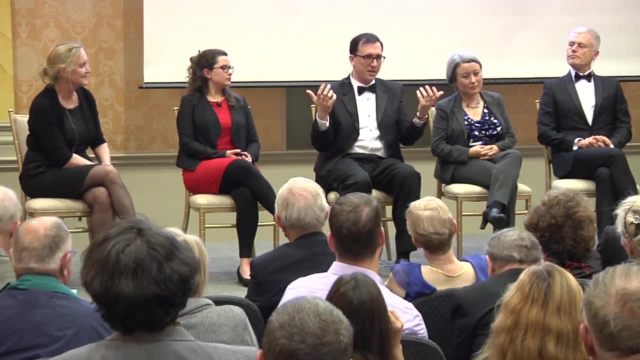 in general terms, like you know, you want to look for a motivation for life to be doing something, some sort of metabolism to get energy from and then detect the byproduct of that metabolism. Those are the kinds of things that would be very, very strong. 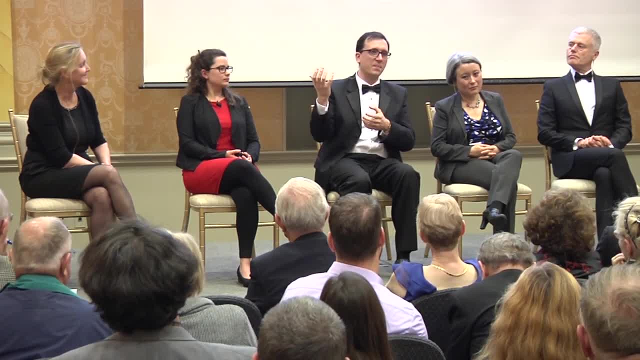 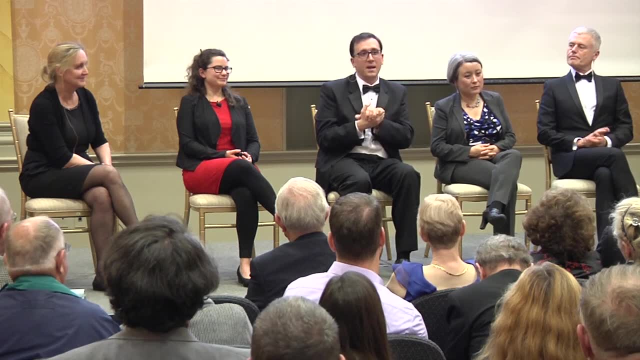 indicators of life, And that thing that it's producing can't be produced abiotically at a fast enough rate to accumulate to a detectable amount. So but we want, we need to be more quantitative And I think over the next five to ten years. 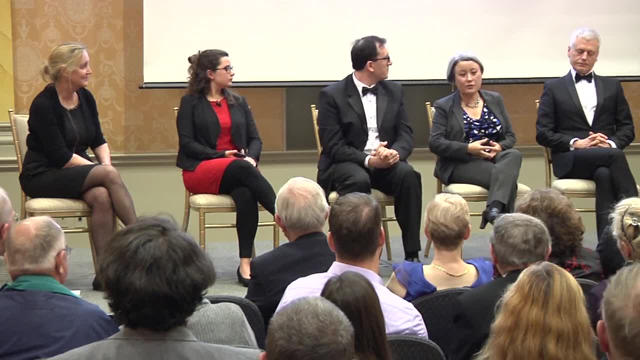 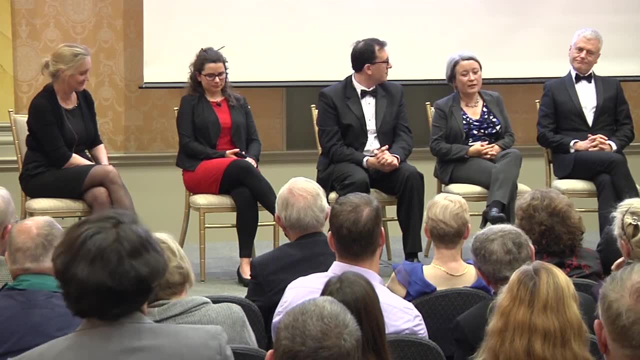 we'll get there. Yeah, I think in the you know ten, fifteen years ago it was kind of put rather as a simple observational problem: Detect oxygen, you're good. Then it got okay. well, alright, you need to detect. 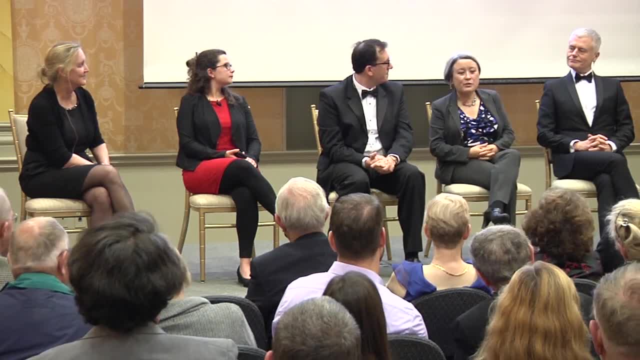 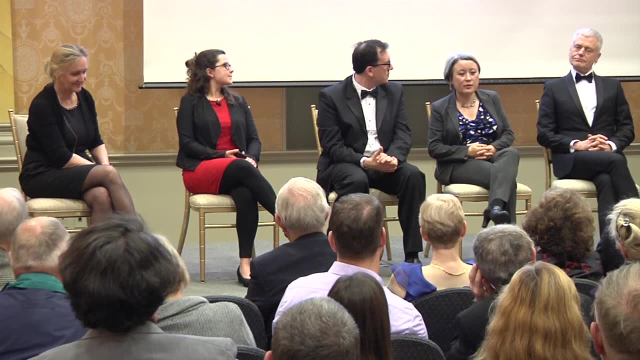 oxygen and methane. But now I think the real answer is: you need to measure. you need to try to measure all the abundances of all the primary constituents of the atmosphere and figure out what all the sources and think rates are, And only when you see something that 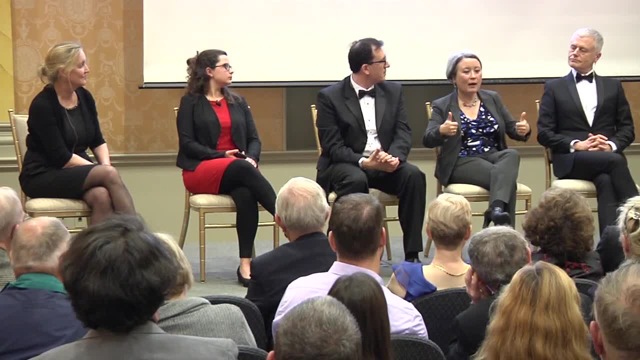 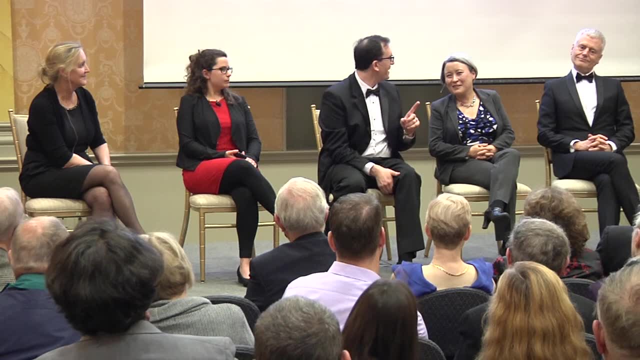 doesn't. that is anomalous. that's not physics or chemistry, biology, Although you. it's important to have the motivating thing, Because I don't believe in a life between the gaps method of finding life Right. There needs to be that. you know This isn't totally settled yet. 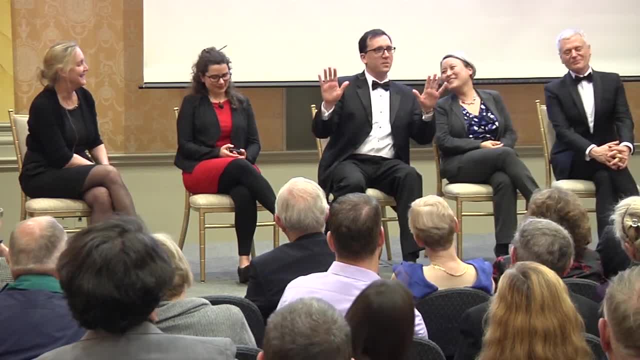 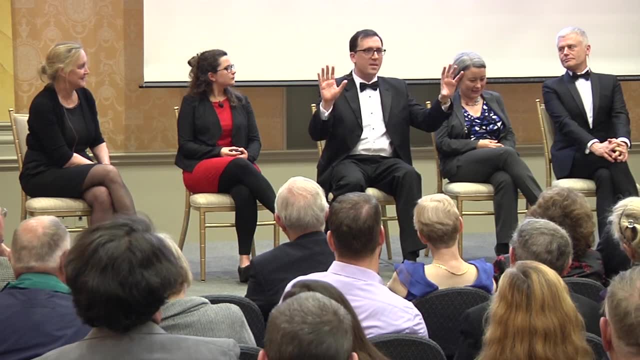 Absent. I mean to me, if you didn't know, the biosignature was there and you said: life is on this planet, what would it be doing? You should predict the thing that you, that life, would be making, the thing you think is the biosignature. 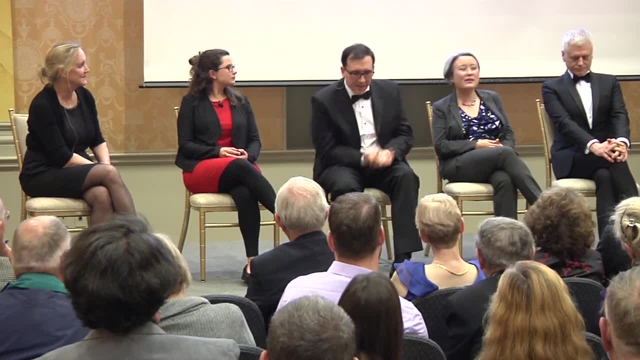 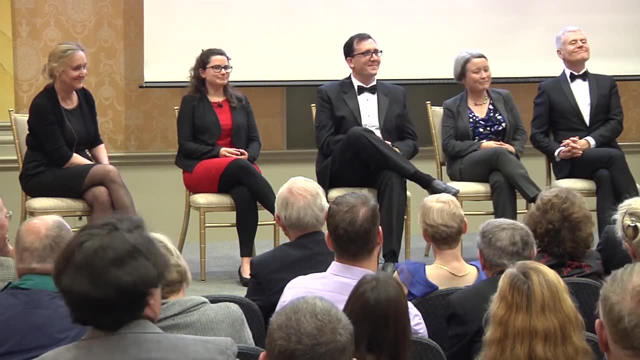 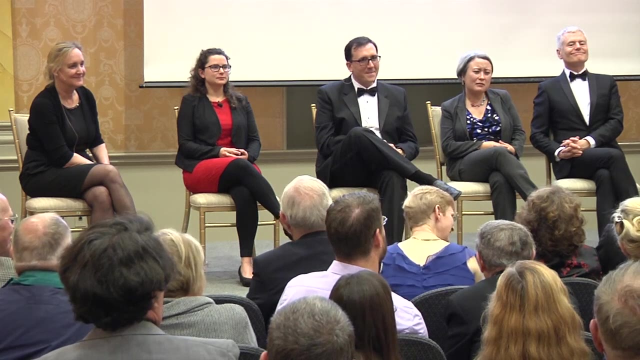 Right, If you have a planet, Okay, identify a food and a waste product. Yes, Predict the waste product that you're identifying. This isn't. we haven't completely figured all of this out yet. That makes sense, though. Complex organics. 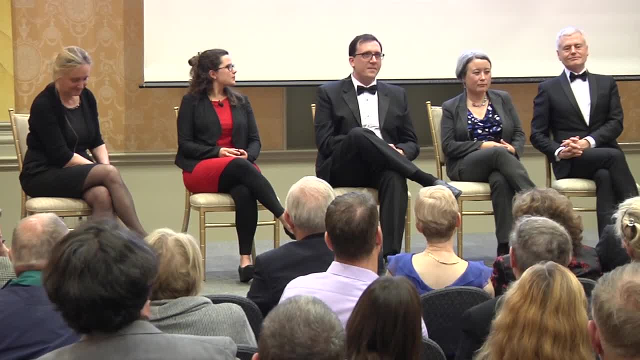 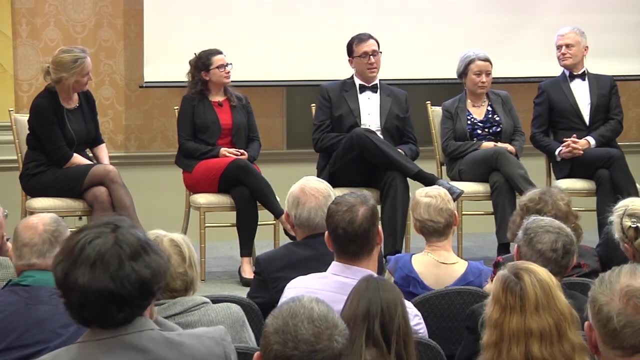 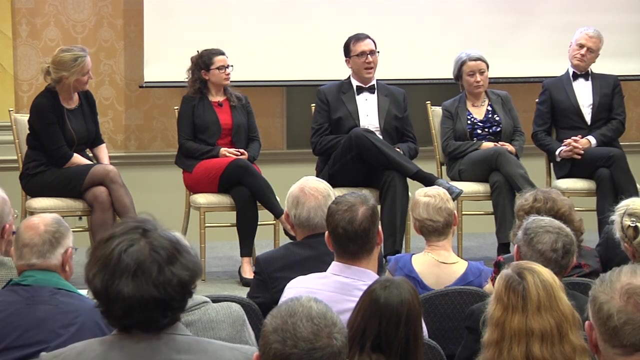 So there's a paper we have in review right now that suggests that the hazes that Hannah wants to look at, that some of them that we think existed or are present on ancient Earth in certain atmosphere contexts can only occur if there's biology making a lot of methane. 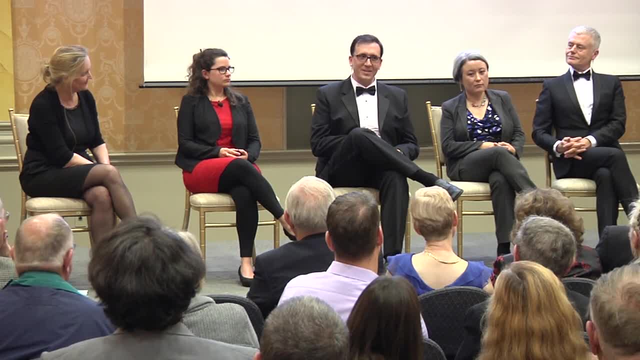 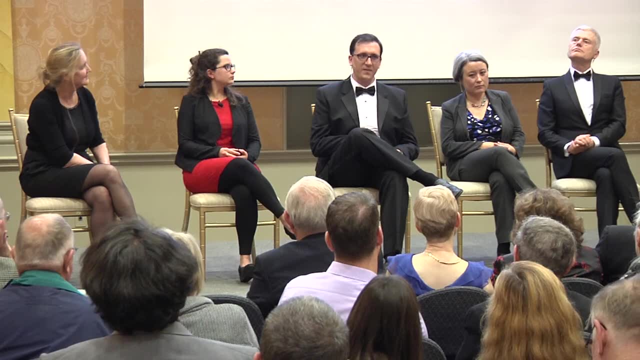 Now the problem with that is there's plenty of non-biological ways to make methane, And the biosignature might be- and this is a might, because this one- we haven't thought about the false positives yet- is when biology makes methane, it also releases. 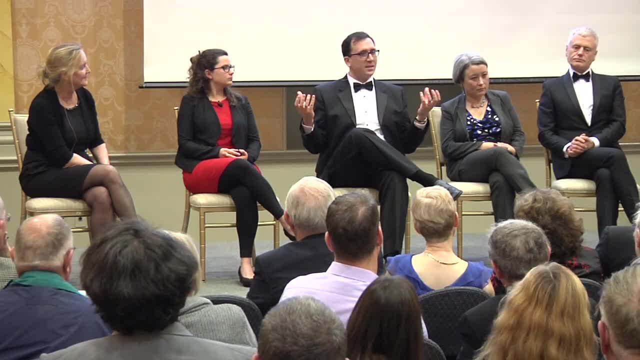 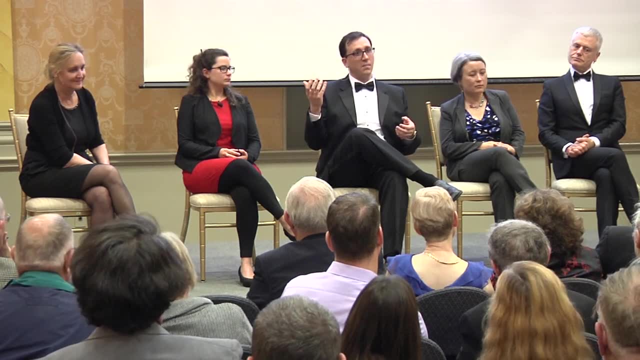 a bunch of other organic compounds, And those organic compounds are more easily split apart by photolysis in the atmosphere and by kinetic reactions in general. that is going to facilitate haze formation much more readily than methane. that's coming from non-biological sources, And so if you've got the 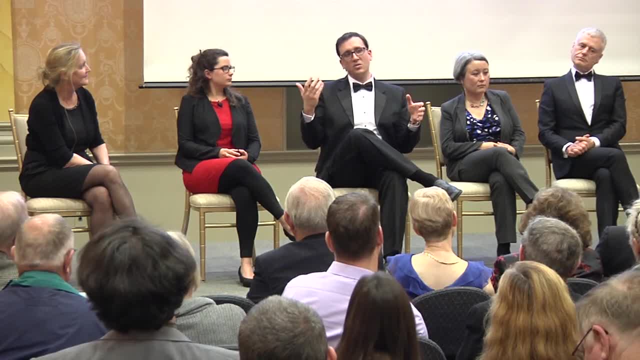 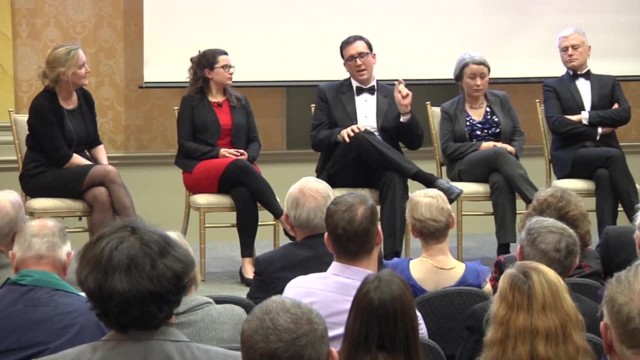 haze and you can get that atmosphere context to know how fast the haze could be produced with just a biological methane production. you might be able to say something, But the individual complex organic molecules are probably not going to accumulate to a high enough concentration to detect. We'd only see them in mass. 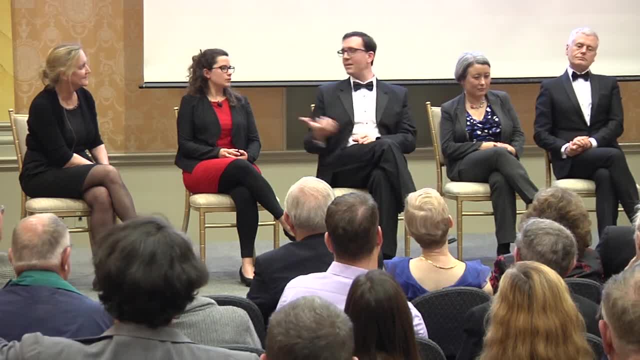 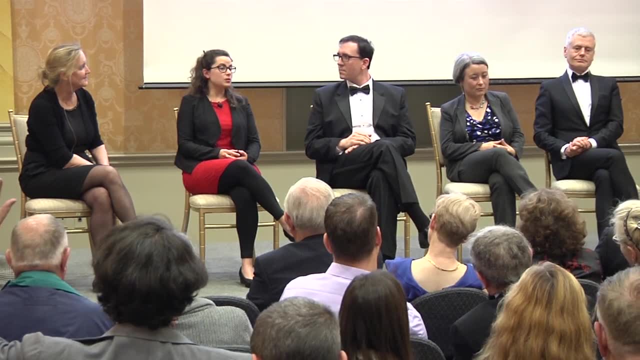 if they're making these large spherical droplets that form hazes that even Hannah's detecting on the gas giants And you know, if you do detect those kinds of things, it tells you a little bit about their dynamics, but it's not a. 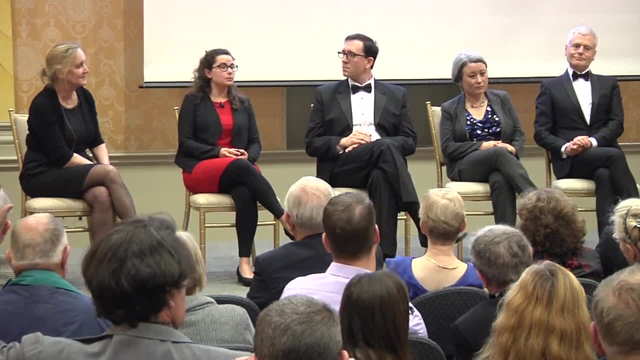 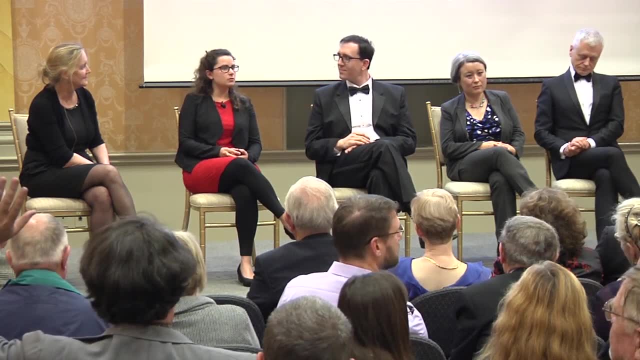 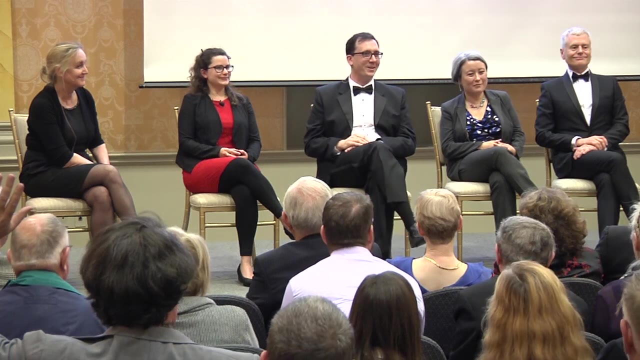 you can't get much more about that planetary atmosphere beyond. something has to be lifting it up and sustaining it at that altitude. So it gives you some things, but it really hinders a lot of other investigations. Have a Europa or Martian scientist come and ask that question again. you'll get a good answer. 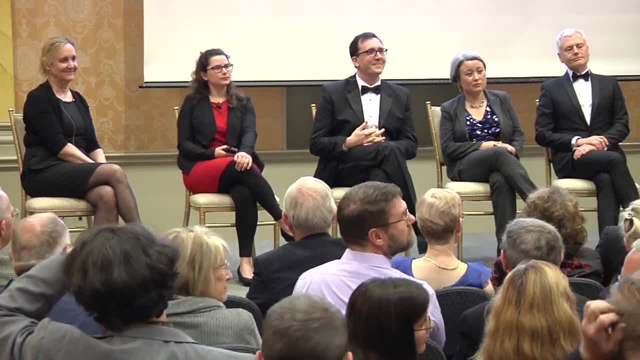 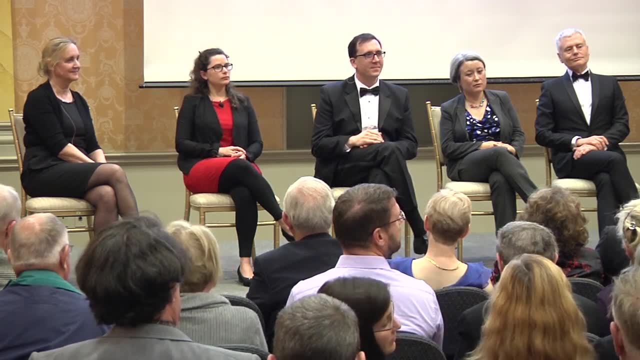 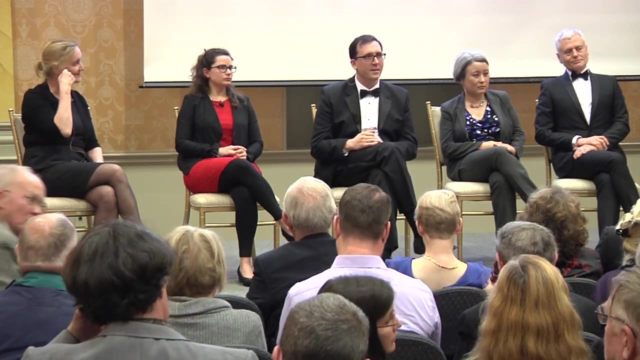 Isaac Shomer. I'm a member and my question is about: in the third lecture there was something about hydrogen in the atmosphere that was being blown away or lost, basically, and I'm wondering if some of that hydrogen could be regenerated by protons coming in from the stellar wind. 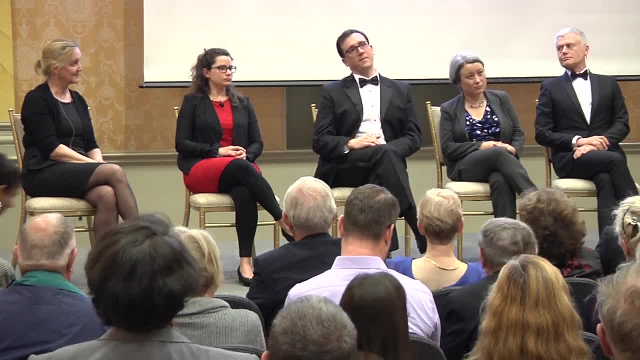 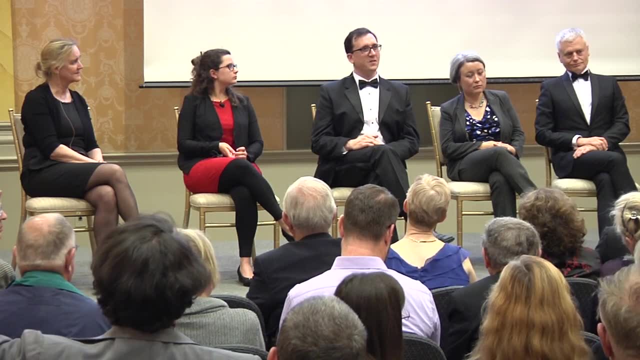 Yes, and it could also be regenerated from volcanoes at the surface of the planet. We're a bit paranoid about these false positives because we don't want to do the thing I started off talking about spending our whole lives on these careers, not to mention a considerable amount of taxpayer dollars, only to have the wrong search strategy. So we're being paranoid and we're trying to invent concoct planets that'll make the gases we think are biosignatures. So you're right, You would need to not be accumulating hydrogen from. that stellar wind. You also would need to not have volcanoes putting hydrogen into the atmosphere, like volcanoes on Earth tend to do. So you kind of need the just right planet, But I also don't want to rely on the just right planet, not. 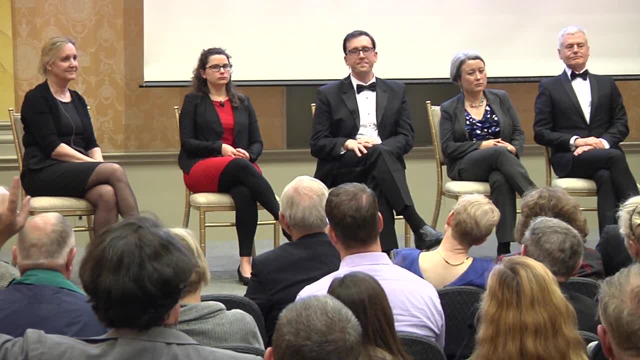 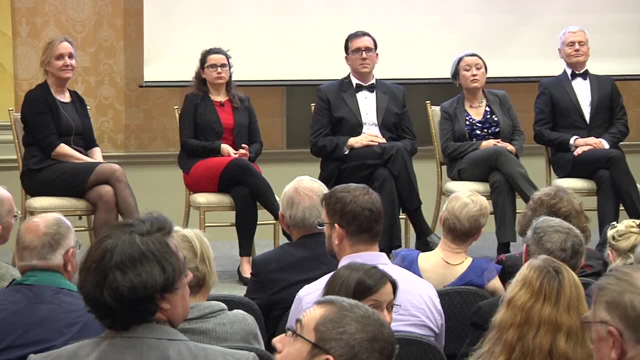 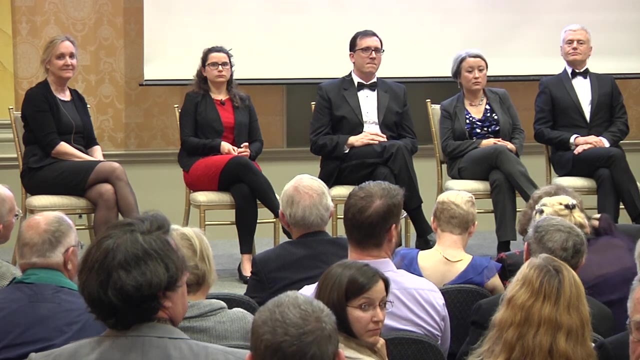 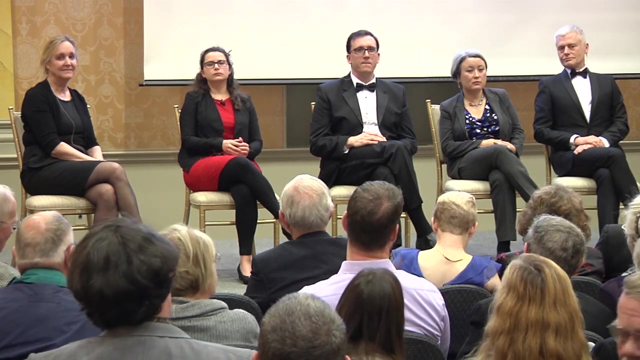 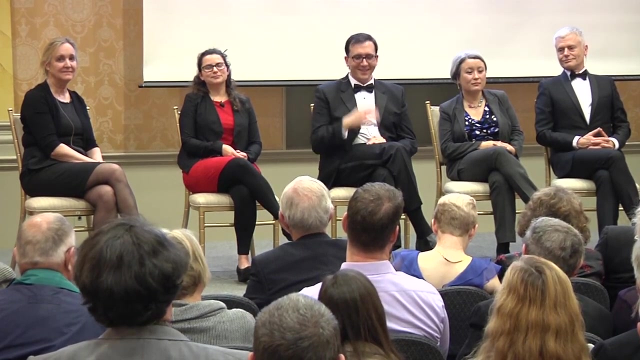 existing before we go forward with a mission like this. Yeah, Bob Abramson member. From the standpoint of looking for intelligent life that might inhabit some of these exoplanets, any thoughts on the collaborative use of radio frequency astronomy in ways that might either? 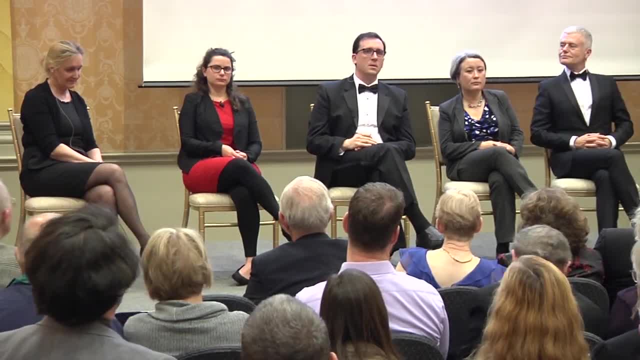 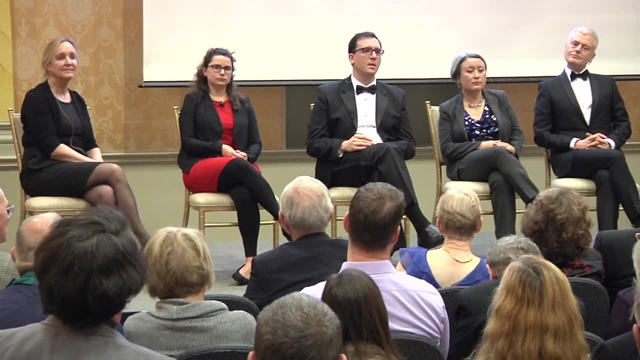 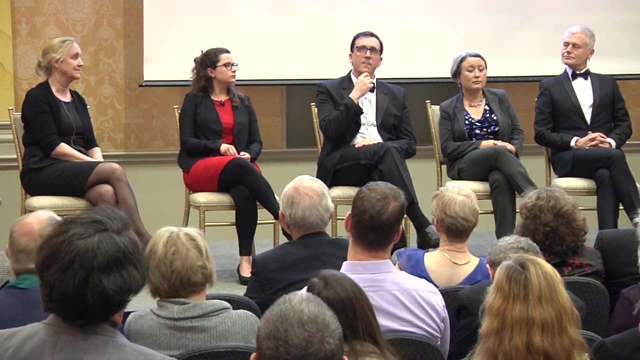 guide searches or, if we do hear signals that appear to be of potential interest, to try to correlate those against specific observations with web or other resources. So I think there's an interesting story here with there's a history of NASA of not funding much SETI work, But there is one. 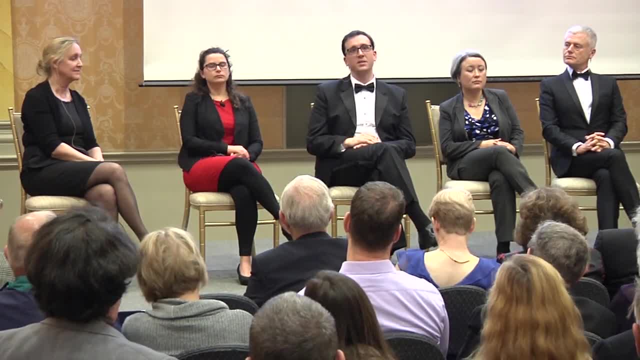 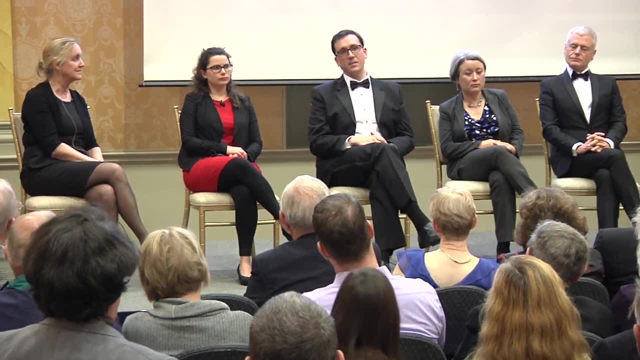 grant that NASA has out to fund a little bit of radio telescope observations, And that's for some of these Kepler worlds Which, as Dr Fisher mentioned, they're too far away for us to do the direct imaging spectroscopy that we'd like to do to look for. 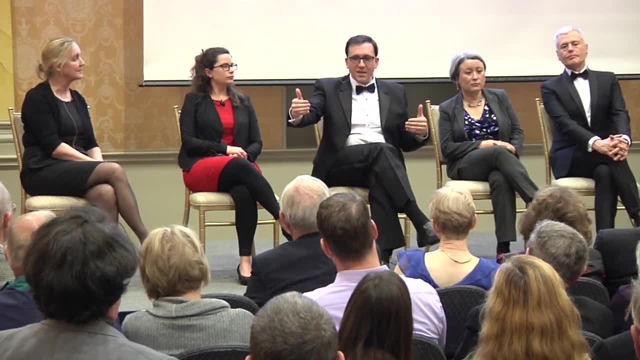 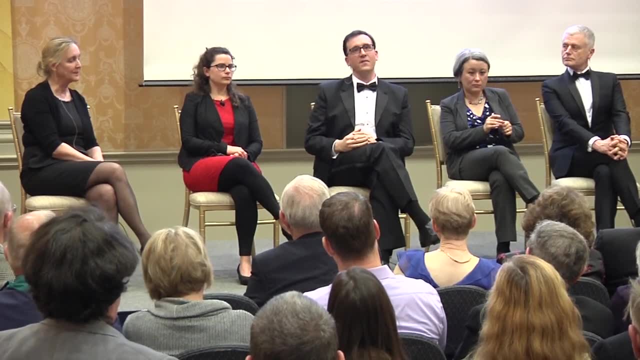 chemical biosignatures in the atmosphere. So the only next step you can take to test the hypothesis of whether or not they have life is to do a search for radio signals And so the one sort of small part of SETI that's NASA funded, to my understanding. 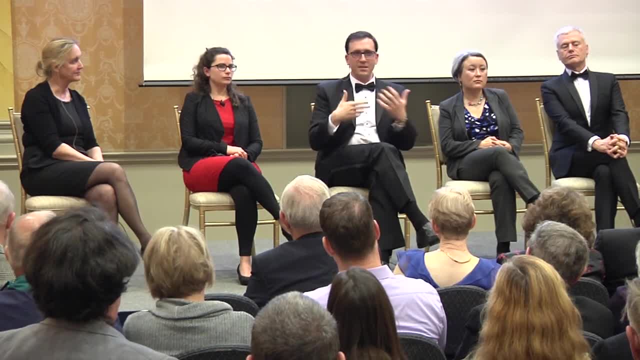 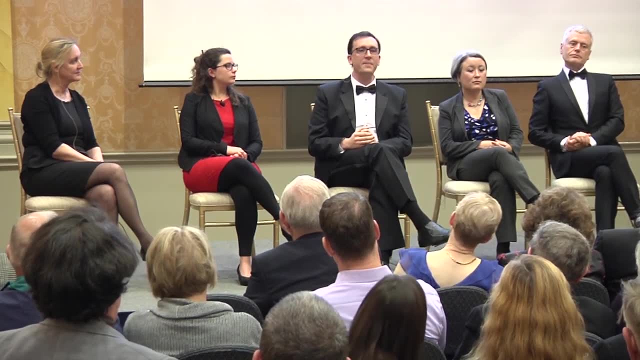 is to do just that with Green Bank, And I think if we found any of these worlds, then yeah, of course we'd be looking at what signals might be coming from them. I actually think that that's a better time to do it when you. 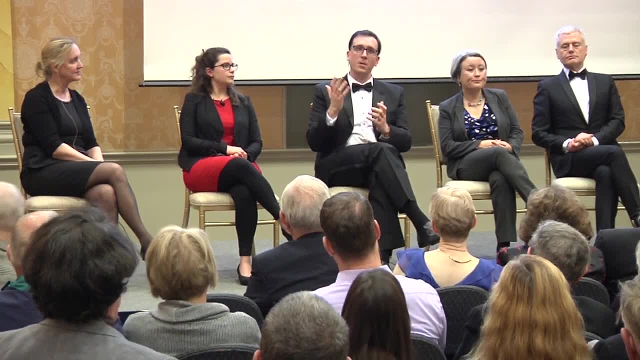 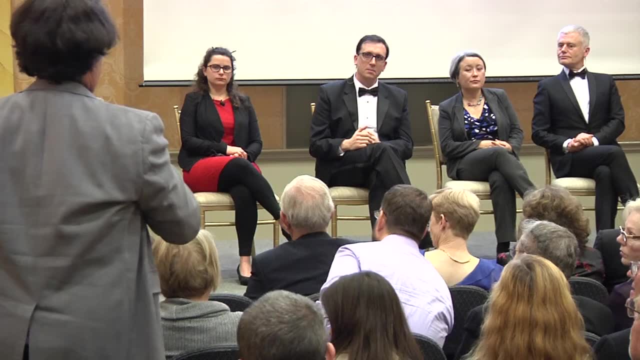 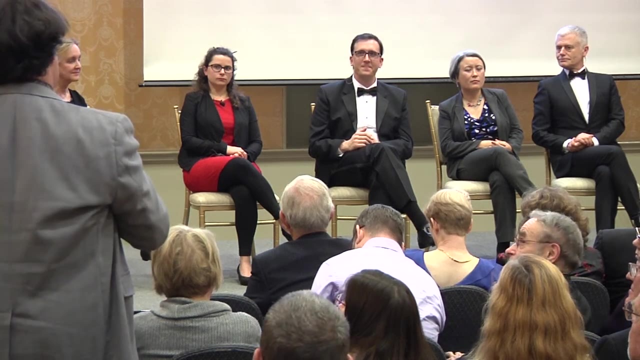 have a more directed hypothesis to be testing. That's just me personally. Marshall Eubanks, a guest, You said something interesting that caught my mind and I didn't quite understand it. You said, instead of looking for chemical disequilibrium, you should look for kinetic. 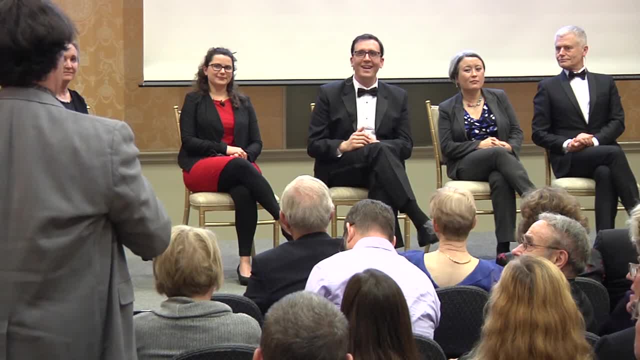 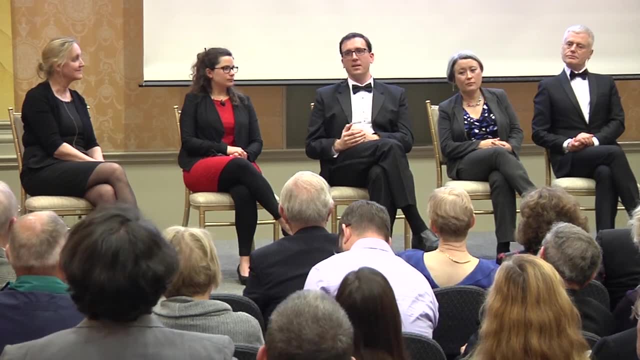 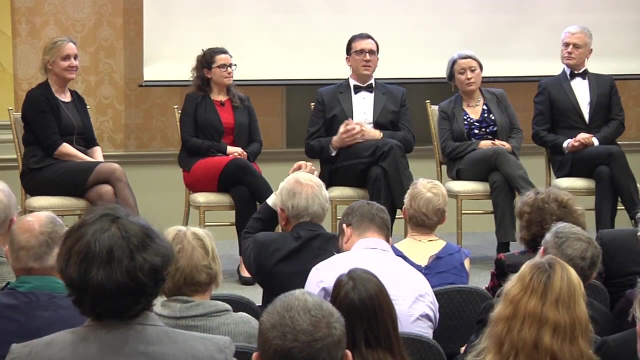 disequilibrium. I'm presuming you're not talking about bullets here, So what are you talking about? So what I mean by that is kinetic chemistry as opposed to thermodynamic chemistry, And the difference is thermodynamic chemistry is essentially the the it's the difference between. 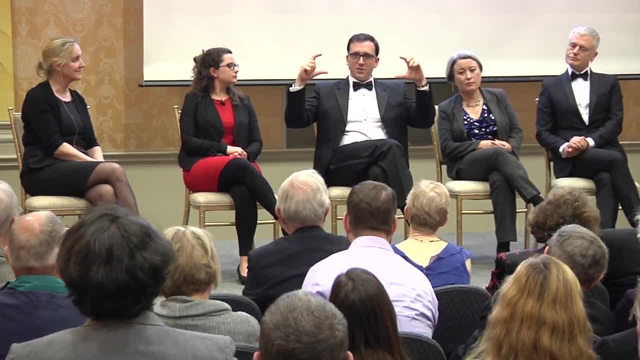 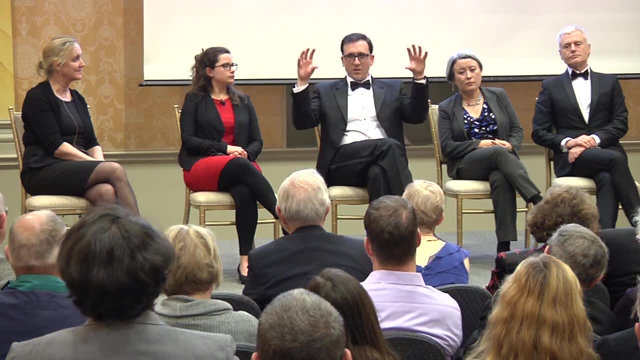 the energy that you could get from having those two molecules in the atmosphere together. Sort of you could make a measurement of how much energy you get from reacting them together, Two molecules that shouldn't be in the atmosphere at that temperature and pressure. That's the thermodynamic argument. I don't like, personally I don't like that argument because if there's something that biology could get energy from in the atmosphere, I don't think that's a good biosignature, because the biology should be getting that energy from that source. 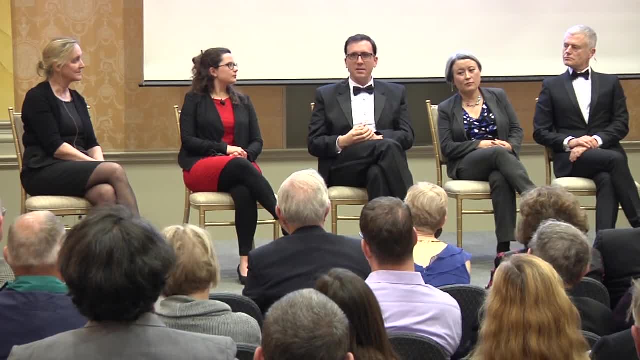 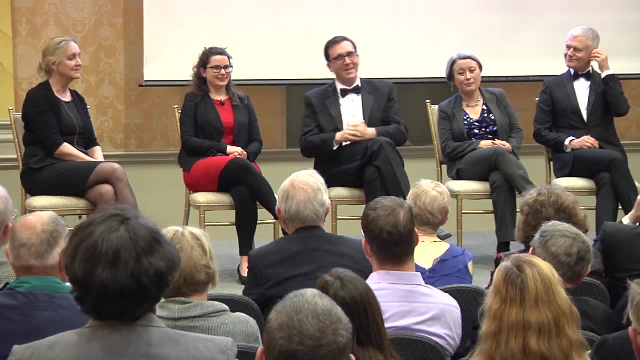 We actually just saw a work out on Enceladus along these lines, where they detected hydrogen, which is great because it's an energy source. but it's not great because it's an energy source, and why isn't it being used if there's life there? 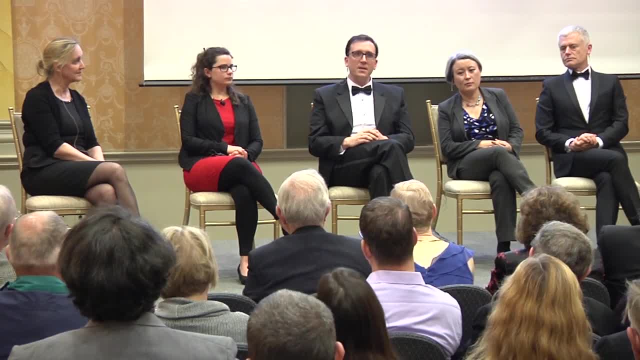 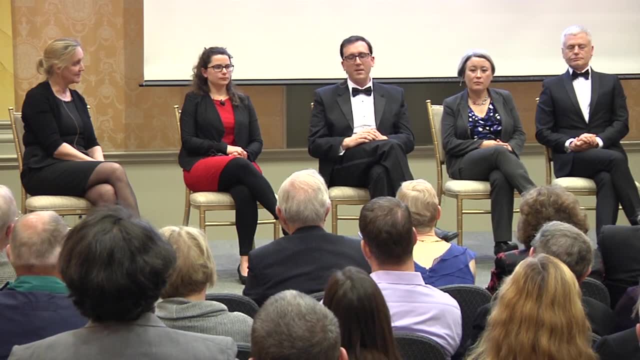 The kinetic one is more just about production and destruction rates. If it's being destroyed really, really, really, really fast, then it has to be replenished really, really, really, really fast. And if the replenishment rate is orders of magnitude greater than any of the 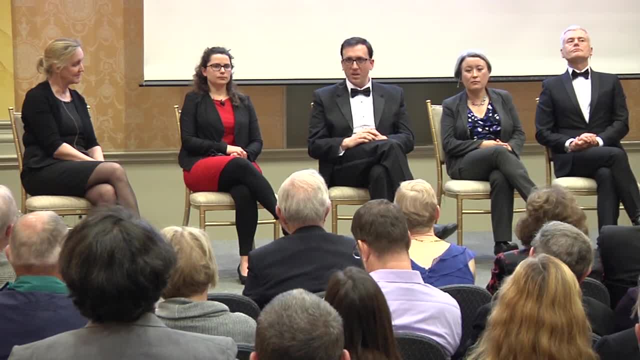 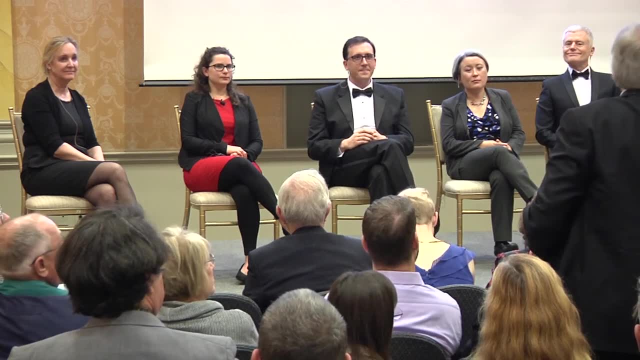 non-biological production rates, but consistent with what you would predict from biology. then you're on to something I think Right Practicing swallowing the mic. Frank Robert, a member, I don't envy you the task of distinguishing methylens on Titan. 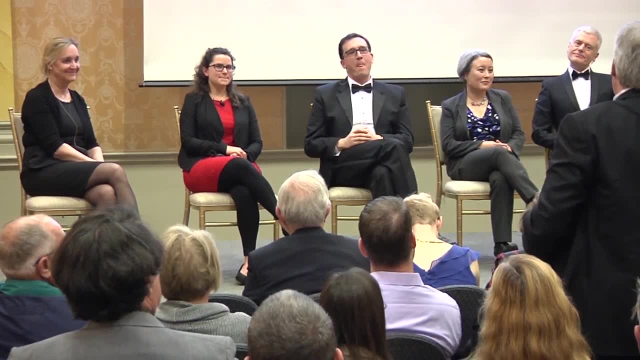 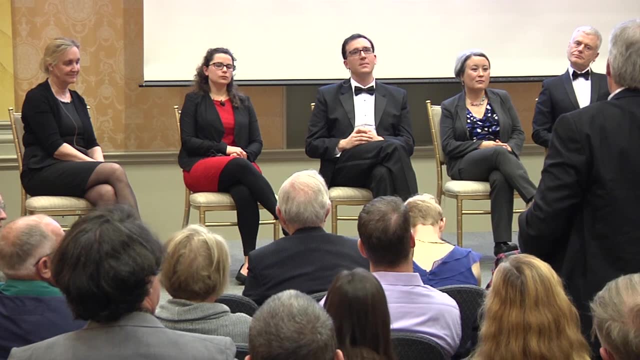 equivalent on an exoplanet from those of life, but probably an off-the-wall question. Would the use of a background star for occultation, thinking of the discovery of the rings of Uranus and so forth, be feasible at these distances, or is this complete pie in the sky that you could image? 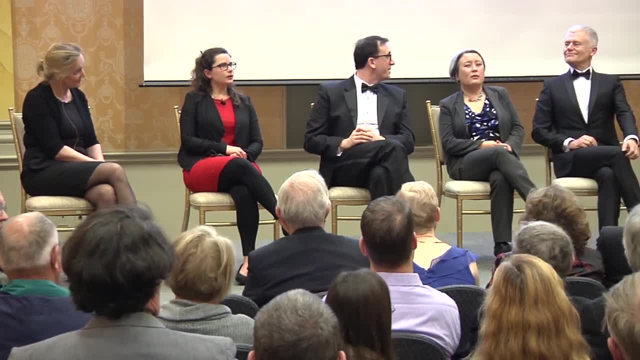 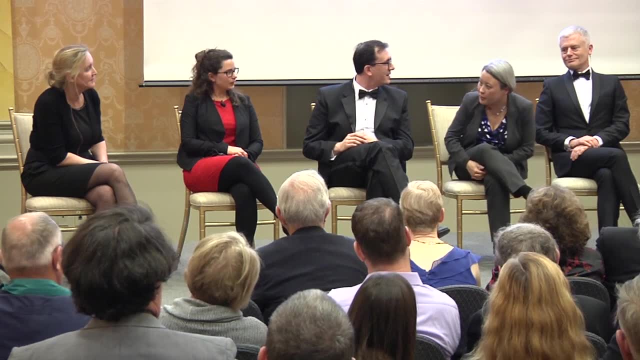 that way I'm going to punt. A background star, an occultation, a background star occulting a planet, not the host star. A background star, yeah Well, the problem with that is to know when that's going to happen. you have to. 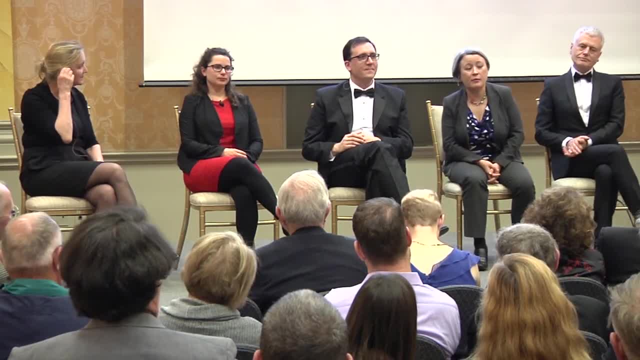 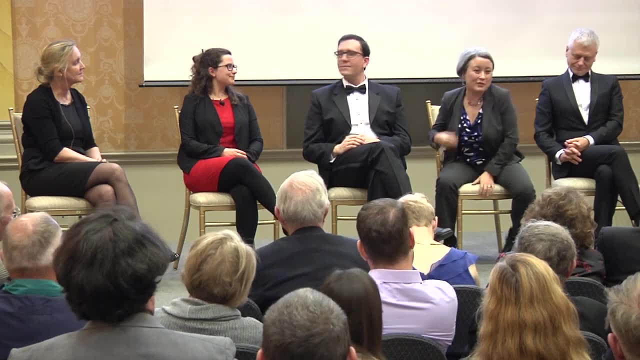 have the planet's orbit. So you have to find it first. You have to find it first. and, oh lord, I actually did some work in eclipse and occultation work when I was an undergrad, with Jim Elliot actually, and that is yeah. that is a major pain in the butt And you would have to know the planet's orbit to exquisite precision and the proper motion of the star itself, the host star itself. You'd have to know every orbital piece, of orbital information to like crazy. 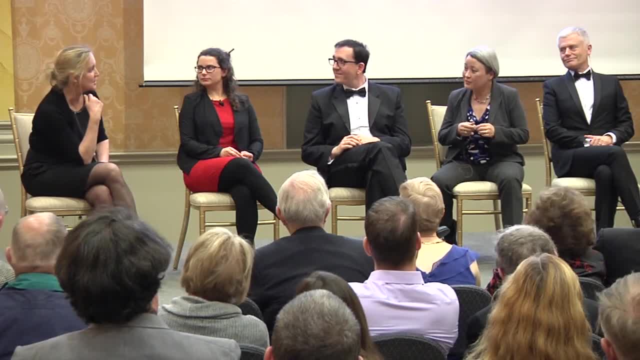 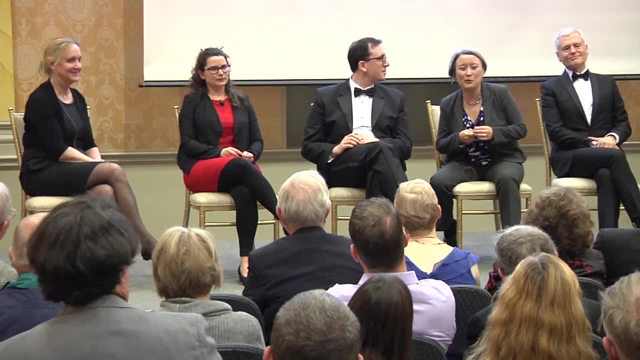 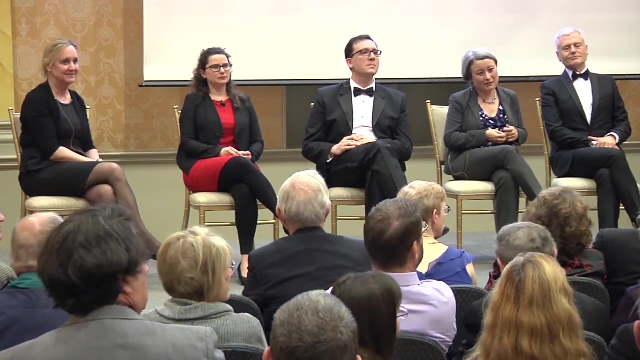 precision for that to even have a hope. I think for that one. It makes star shades sound easy. Yeah, Yeah, that's yeah. I think there are easier ways of doing this than that. Yes, again, my name. 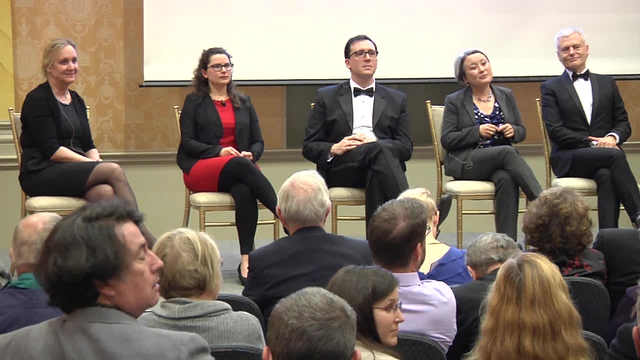 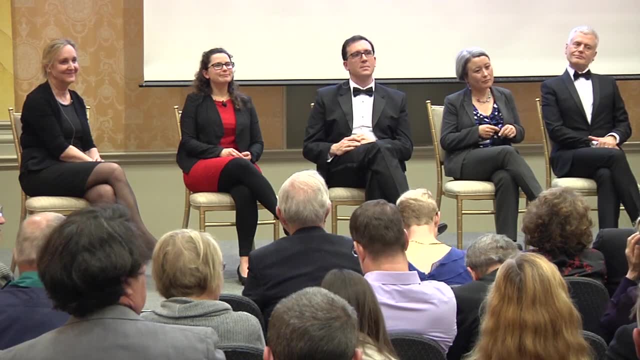 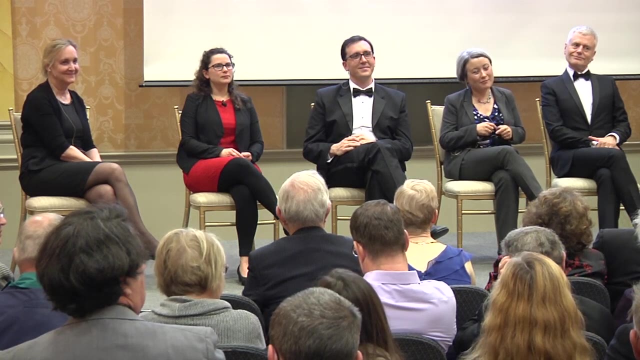 is Alon Lanier, I am not a member. Just each time they've discovered planets that could that excited the that caused excitement in the news, like the Trappist system and before that, the Proxima Centauri system. we got cold water because 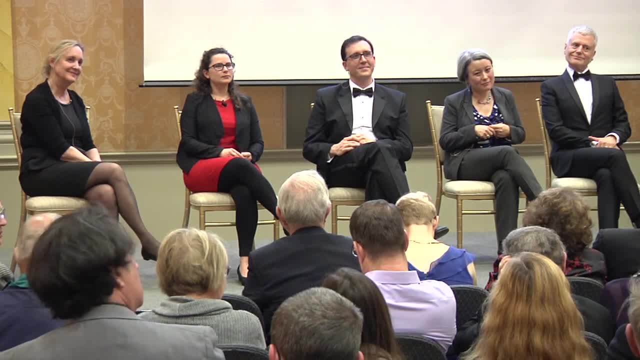 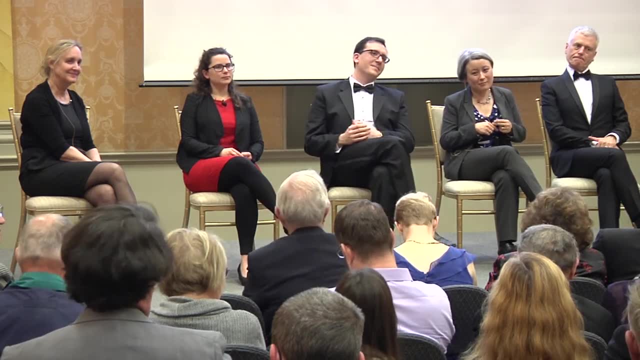 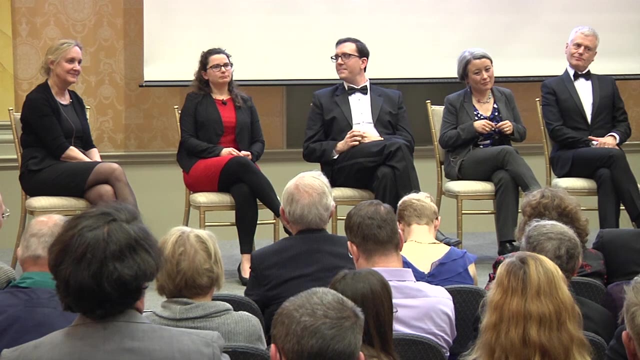 we're told that the M-dwarf stars are too active and cause solar winds that cook the atmosphere. You alluded to that today. Do we have any candidates out there left that their stars are not too active? that James Webb may be. that will fall. 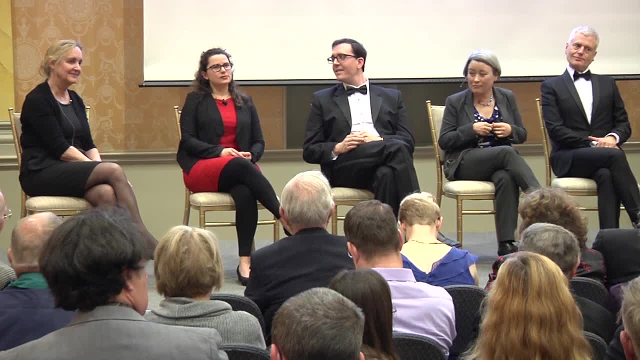 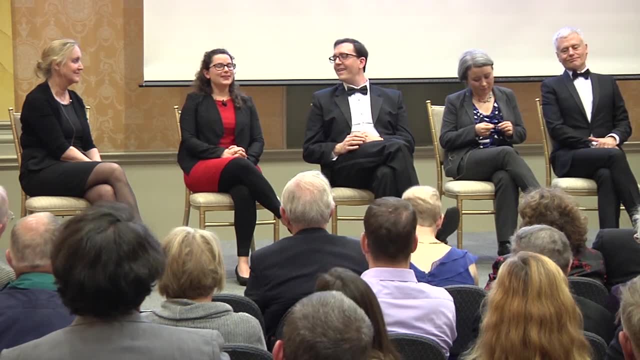 in within the range of James Webb. That's like if you'd have to guess which is the best candidate, what would your guess be? So the Trappist system is still by far the greatest candidate for these kinds of observations, certainly with the James Webb. Space Telescope Kepler has discovered a number of planets which are around larger stars. so the Trappist-1 star is much smaller than our Sun, so around larger stars that are in the habitable zone. younger stars rotate quicker and are more active, so that's an issue. 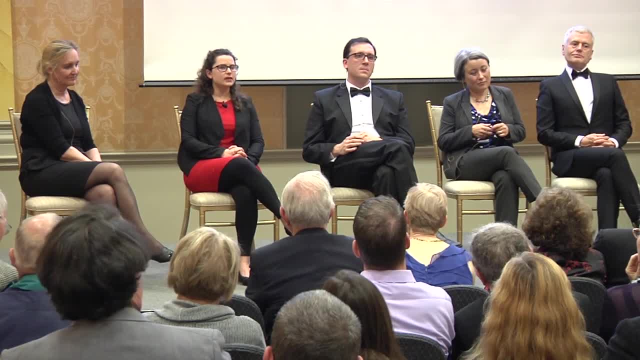 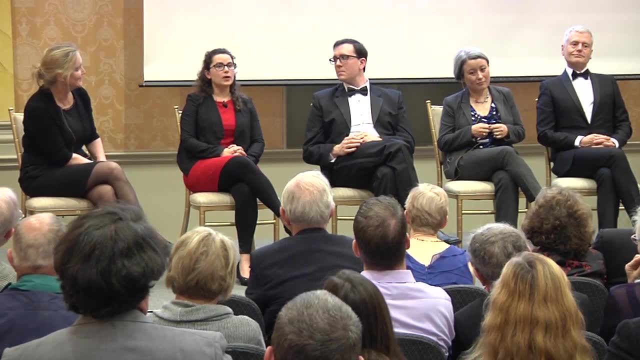 as well, so we need to understand the ages of these systems. Unfortunately, the Kepler- most of the Kepler planets- are very far away and very dim, so when we're pointing our photon bucket at these stars, they're not collecting enough, and certainly not enough that's shining. 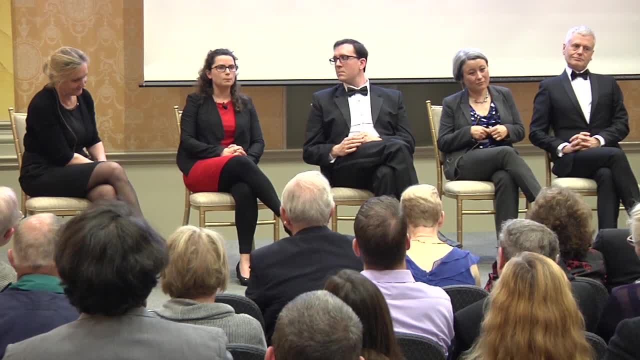 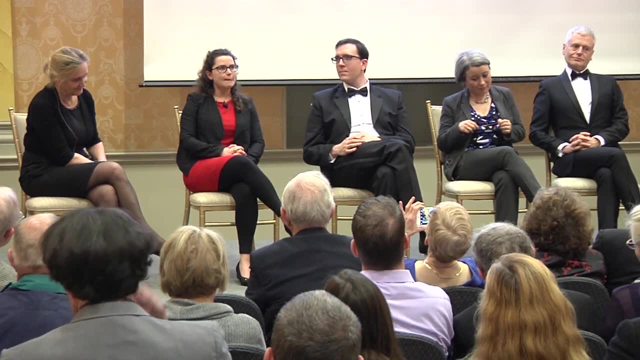 through those atmospheres. so the atmosphere is 1% on 1%. we're looking at a point source on a point source and we're trying to work out what the environment's like. So for the Kepler target it's very difficult to do. 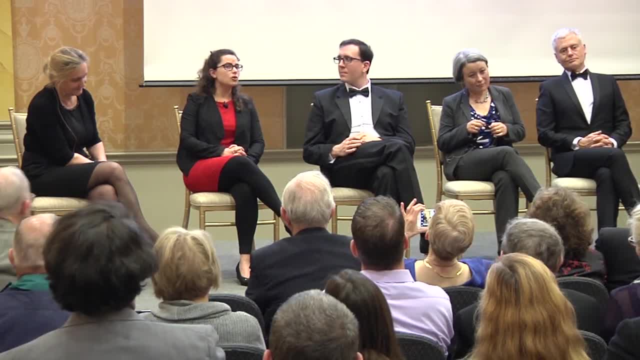 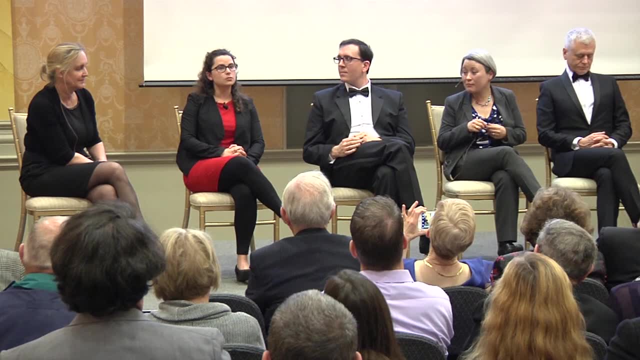 You'd need something like LUVOIR, which is why that kind of instrument is so important. that size of telescope, that kind of instrumentation that will be developed for that kind of telescope, is going to be amazing for these kinds of studies. But the M stars we're trying to really 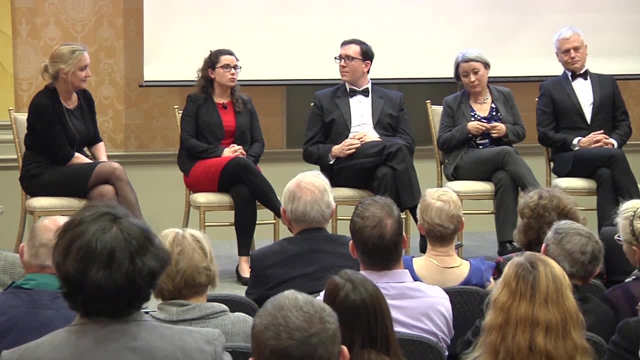 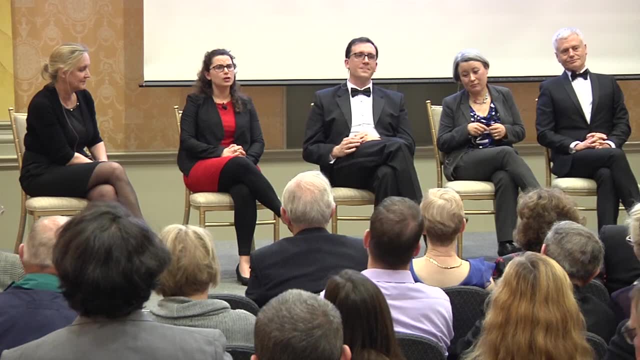 understand those and trying to understand the environments they do cause on these planets. because we know loads about our Sun- It's right there. We've even thrown a couple of things at it And we're trying to understand other stars and how that impacts. 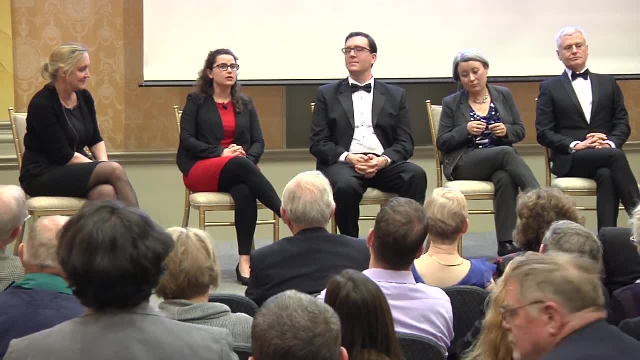 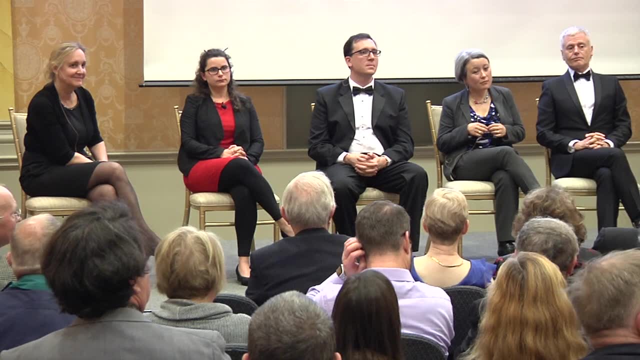 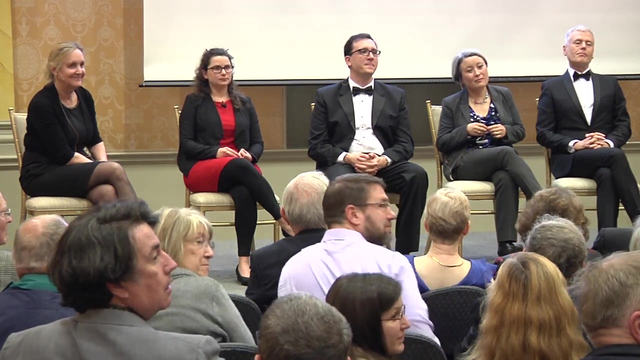 the possibility of life. So these types of stars and looking at different types of stars and types of planets is really key for that. I think we'll have one more question before we move on to Okay two. Thank you. I'm Joe Shulman. I'm a member, You know, Carl. 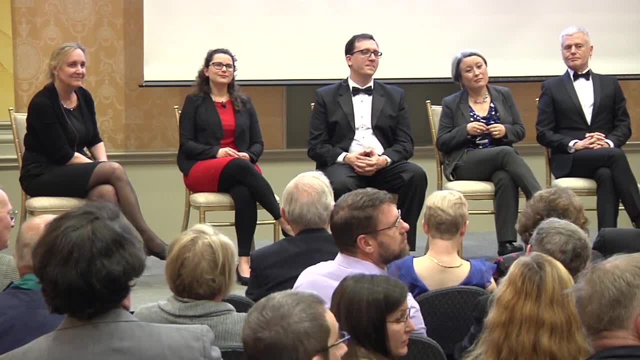 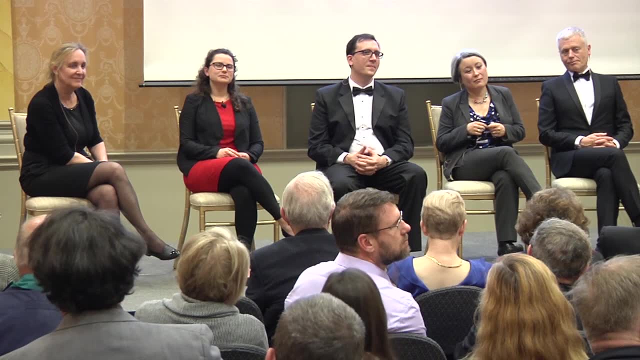 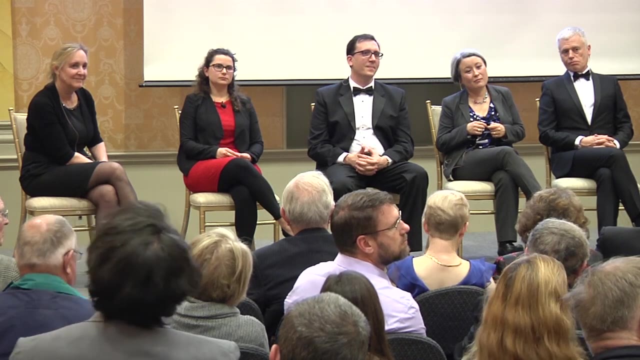 Merrill asked a key question, in my opinion. Imagine that you were. You had some imaging device way out in space And you wanted to look at the Earth, where we know there's life, And asked the question: how do you know there's life on Earth? 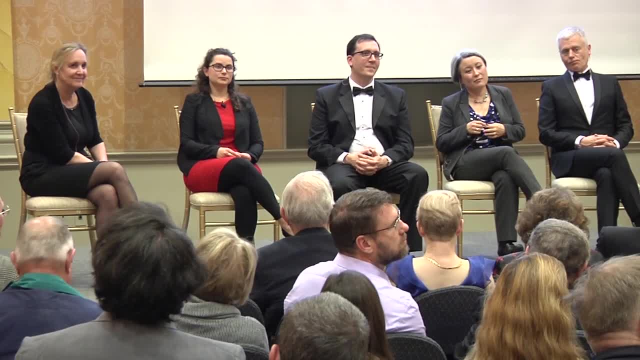 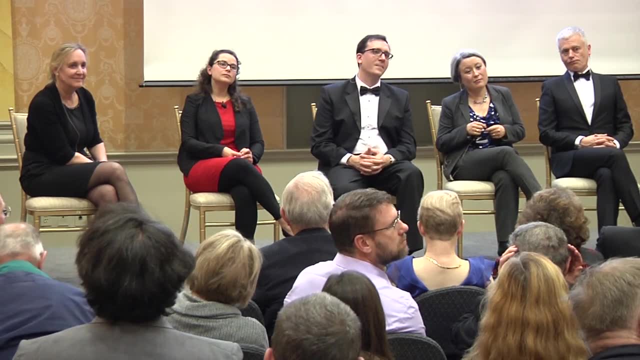 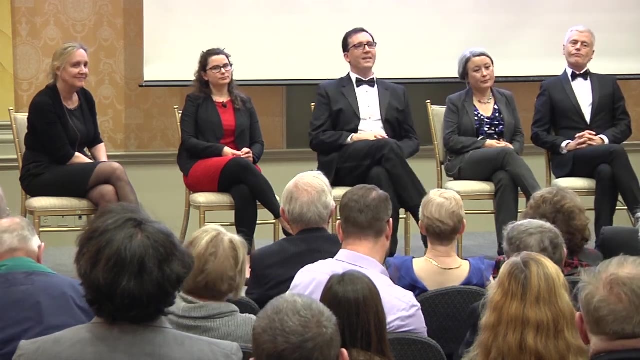 It seems to me that about the only marker you could think of- at least that I can think of, that for sure would tell you there's life on Earth- would be the spectrum of chlorophyll. And you know Because all these other things? 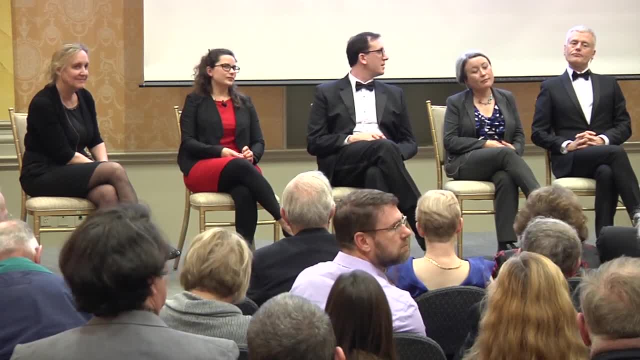 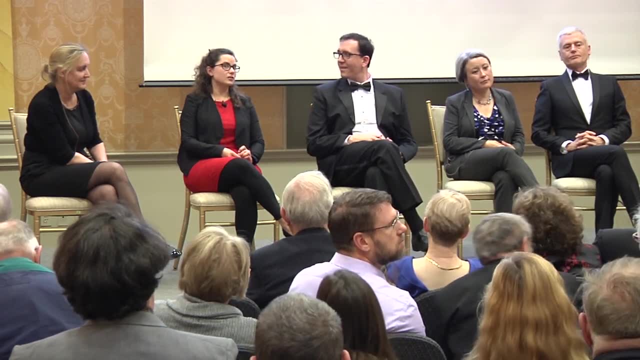 you know, can arise in all sorts of ways that have nothing to do with the proof of life. That's my question. So there have been studies of Earth as an exoplanet, Trying to look at, So we can look at, the Earth's light. 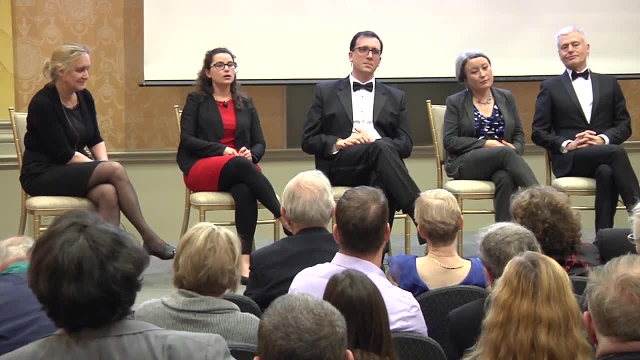 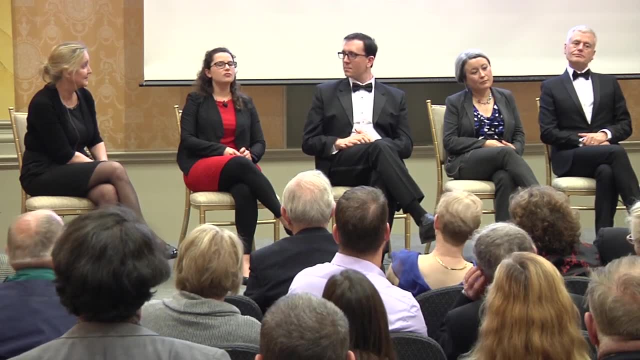 that's filtered through the atmosphere. by looking at the Moon as we eclipse the Moon, We can study the Earth's atmosphere in the same way. we're studying these exoplanet atmospheres And looking for Earth as an exoplanet, And a number of other things have been done. 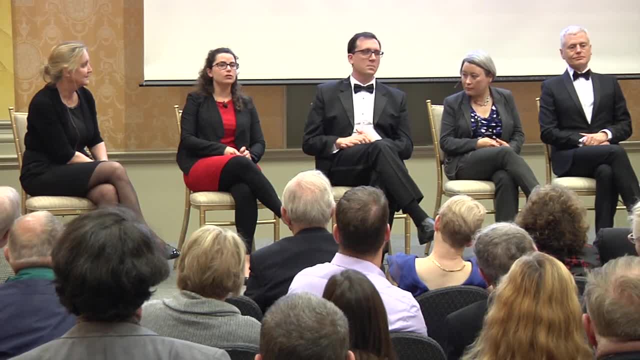 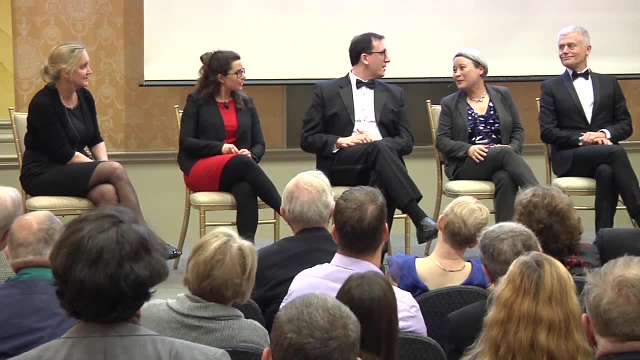 to that effect, trying to understand what our spectrum looks like on a global scale and how much we can resolve from that. Sean can probably talk more to the chlorophyll, but Can I just say my piece about the red edge: Go ahead, give the bad news. 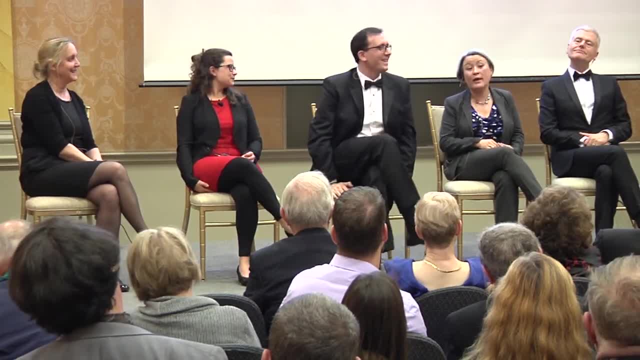 then I'll give the good news. I'm going to give the bad news on that one. Yeah, it would be great to detect the red edge, the photosynthetic red edge, spectral red edge. That would be fantastic. The problem is: 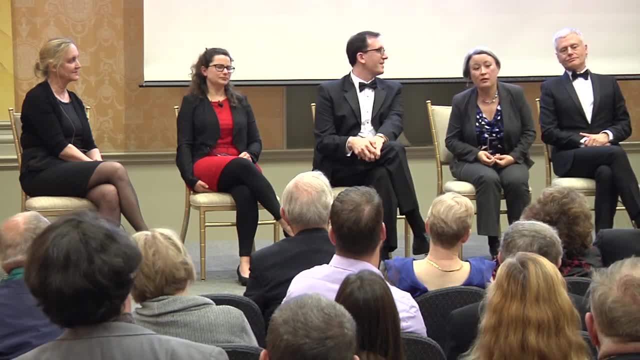 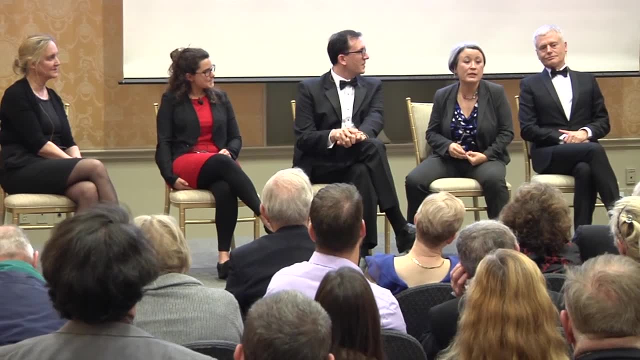 it's an extremely weak feature. It is observationally, probably pretty much. if we were looking at for that feature from interstellar distances, we just could never see it. I mean, you can't even see it in the Earth's shine. 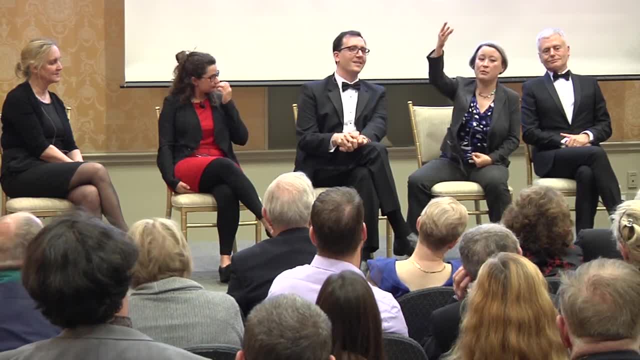 When the Earth's light- you know sunlight comes- hits the Earth, bounces up to the Moon, to the shadowed part of the Moon, bounces back down at the telescope. This is like a poor man's exoplanet spectrum. 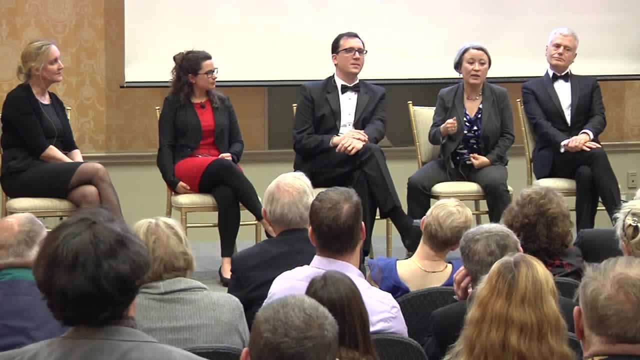 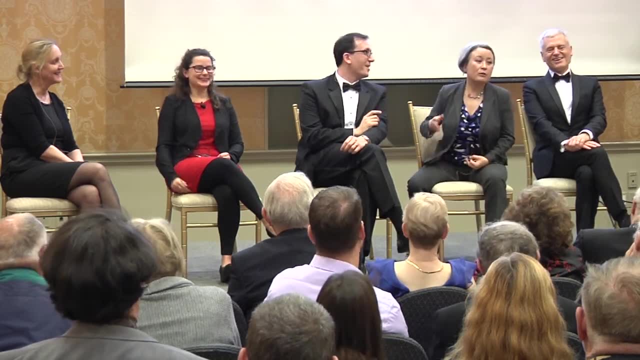 Even in those Earth's shine spectra, you can't see the red edge unless it's a clear day and Brazil is facing the Moon. So the only way. So you, really, only you, can really only see it. you would really only see it in. 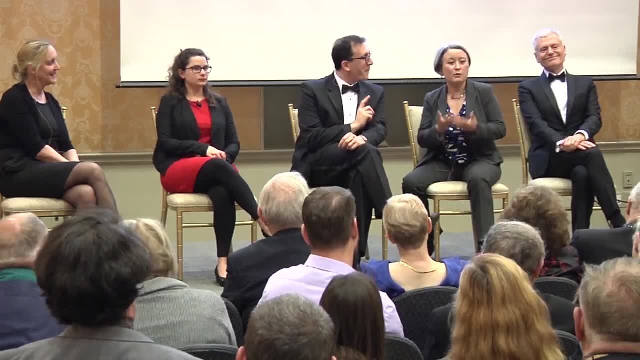 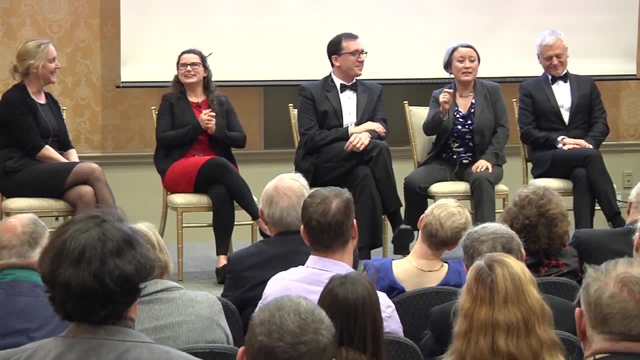 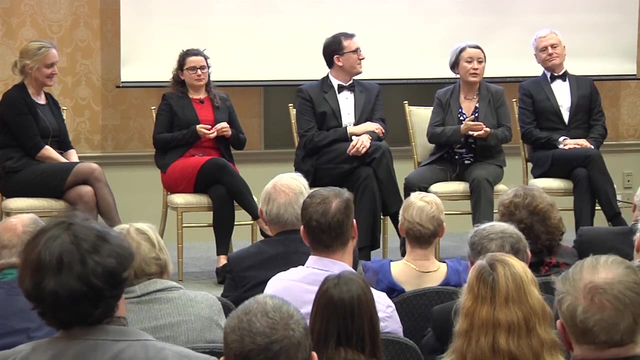 like some sort of jungle planet that was completely covered with vegetation. and even then So, and even then, there's no guarantee that it would be exactly at that pigment. that light absorbing pigment, would be at exactly the same wavelength as Earth's chlorophyll is at. 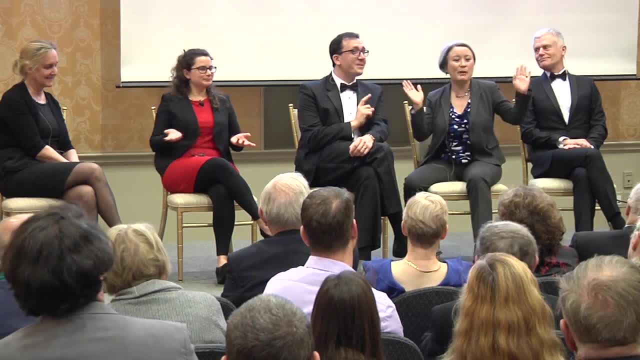 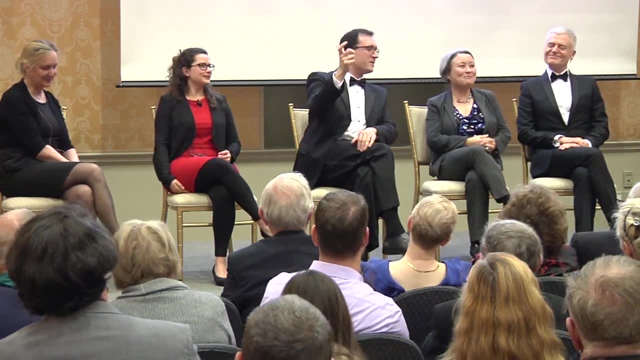 So how would you ever know? that's what you were looking at. So that's the bad news. But Brazil, the good news is sometimes Brazil does face the Moon. So that map I put up there where I said the planet spun underneath the 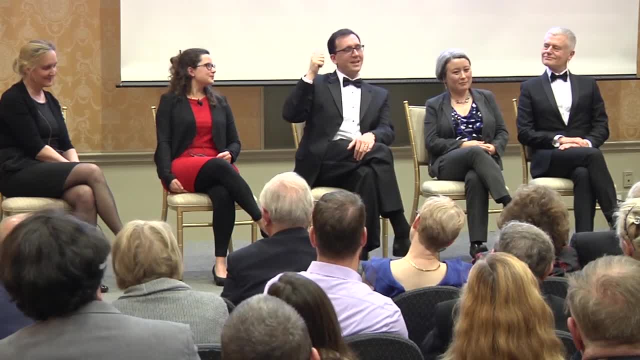 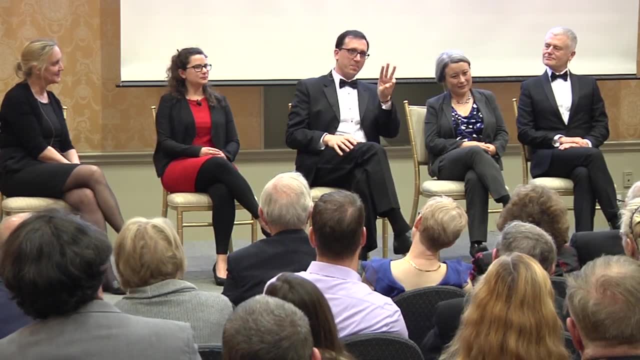 planetary spacecraft, the author of that paper. it did not put this in the paper, but he'll tell you over a beer that the three dominant signals in the data that he pulled out of the principal component analysis correlated to continents, oceans and clouds. 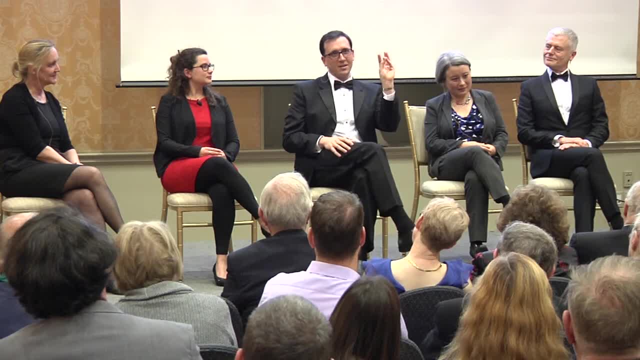 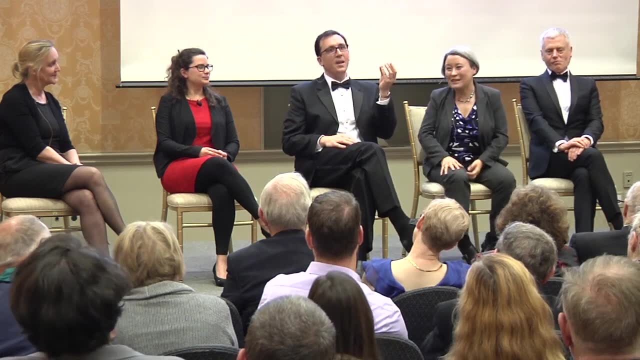 And that's what's in the paper. What's not in the paper is the fourth major signal, which he couldn't quite detect to a significant degree was actually a chlorophyll. It was a pigment signature Green, It was green Now. 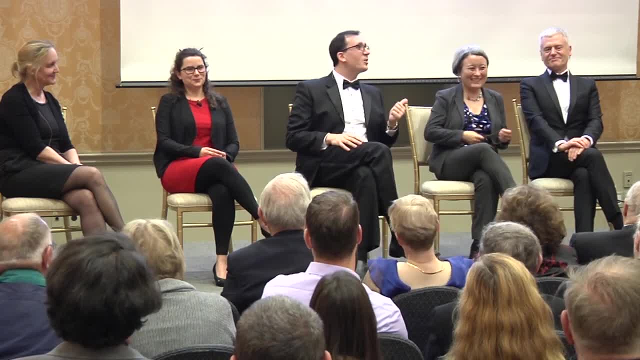 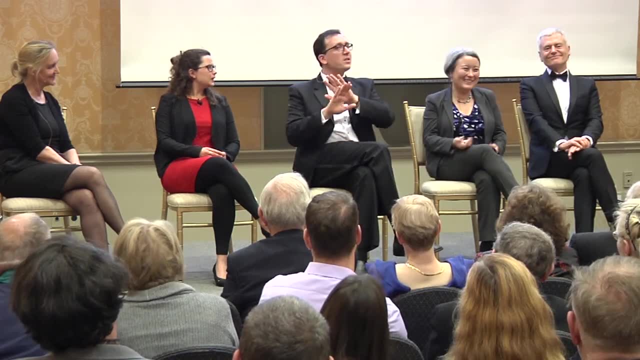 I think, because of the difficult, It wasn't chlorophyll, it was green, But it correlated to where chlorophyll exists on Earth, right, Yeah, And also the peak output of the Sun. Yes, So I think with all of this, it's not the thing you build the telescope around. No, But you want to. the telescope should be able to try to see that, because if you see the oxygen, you see the methane, you see the water, you see continents and oceans if you stare at it. 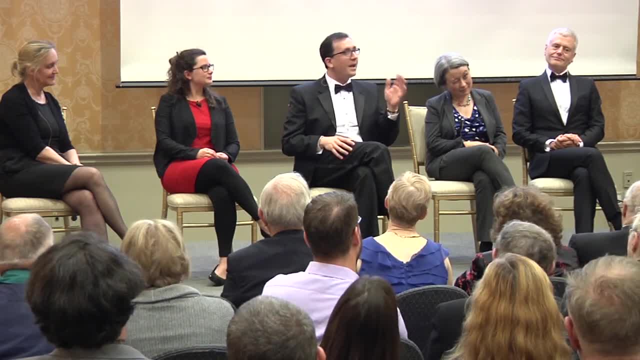 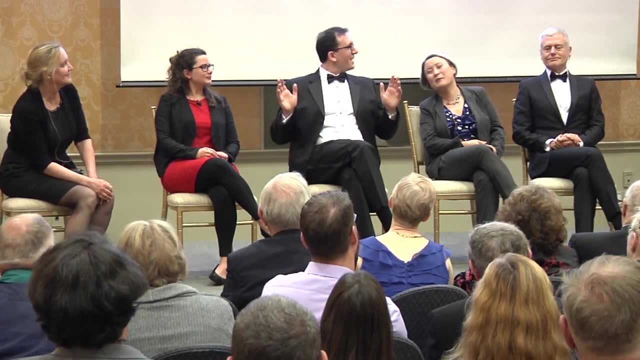 more and you start to see the difference of a red edge feature. I do think that's better than not having the red edge feature at all. personally, There are plenty of mineralogical species that have edges in their spectra too. Yes, there are. 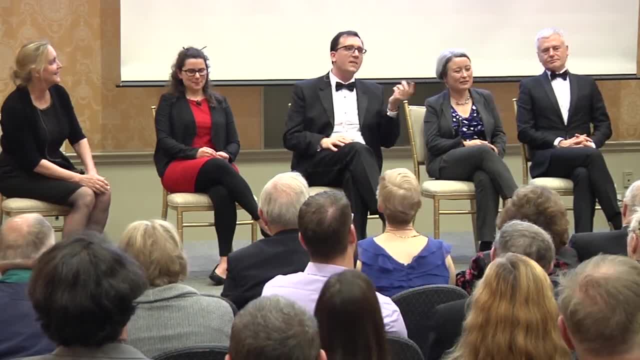 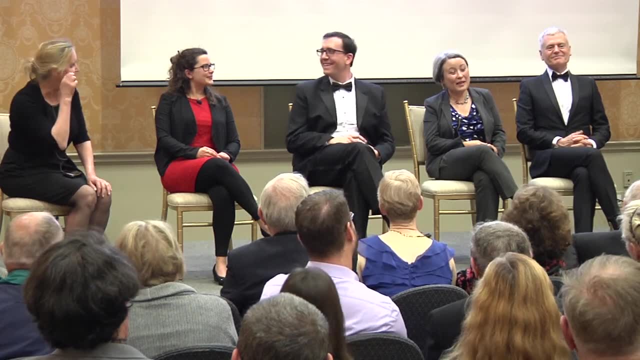 It's not the first thing you look for, but I think of it as a secondary biosignature. Clouds are really. Clouds are important. I really think it's a red herring. I genuinely think it's actually a red herring. 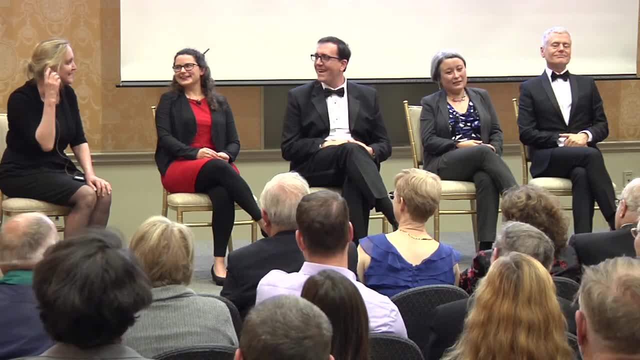 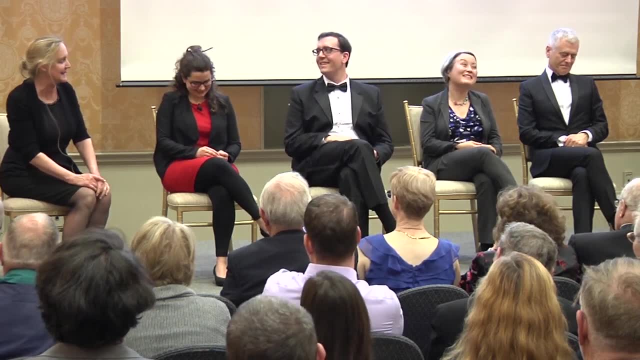 I want to just bring up, just to remind you of the history of exoplanets, when in the early 1990s, people said: this is too hard, we're not going to find planets. they probably don't exist around other stars. 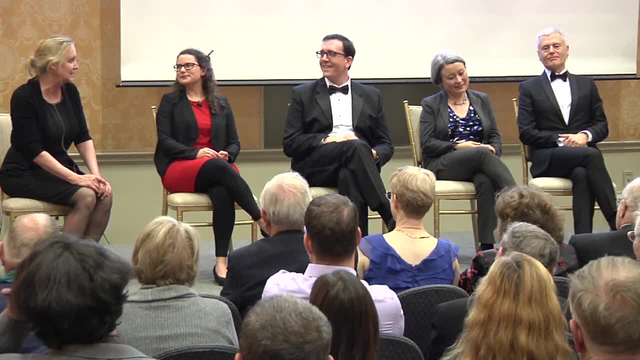 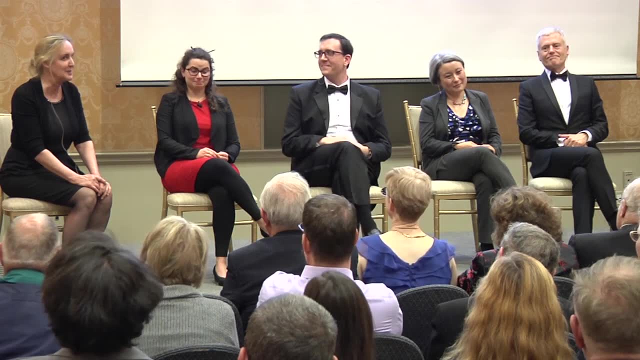 and what we found just completely revolutionized the way that we look. So right now we're going into this with a bias of what we think life might be like. We could be completely shocked. it could be much harder than we expect and it could be much easier than we expect. 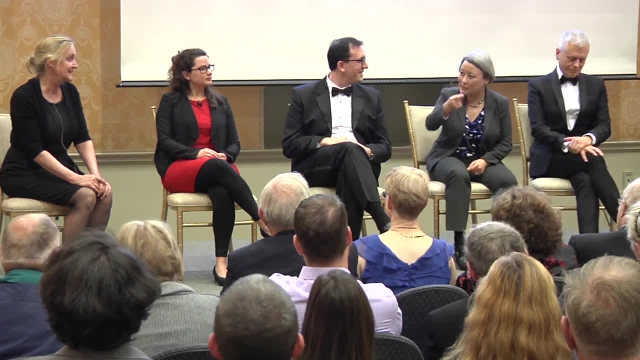 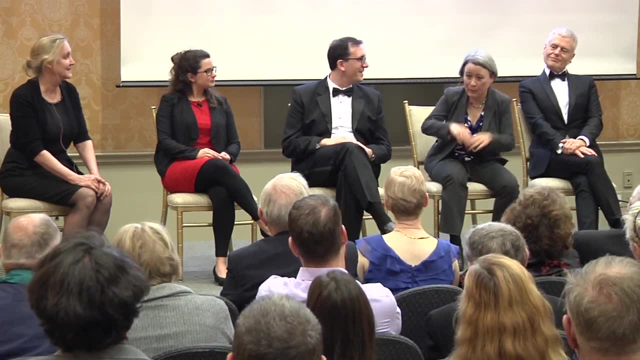 but we have to look. The problem with this particular one is that we are biased on both sides. We have it on Earth. Your bias is that we have it on Earth. It's a sign of life on Earth. My bias is, yeah, but we can't see it even. 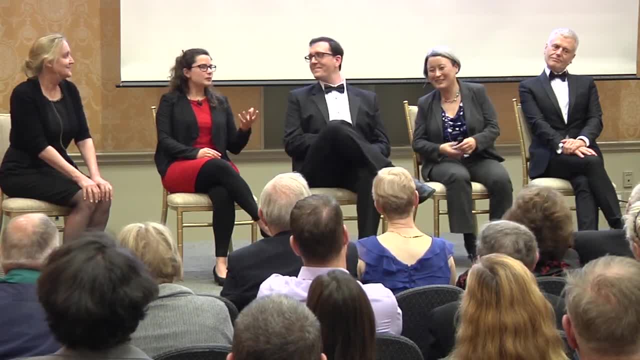 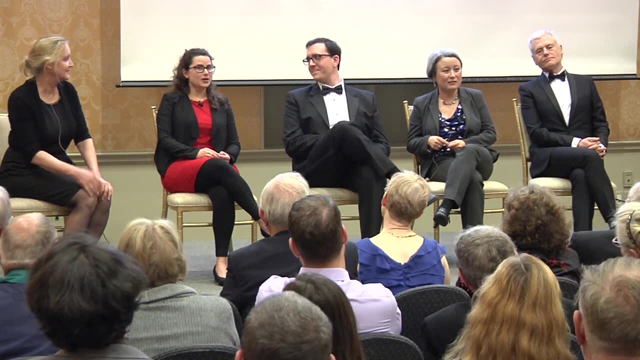 when we're looking at the Earth. So we are both still Earth-focused on this. I mean, this comes back to what Sean was saying about we need to put simulations which can't make biological Earths. We need to understand how to do that and we've 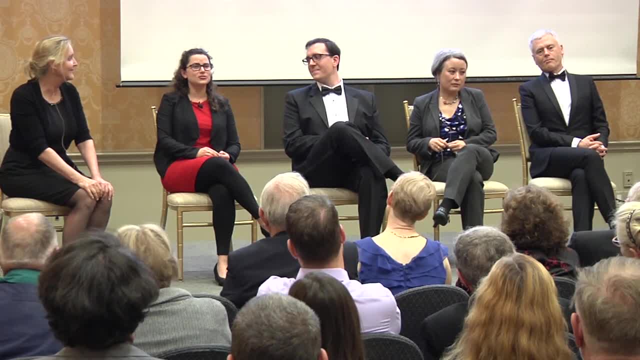 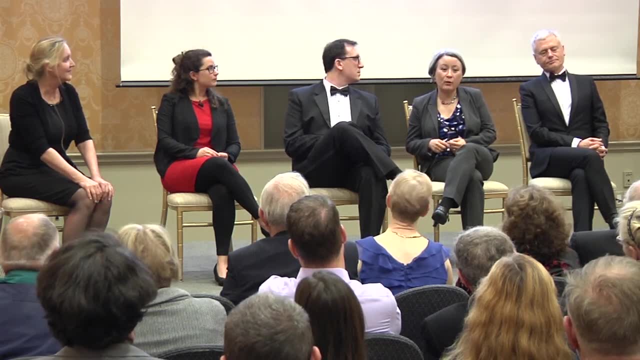 got to be asking the questions without those biases which are just inherent in our brains from birth. It's tough, It's a real tough thing to do. That is a generally fascinating question. We have no idea what a habitable planet that's not inhabited. 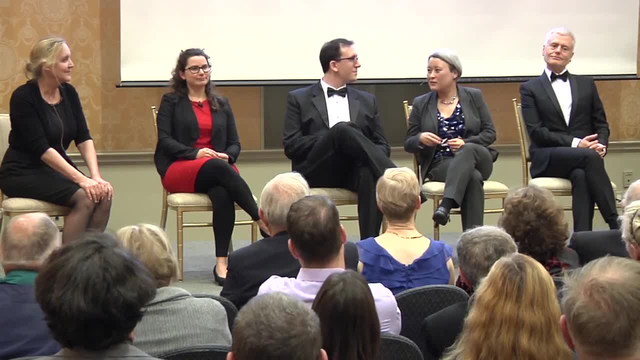 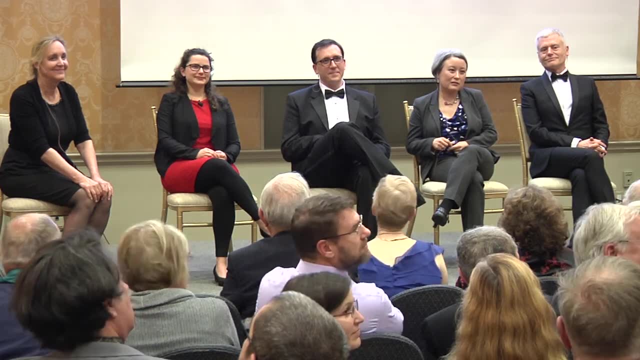 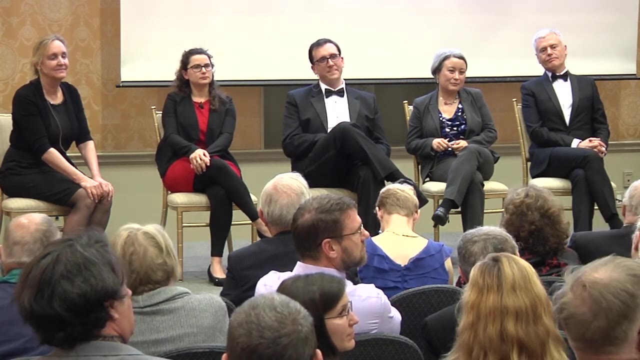 actually looks like. Hi, I'm Jim McCormick and I am a member, So last question: feel free to just say no. There's no doubt that there's a lot of pure science in what you're doing, but where you are, you have to be. 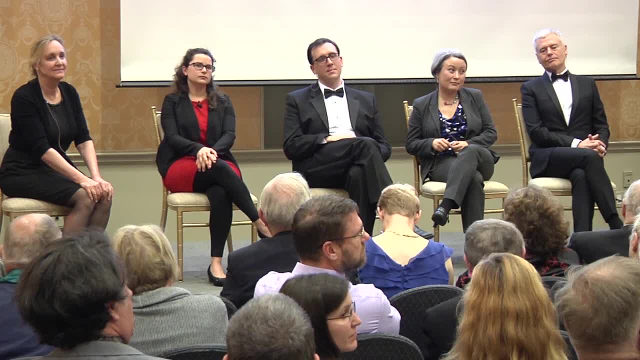 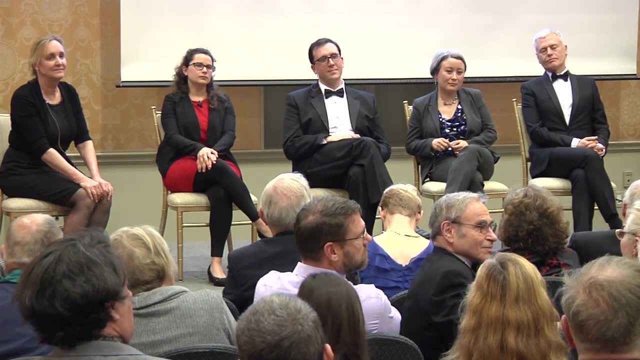 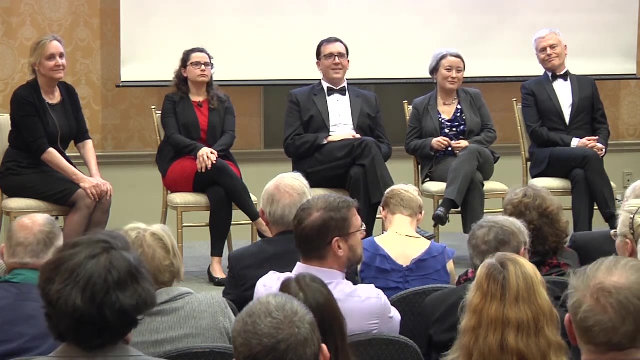 just really in tuned to budget, to aspiration, right. There are social impacts on what you do in social significance, which is why you do what you do. Can you say something not obvious about the social impact on what you do, whether it's science? 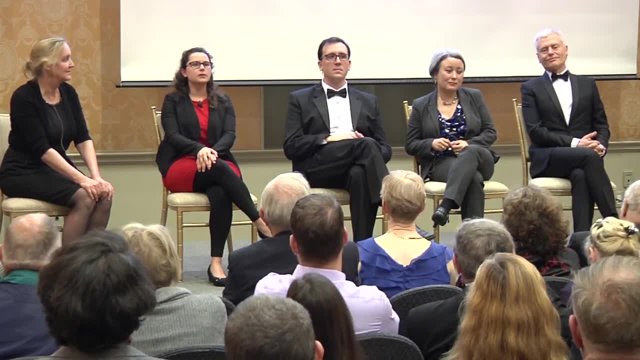 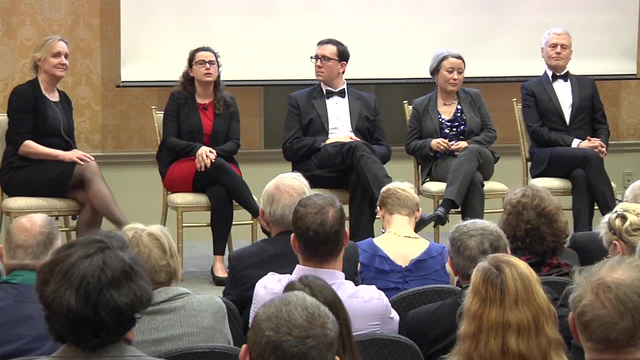 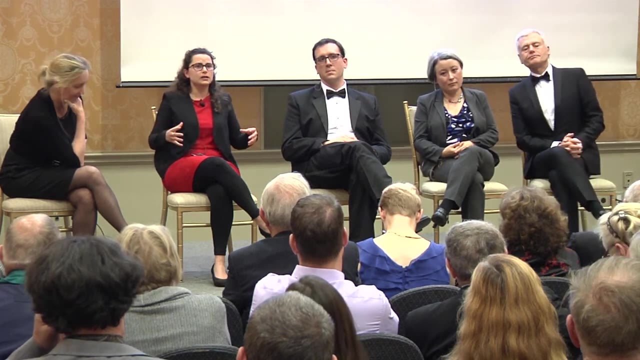 national, global. This is an inspiring topic. It's the first question that man has ever had looking up at the heavens. That's how we were defined: by looking up at the stars and trying to really understand and use them to live on this planet. 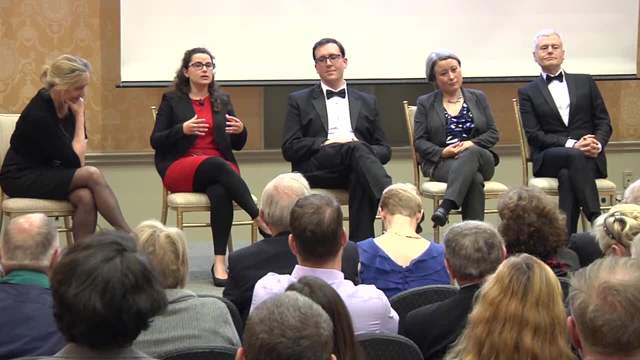 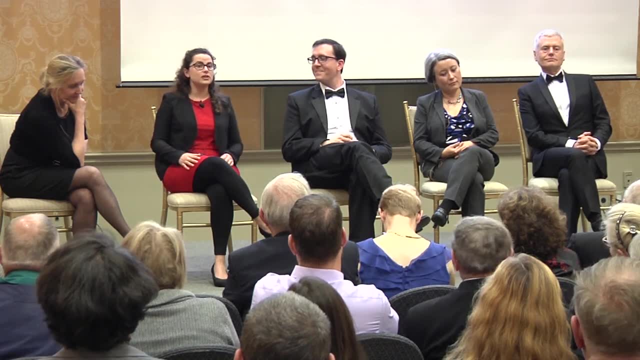 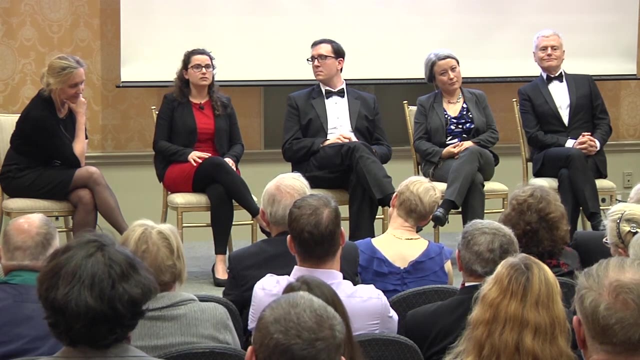 This is an inspiring topic and it generates people and young children to go into science, to understand more, to go into engineering. build that telescope. The people that are building the telescopes- and Mark was telling me this earlier- they're so excited to be just. 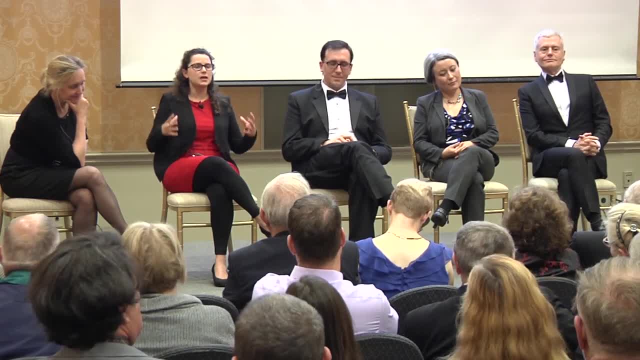 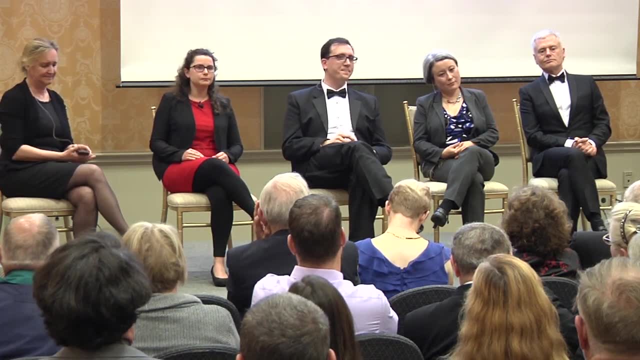 part of this big big mission, this big question that we all have inside of us and that is so important, and I don't think that should be ever understated. But what if you turned it around? and what if actually? 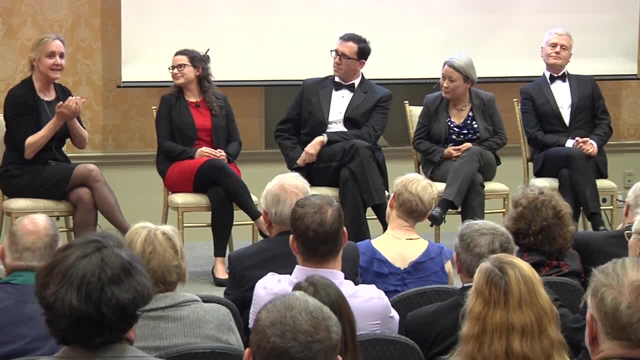 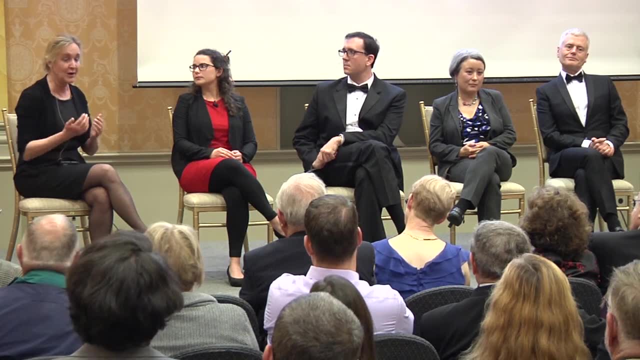 I could. I have the answer in the back of the book and I can tell you that among the 200 closest stars, that 75 of them have planets with life on them, And I know that that's true. Would we just not bother to look? 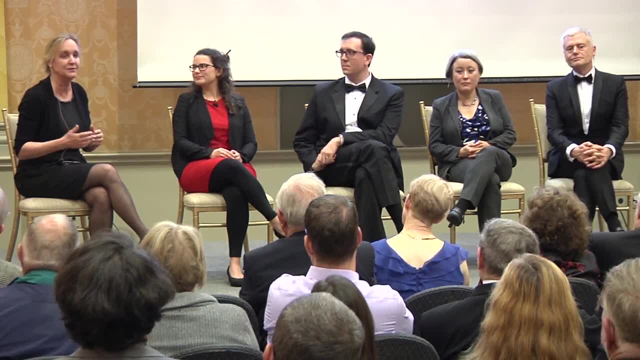 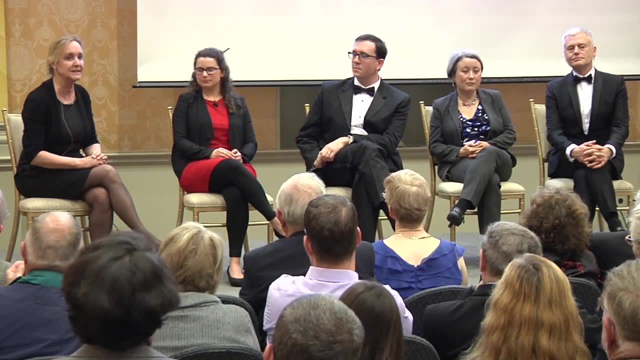 So for some people maybe the answer is yes. Maybe that's not what they're interested in, But I think for most of humanity that it's just too compelling and too interesting. If it's really there, we have to find out. 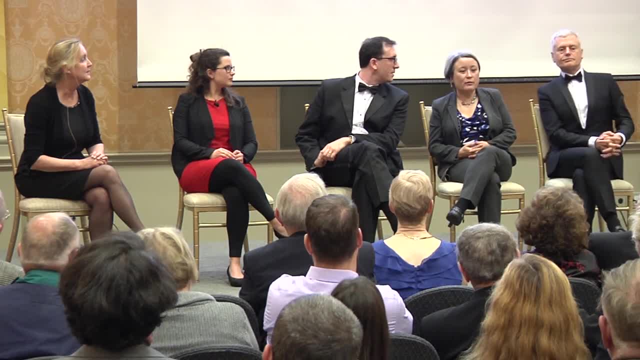 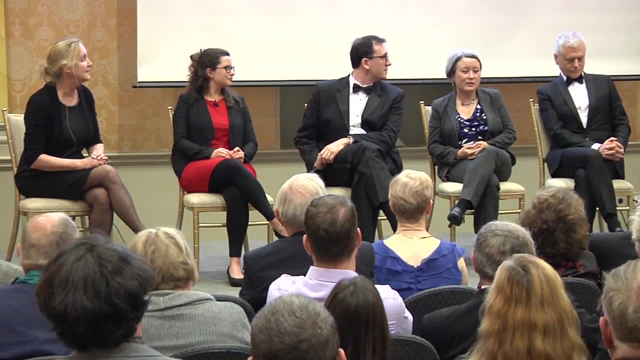 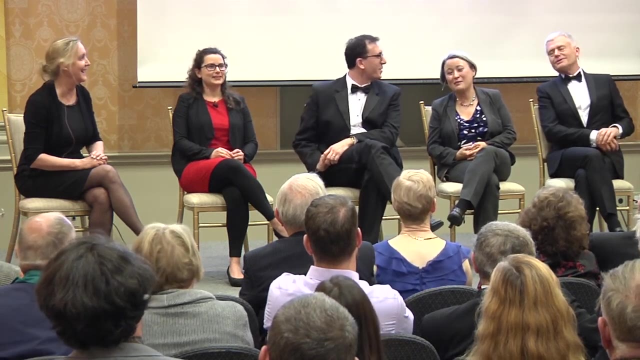 And I guess I'll add too that I have a view that, like I don't intend, this species goes out when the sun does. You know, someday we need to find new homes, Ones that are nicer than Mars. Mars ain't bad. Wow, That is a big thought For me. I want to know how planets work, and I want to know how rocky planets work, and I think that the more sample size we get in understanding how especially rocky planets that could harbor life work, I want to know how. 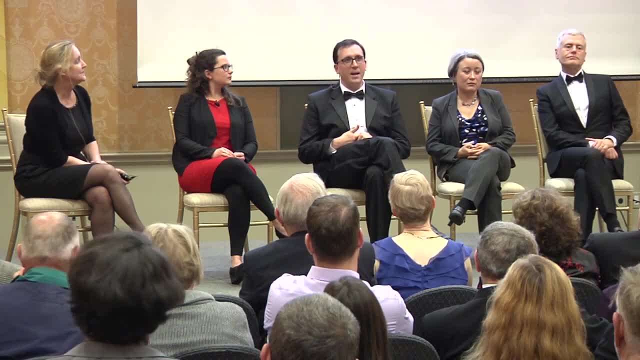 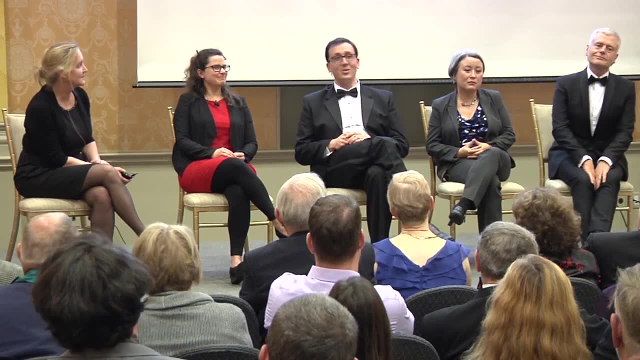 those things operate. We're finding out a lot already about how planetary systems work. Hannah's finding out a lot about how gas giants work and is going to be finding out about whatever increasingly smaller planets do and how they work. But eventually I want to know, like how? 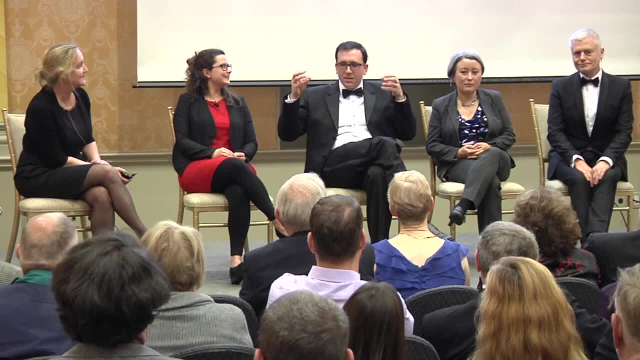 every time there's like one of these planets, like we have these nerdy conversations at lunch, like oh, that's going to test the carbonate silicate feedback cycle, which is like a major Earth Sciences hypothesis, I want to. 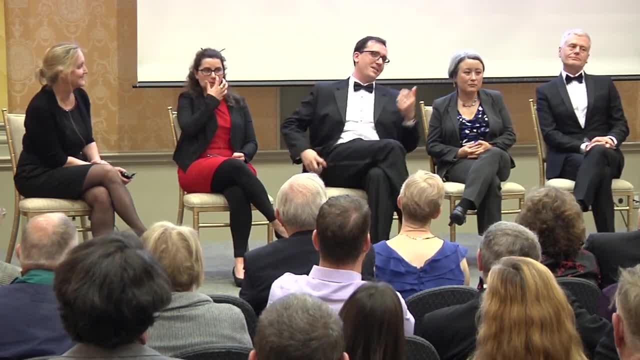 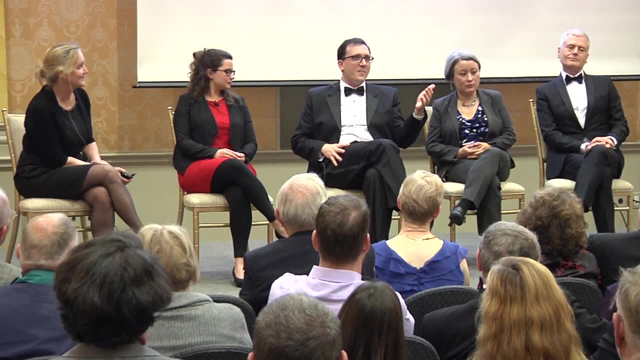 test that on these exoplanets And every other hypothesis we have. The secret to this is: you know, 50 years from now, the press headlines will be written about whether or not we found life, But I think all the scientists will be. 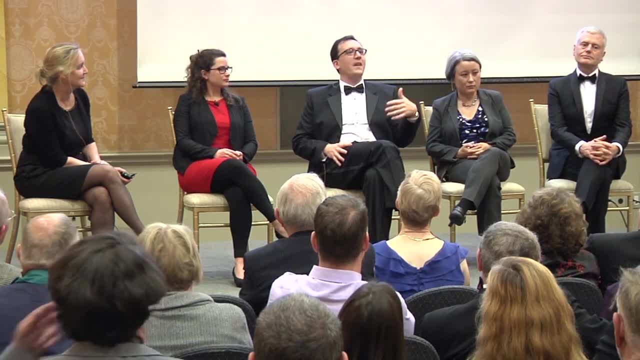 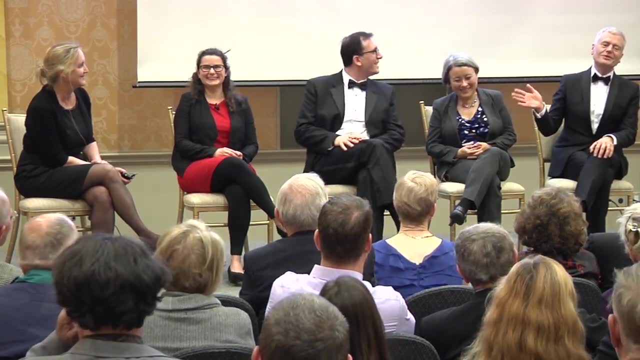 remembering this as the comparative planetology mission that got us 500 worlds to compare our own solar system against. So you've seen how engaged these folks get in their subjects At Goddard. you know we do hundreds of those every year, for you know. 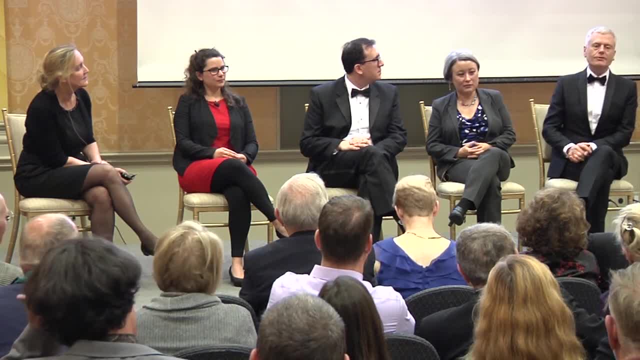 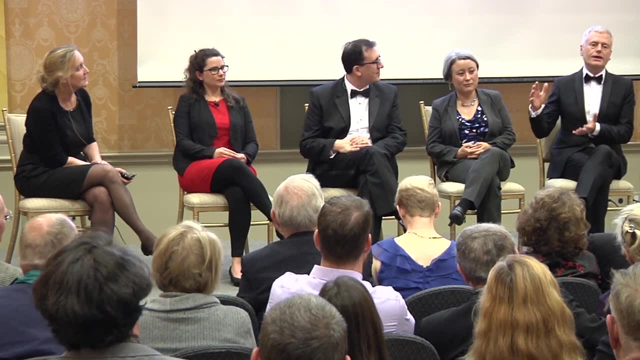 various STEM programs, kids from five years old to 15.. And the one thing they all ask about is this. So it's just the best book for getting kids engaged in science and starting to think about the world they live in and the universe they live in. 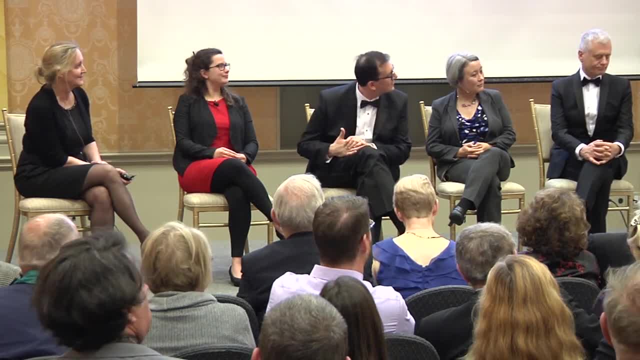 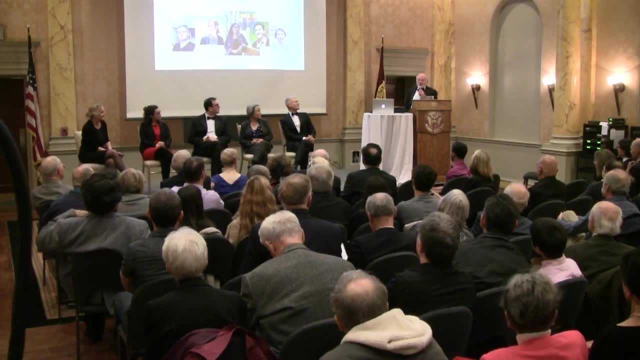 So I'm going to add a note to that. I think we all think the great thing about science is what we know, but actually the really great thing about science is what we don't know and what we find out, And I'll quote Frank Zappa. 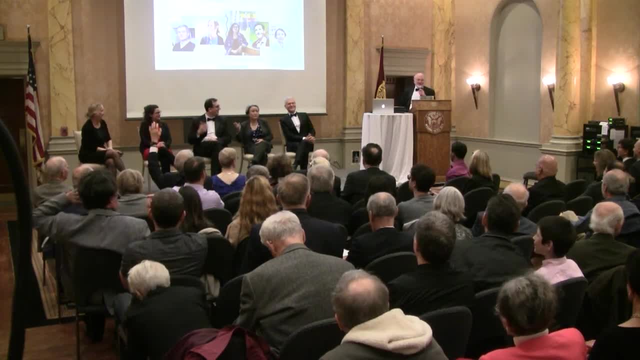 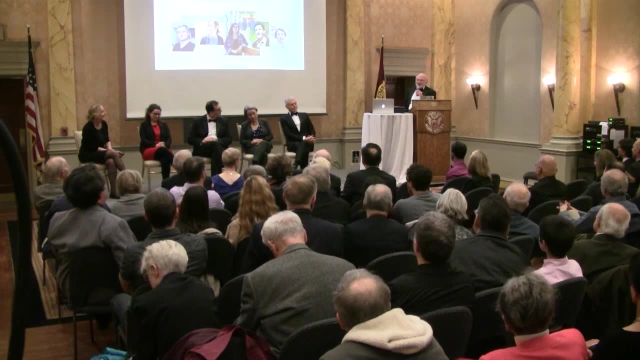 How many of you know who Frank Zappa is? Okay, most people know Frank Zappa as a rock and roll musician and a little bit of a philosopher, And he quoted Edgar Perez, I think, who said: the contemporary composer refuses to die. 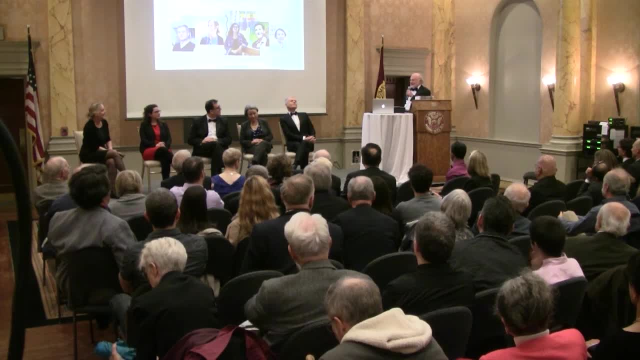 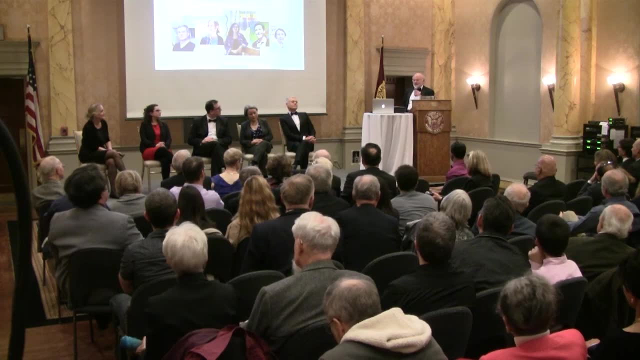 And I'd say the contemporary scientist refuses to die, And what he was getting at was that you always have the contemporary scientist or artist who's after something that the rest of us don't really get Because we're not out there on the edge. 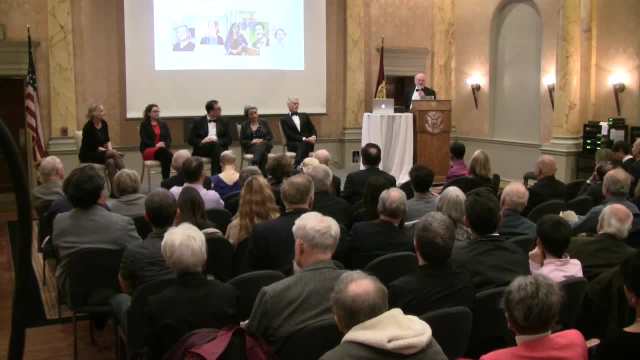 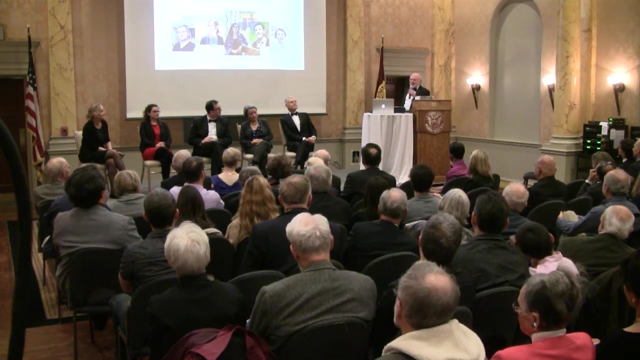 And this is what creates knowledge and creates beauty, And that in and of itself is more important, I think, than an engineering project that might be designed to achieve some practical goal. So I think, in the end, this is how we create our future, And there's really probably. 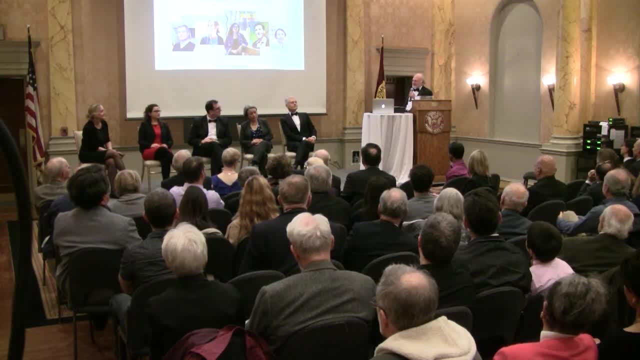 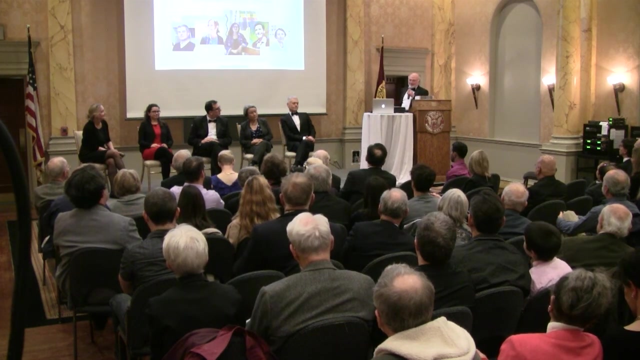 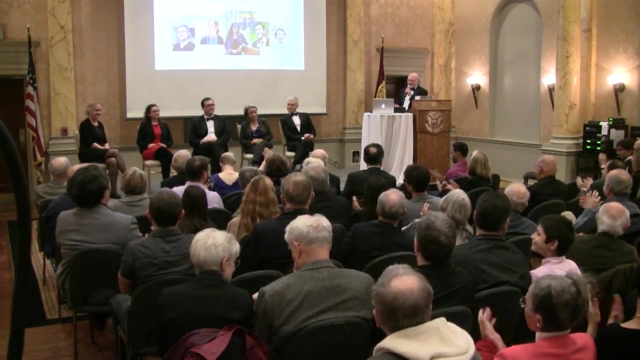 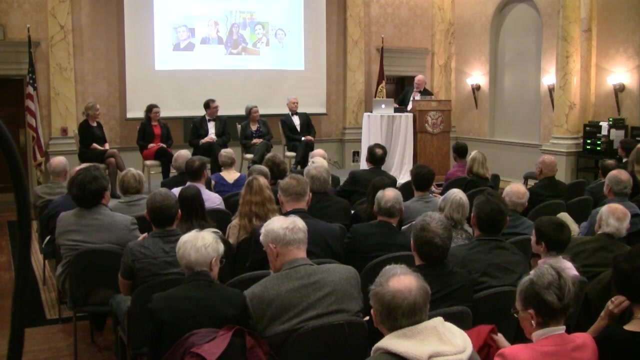 no more interesting question than are we alone? And I think I agree with Deborah- There's probably a lot of life out there And there's a lot to be learned by looking for it. So I'd like to thank our speakers Before I let them escape. I have to. 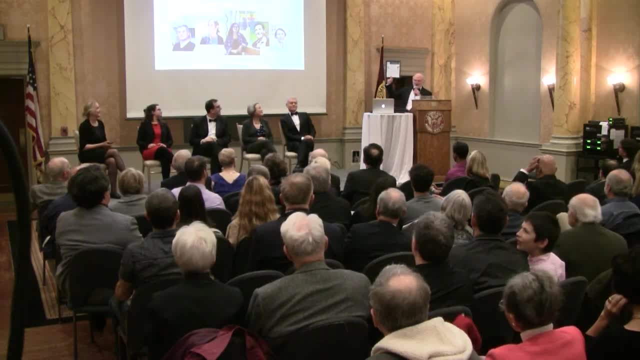 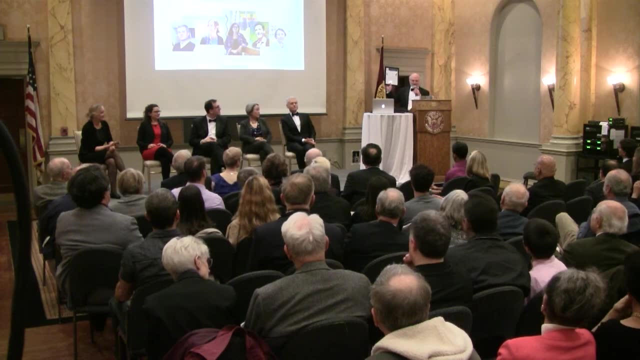 give them a little present to thank them for their time and their expertise and for opening up new worlds for us. And that is a framed copy of the announcement of this Joseph Henry lecture. And I have one for each of them Which I'll give them in a minute. 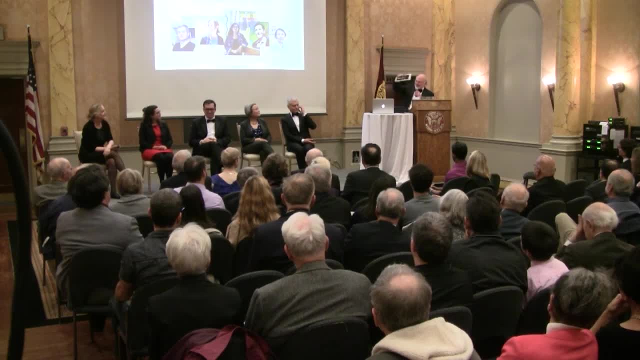 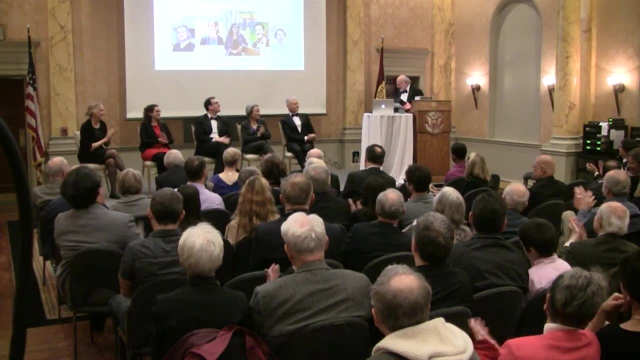 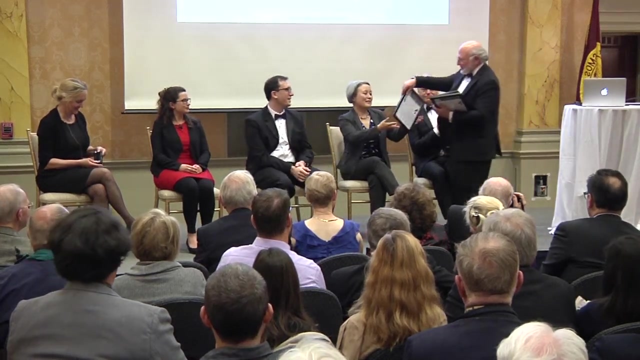 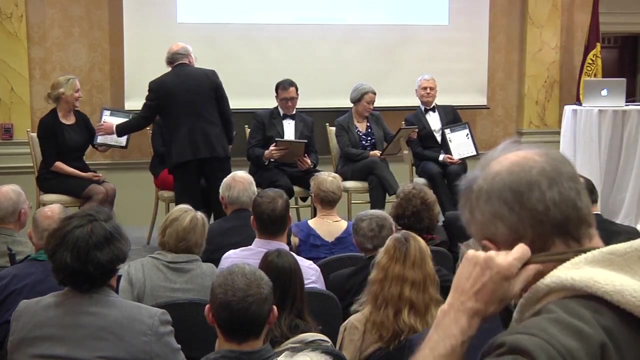 And I also have a copy of the volume on, Since they're all members now And signed by me, So it's a special one. Thank you, Thank you, Thank you very much, Thank you. So, if you can hold it, facing the: 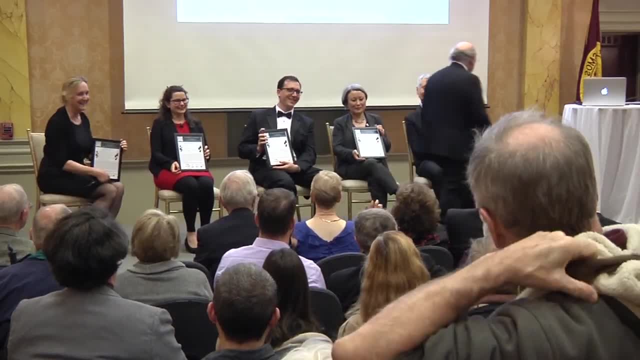 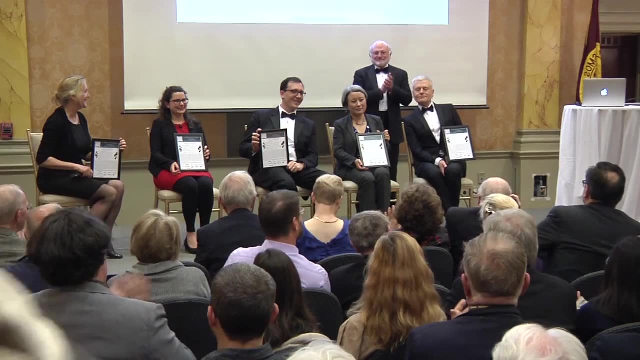 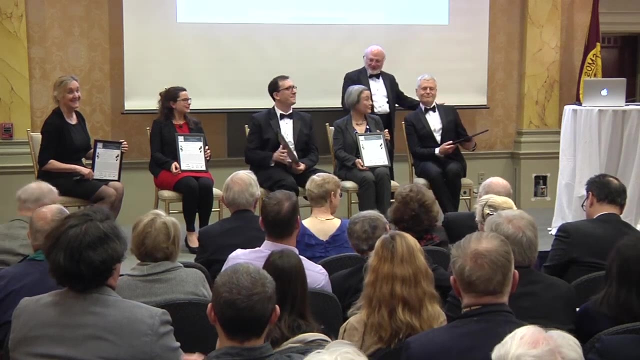 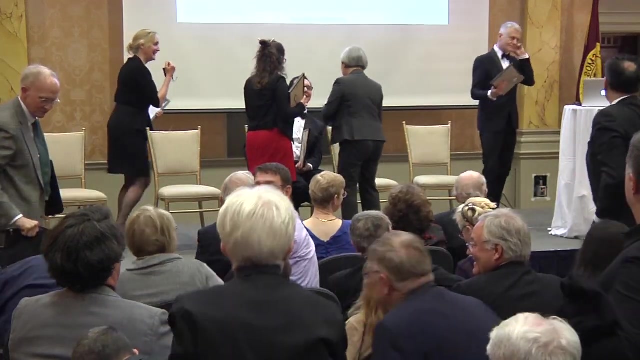 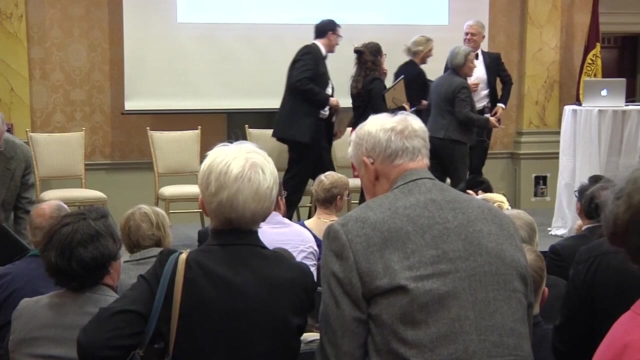 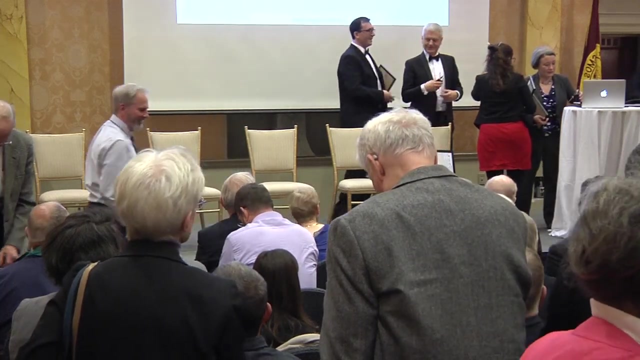 right, Wow. Before you go, there are a few closing announcements. First and foremost, thank you to all of our members, sponsors and supporters. If you're not a member, please apply for membership, Which is easy to do: Just go to our website. 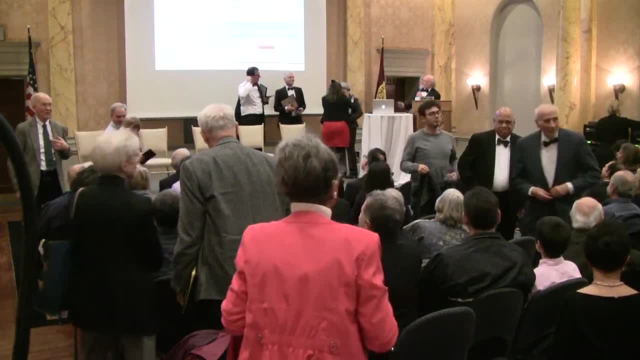 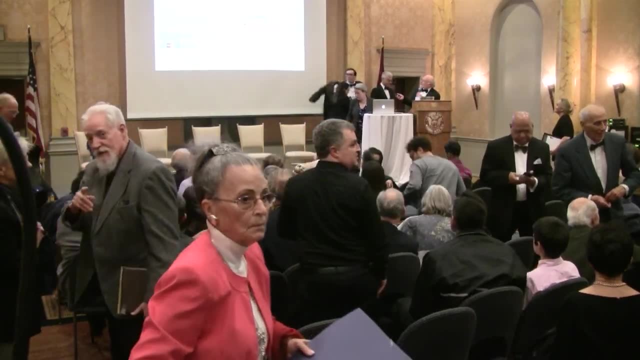 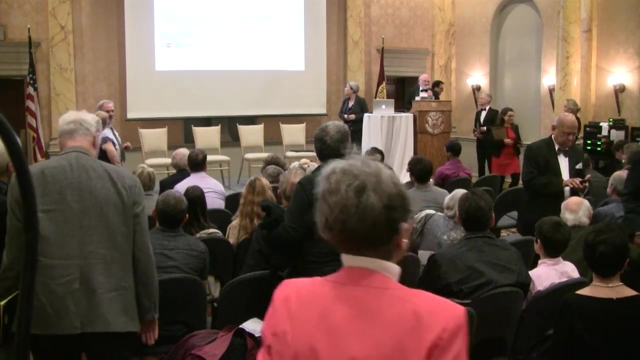 and click on the membership button, And that will bring up a screen. Fill out the form and hit the submit button, Which will bring up the dread PayPal screen. So just ignore all these references to PayPal, because PayPal is just serving as our merchant bank to process your payment.